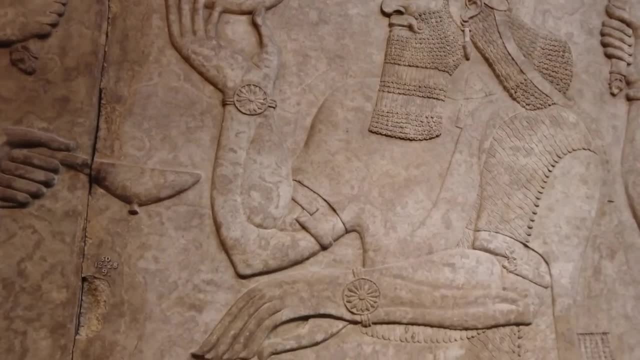 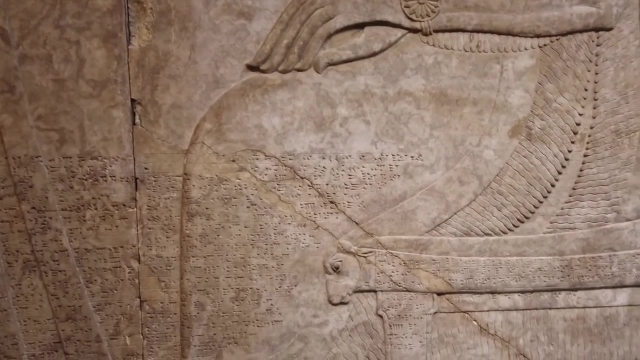 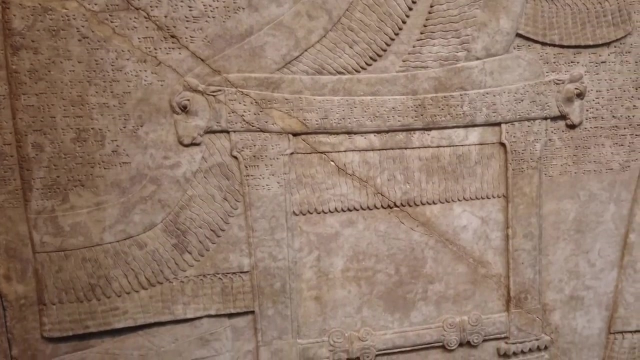 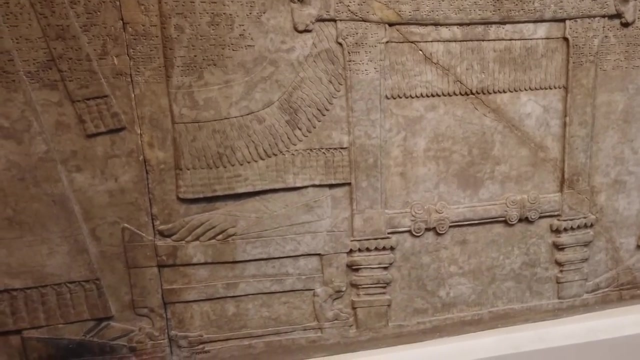 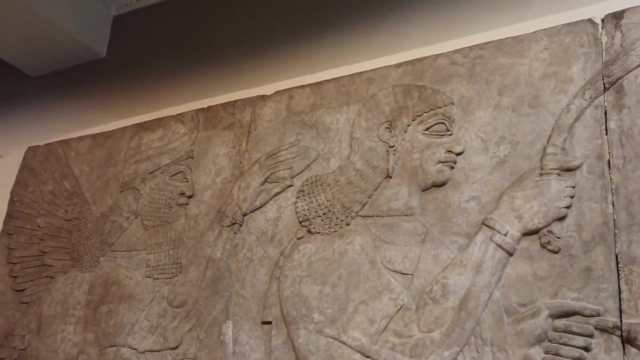 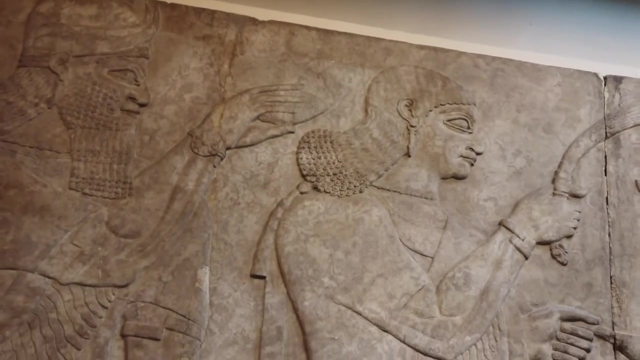 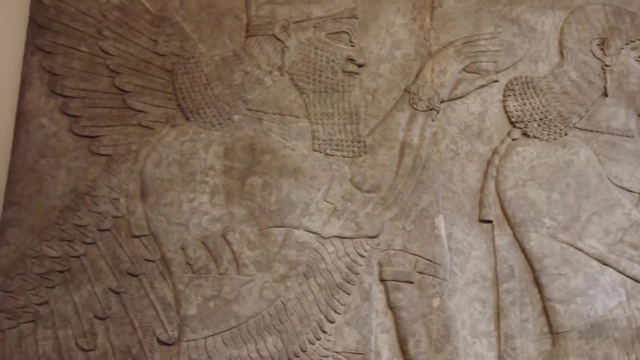 Thank you for watching. through. the Old Testament and the nascent field of Near Eastern studies had unraveled the enigma of the Akkadian language that was widely used throughout the region in ancient times, But the discovery of the Sumerian brought to light the existence of the Sumerian culture. which was the oldest of all the Mesopotamian cultures, Although the Sumerians continued to get second or even third billing compared to the Babylonians and Assyrians, perhaps because they never built an empire as great as the Assyrians or established a city as enduring and great as 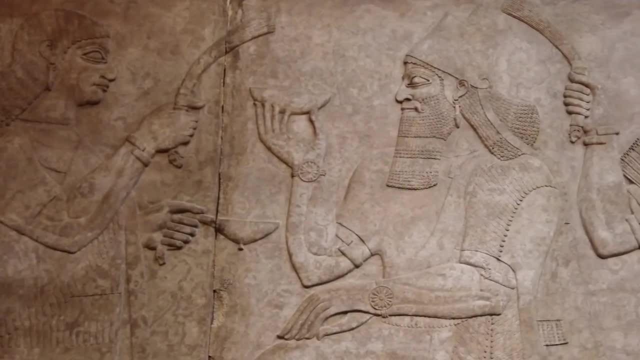 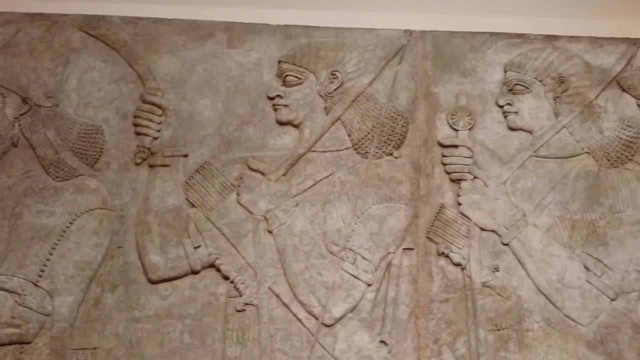 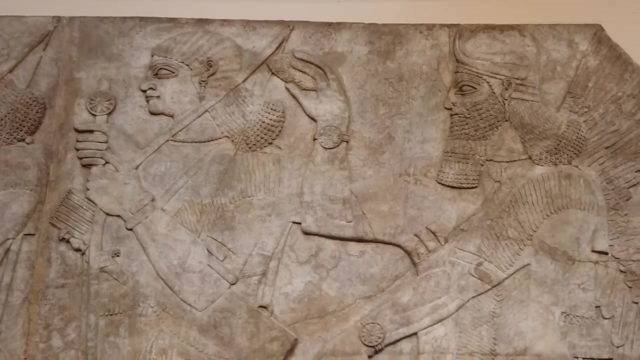 Babylon. they were the people who provided the template of civilization that all later Mesopotamians built upon. The Sumerians are credited with being the first people to invent writing, libraries, cities and schools in Mesopotamia, and many would argue that they 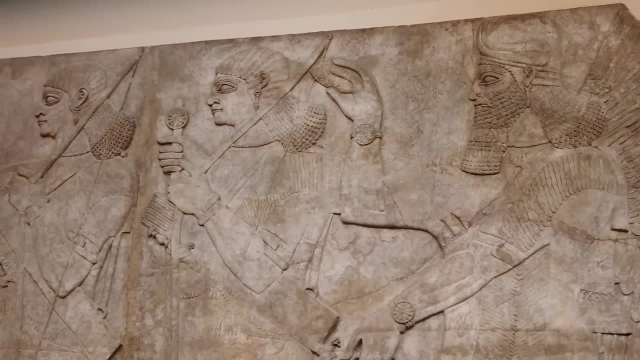 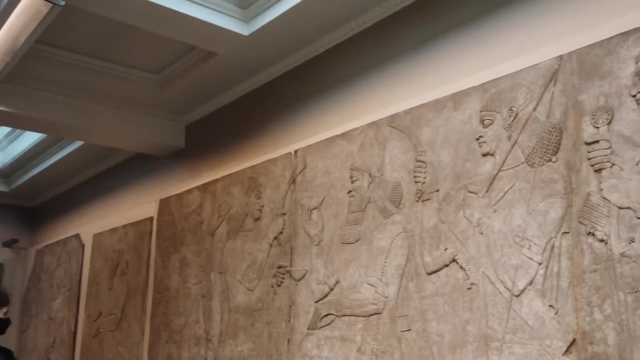 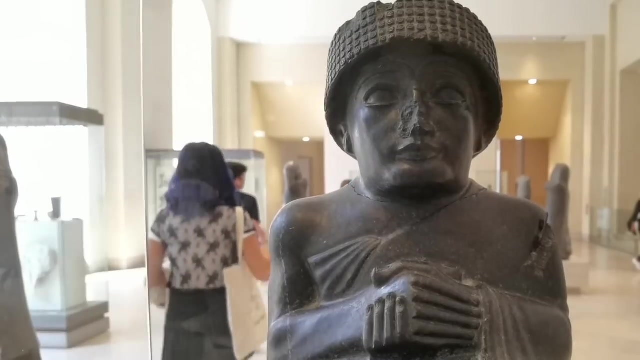 were the first people to create and do these things anywhere in the world. For a people so great, it is unfortunate that their accomplishments and contributions, not only to Mesopotamian civilization but to civilization in general, largely go unnoticed by the majority of the public. 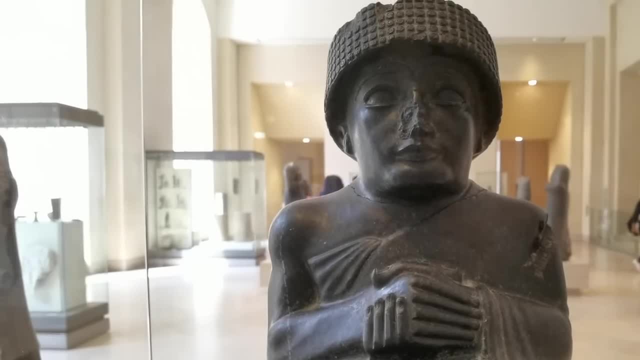 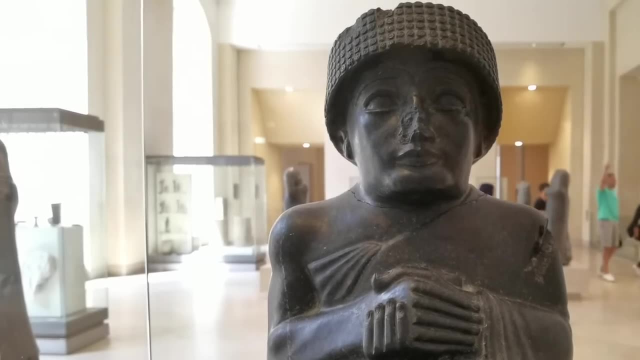 They gradually entered the historical record, establishing a fine civilization, and then slowly submerged into the cultural patchwork of their surroundings. They also never suffered a great and sudden collapse like other peoples of the ancient Near East, such as the Hittites- Assyrians. 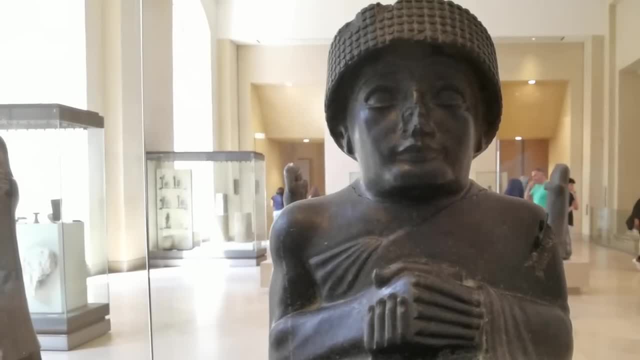 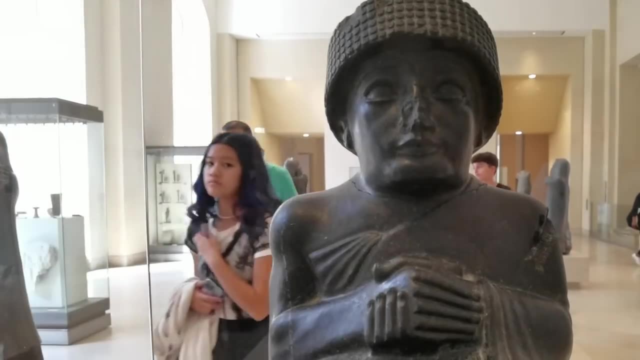 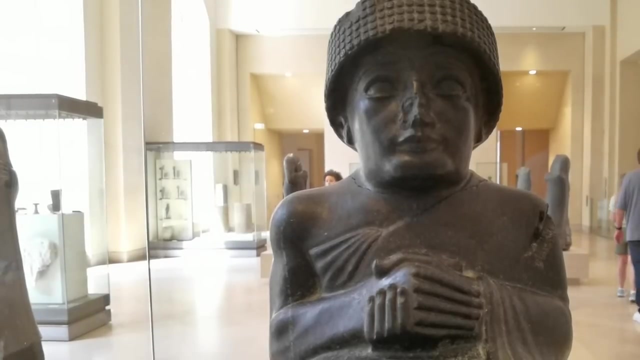 and Neobites. A close examination of Sumerian culture and chronology reveals that the Sumerians set the cultural tone in Mesopotamia for several centuries in the realms of politics and government, art, literature and religion. Even today, the world owes the Sumerians a tremendous amount. 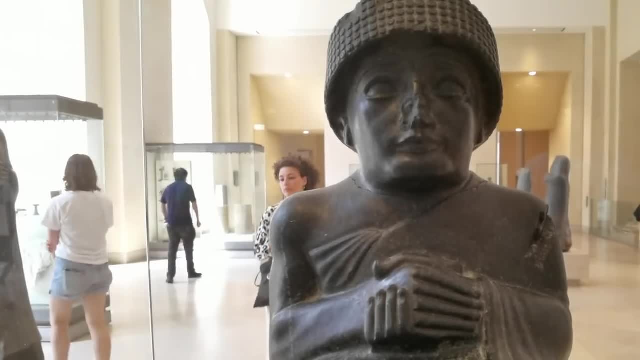 When Western Europe was still in a stone age. it was the Sumerians who invented writing and the wheel, divided time into minutes and seconds, tamed nature and built a new world. The Sumerians built gigantic cities, They embraced culture and the arts, and their caravans crossed the desert. 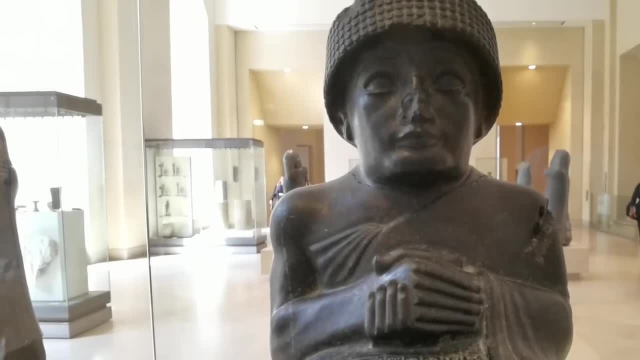 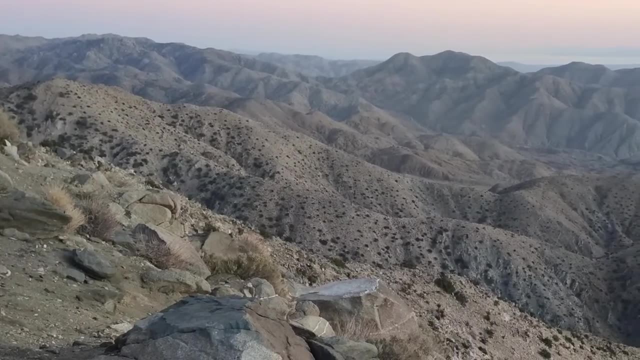 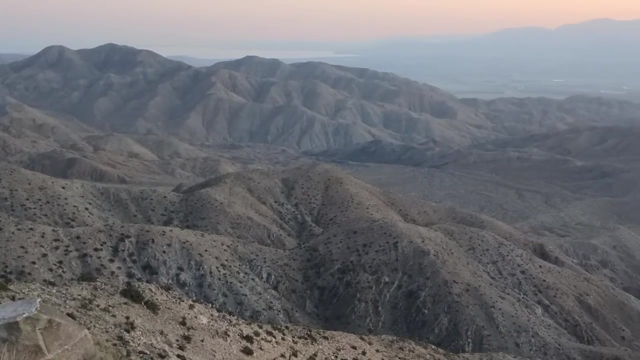 opening up the first trade routes. Their myths and legends inspired various origin stories, and their memory lives on in the Old Testament. The heritage of the Sumerian civilization and their successors is everywhere. There were many great cities in the ancient Near East that influenced the course of history. Babylon and Jerusalem are two of the better known. but none of them are the same. The Sumerians were the first to build gigantic cities, and the greatest cities in the history of civilization are the first to build huge cities. The Sumerians built huge cities like Canaveral, Damascus, Ur, Uruk, Memphis, Thebes and Sidon were just a few. 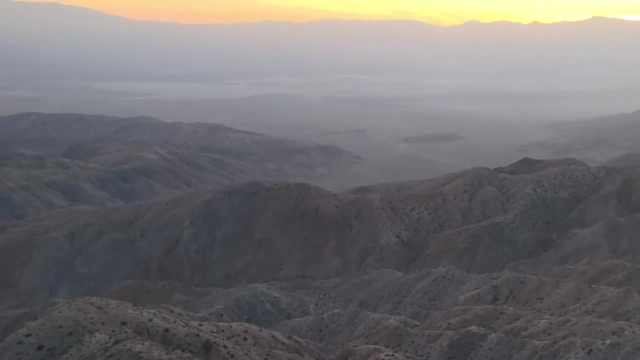 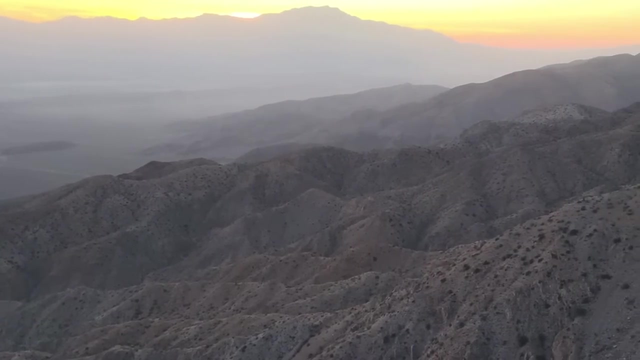 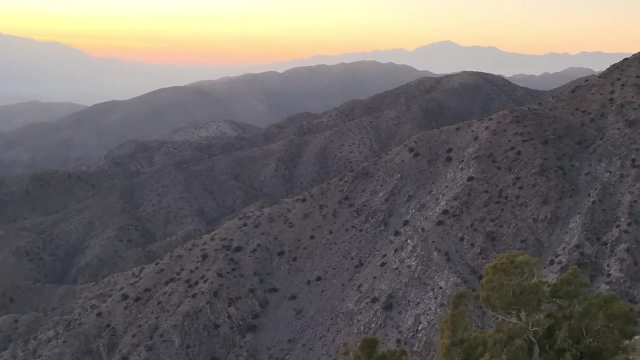 of the great cities where science and literature were created, theologies proposed and empires born. There are numerous reasons why these cities became prominent, many of which were related to the fortuitous circumstances of environment and politics. but for every one of the great cities, 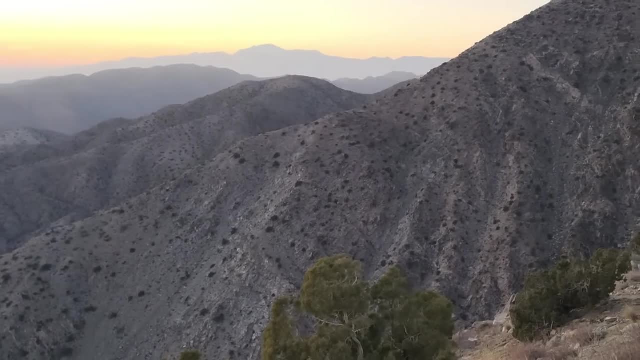 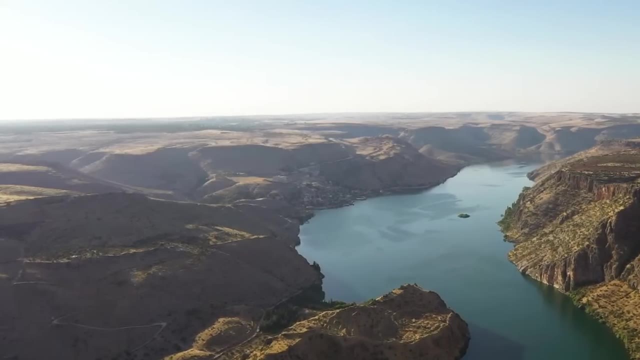 there were many more that flourished and then had their prestige overshadowed by the growth of their nature. These cities often played important roles in the historical processes of the region for a time, but due to numerous circumstances, their influence proved to be ephemeral. 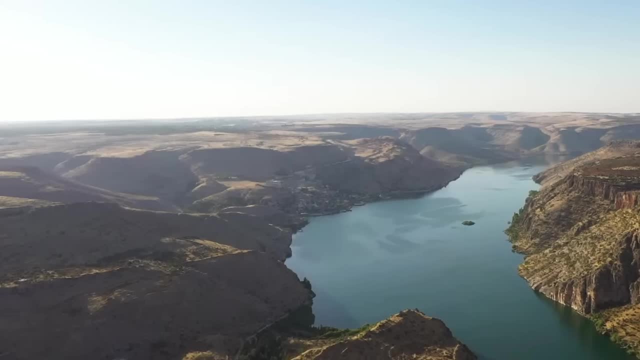 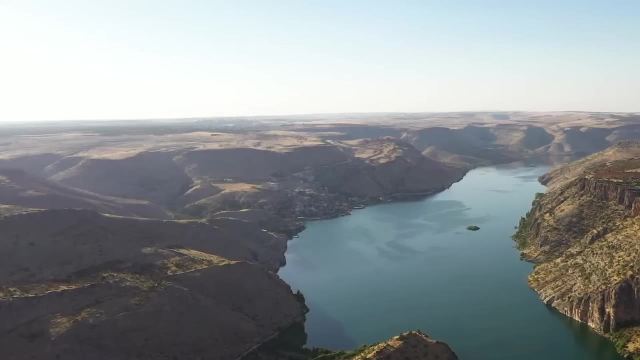 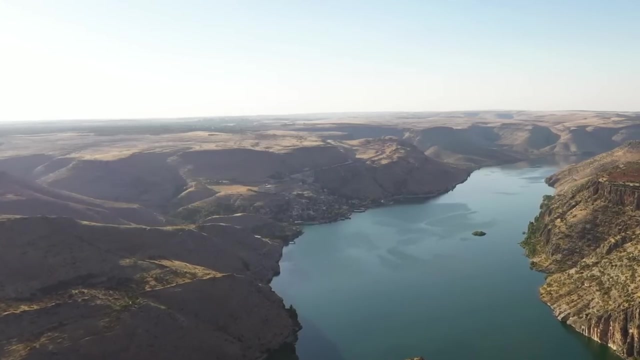 One of the most interesting of these early ephemeral cities was Puma, Located in the southern region of Mesopotamia, known as Sumer. Puma became a prominent Sumerian city in the early 3rd millennium BCE, and while Uruk was the most important Sumerian city during that era. 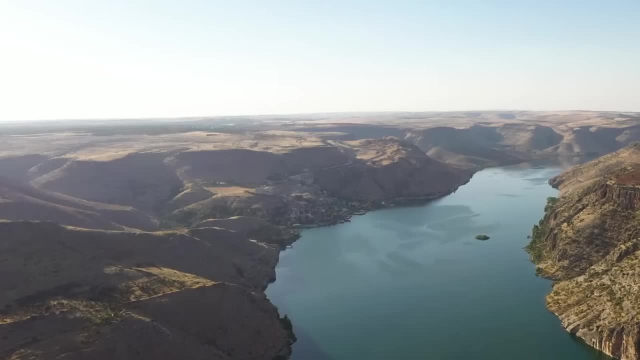 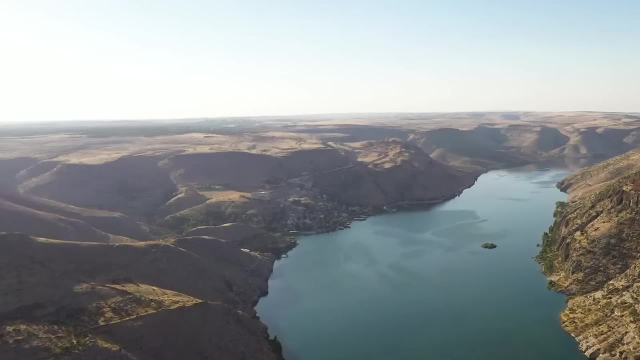 Uma was close behind in influence and power and for a time seemed poised to become the most important place in Sumer. A powerful dynasty arose in Uma that expanded its influence across southern Mesopotamia, uniting Sumerian cities under one government. 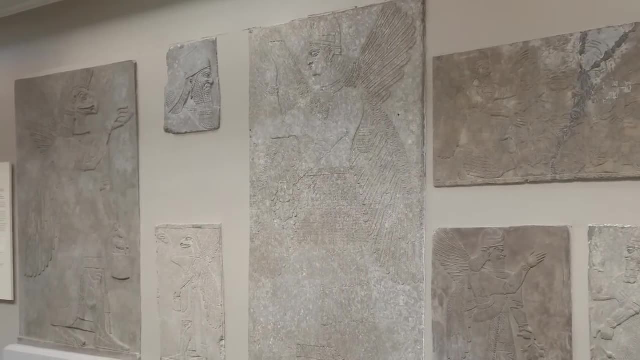 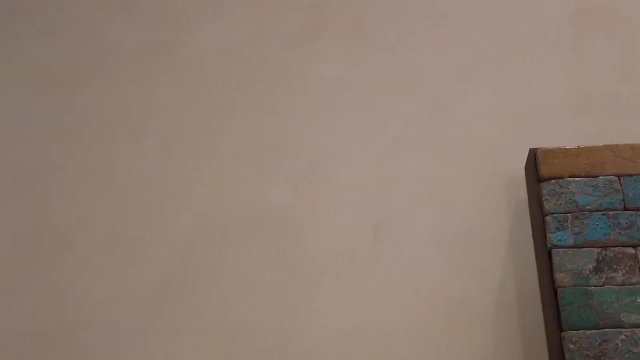 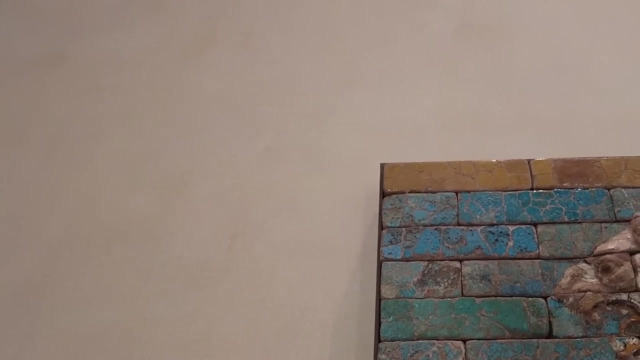 but the central position that Uma enjoyed proved to be temporary, because Semitic conquerors from the north forced Uma and the other cities to accept their rule. Uma continued to exist and even prosper, and it eventually became a somewhat important city again under the Neo-Sumerian 3rd dynasty of Ur in the late 3rd millennium BCE. 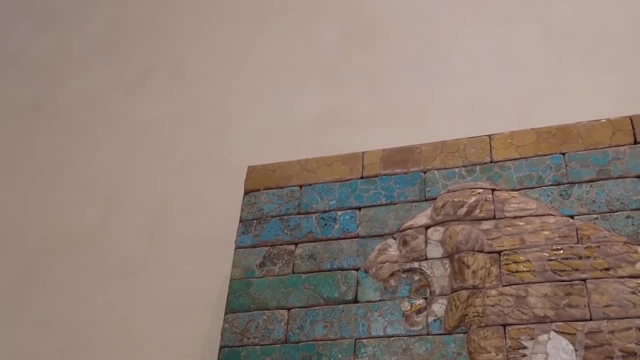 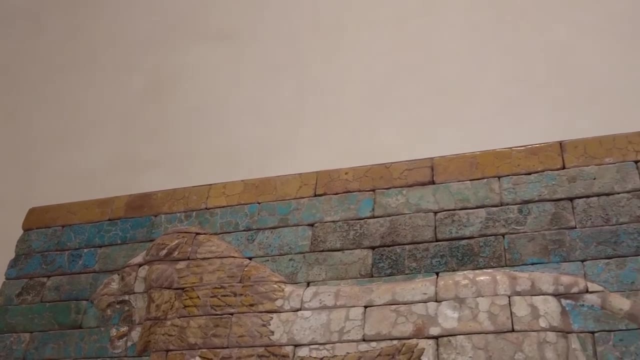 It was not until the 6th century BCE that Uma went unmentioned in the historical record during the Neo-Babylonian period. By then, the city was a shadow of its former self, but some of the earliest known Mesopotamian historiographical inscriptions were recorded in Uma. 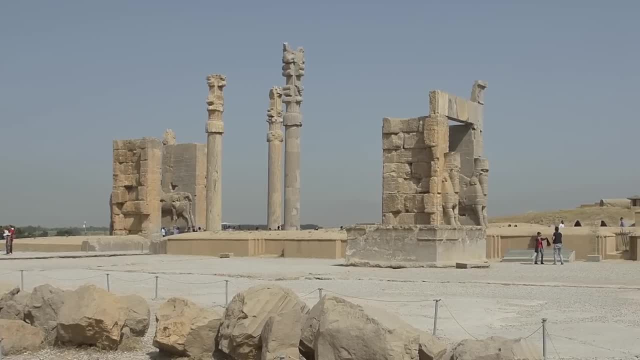 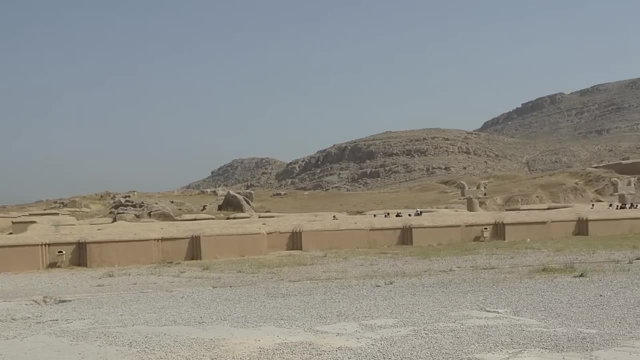 The god of its city became an important deity to the Mesopotamians. The Mesopotamian pantheon and its merchants became well known for introducing a type of silver standard for trade. Thus, even as Uma was forgotten, even as far back as ancient times. 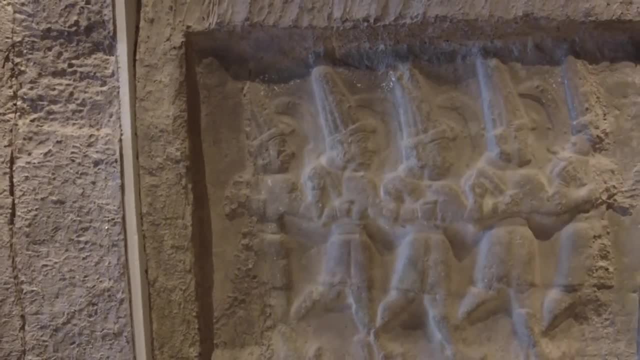 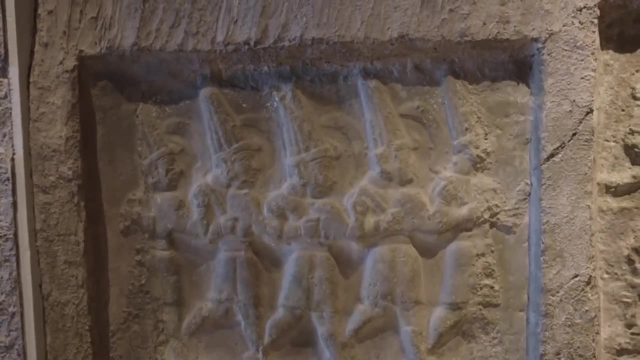 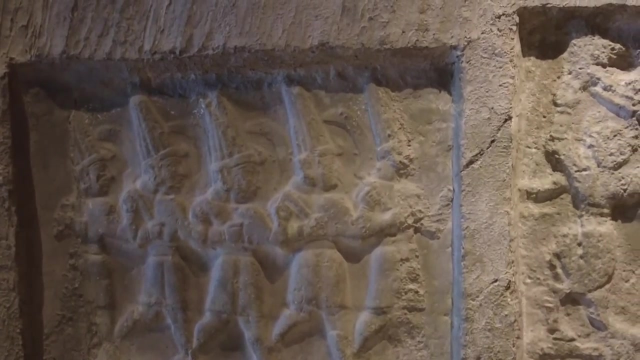 it continues to fascinate modern historians and archaeologists. The word Mesopotamia highlights the central theme of life in the Fertile Crescent, coming from the ancient Greek for land between two rivers. These rivers were the Tigris and the Euphrates. 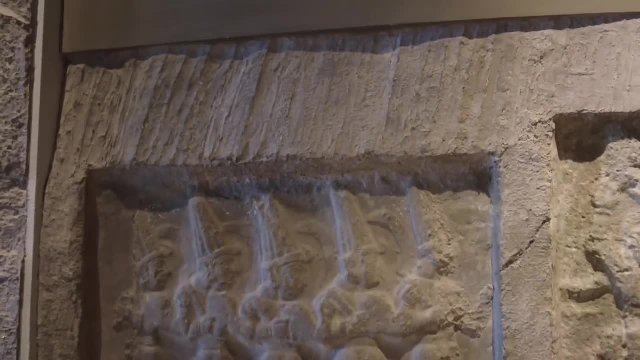 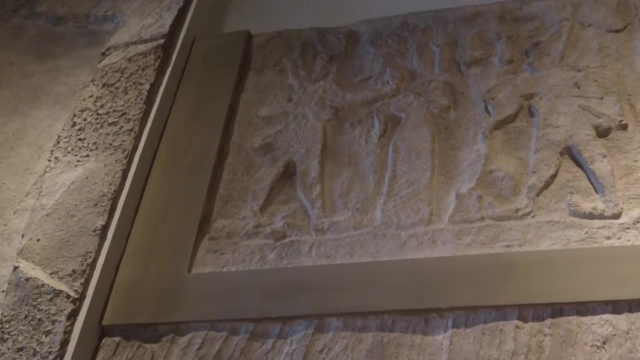 both rise in the Taurus mountains of Anatolia and flow through present-day Syria and Iraq and into the Persian Gulf. Civilization was born on the banks of these two rivers and the sediment that was carried by the fast-flowing waters of the Anatomian highlands. 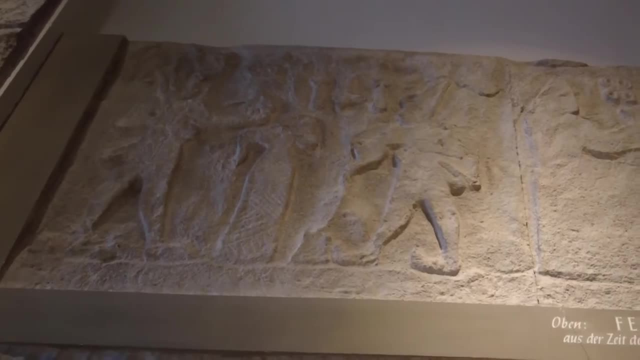 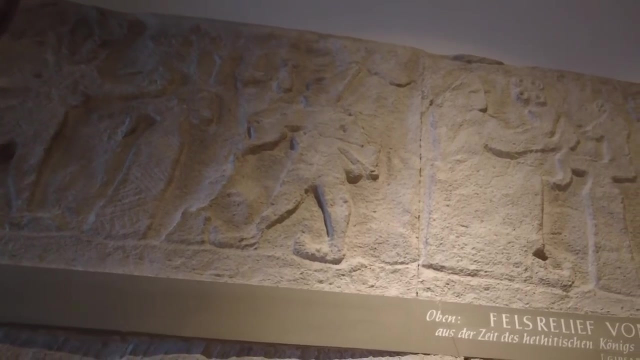 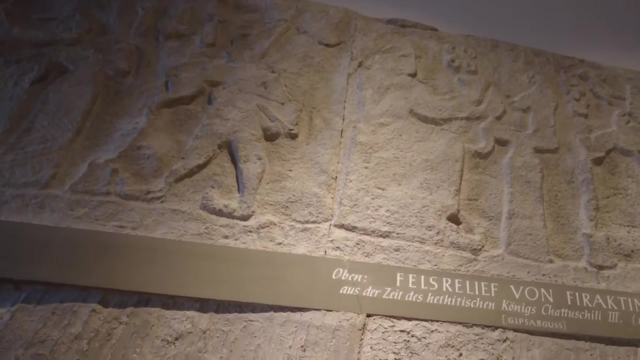 gradually settled as it reached Iraq. as it became calmer, Seasonal floods distributed the nutrient-rich sediment along the river banks all the way to the Persian Gulf, creating an alluvial plain where irrigation could flourish. The people who settled in Mesopotamia were inextricably connected to their environmental context. 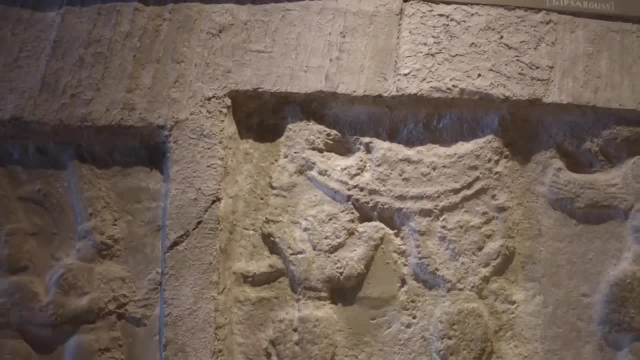 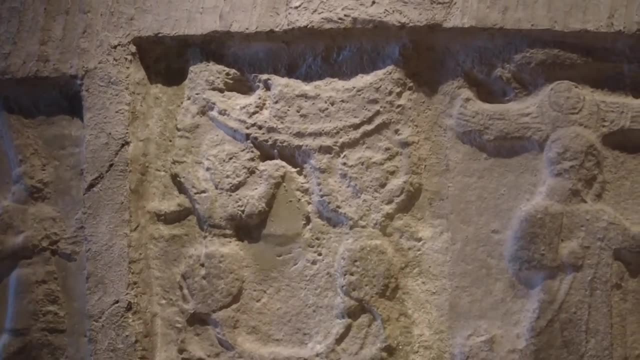 In central and southern Mesopotamia, the low hills and fertile plains were juxtaposed with swamps, jungles and countless streams, where the Tigris and Euphrates drained into the Persian Gulf, most of which have disappeared over the course of time. 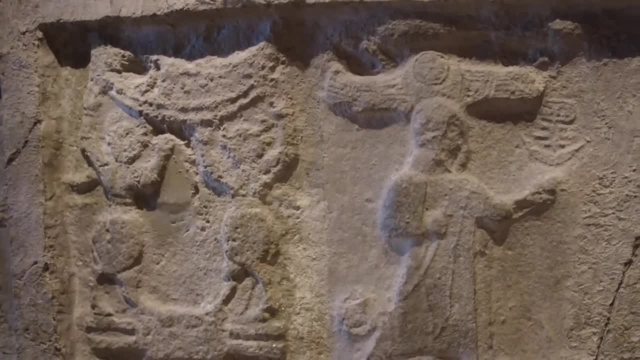 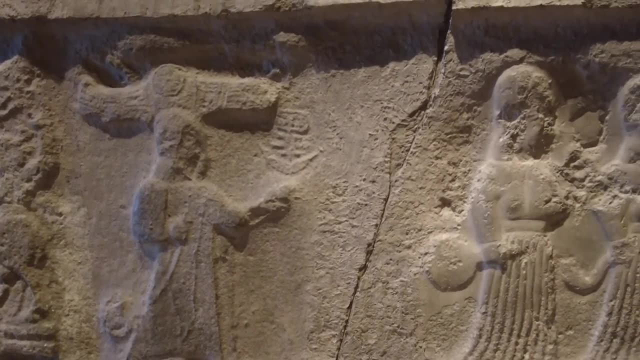 Water was vital for farming, drinking and transport across the region. It facilitated trade and goods and facilitated communication between complementary economic spheres. Mesopotamia had few natural resources. No stone, wood or precious metals could be found in southern Iraq. 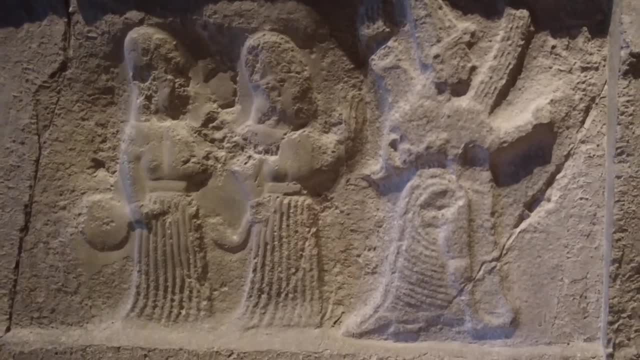 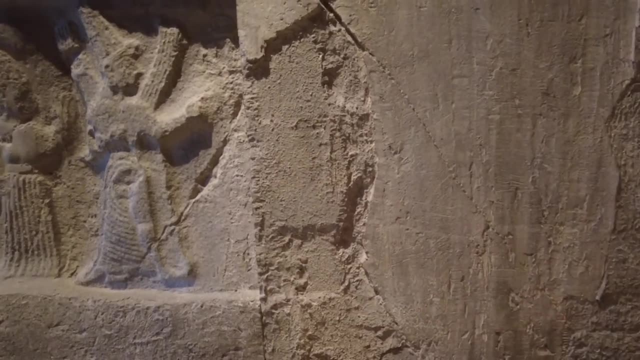 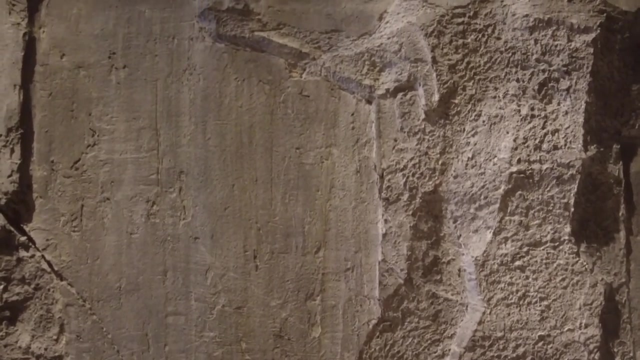 There was only water and a rich alluvial soil with which a hard-working people could transform a land of scarcity into a land of plenty. The Mesopotamian civilizations are among the world's oldest, with archaeological evidence stretching back beyond 6,000 BCE into the Neolithic. 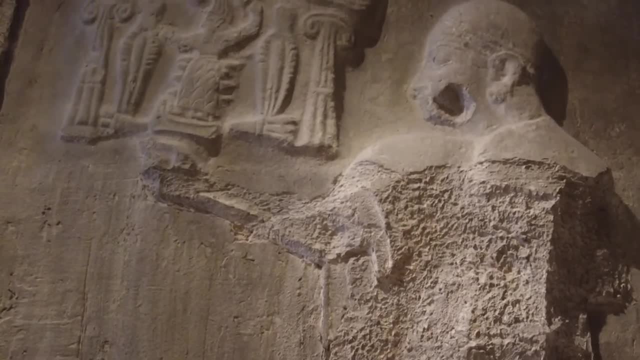 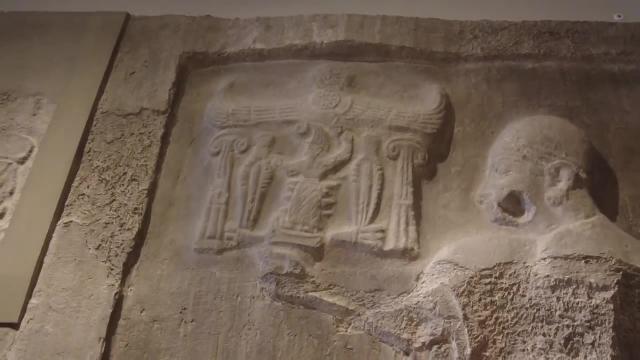 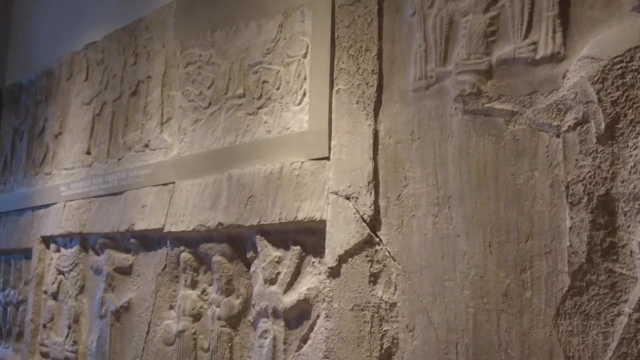 As hunter-gatherers discovered ways to farm and store their food for weeks and months at a time. instead of being itinerant, they decided to colonize lands along the fertile banks of the Tigris and Euphrates During the Ubaid period. 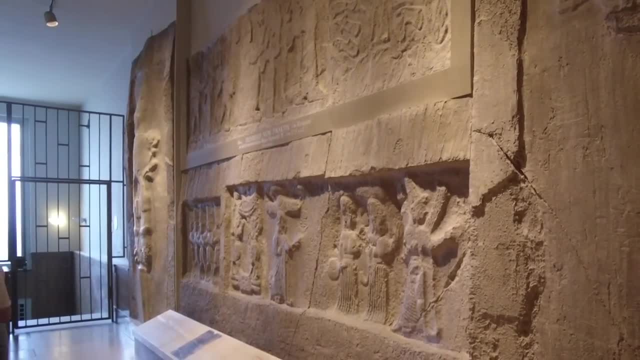 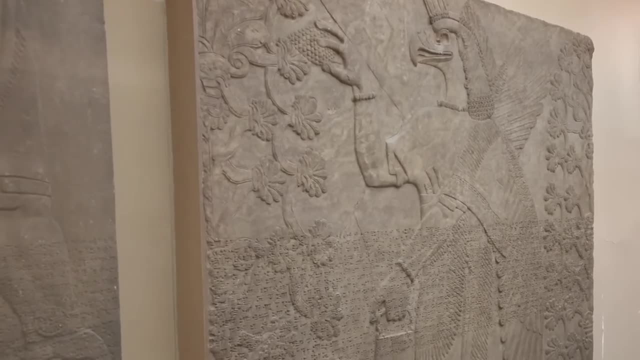 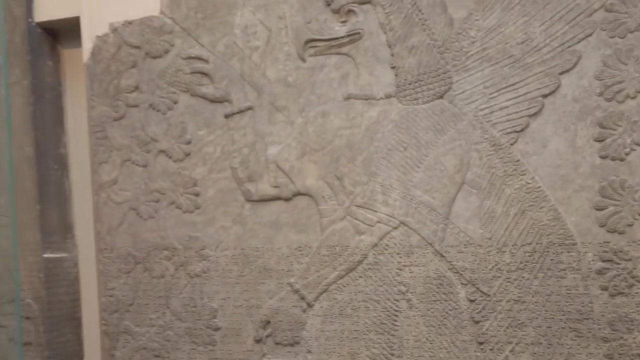 the earliest settlements were established in southern Mesopotamia. Thanks to a number of technological breakthroughs, including the adoption of the wheel, the mass production of mud bricks and irrigation, the people of Mesopotamia managed to successfully reside at single locations for generations. 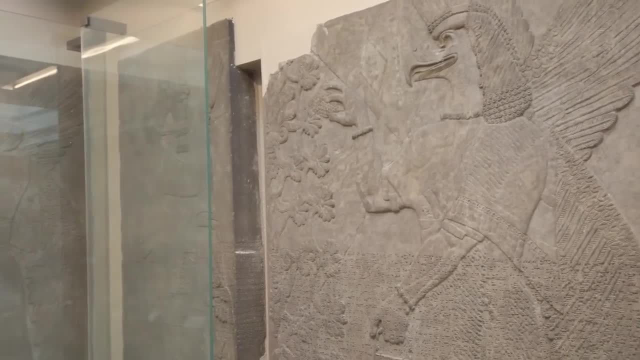 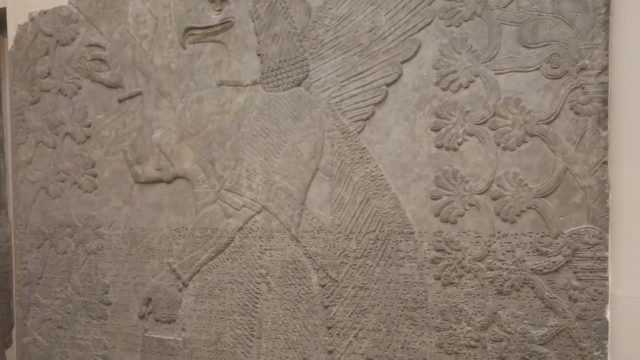 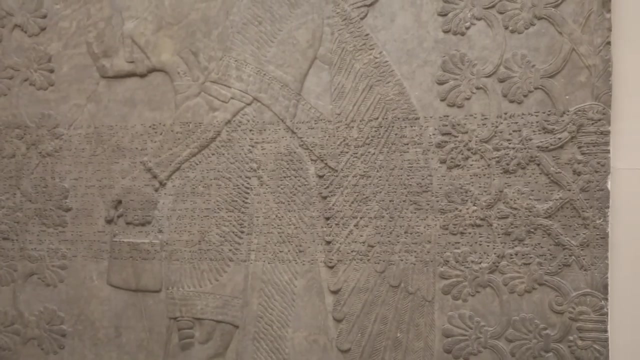 and over time their settlements grew in size and formed so-called tell sites. Many of the smaller villages were clustered in relatively close proximity to one another due to the nature of irrigation on the alluvial plain. The large cities would have had a number of smaller satellite towns in their hinterland. 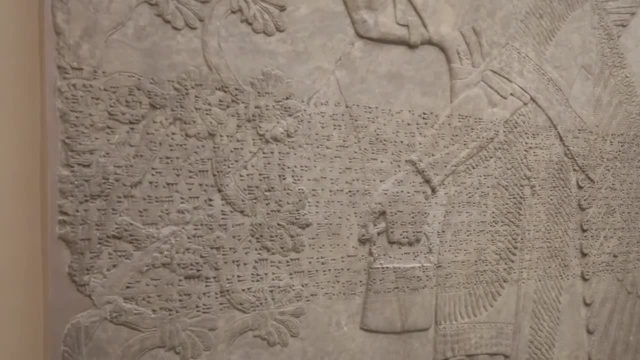 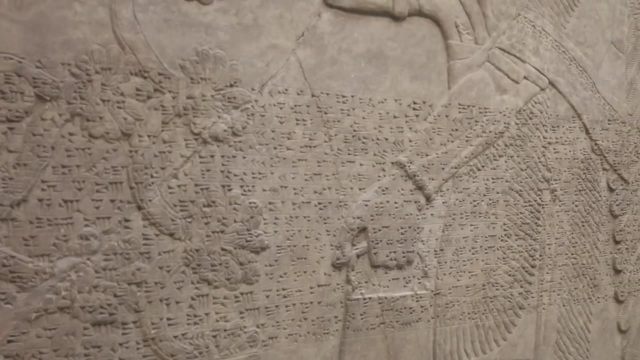 The archaeological remains of the latter have largely disappeared over time, so it is large sites like Eridu that archaeologists must look at to build a picture of life in ancient Mesopotamia. The bulk of Mesopotamia is in what is now Iraq. 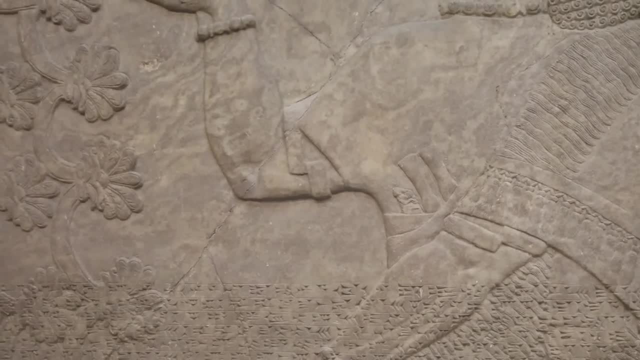 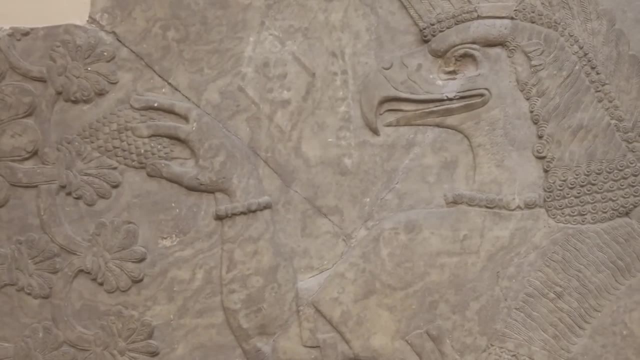 but in ancient times this land was divided between two broad groups: the Sumerians and the Akkadians. The Sumerians lived in the south and spoke their own unique language. The Akkadians to the north, by contrast, were Semites. 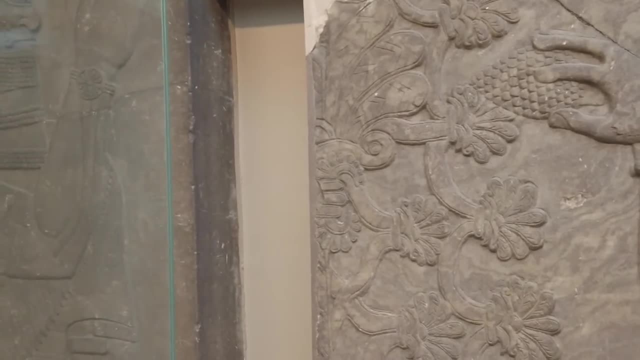 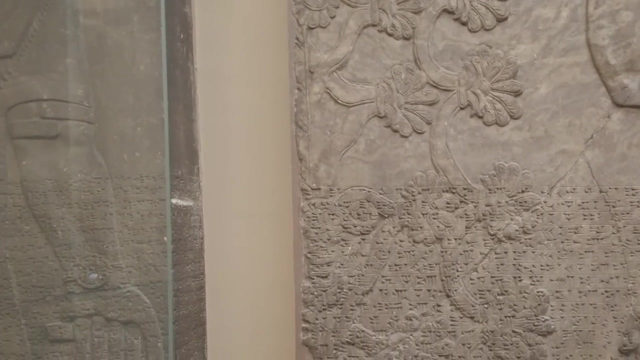 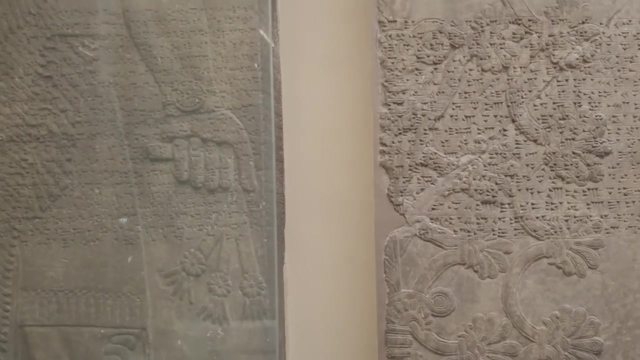 who spoke a language whose modern relatives include Hebrew and Arabic. The Sumerians were able farmers who dug ditches to divert the life-giving waters of the Tigris and Euphrates to their fields and, thanks to the abundant food supply brought by their ingenuity, they flourished. 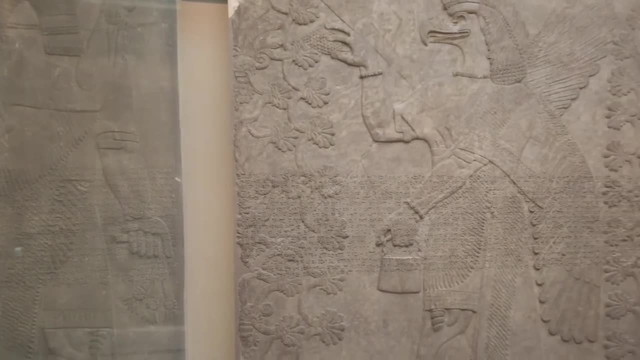 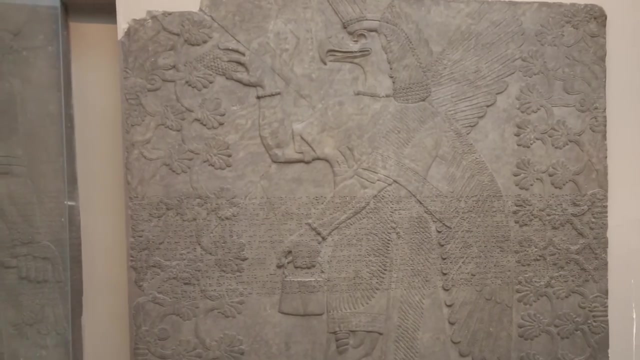 Sumerian city-states grew to a size of many hundreds of thousands of people each being organized around the worship of an individual deity associated with the temple of the main city. The semi-nomadic Sumerian culture arrived in Mesopotamia. 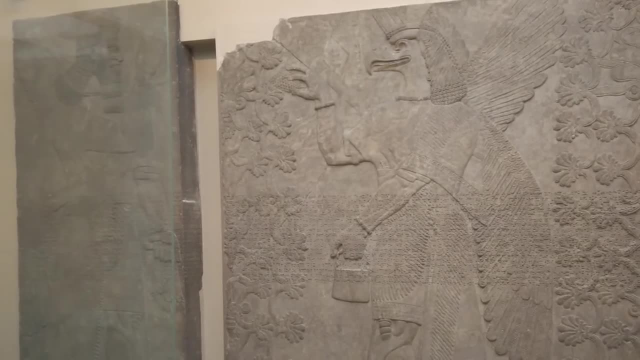 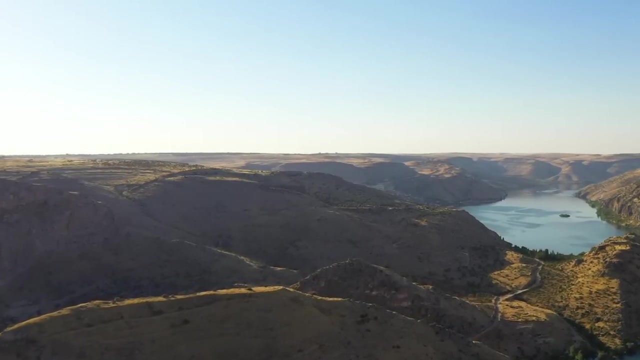 in the middle of the fourth millennium BCE, and they eventually came to dominate the southern part of the region. though their origins before they moved into Mesopotamia remain shrouded in mystery, Their culture became concentrated in the major urban centers of the region. 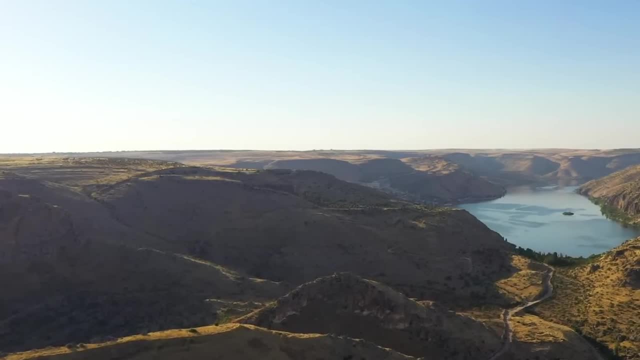 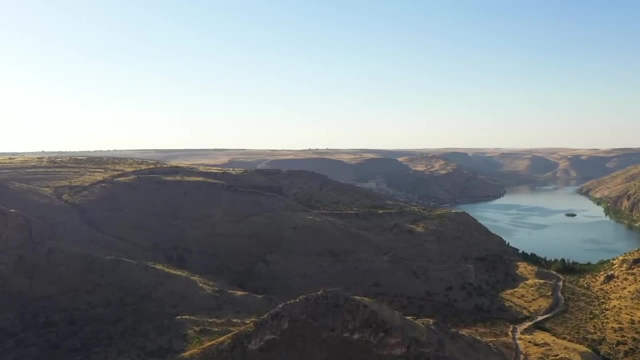 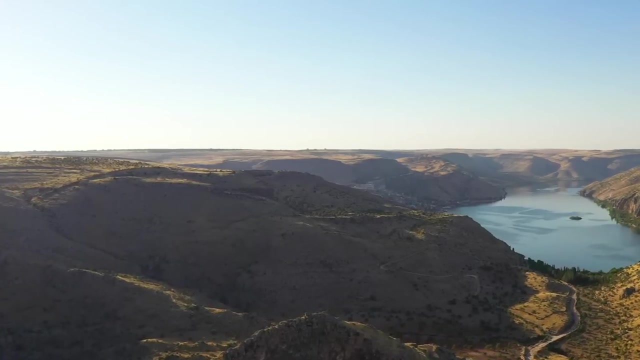 namely Eridu, Ur Uruk, Larsa and Nippur, But they were not perfect. They were not the only residents of southern Mesopotamia. Early villages were composed of settlers from many different regions, many with their own distinctive characteristics that differed from those of the Sumerians. 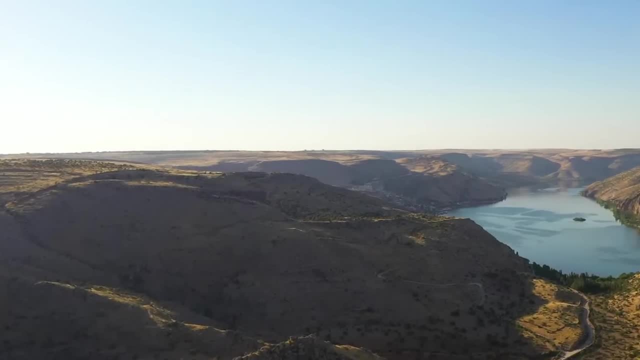 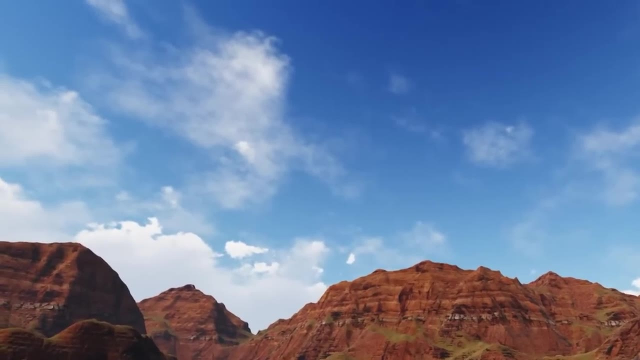 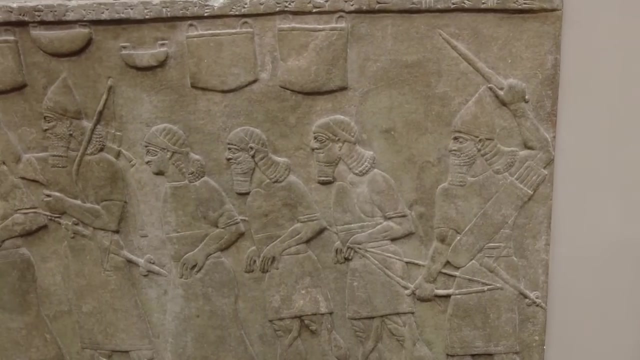 Some have argued that it was these cultural differences that contributed to the many technological inventions and innovations that occurred in Mesopotamia in the formative stages of urbanization. It also partly explains the complexity of the region's religious systems. The Sumerians were great inventors. 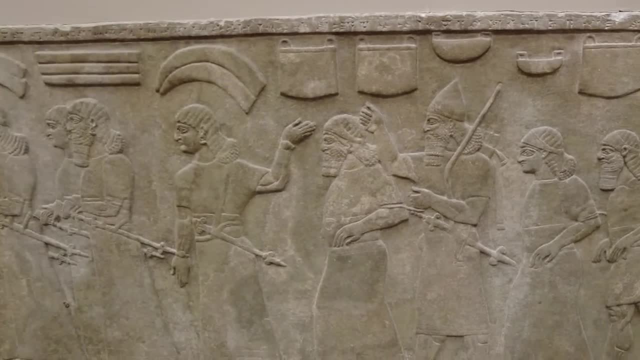 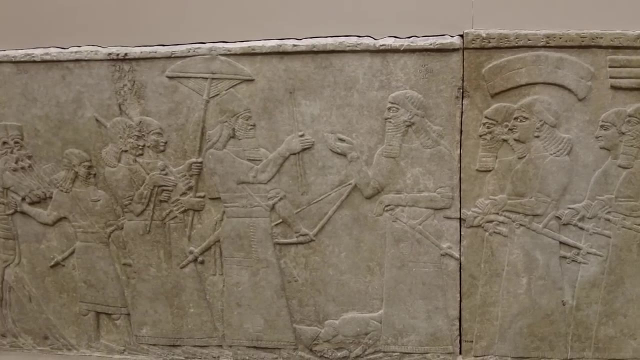 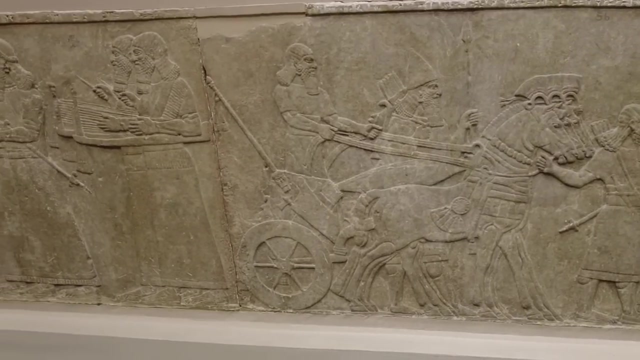 and none of their inventions was more important than writing. Writing systems emerged at an early stage in the mid-fourth millennium BCE, first through pictographs and later by the cuneiform script. Cuneiform became the most dominant form of writing across the region. 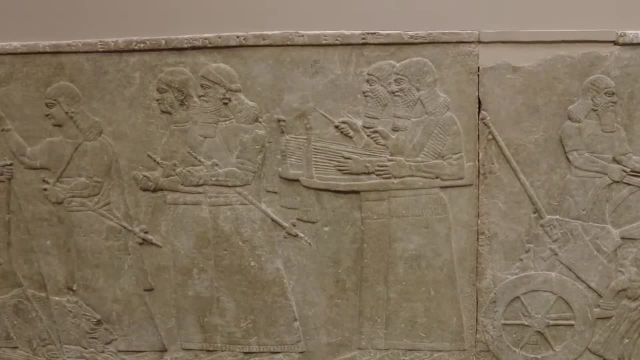 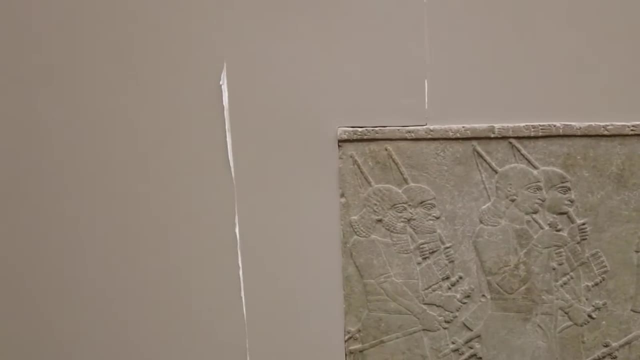 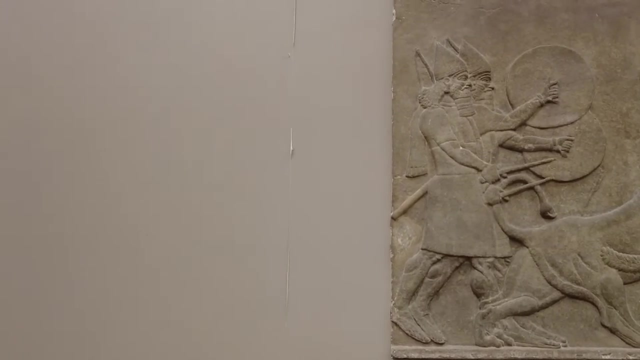 the letters of which were pressed into clay tablets with a triangular stylus, And it is thanks to this writing system that scholars have been able to reconstruct life in ancient Mesopotamia in such vivid detail. The book of Genesis said that the first cities arose in the beginning. 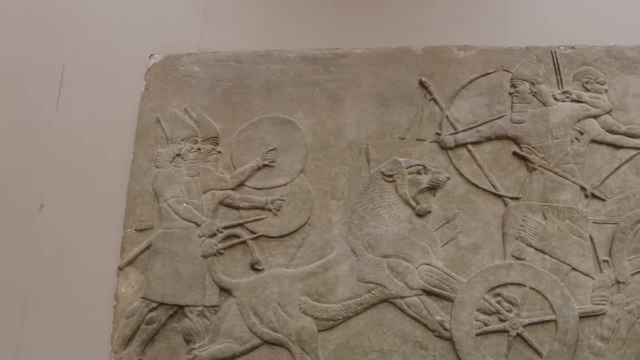 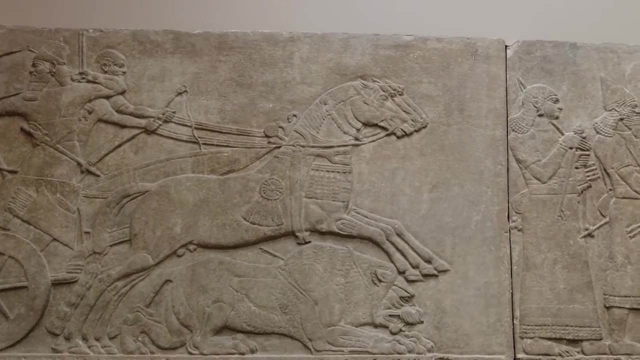 when God let dry land rise from the water. But the Bible was not the earliest of such narratives. According to the Sumerians' own myths, in the beginning there was the city of Eridu, Given the many fanciful myths about Eridu. 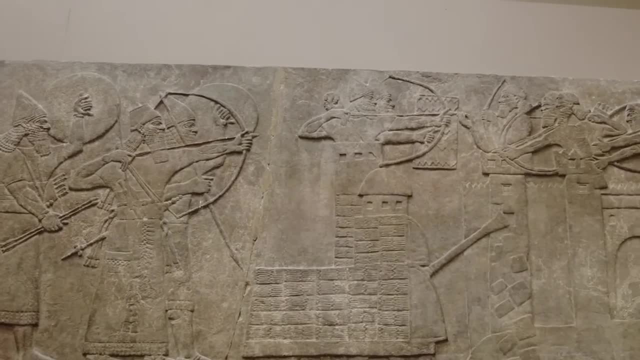 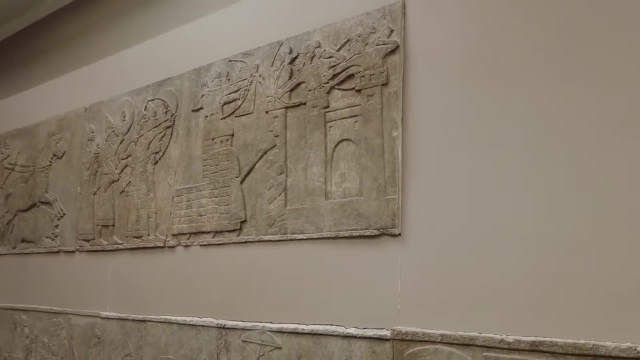 it surprised many people to find that the city was in fact a real place after it was discovered by archaeologists in the mid-nineteenth century. In the wake of World War I, the region came under British control with the name of State of Iraq. 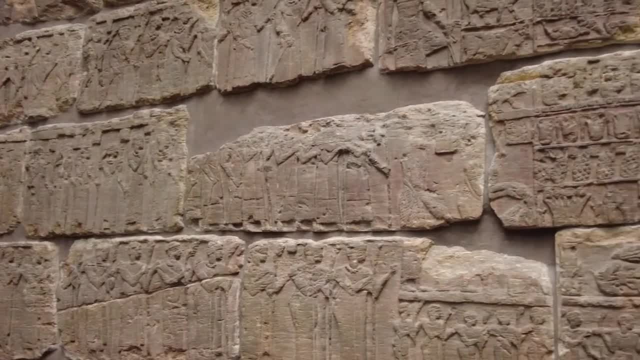 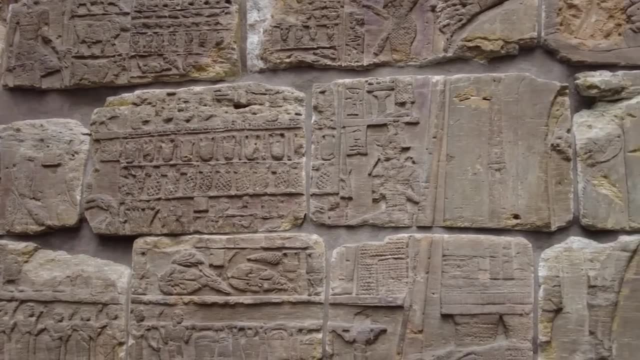 and the British Museum organized a number of archaeological expeditions to Mesopotamia. Their role was not only to protect the heritage of the region, but also to acquire objects to be brought back to London for exhibition In the 1850s. 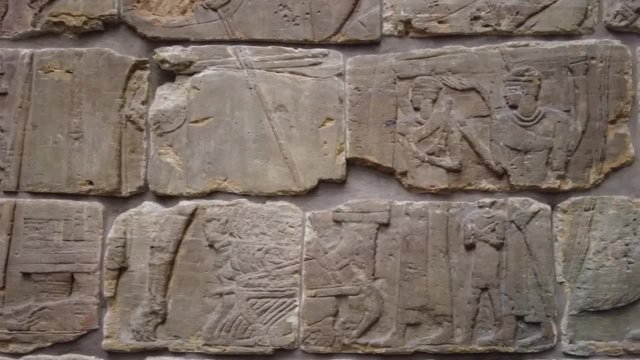 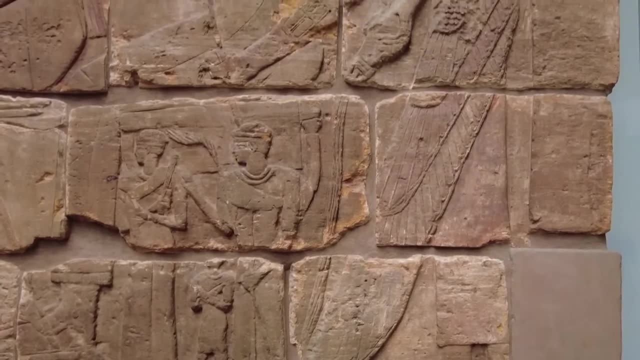 when archaeologists first went to Iraq, they went in search of the region's biblical past. In the mid-nineteenth century, all that was known of ancient Mesopotamia was what could be read in the Old Testament. French and British archaeologists competed to discover. 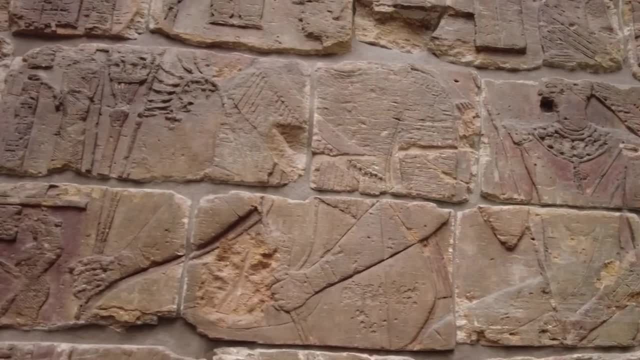 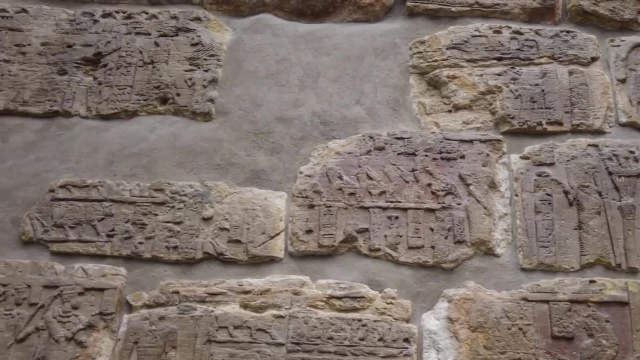 what they could find of these semi-mythological lands, focusing their interest on the site of Babylon and instead finding the remains of much older civilizations. They uncovered an unsuspected civilization buried beneath the sands. But what was so special about what they found? 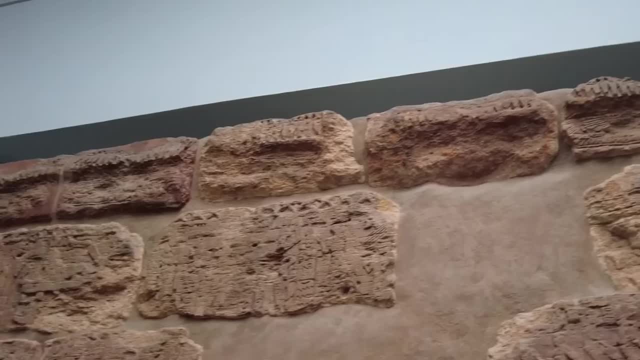 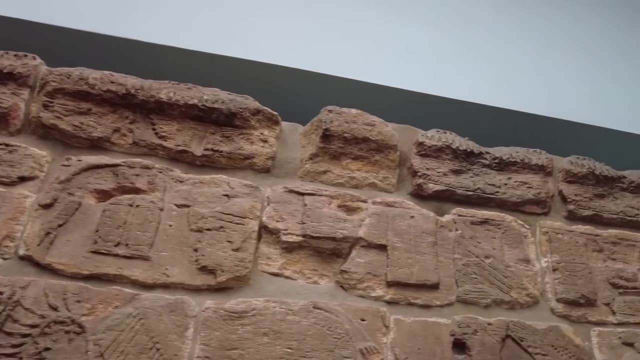 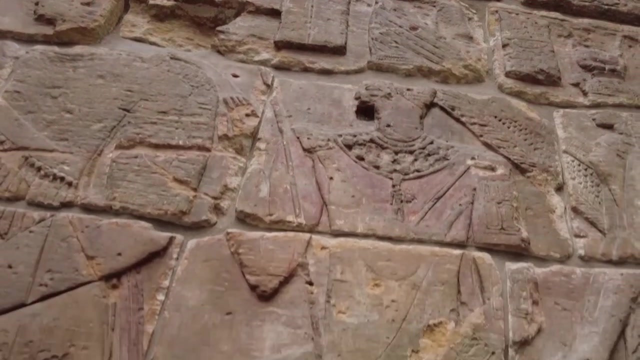 And why did a civilization develop in that part of the world at all? These were the questions asked by Mesopotamia's earliest researchers. The first archaeologists to see the ruins of Sumerian settlements must have been speechless, because before them lay a confusing landscape of narrow streets. 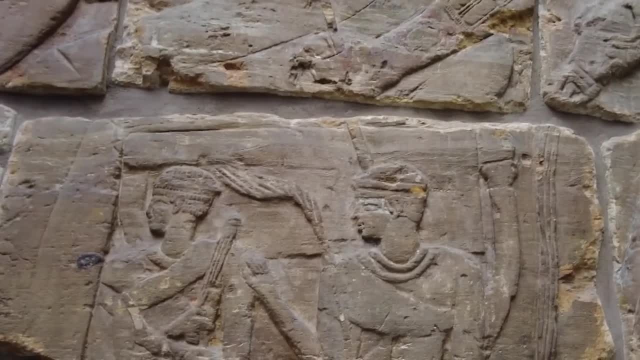 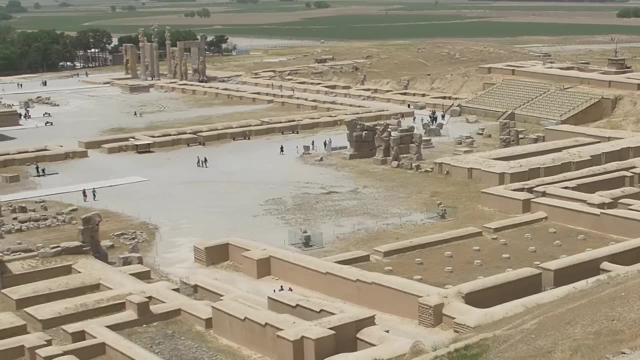 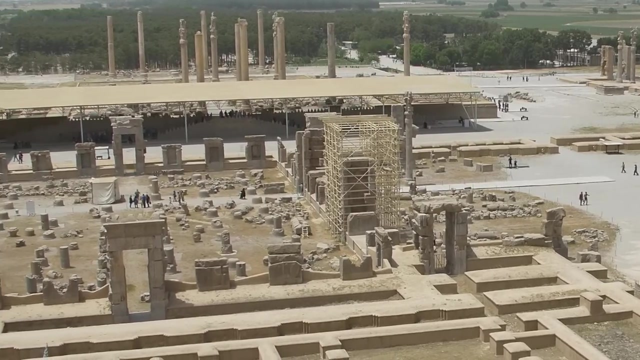 squares and remains of houses, granaries and temples. Today, the land around the ruins is desert, making it difficult to picture it as a once-thriving region in which its inhabitants lived off the land When they found the ruins of Sumerian dams on this barren land, 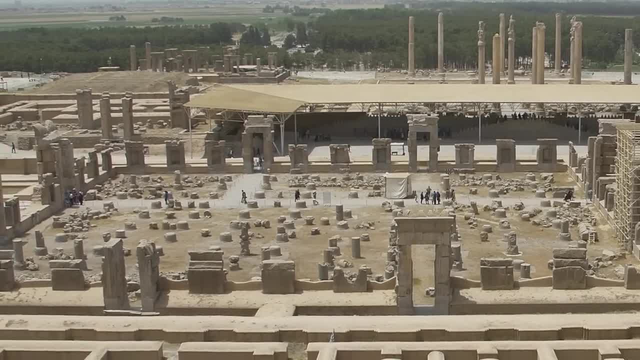 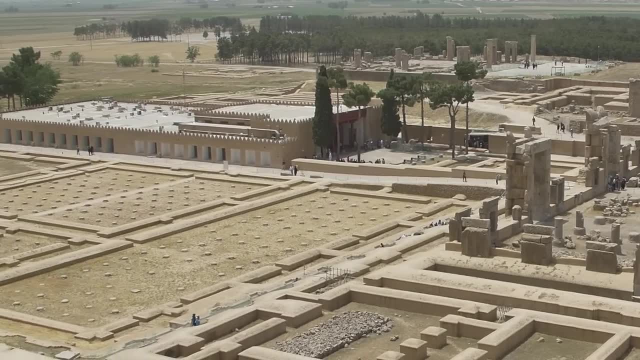 the archaeologists of the nineteenth century faced an enigma in attempting to figure out how people could have lived in this desert so far from a source of fresh water. In fact, when Ummah was discovered during the great rush of archaeologists to Iraq in the nineteenth century, 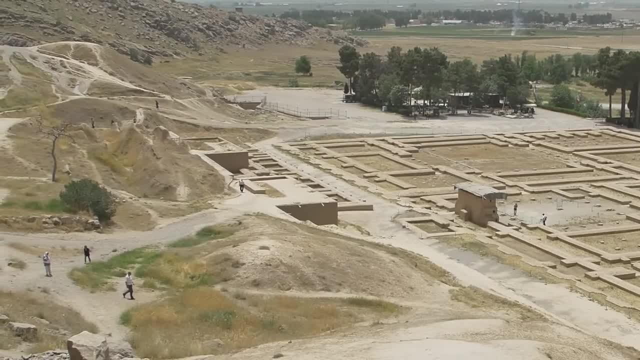 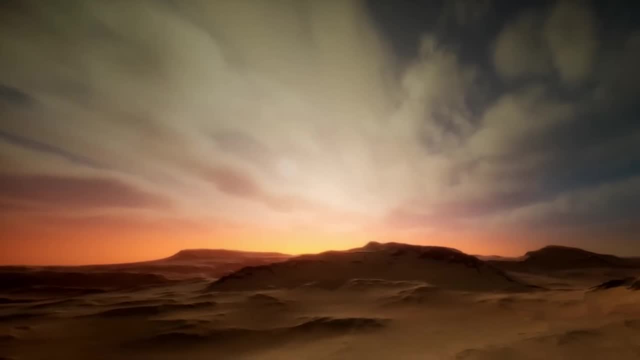 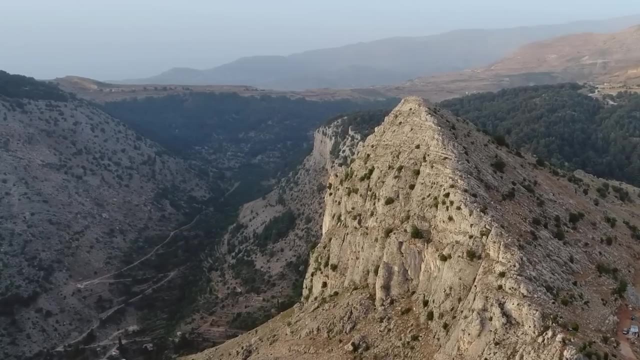 it was not widely known that it had actually been discovered. As will be discussed later, Ummah had several different names throughout its history, so philologists had to get together with archaeologists to find out what they had in fact found, Located in the southern Mesopotamian region of Sumer. 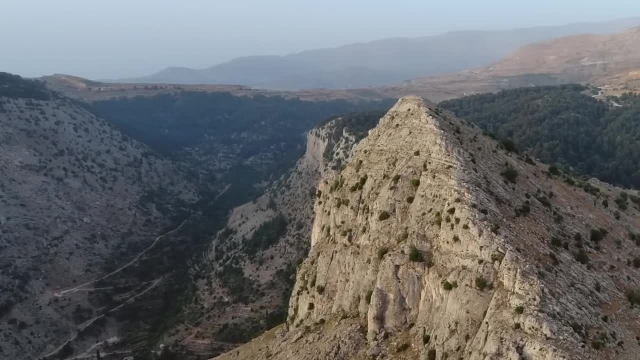 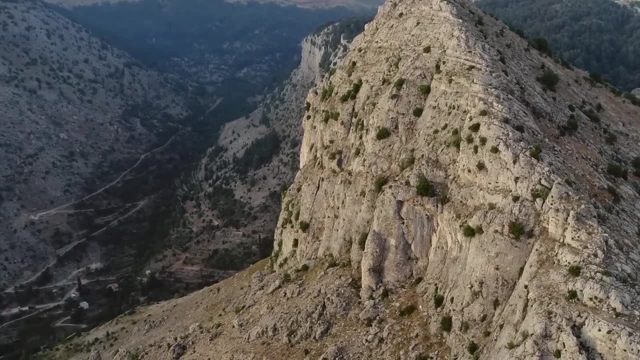 Ummah was one of the earliest cities built by the ancient Sumerians and, despite the fact that Uruk and Ur stand out as more important cities that were built before and after Ummah, respectively, Ummah's general proximity to both of these cities. 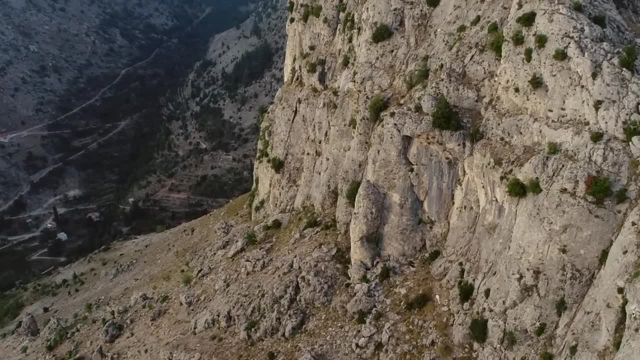 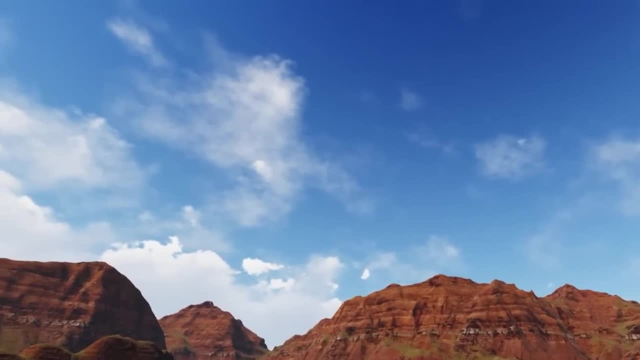 helped make it important, as did its contemporary Mesopotamian history. Unlike Uruk and Ur, which were located close to the Euphrates River, Ummah was in the middle of the rich alluvial plain between the Euphrates and the Tigris. 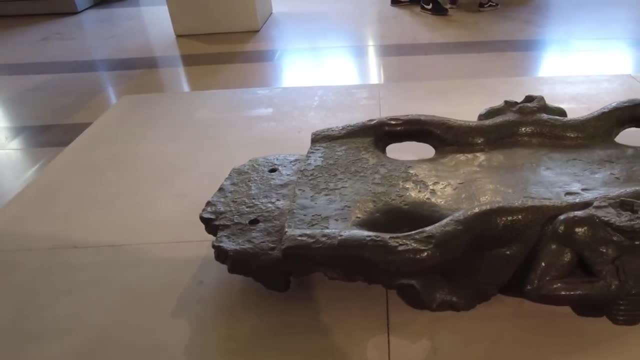 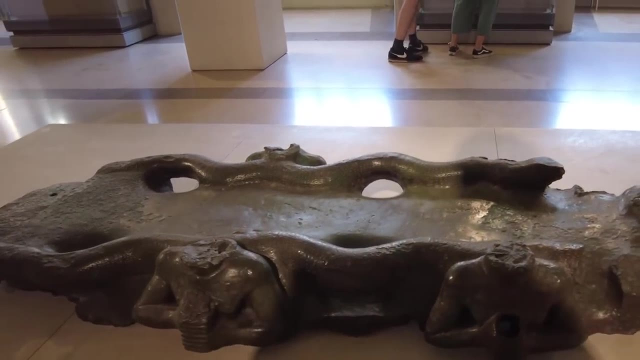 From this position, the Sumerians built an intricate network of canals that brought water to the fields and people of Ummah and linked the city directly to the two major rivers of Mesopotamia. When the Sumerians first began building cities in Mesopotamia, 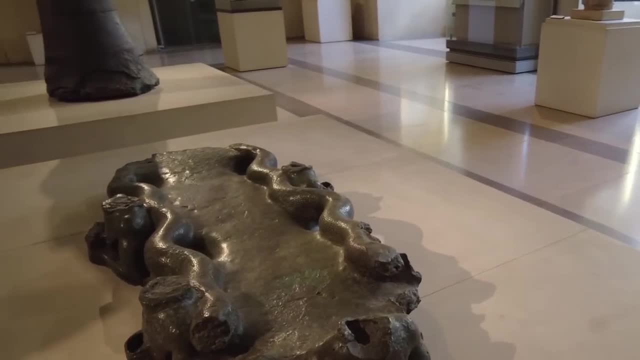 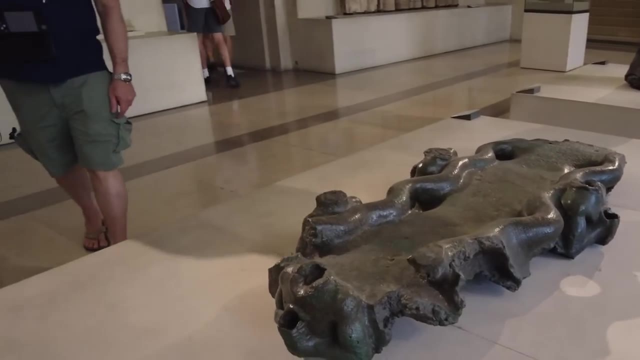 in the late fourth millennium BCE. Ummah was one of the first. Given that fact, it's important to keep in mind that most ancient Mesopotamian ethnic groups were Semitic, but the Sumerians spoke a language that, while yet to be categorized, was not Semitic. 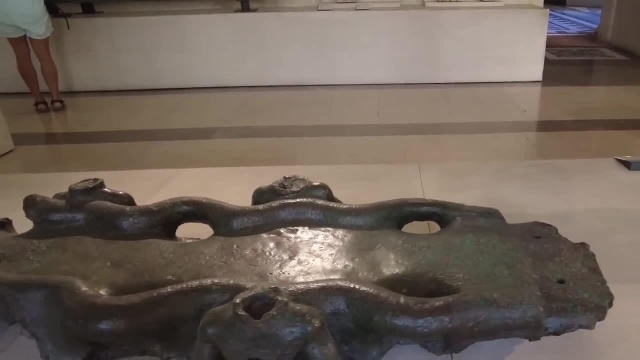 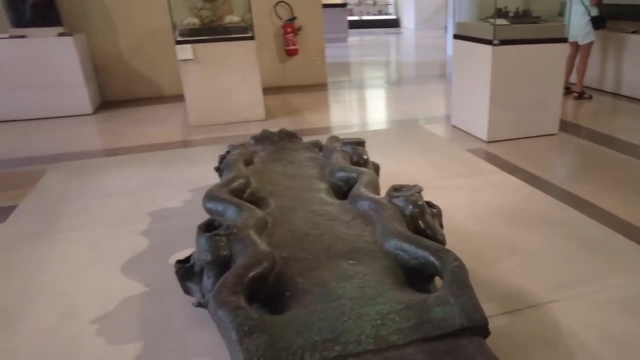 being made to believe they migrated to the region from the east. That said, since there is no solid evidence of any Sumerian migration, other scholars believe that the Sumerians were either native to the region or at least there before the other Semitic groups. 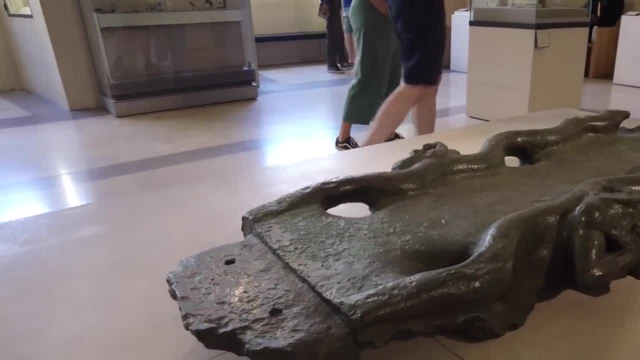 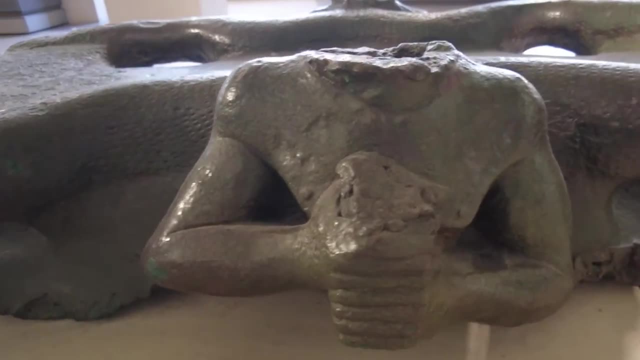 What scholars do know is that by the last couple of centuries of the fourth millennium BCE, the Sumerians had developed a culture that had all the hallmarks of an advanced civilization. The Sumerians discovered writing, which allowed them to record their religious ideas. 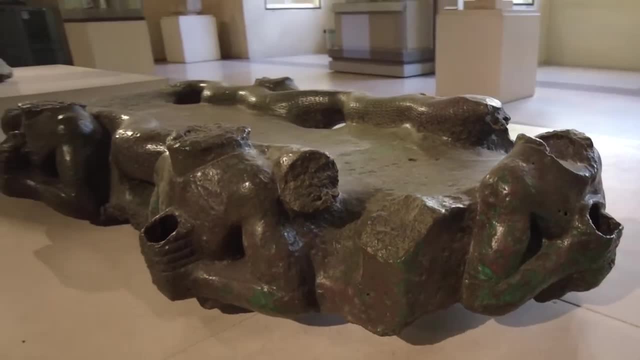 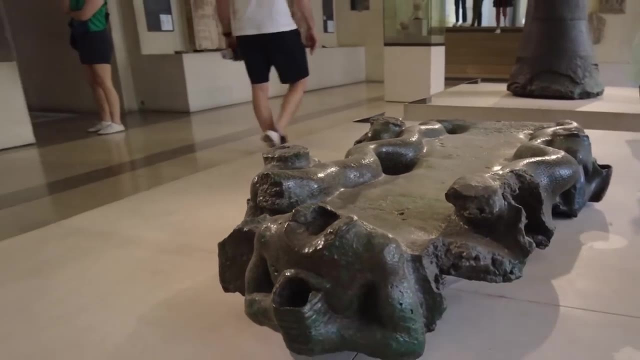 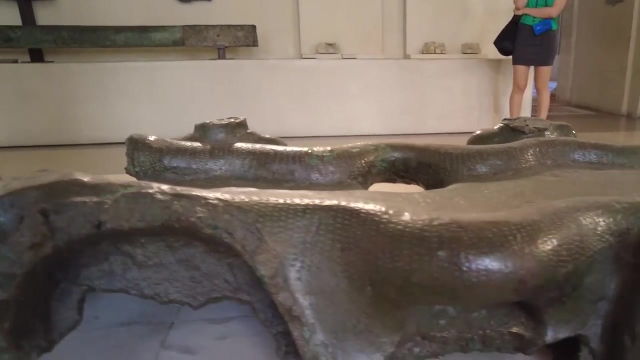 royal records and king lists and bureaucratic records. The Sumerians also divided their society into classes, developed the sophisticated irrigation system mentioned earlier and built some of the world's first cities. It was in the temples of these cities where the first Sumerian scribes began writing documents. 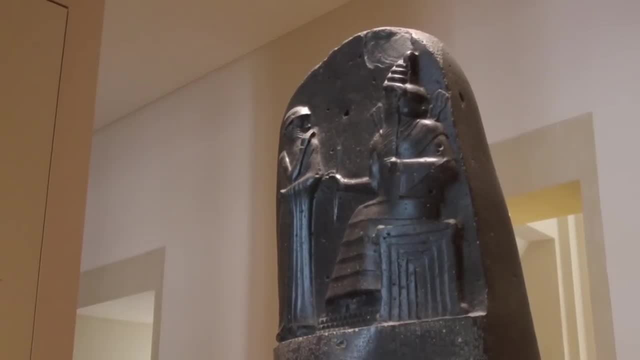 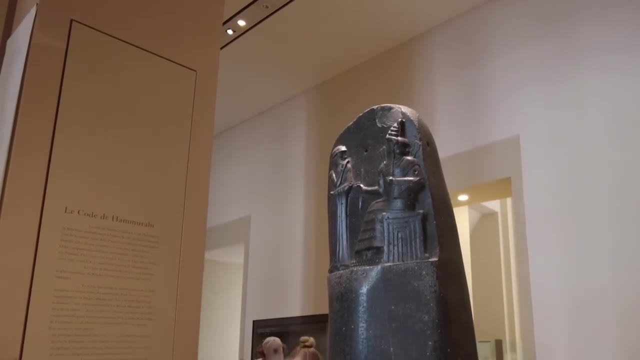 on clay tablets in the Sumerian language using the cuneiform script. Thanks to these Sumerian scribes, modern scholars know a fair amount about the political life of ancient Sumer in general, and more specifically about the inner workings of many of its cities. 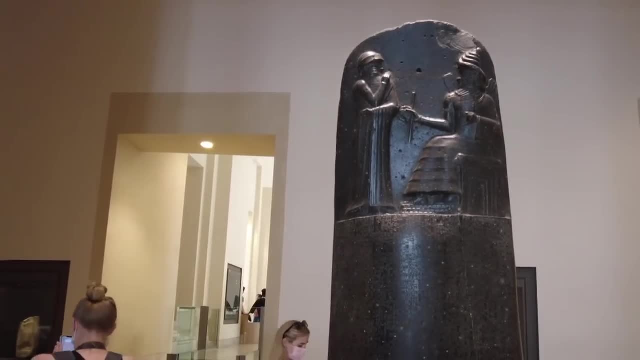 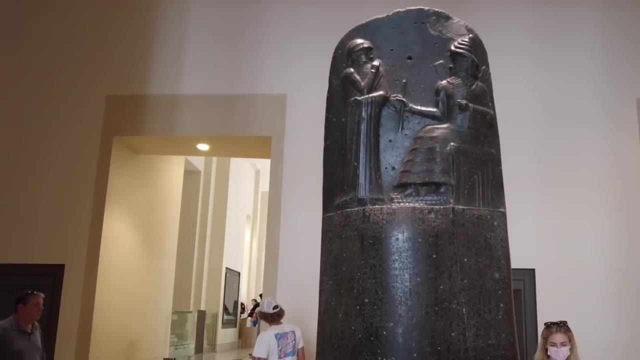 including Uma. When the first Sumerologists began translating cuneiform texts from Mesopotamia, Uma was not initially recognized as a great Sumerian city. The problem was not that Uma was small, as will be discussed later. it was a fairly large Mesopotamian city. 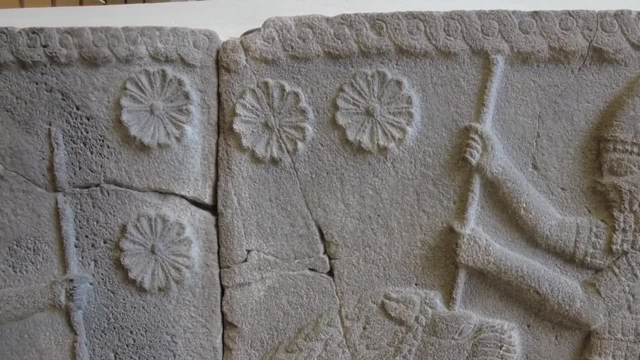 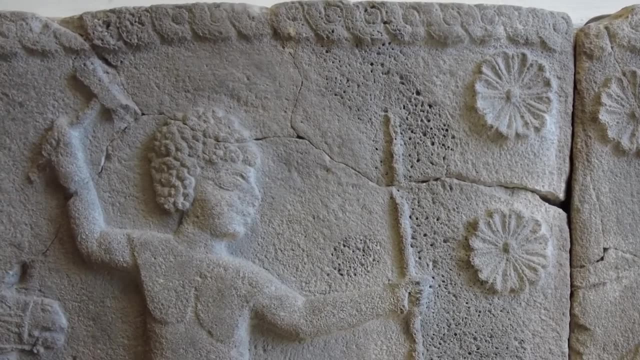 or that it was wiped out in one fell swoop, but that it was actually known by many different names throughout its long history. It is important to point out that Mesopotamia, unlike its contemporaries in Egypt, was quite ethnically diverse. 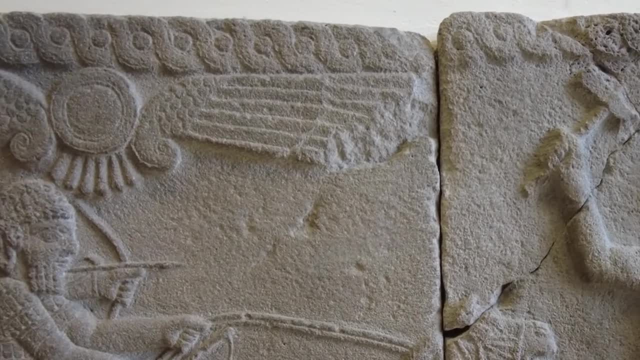 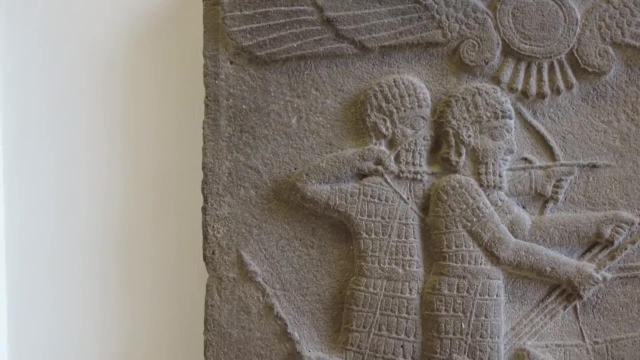 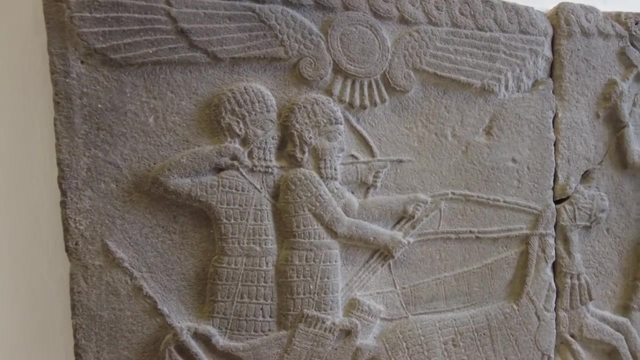 In addition to the Sumerians, already Mesopotamia was populated by Semitic speakers who had also varying regional dialects, and because of this unique feature of Mesopotamian civilization, Uma was known by different names to different people. Uma was actually the late Babylonian era. 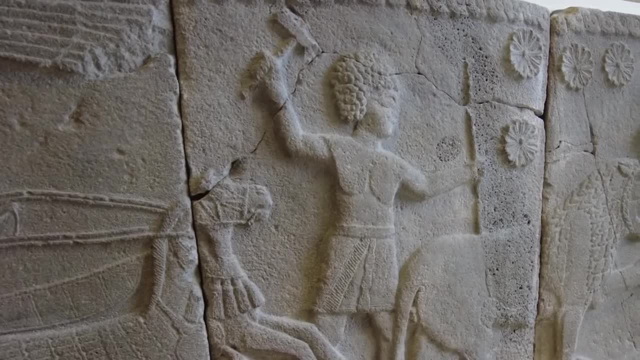 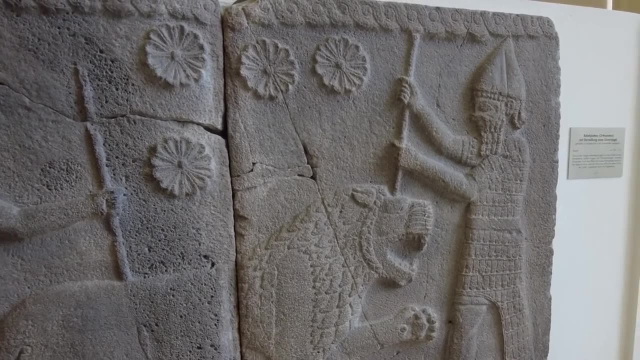 rendering of the name of the city, which the original Sumerian inhabitants referred to as Shardish. The people of the nearby rival city of Lagash referred to Uma as Gishkushu in their texts. It was during the Ur III dynasty. 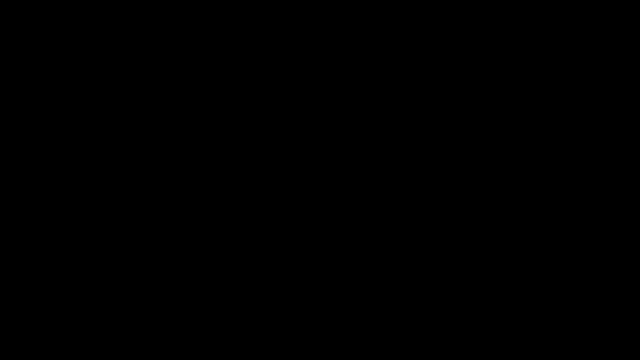 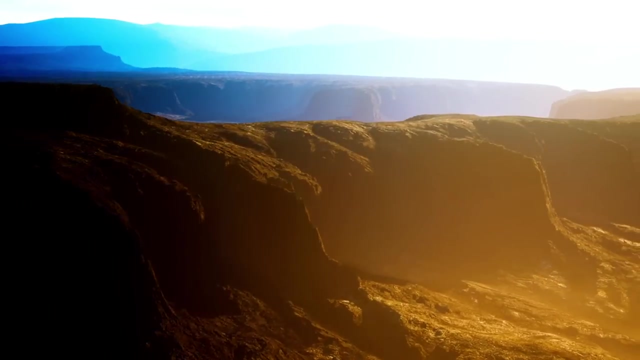 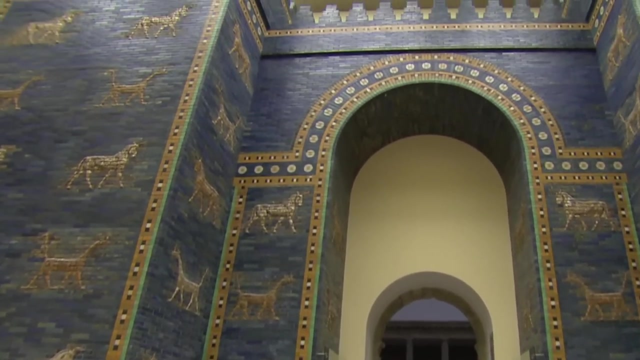 that the locals began referring to their city as Shauma, which became Uma in later Babylonian texts. Uma may also have been referred to as Kisha by Akkadian speakers in the old Babylonian period, Thus properly identifying the city and determining that it had many different names. 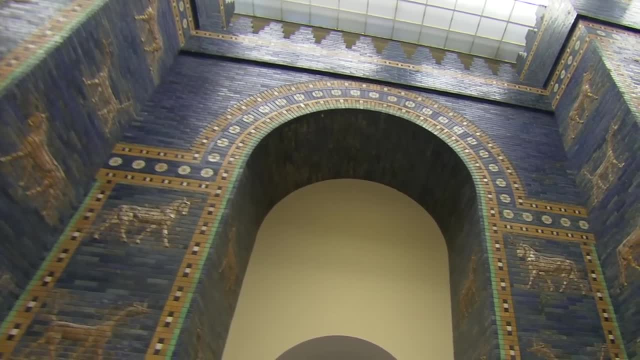 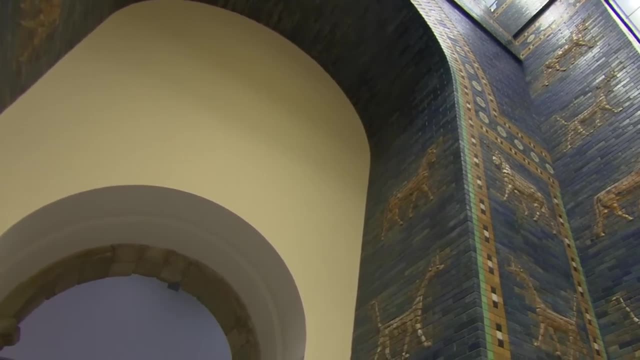 was the first impediment to uncovering Uma's secrets. Modern scholars were then faced with the task of unearthing as much of the city as they could from the fields of Iraq. The discovery of Uma happened after Europeans flooded the region in the mid-19th century. 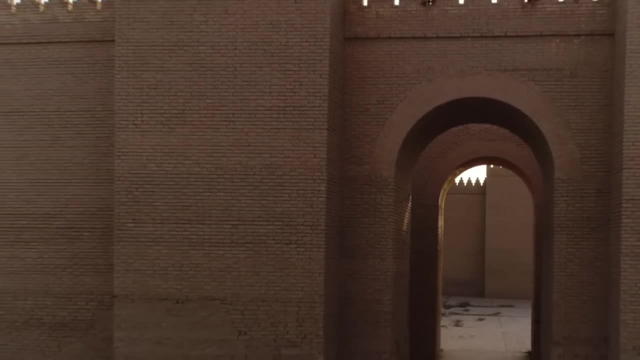 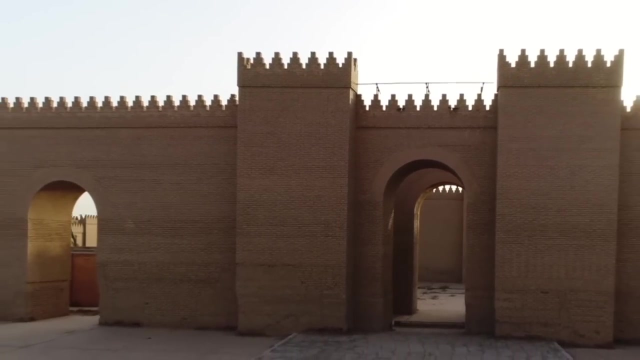 which came in the aftermath of the Enlightenment. During the Enlightenment, historians shifted from the religious and mystical to a more scientific understanding of the past. With that said, much of the impetus that drove people to unearth Mesopotamia in the 1800s. 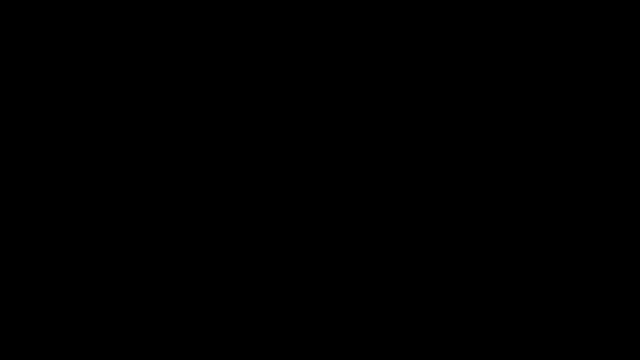 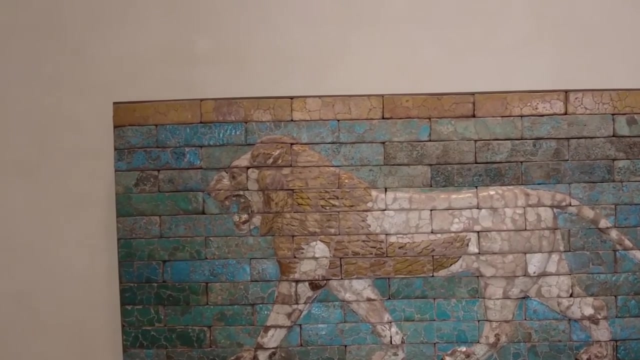 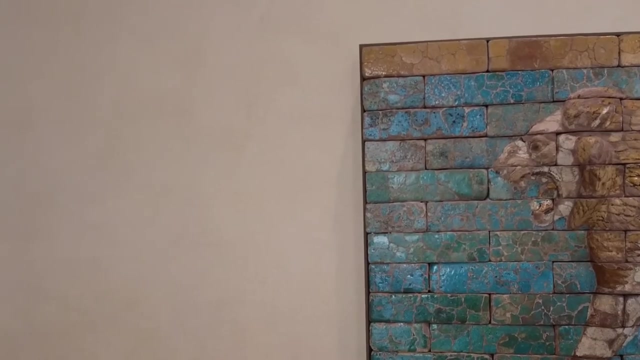 was based on a desire to discover the locations of cities mentioned in the Bible. Although Uma was not a city mentioned in the Bible by name, the nearby center of Uruk, Erek and Ur are featured in a number of verses, so the initial discoveries and excavations of those sites, 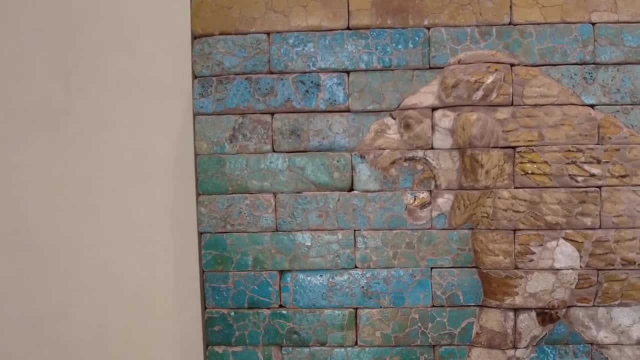 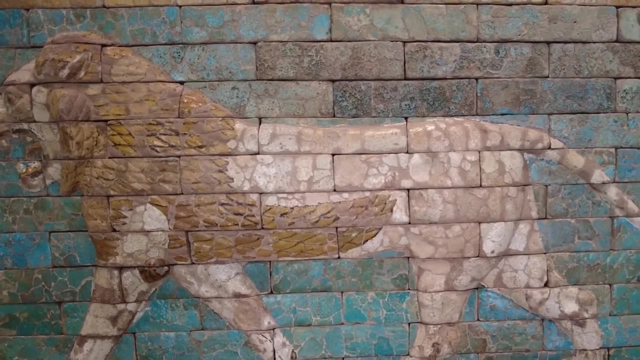 helped to open up Uma to a certain extent. Uma was eventually identified with the modern site of Tell-Yukah, But in recent times academics have argued that another village named Um al-Aqarib, which is about five miles from the city. 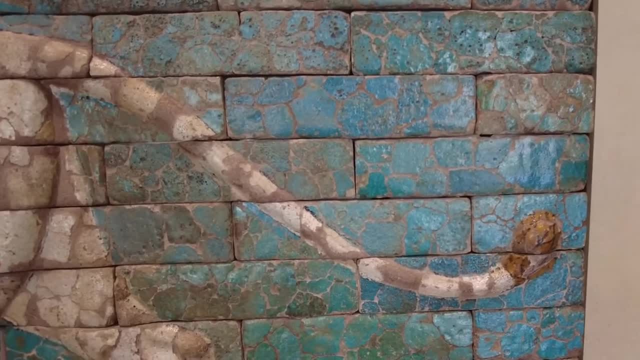 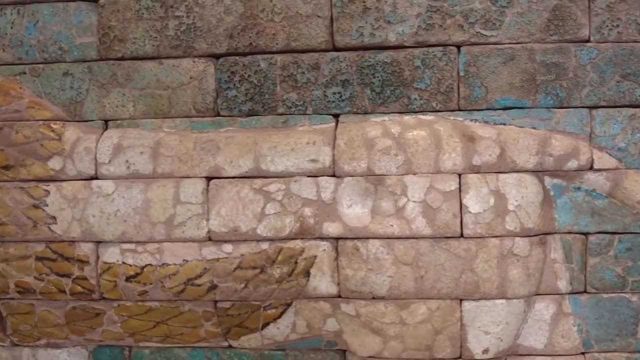 which is about five miles from Tell-Yukah, was Uma. If anything, Uma was much more than the city of Uma proper. By the time of the Ur dynasty, Uma was actually a region that encompassed several smaller towns and villages, as well as an immense rural area. 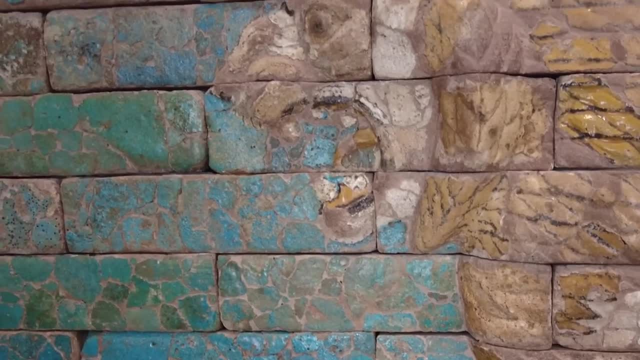 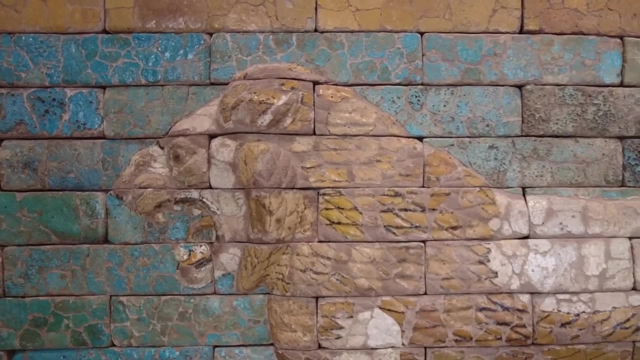 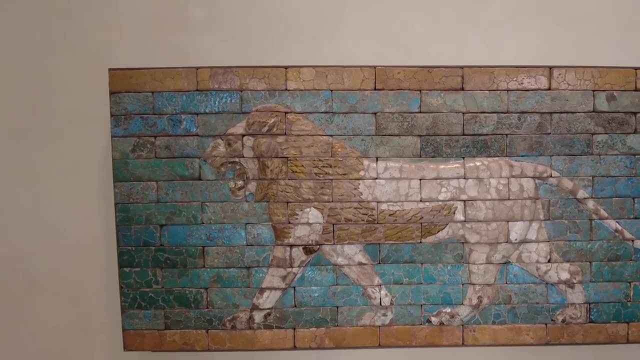 So pinpointing the actual location of urban Uma may be difficult. Taking that into account, distinguishing one site from another may be almost impossible, especially considering the state of decay that has taken place at the sites over the last 150 years. The area of what is today believed to have been Uma. 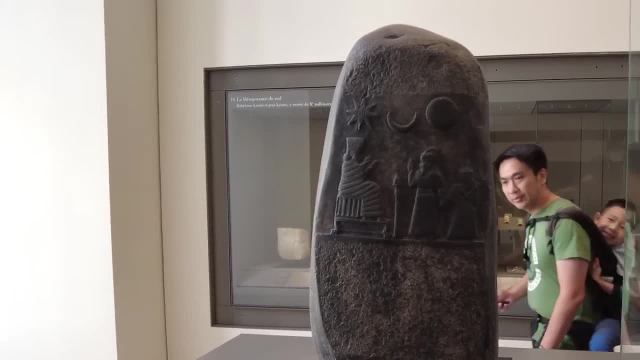 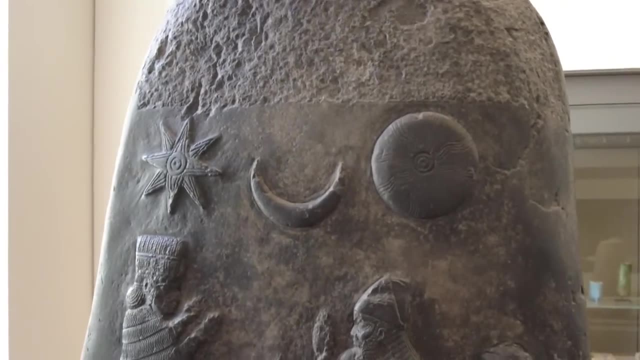 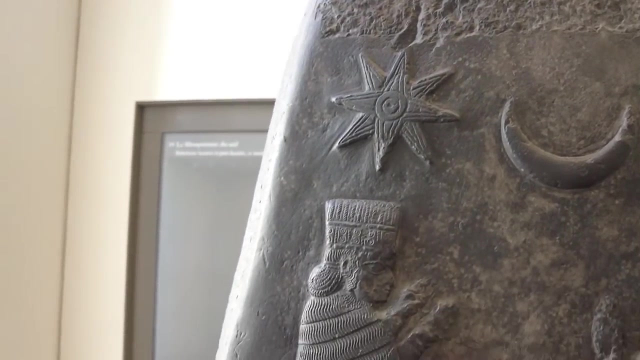 lies on the northeastern edge of the more heavily excavated areas of the 20th century archaeological missions. The site was first recognized and visited in the late 19th century by early British archaeologist William Loftus and American scholar John Peters, But neither one conducted any long-term. 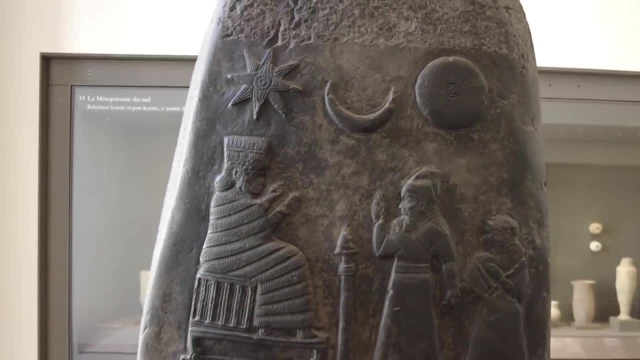 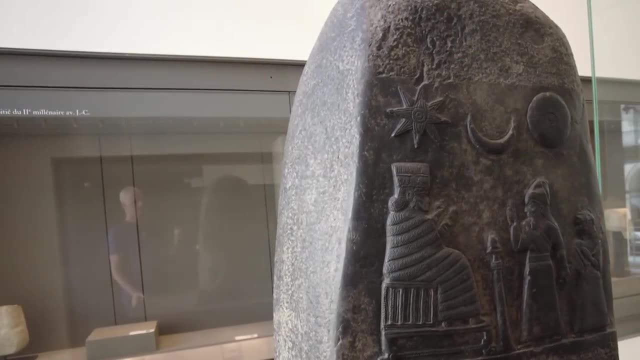 or in-depth work at the site After excavations began in earnest throughout Mesopotamia in the early 20th century, Uma was for the most part overlooked by archaeologists, but others found value in the ruins. In 1911, many of Uma's tablets were looted. 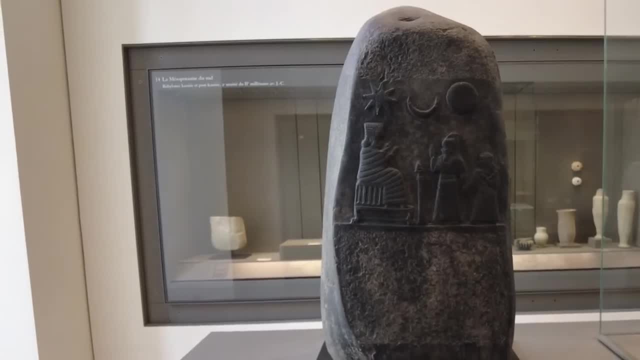 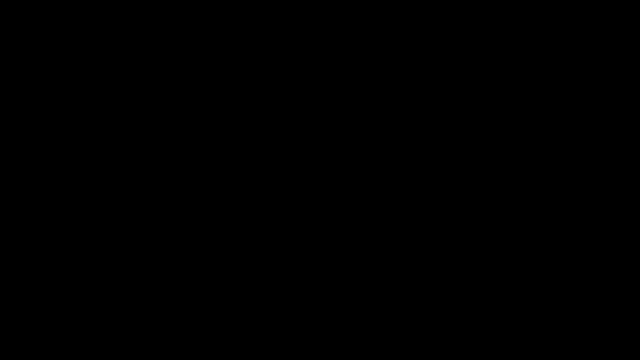 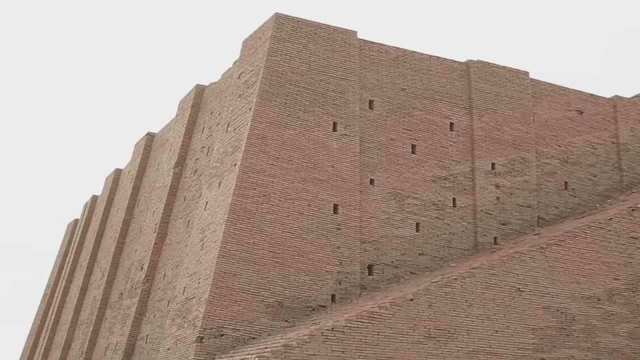 from the site and sold on the black market. Fortunately, most of the tablets ended up in museums throughout the world, where they have been studied, and they have provided valuable insight into Uma's social and economic life. Since World War II, German archaeologists have carried out: 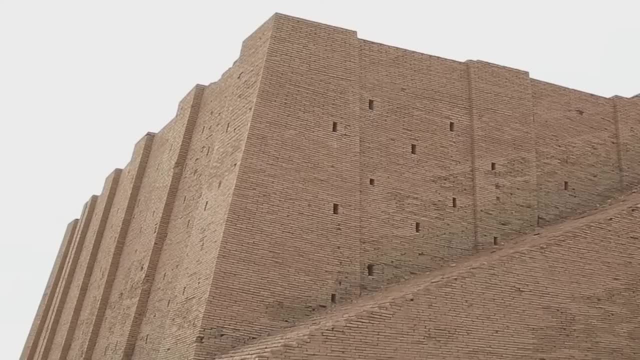 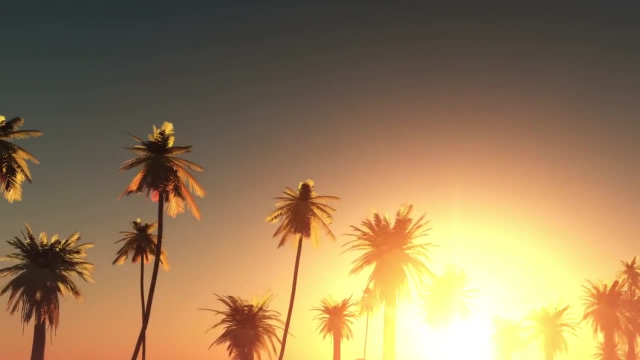 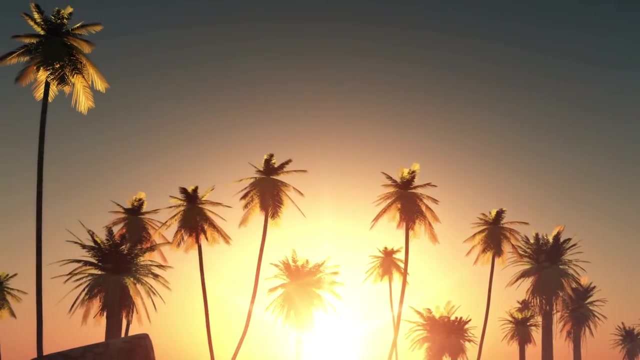 most of the digs in southern Mesopotamia as part of the Uruk Varka survey, although, again, Uma has remained at best of secondary importance to most. Saddam Hussein's regime protected foreign archaeologists which allowed excavations, and Iraq protected Mesopotamian antiquities. 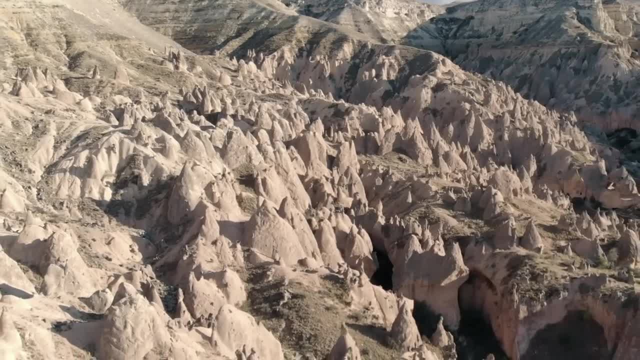 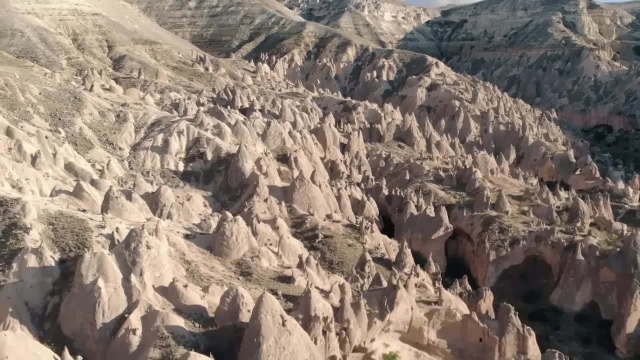 in general from looters and the black market, as the sites and artifacts adhered to Hussein's propagandist worldview of a greater ancient era. As a leader who was arguably more secular than religious, Hussein often promoted elements of Iraq's pre-Islamic past. 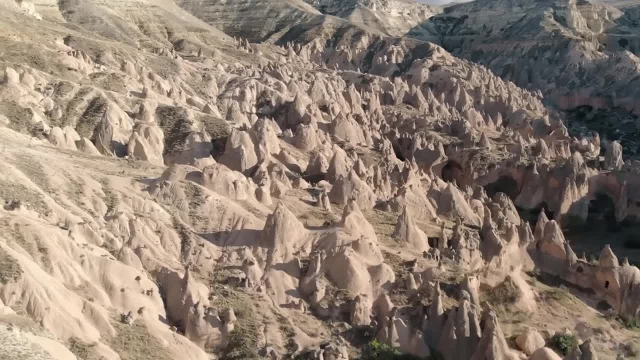 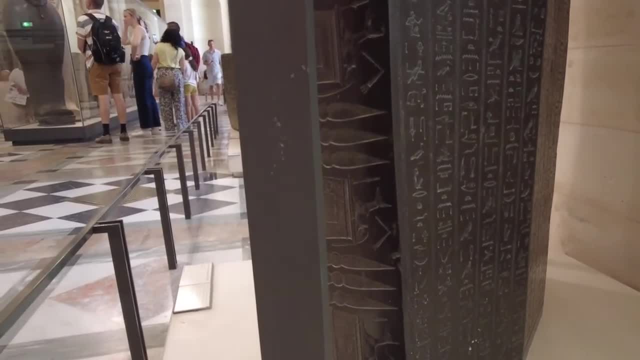 as a sign of its greatness, and his regime constantly asserted that Iraq was home to one of the planet's first civilizations. However, the collapse of Hussein's regime brought destruction and devastation to Uma and many of the other sites in Mesopotamia. 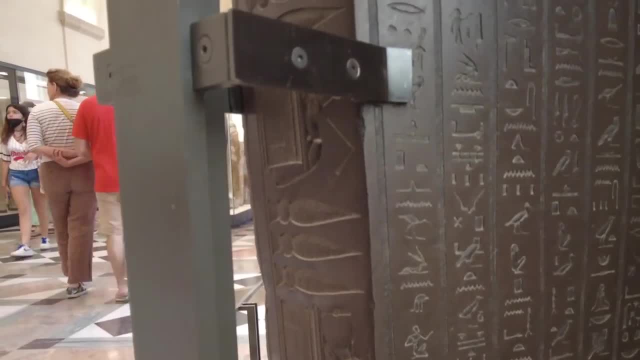 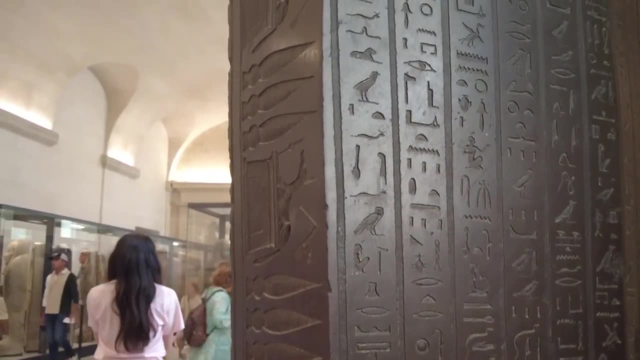 Coalition air bombings in 2003 hit the site, which was followed by another wave of looters at the site and Iraq's antiquities museums. In the end, the site was left with trenches and holes that all but leveled the surface of what was visible. 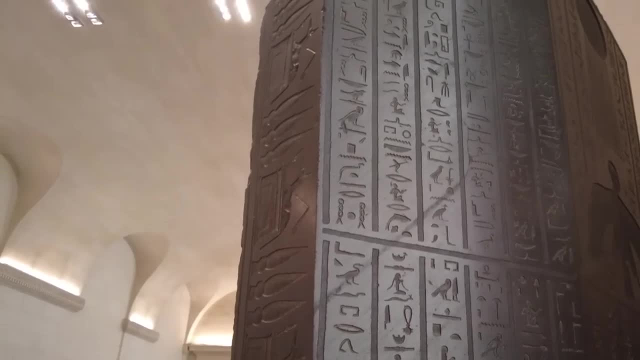 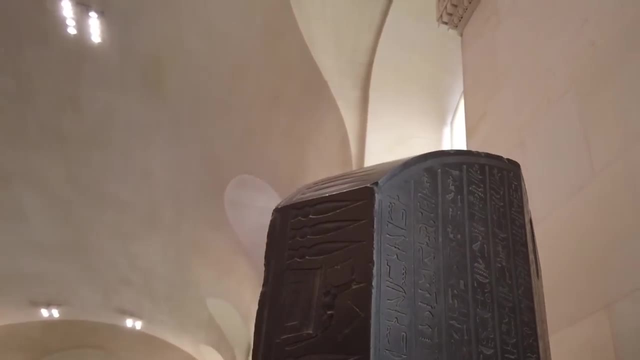 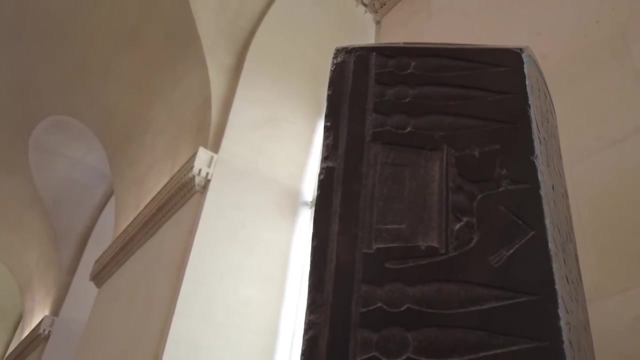 Due to the current political instability in Iraq, it is unlikely that any major archaeological work will unearth the mysteries of Uma any time soon. The precise size and even the layout of Uma before the Ur III dynasty is difficult to determine. Mesopotamian cities in general. 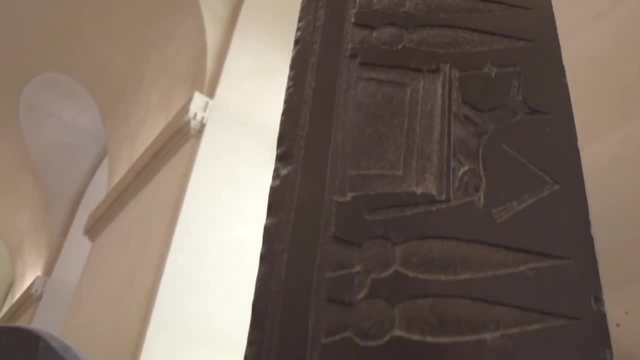 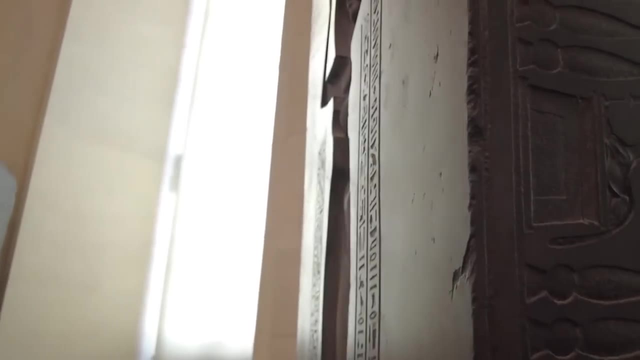 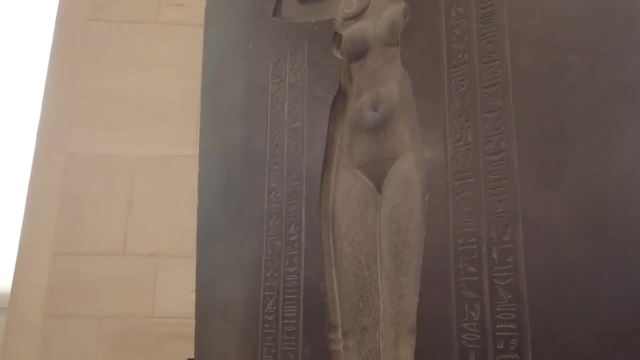 did not have closely delineated boundaries and usually included a large agricultural area that was several times larger than the city itself. Most of the inhabitants of Uma were employed in the agricultural sector in some way, which included the small number of artisans and merchants who sold goods to the peasants. 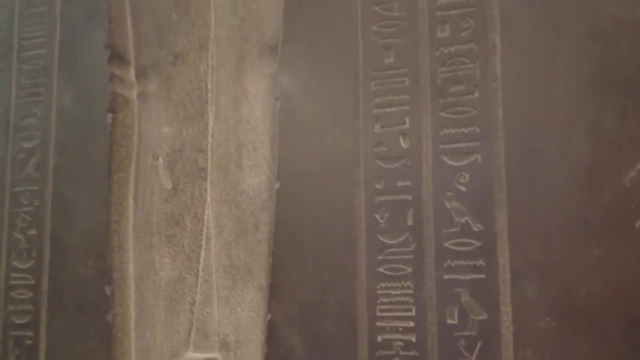 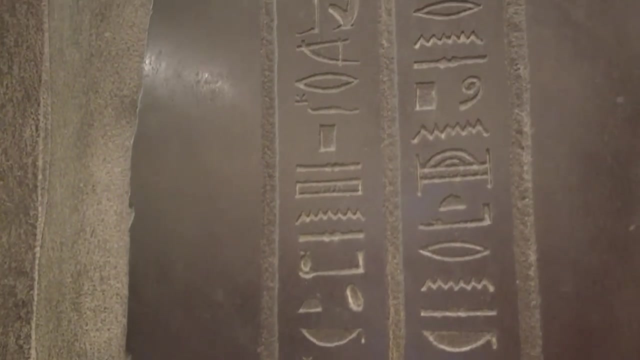 Excavations and texts have shown that Uma had a wall in the first part of the early dynastic period, indicating that it was large enough to need protection from other city-states Throughout most of Uma's early history, the city that it competed most with, 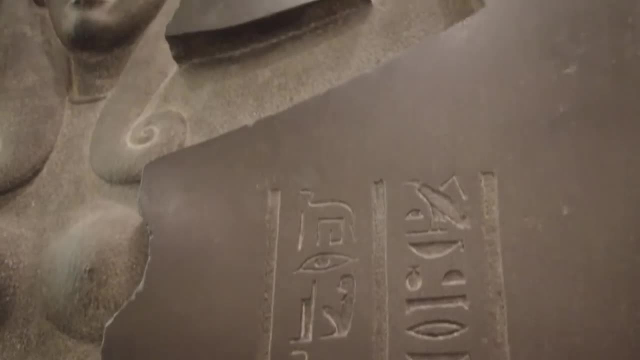 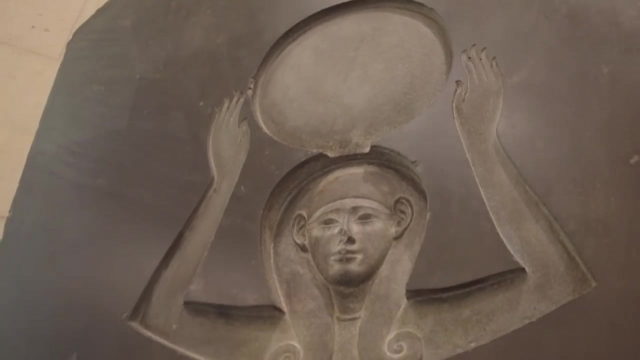 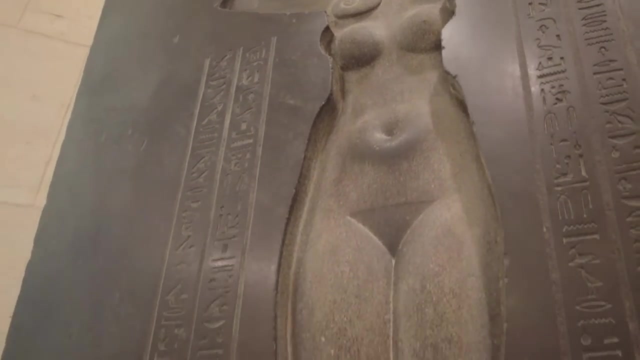 was Lagash Around 2450 BCE. Uma's history becomes a little clearer thanks to texts that describe its endearing competition with Lagash over control of the fields and canals in the region Located a little more than 50 miles to the east of Uma. 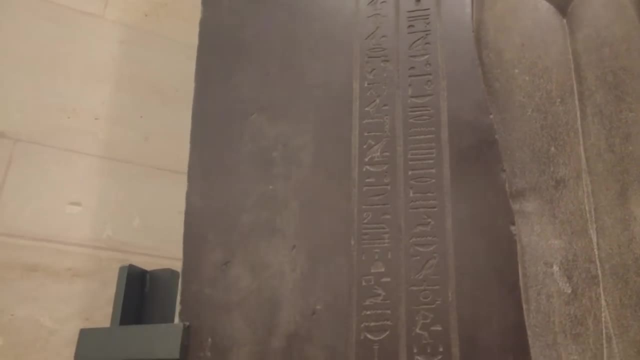 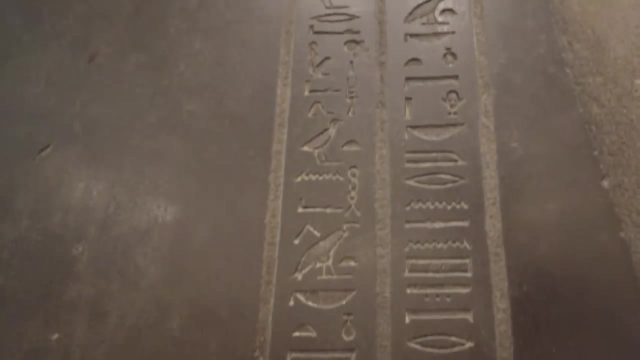 Lagash was the other major player on the alluvial plain. As ethnically diverse as ancient Mesopotamia was, Lagash was even more politically diverse. especially in the early dynastic period, Each city of Mesopotamia represented a separate city-state. 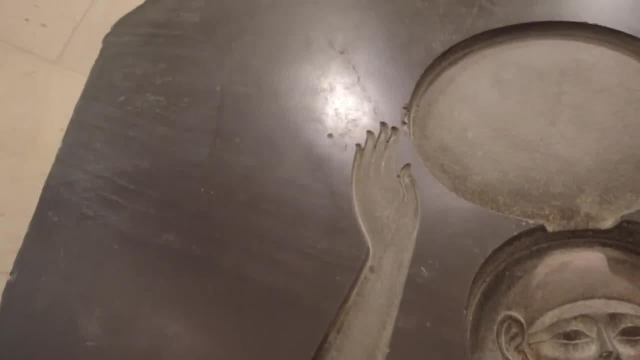 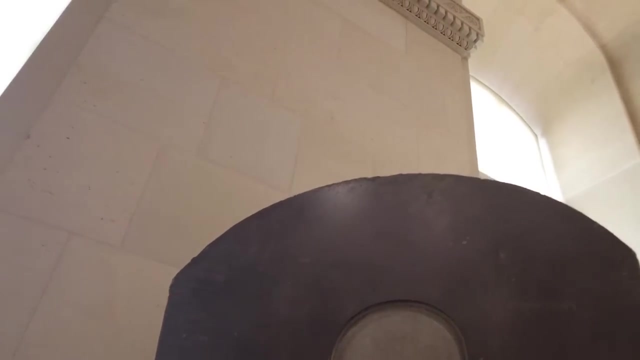 that was ruled by a king who patronized a specific god or goddess, which meant that, even though all of the early dynastic city-states followed essentially the same religion, with the same basic pantheon, the god of a particular city took precedence over all others. 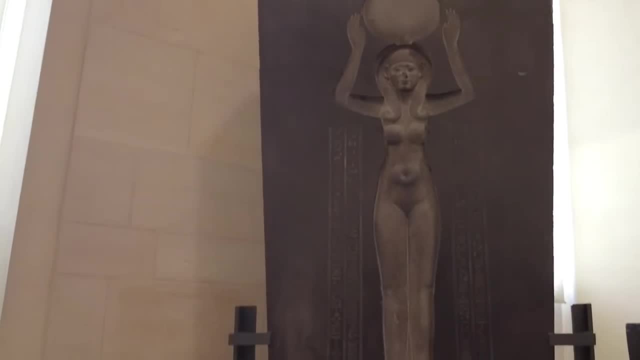 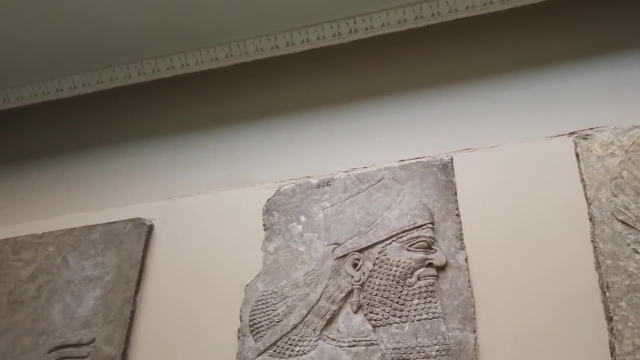 Religion may have played a role in some of the city-state conflicts of the early dynastic period, but wars were more traditional in nature, motivated more by the desire for power and the acquisition of resources. Mesopotamia may be one of the most productive. 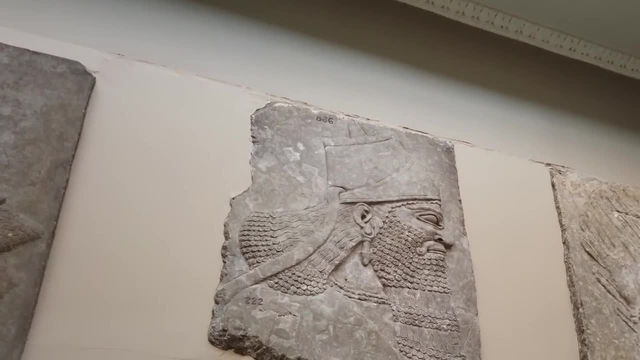 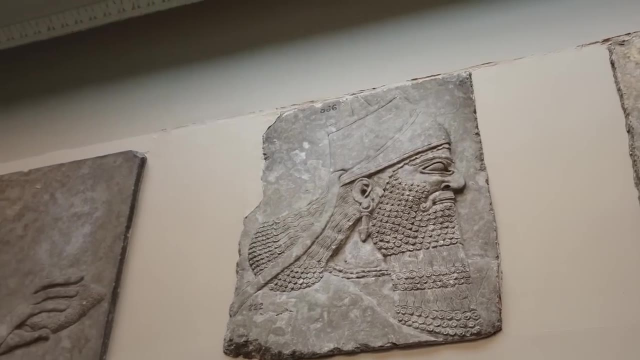 agricultural tracts of land in the world, but it is devoid of other resources and it is also densely populated. Wood often needed to be imported into the region, and although cropland was abundant, the ever-growing population meant that land became a premium. 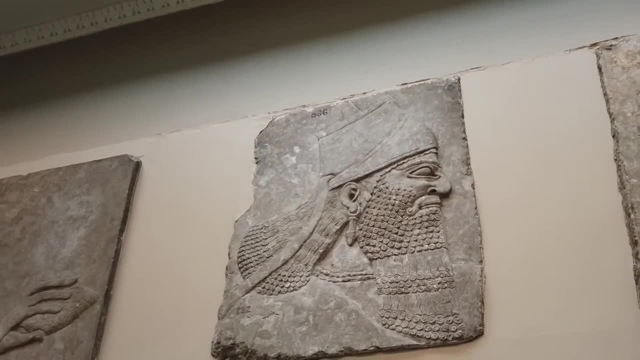 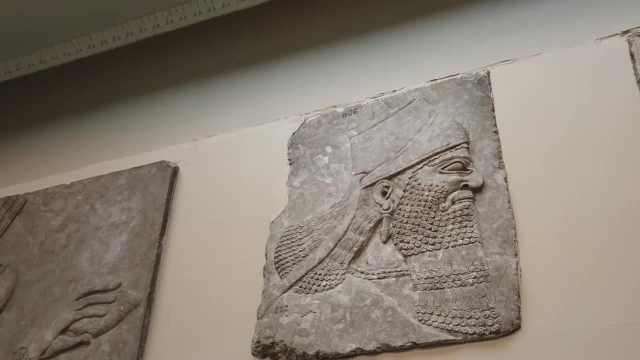 and something that many city-states were willing to go to war over to acquire. Mesopotamia was filled with thousands of canals that brought water to the people and the fields and also served as a medium of transportation. so croplands and canals. 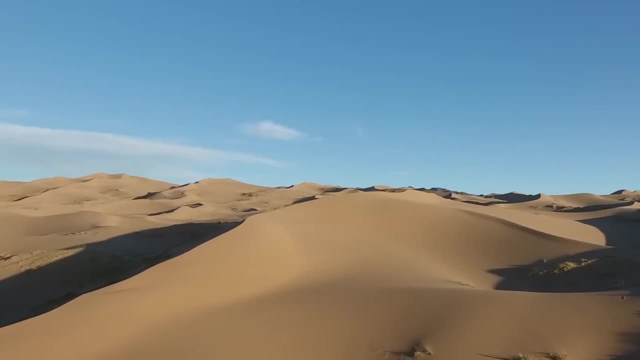 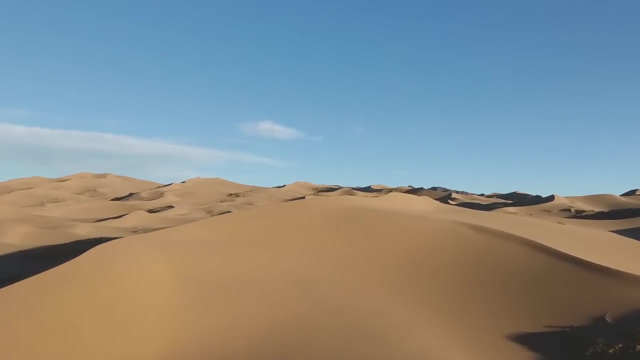 often became sources of conflict between the city-states, and the enduring conflict between Ulna and Lagash was the best known and most documented in early dynastic Mesopotamia. Most historians believe that the conflict was simply a border conflict for resources. 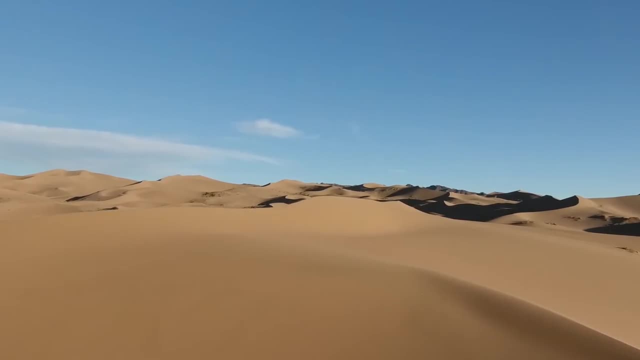 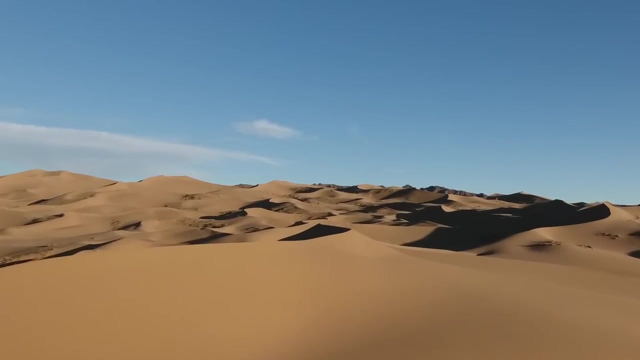 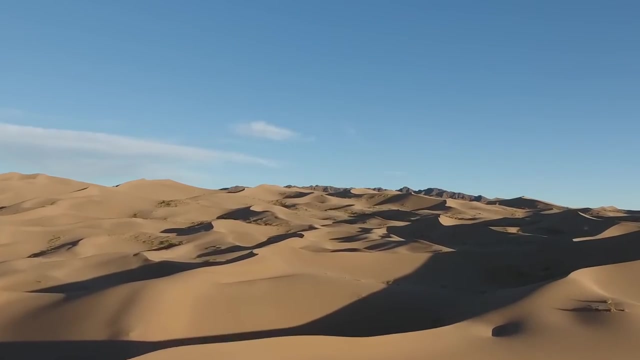 but in many of the texts it is depicted as a war between Shara, god of Uma, and Ningirsu, the patron god of Lagash. This has led some historians to believe that the conflict was actually religious in nature, or that it had at least a religious component. 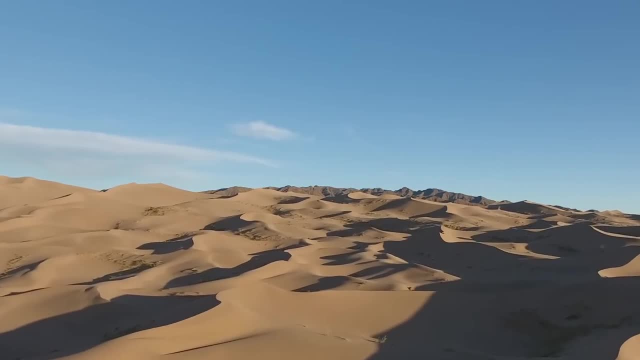 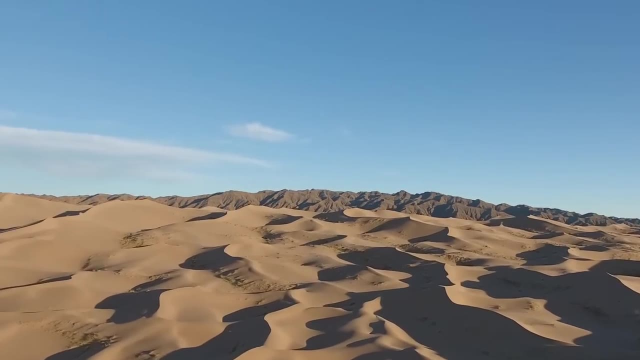 Although this argument has been advanced by some respected individuals, such as Daniel Snell, most others believe that religion actually had little to do with the two cities' conflict. One of the most prominent Mesopotamian historians, Thorkell Jacobson. 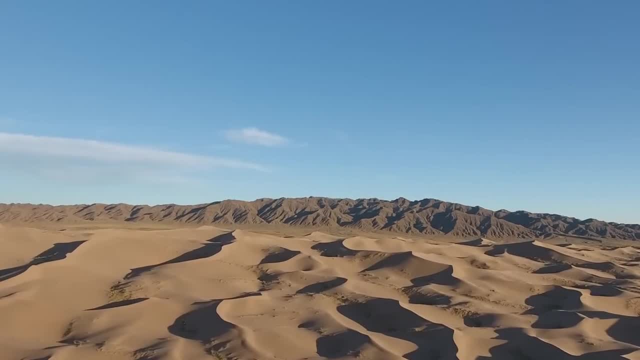 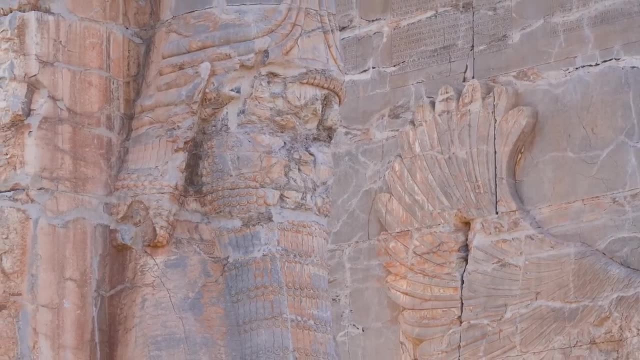 pointed out that King Iannatum of Lagash actually depicted Shara as rejecting Uma and its rulers. Iannatum was therefore not going to war against Shara, but against those who failed to worship him properly. The fact that King Iannatum 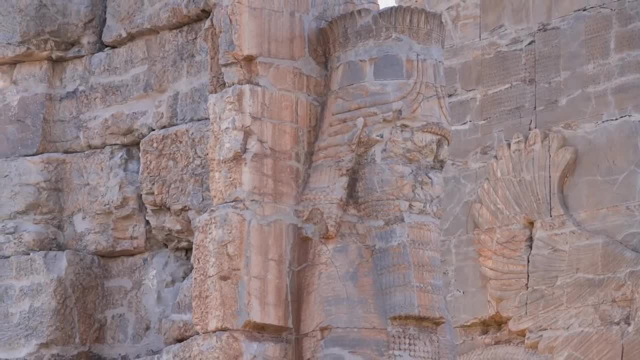 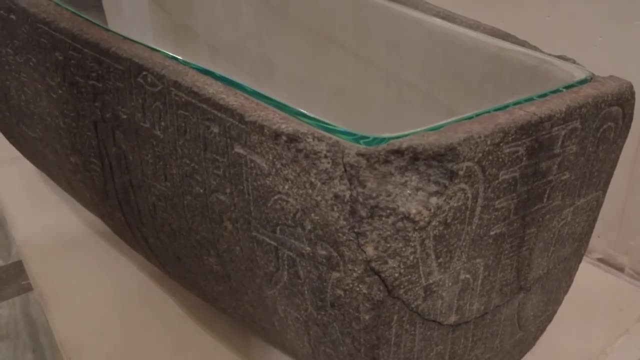 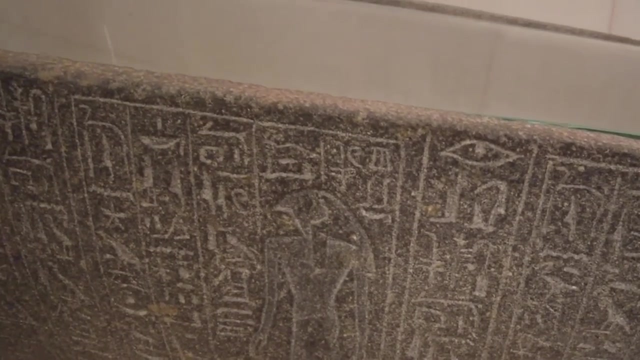 can even be identified as evidence of the fact that many groups in ancient Mesopotamia recorded king lists from the dawn of their history. In some cases, the lists went all the way up until the Seleucid Greeks took control of the region, although the lists varied in accuracy. 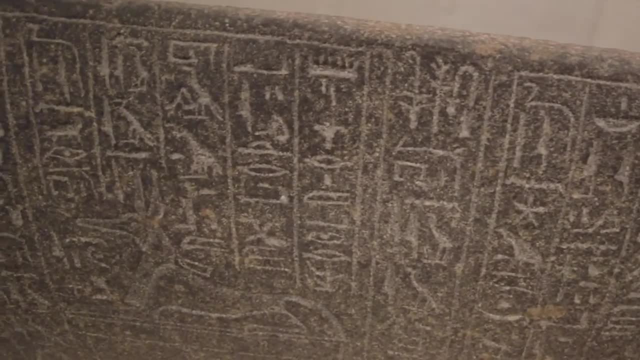 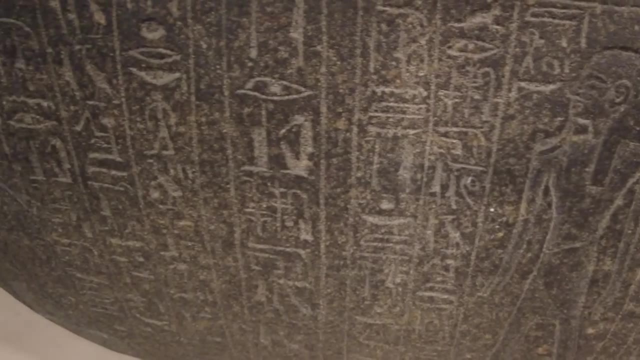 depending upon the city and period. The longer back a list went, the more it tended to mix myth with history, and many of the less important cities were nearly overlooked altogether. Uma was lost over for the most part in the early king lists, but fortunately, a number of other documents. 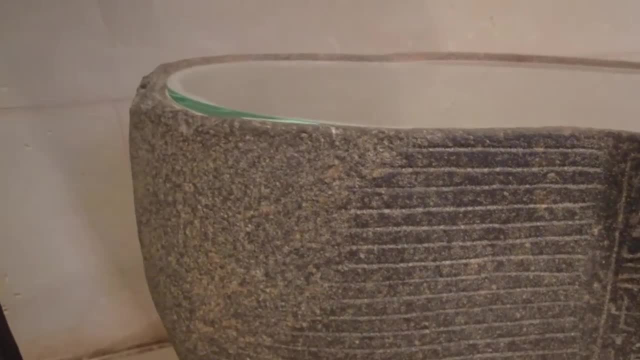 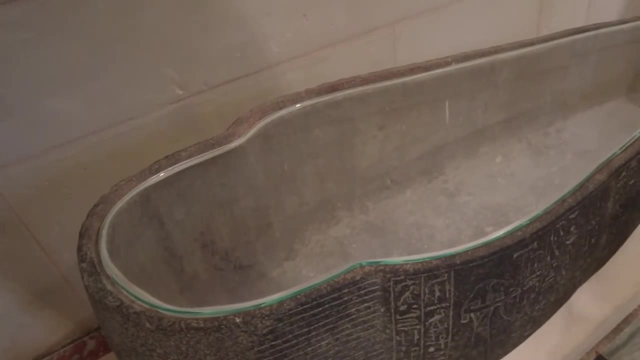 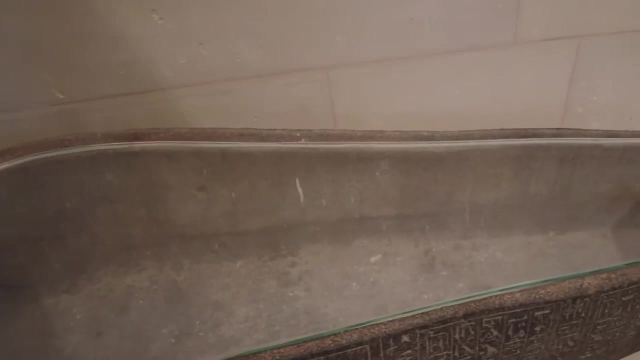 have made it possible to reasonably reconstruct Uma's royal chronology. A combination of royal inscriptions and administrative documents from Uma, along with similar documents from rival city Lagash, have been utilized to create an accurate chronology, albeit one where the dates of each king's rule 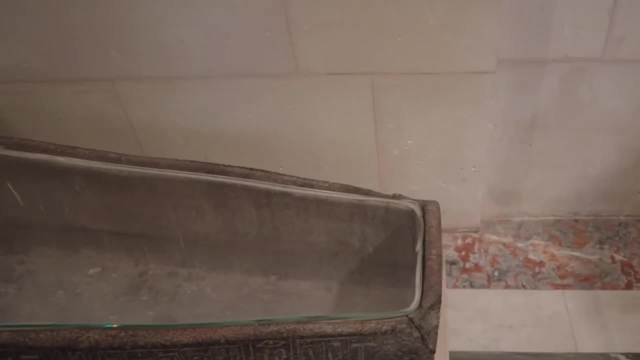 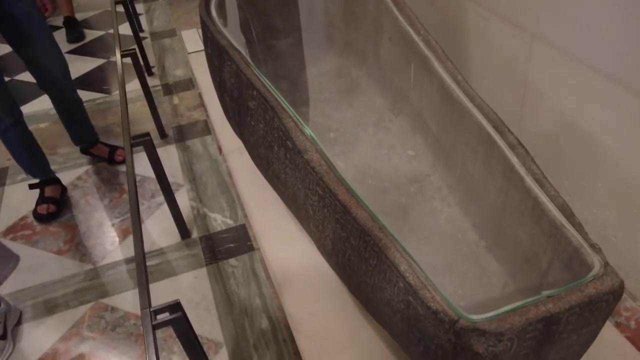 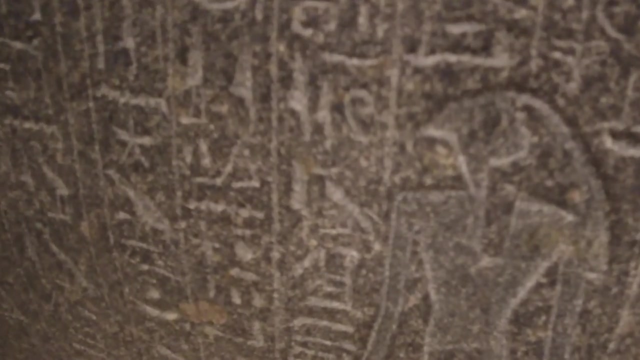 are far from precise. All of the rulers of Uma in the early dynastic period held the title ensi, which was equivalent to governor instead of king. to a certain extent, The Sumerian word had a somewhat wide-ranging and subjective meaning. so even as the ensis of Uma, 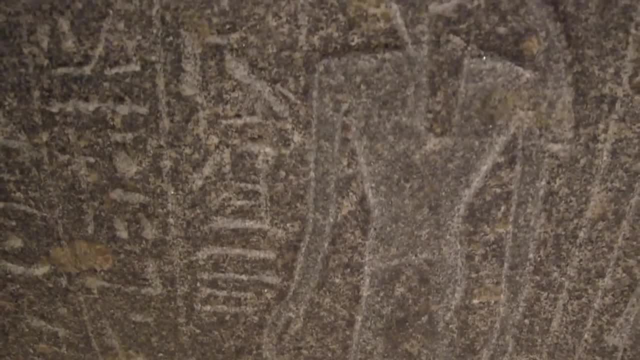 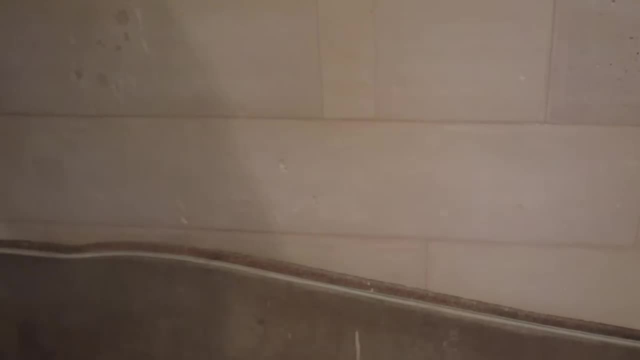 were not considered kings in the early dynastic period. they essentially behaved as kings by establishing true dynasties. The ensis of Uma also had complete power over the city-state, as they were not beholden to any other power, Unless they were defeated in war. 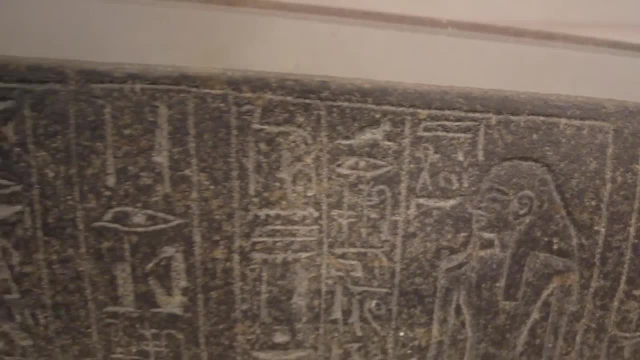 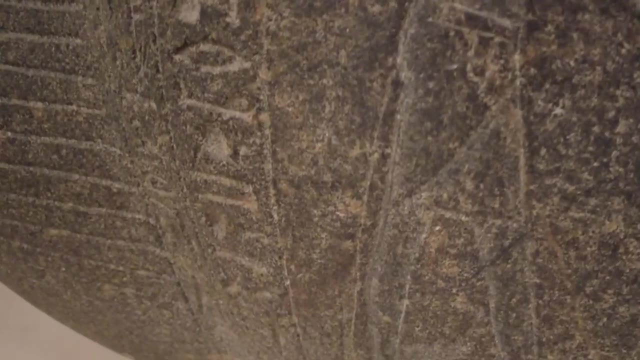 The ensi decided tax rates, conscripted workers into the army or work gangs and lived in a palace. By all accounts, the early dynastic ensis of Uma were kings, just not in name. Later, in the third dynasty of Ur, 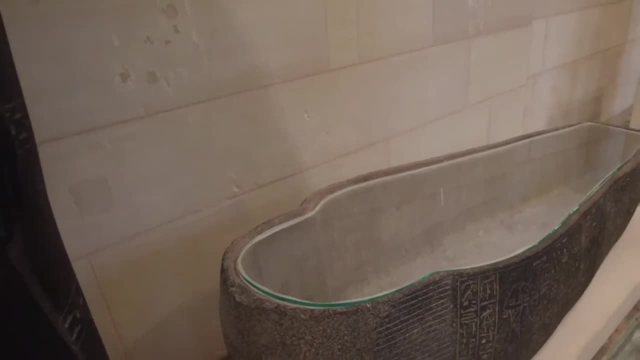 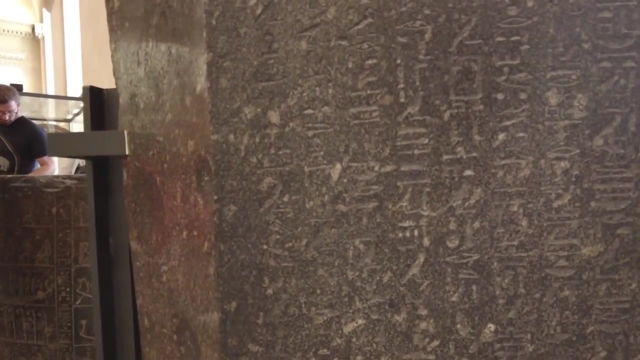 the ensis of Uma acted more as regional governors who were subservient to the kings of Ur, but before that time they were totally independent. The first ensi of Uma known from inscriptions is Pabulgagaltuku, who, according to an inscription from Lagash: 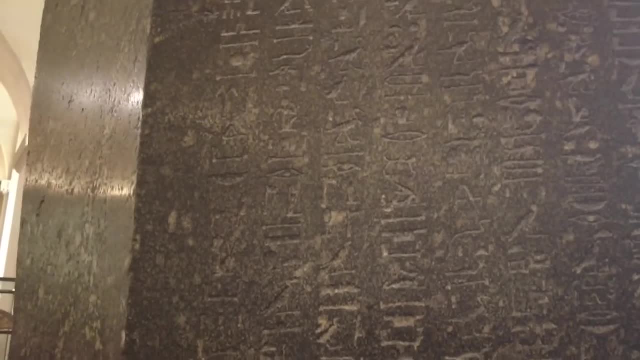 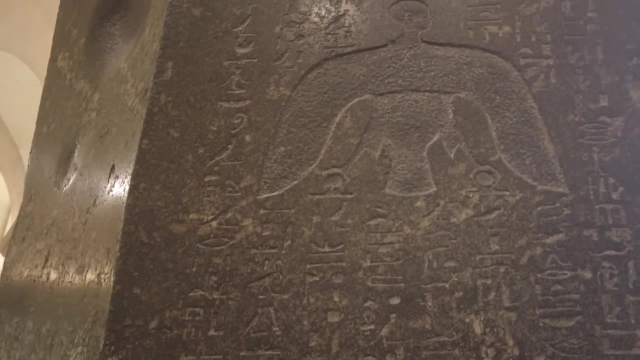 was defeated by Ur-Nanshi of Lagash. The text reads: he seized Pabulgagaltuku, the governor of Uma. It is unknown what Ur-Nanshi did once he seized Pabulgagaltuku or what exactly was meant by that. 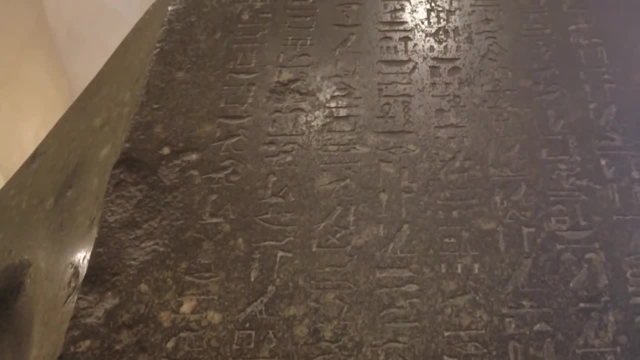 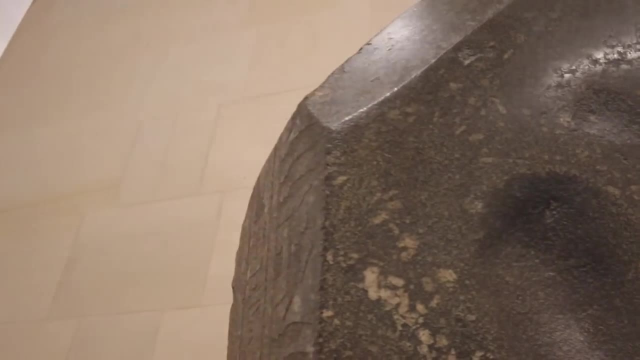 The Uma ensi may have been imprisoned or killed by Ur-Nanshi, or it could have been a case of hyperbole on the Lagash ruler's part, which was extremely common in ancient Near Eastern texts. What is known about Pabulgagaltuku, though? 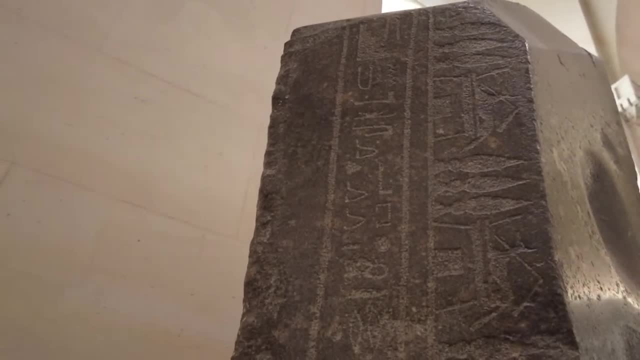 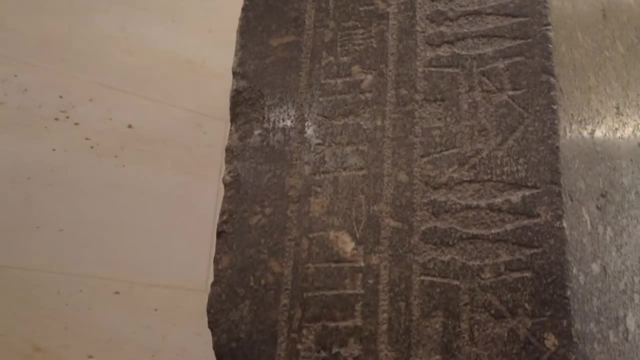 is that it was during his rule that the more than 100 years of conflict between Uma and Lagash began. Thus, while the fate of Uma's first known ensi is unclear, it is known that the conflict between Uma and Lagash became more well recorded after his rule. 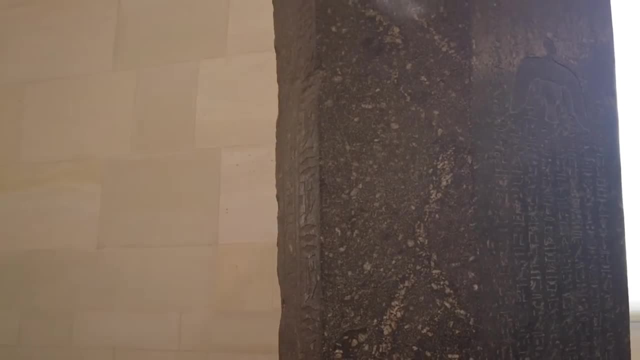 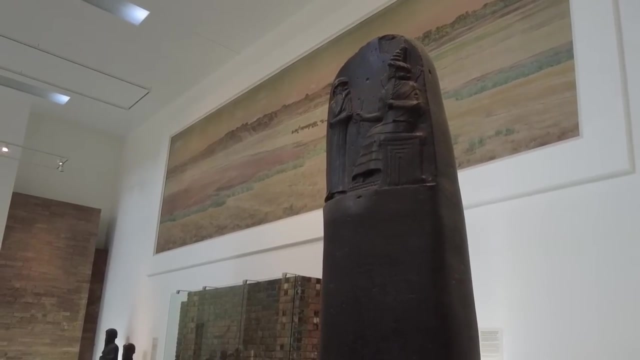 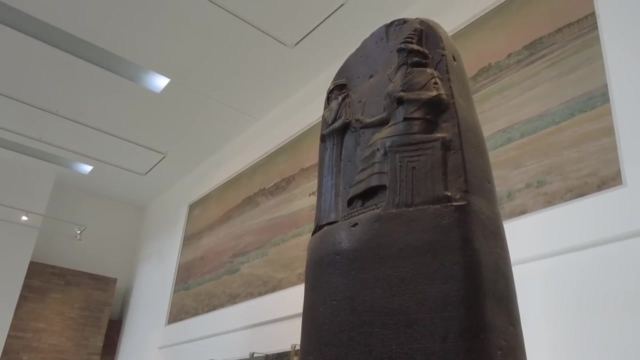 Pabulgagaltuku was succeeded by Minta, who continued and apparently intensified the war with Lagash Again. it may just be that the conflict became better recorded at this point, but it would also stand to reason that Lagash felt it had the upper hand after defeating Pabulgagaltuku. 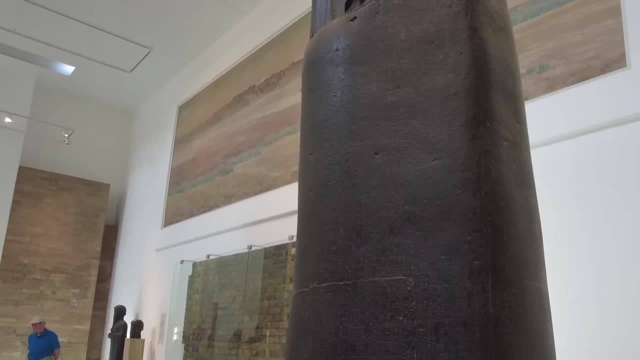 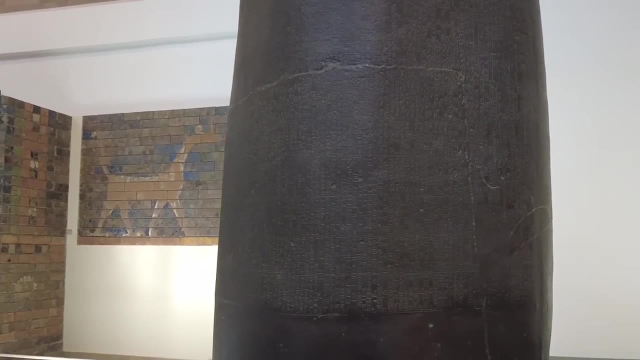 and that, conversely, Uma felt compelled to retaliate. This will be discussed more below, because it was the primary focus of the Stele of the Vultures, And though Minta is not referred to by name, on the Stele of the Vultures. 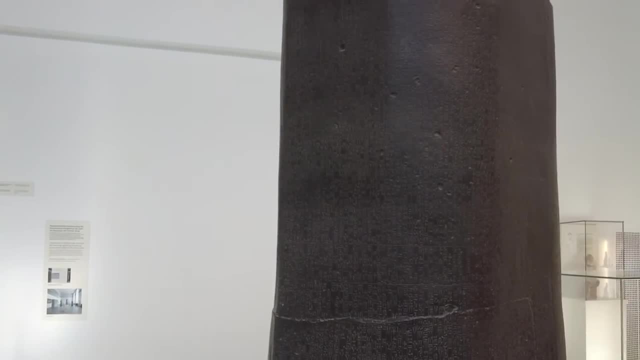 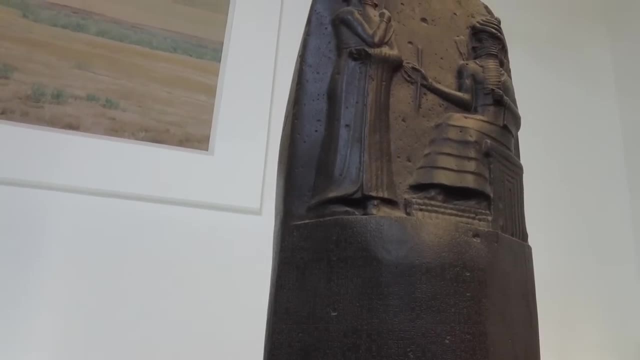 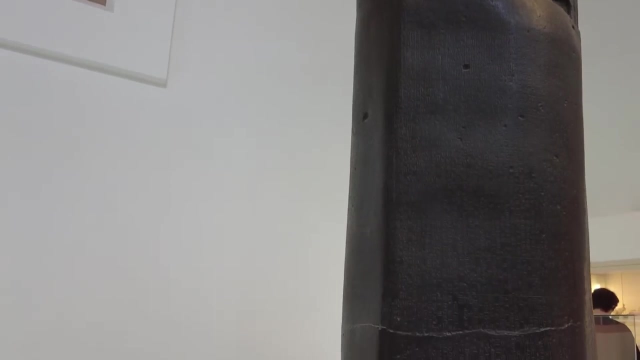 historians have believed for some time that he was the Uma ensi in question. The fact that he was never mentioned by name in a text from Lagash is not so surprising because in ancient Near Eastern texts, the writers composing the text were more important than the other. 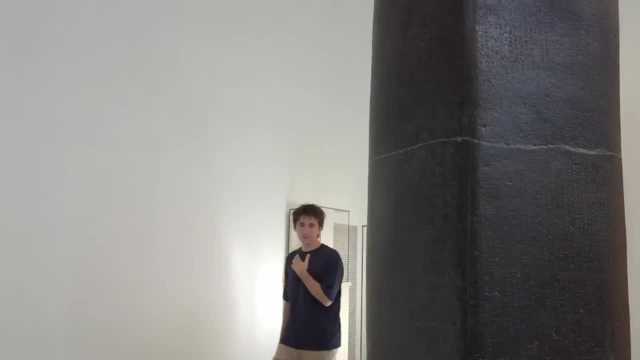 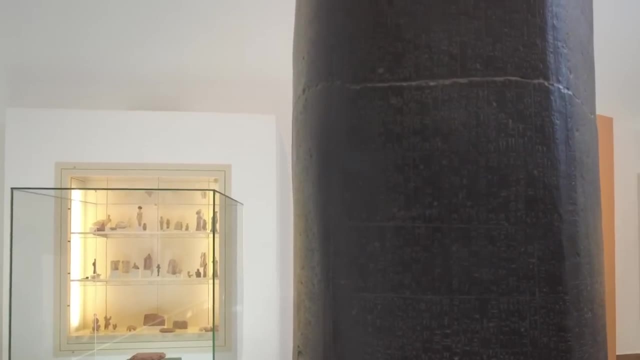 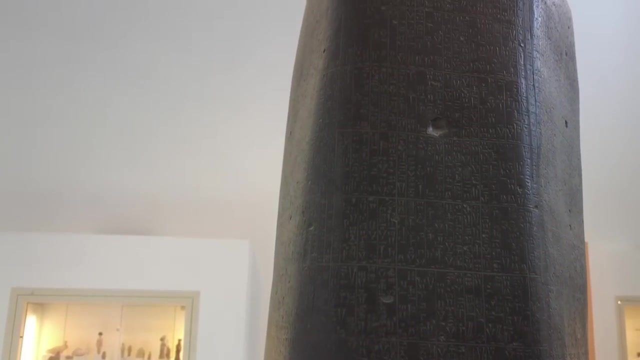 Lagash was the primary agent and the subject of the text. so readers only had to know that Uma was the hostile force and Uma's ensi and power was of little concern. Enakale followed Minta as ensi, but little is known about Enakale from native Uma texts. 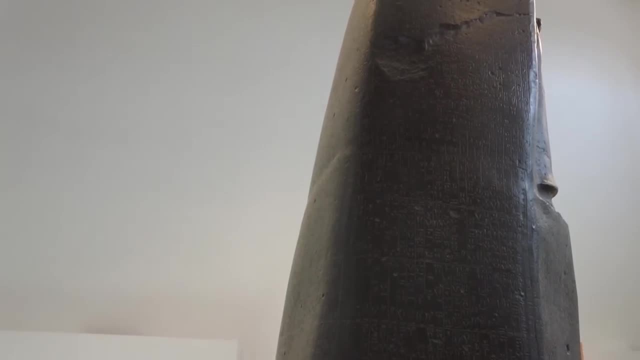 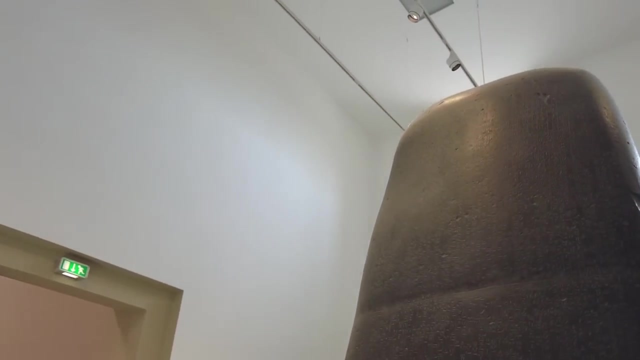 All of the extant texts from Enakale's reign come from Lagash, so they are almost certainly somewhat biased, but they still offer a couple of interesting, relevant historical nuggets. Like his predecessors, Enakale was referred to as ensi. 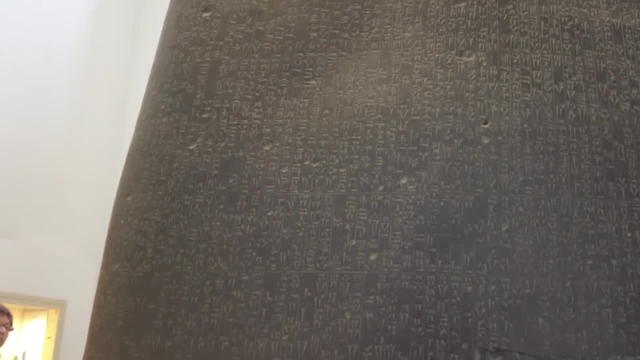 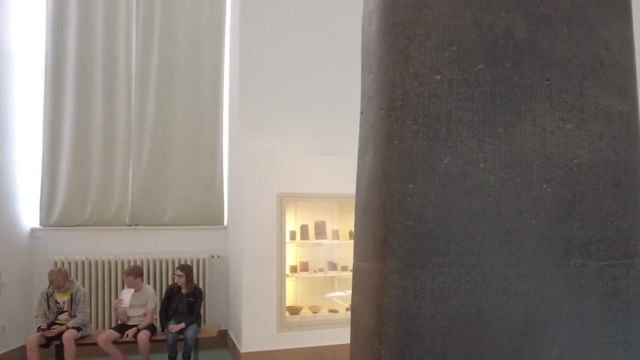 instead of the Sumerian word for king Lugal, which again may say more about the nature of Sumerian history and geopolitics than the reality on the ground. Enakale may very well have considered himself a king Lugal. 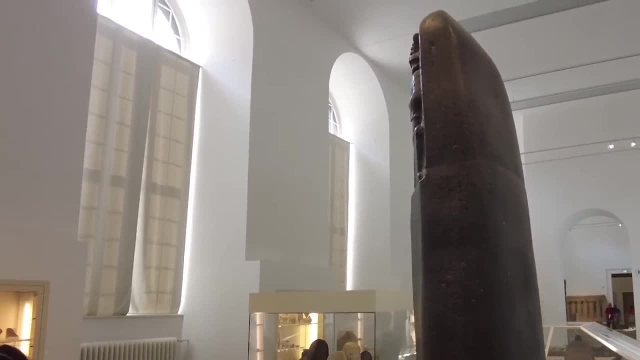 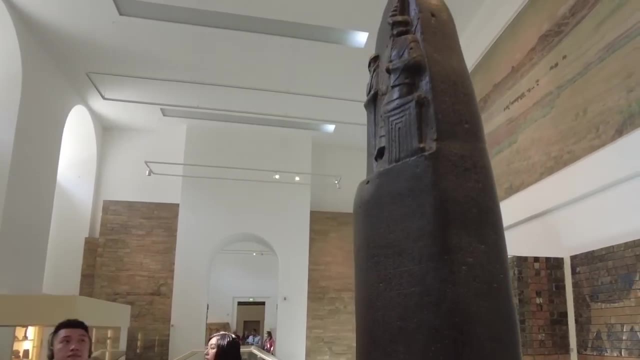 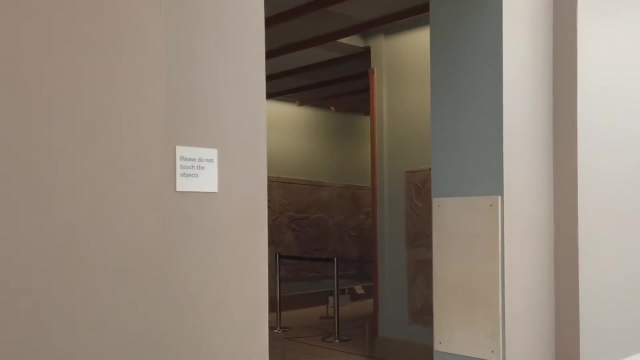 but the rulers of Lagash would never have given him that respect, considering their on-going war, even as the rulers of Lagash in the same period did in fact refer to themselves as kings in inscriptions. A text from Lagash states that Enakale came to an agreement. 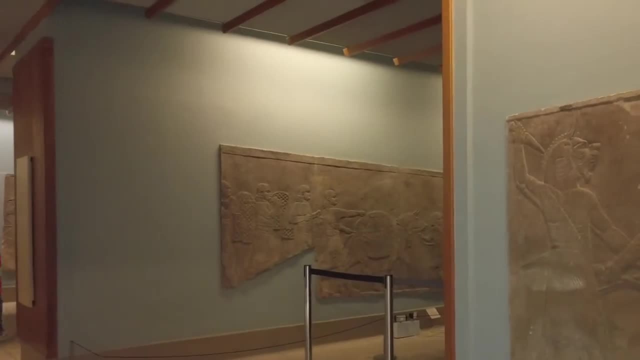 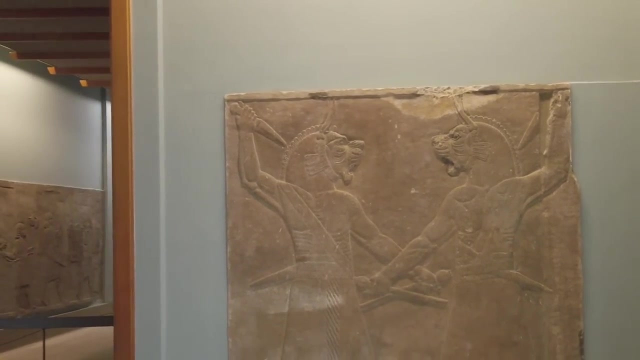 with Lagash over the border, thereby putting a hold on their conflict. Since there are no extant administrative texts from Enakale's reign, his length of rule is unknown, but based on a discovered legal document, he ruled at least eight years. 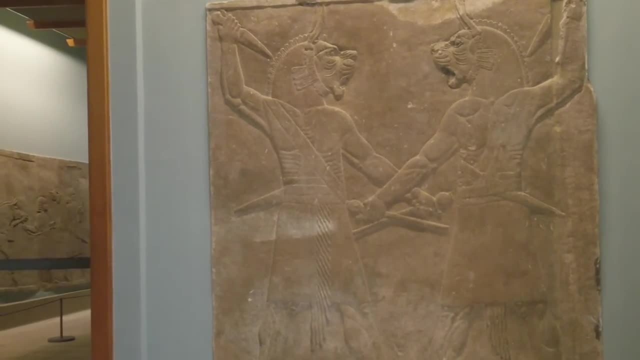 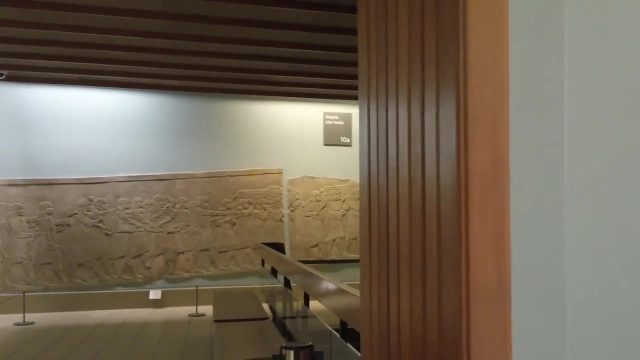 Enakale is probably best known for being the father of Uruma, the next ensi. Uruma continued the tradition of going to war against Lagash, and two votive inscriptions offer some indication on how the conflict between Uma and Lagash was renewed. 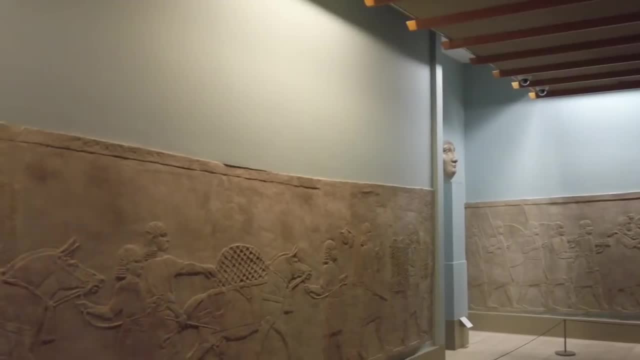 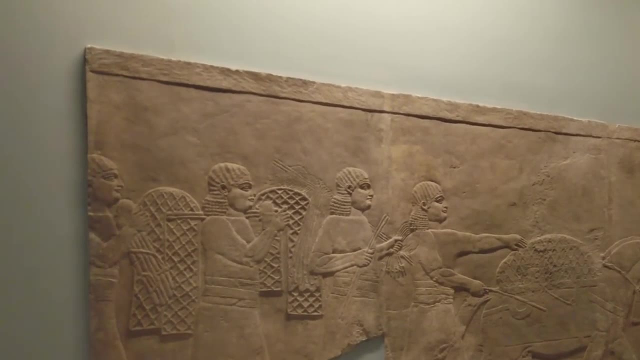 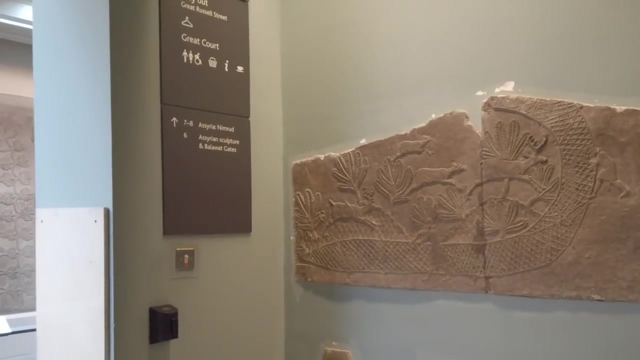 but not necessarily why. According to these inscriptions, Uruma simply quit paying the loans of barley that were imposed on Uma by Lagash. In fact, the Uma ensi not only refused to make the payment, but, according to the text, he took things even further. 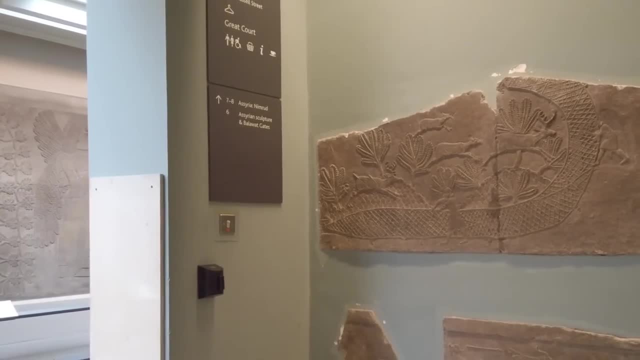 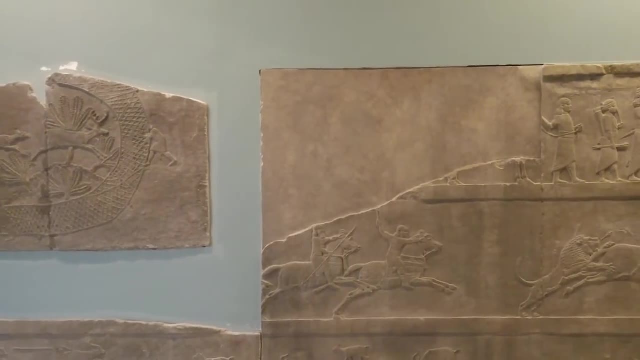 Since he was unable to repay that, barley Uruma, the governor of Uma, diverted the water from the boundary- the boundary channel of Ningirsu and the boundary channel of Nanshi. He sent fire to their stele and smashed them. 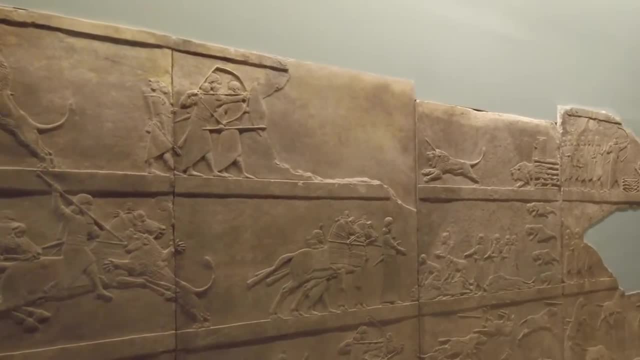 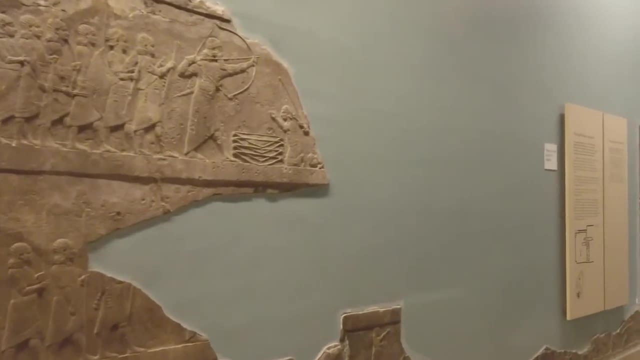 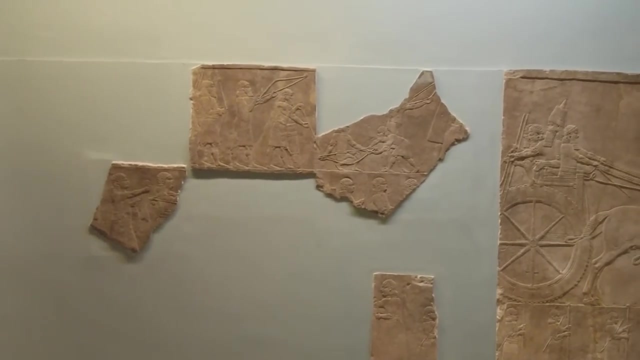 He destroyed the diocese of the gods that were erected at Namnundakigara. He recruited all the hostile lands and transgressed the boundary channel of Ningirsu. The text continues by describing how Uruma escaped with his life back to Uma. 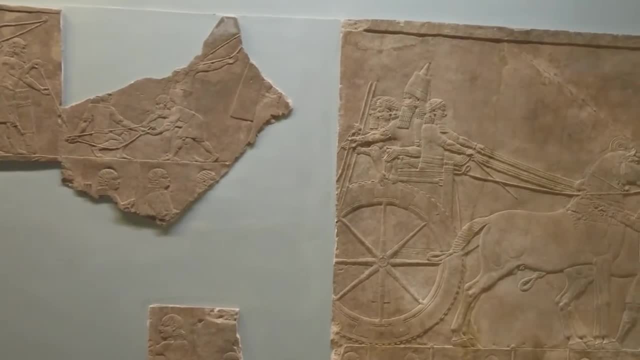 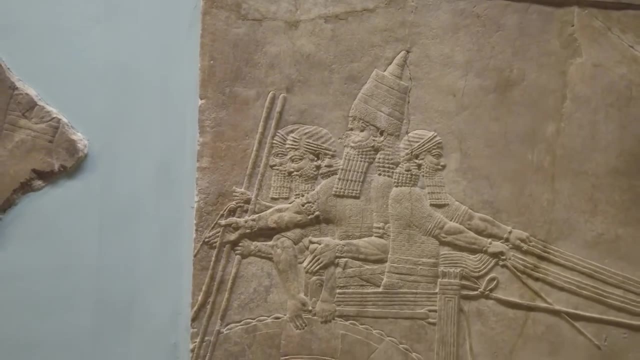 Uruma escaped, but he, Iyanatum, forced him back to Uma. He abandoned his asses- they were sixty teams- at the bank of the Lumunagirnunda canal and left the bones of their men scattered in the plain. 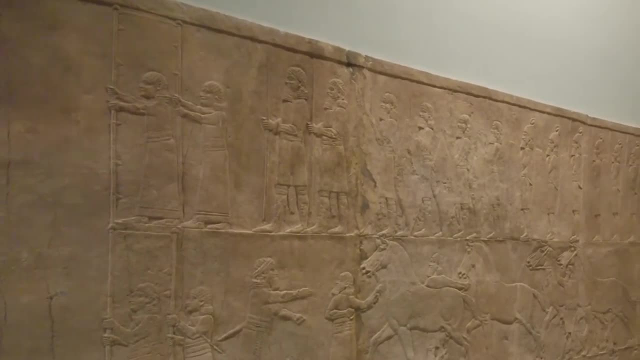 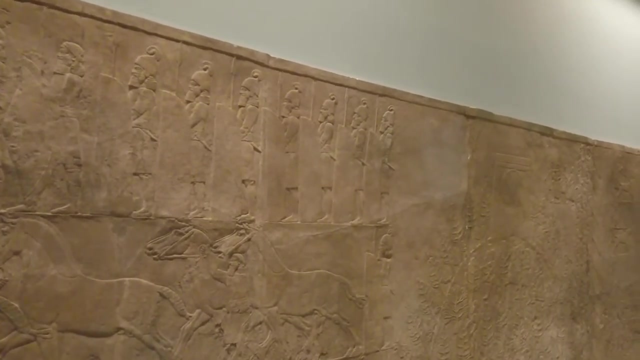 He, in Metena, made burial grounds in five places for them. By the time Uruma was in power, the act of going to war with Lagash had essentially become a rite of passage for the ensi of Uma. It was almost as if the ensi had to legitimize his rule. 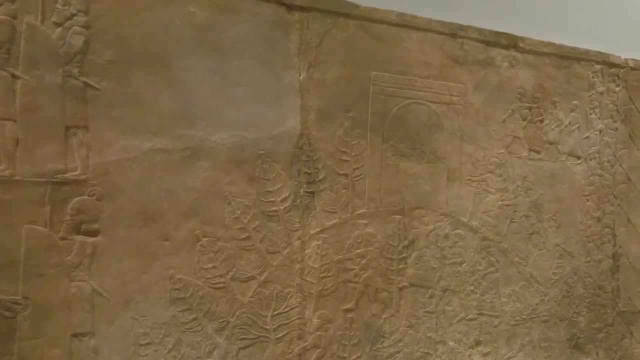 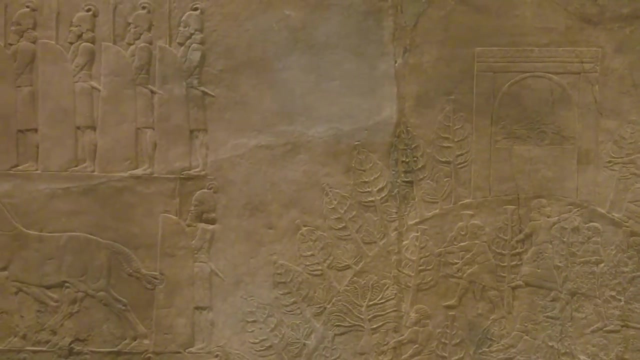 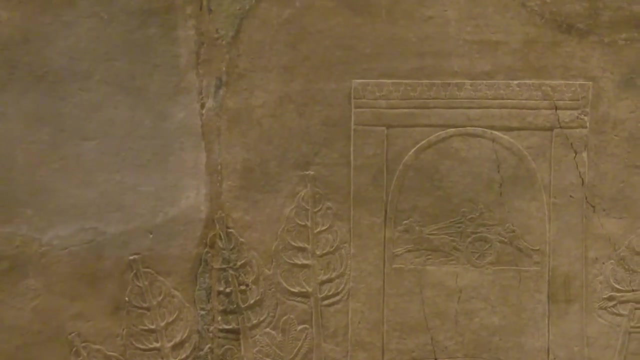 by warring against Lagash, And in the early years of the conflict, it was Lagash that was usually victorious. Nonetheless, other documents from Uma indicate that Uruma's reign was relatively long and stable. As mentioned above, it is difficult to state precisely the length of any of the early Uma rulers' reigns. 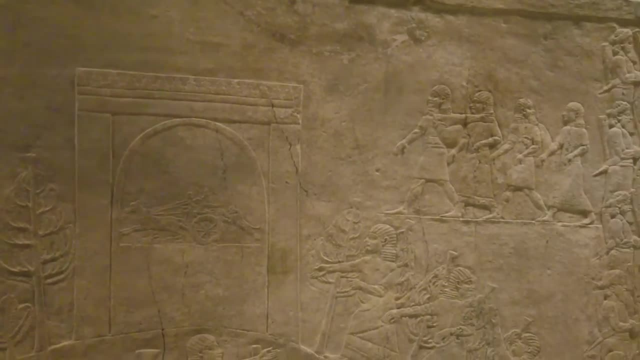 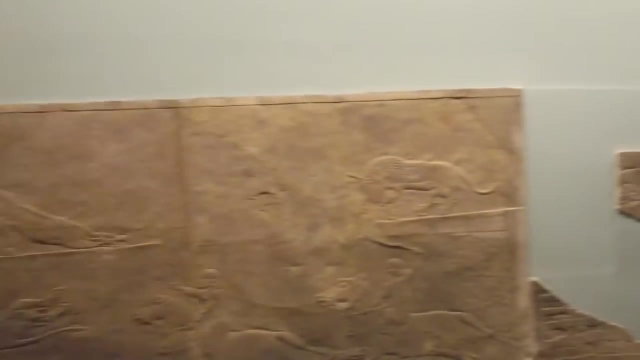 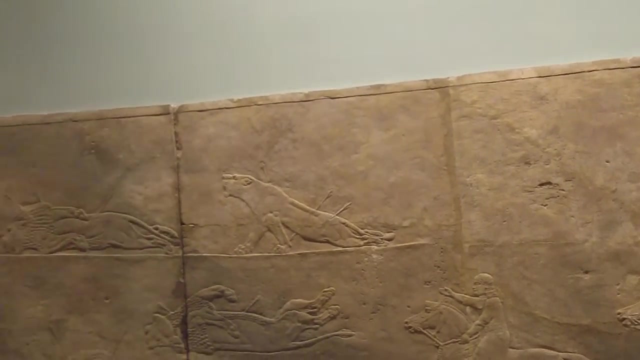 but, based on known administrative documents, Uruma ruled at least twelve years. Interestingly, Uruma is referred to as ensi in an Uma business document, indicating that the title was in fact still used instead of Lugal by the rulers of Uma. 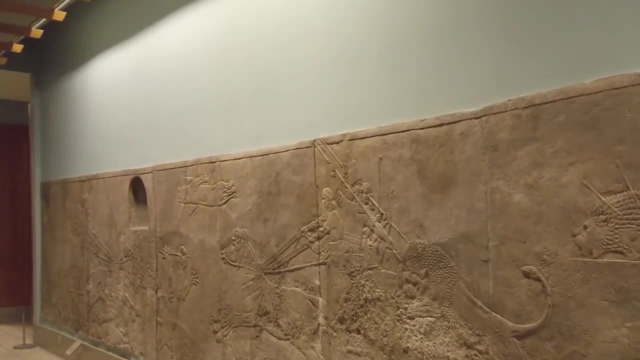 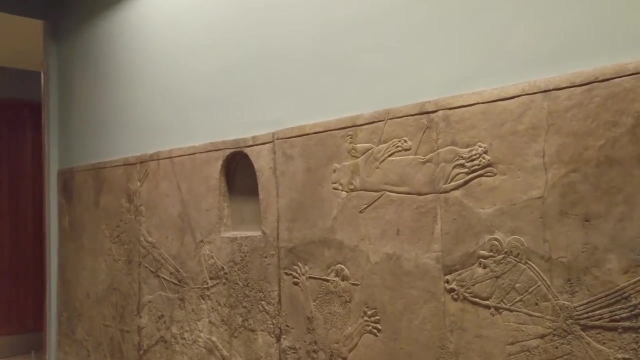 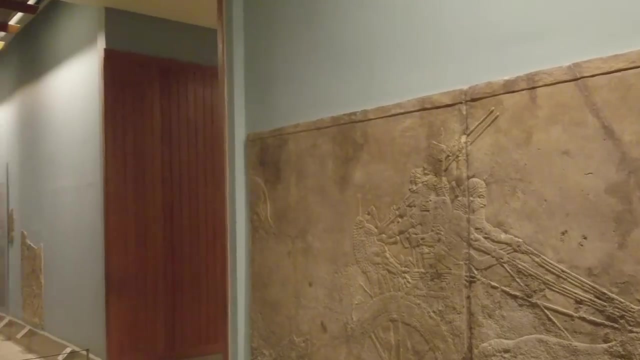 The ongoing conflict between Uma and Lagash appears to have calmed down later in Uruma's reign, but it could just be that texts documenting it are yet to surface After Uruma's reign of twelve to fifteen years. Il, the grandson of Inikale and cousin of Uruma, 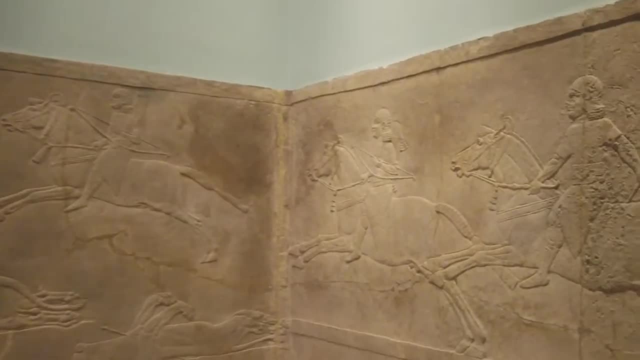 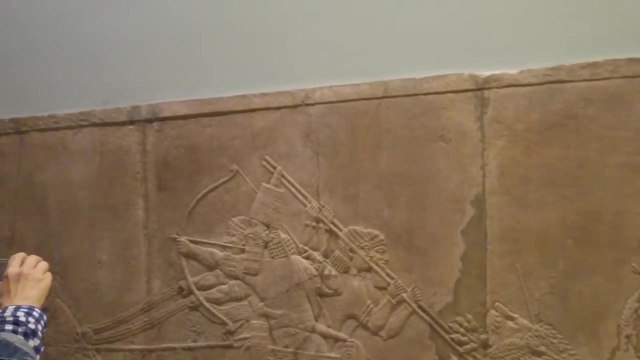 became the ensi of Uma. Il more than likely took a slightly different path to power than his predecessors. The first ensis of Uma were apparently groomed for the position and the succession appears somewhat clear. but if Il was the cousin of his predecessor, 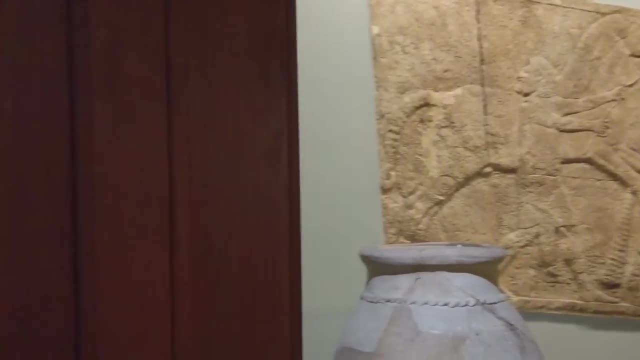 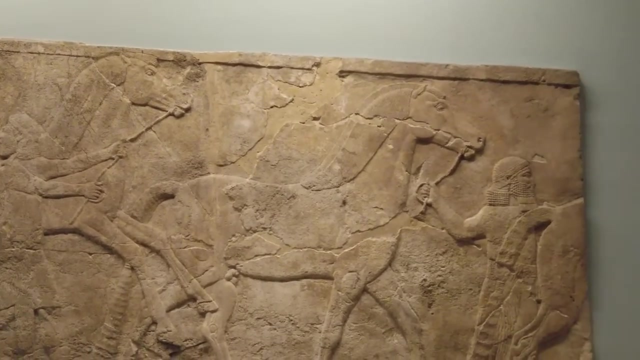 it remains questionable if he was the original heir. Royal and religious inscriptions from Uma suggest Il was a temple administrator, so it is possible that he originally intended to follow a religious path in his life, although it must be remembered that in the ancient Near East, 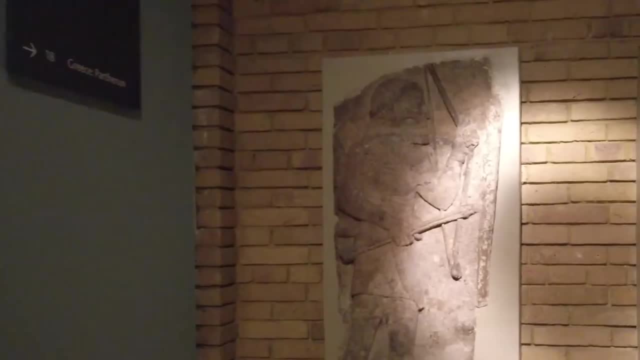 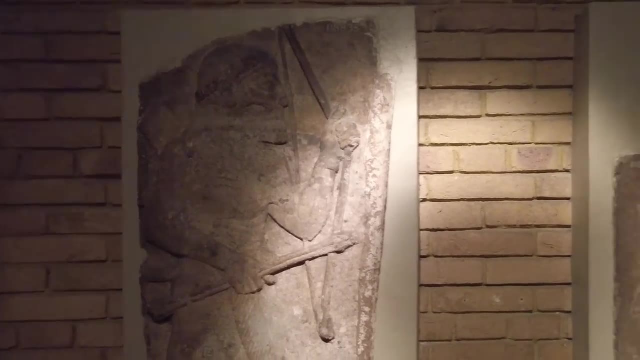 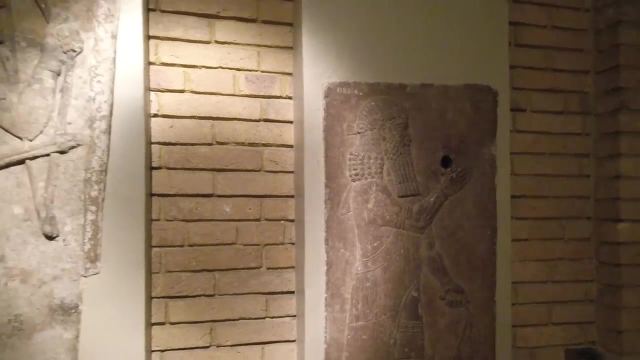 most politics and religion were intertwined. Il ruled Uma for at least fifteen years and he was referred to as Lugal in one of his own texts, but as ensi in other texts. Il continued the tradition of war with Lagash by breaking the ceasefire. 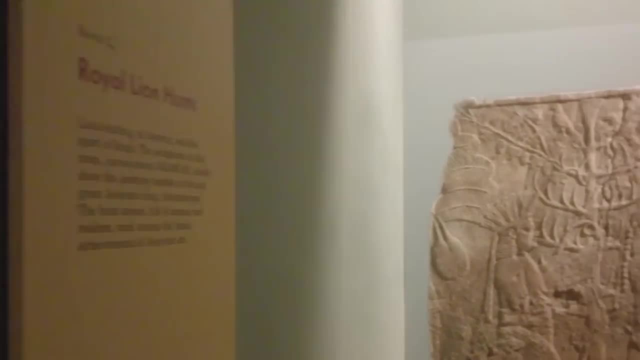 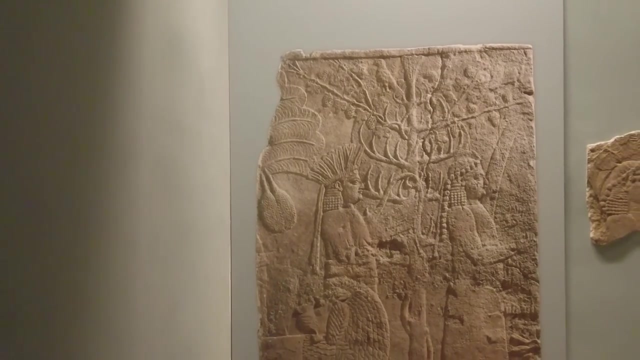 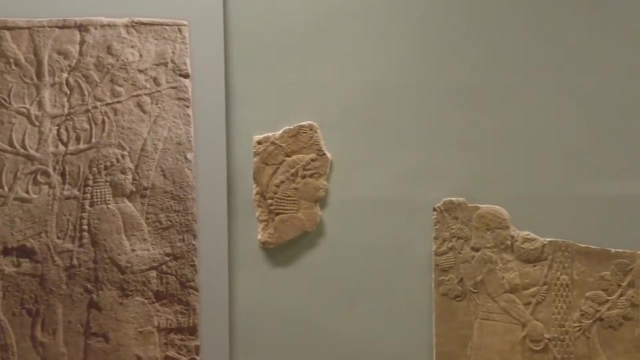 and once more invading the no-man's land, and he was succeeded by his son, Gish-Shakhidu, about whom little can be gleaned from royal or administrative texts. Few texts are attributed to Gish-Shakhidu, primarily due to his short reign of only about four years. 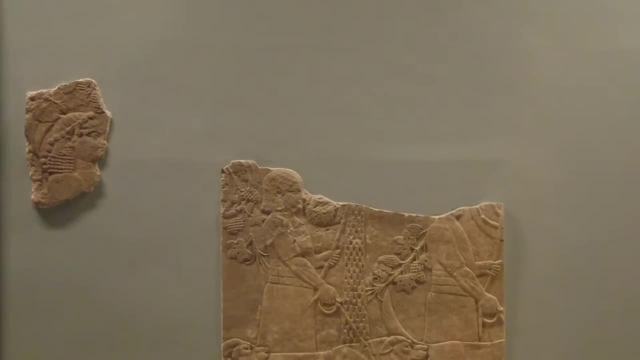 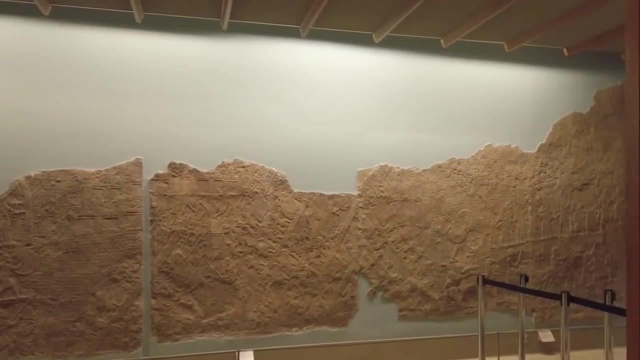 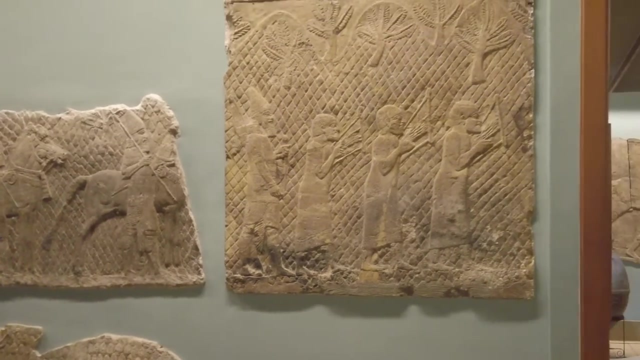 In a votive inscription dedicated to his wife, Gish-Shakhidu referred to himself as Lugal, which perhaps indicates that from Il's reign, the rulers of Uma considered themselves kings and were accepted as such by their subjects. After all, Uma was ruled by an authentic royal dynasty. 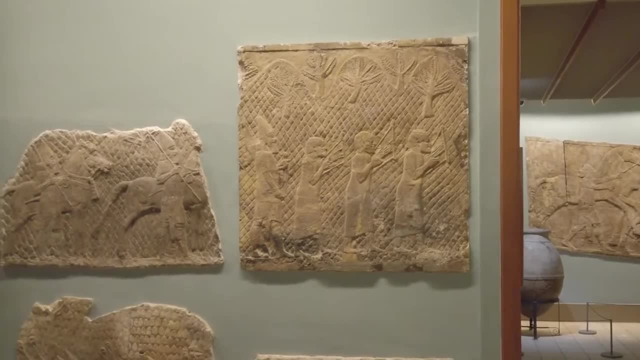 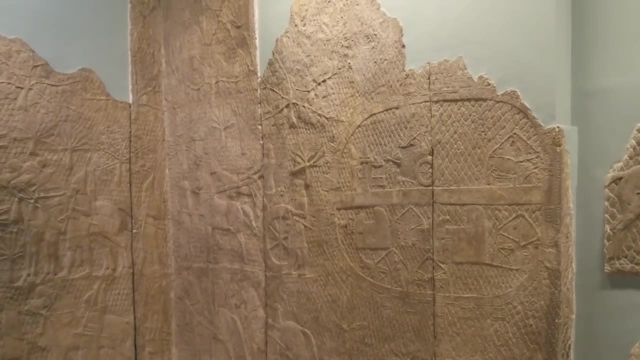 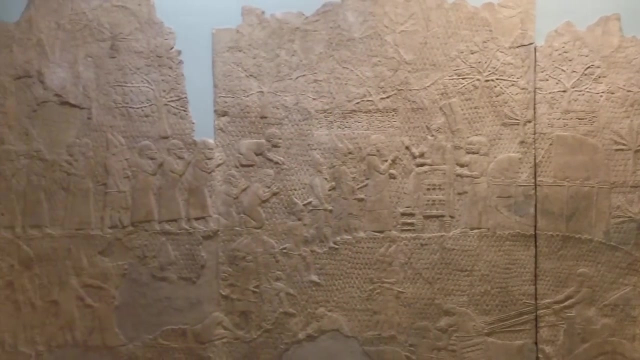 and the people would have known this and apparently accepted the political situation. as there is no evidence of internal upheaval in the early dynastic period After Gish-Shakhidu, the final four rulers of Uma are poorly documented. Gish-Shakhidu was probably followed. 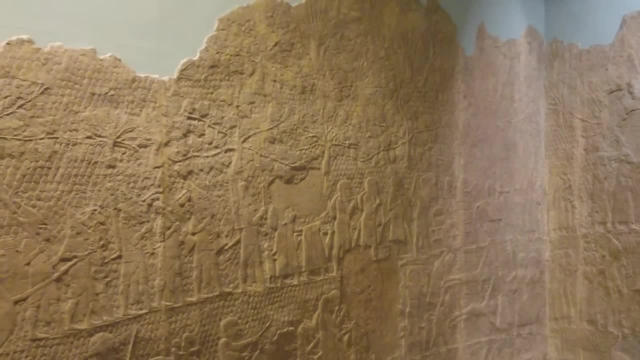 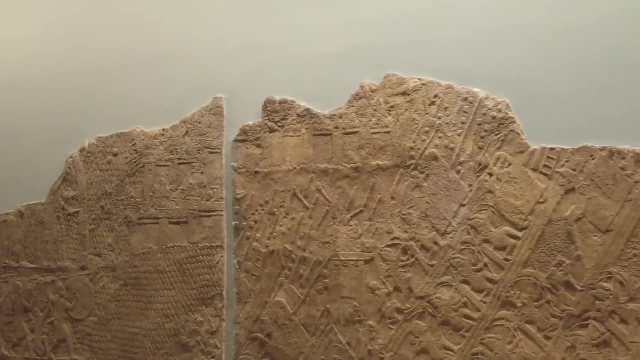 by a little-known ruler named Edin. Edin is known as the ensi in the text, although it is not known what his relation was to his predecessors or successors. In fact, precisely when he reigned and the length of his reign remain unknown. 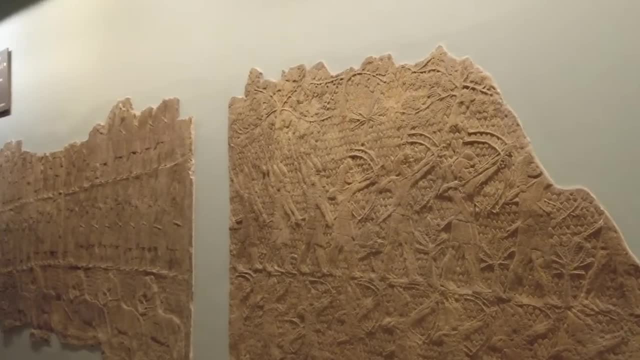 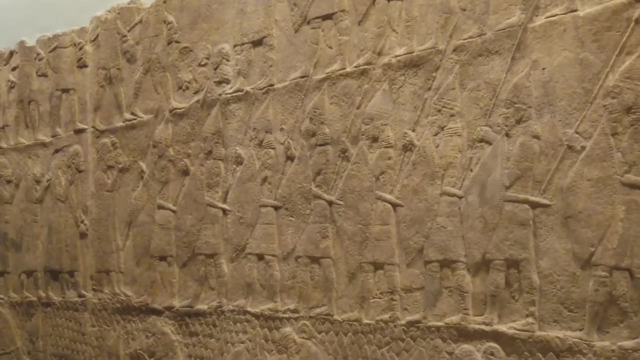 Edin may have ruled earlier or later, but modern scholars currently place his reign after Gish-Shakhidu's Mayan-Edu more than likely succeeded Edin, but again the precise chronology is not clear. There is little evidence that indicates continued hostility. 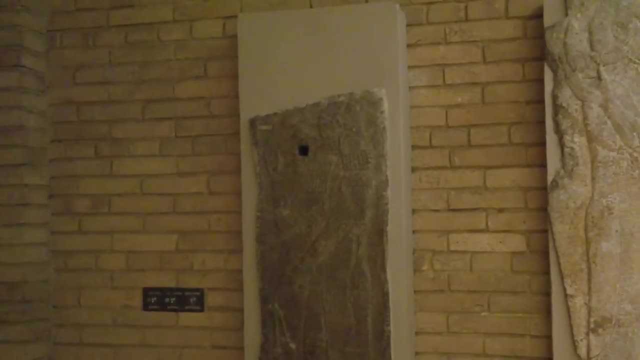 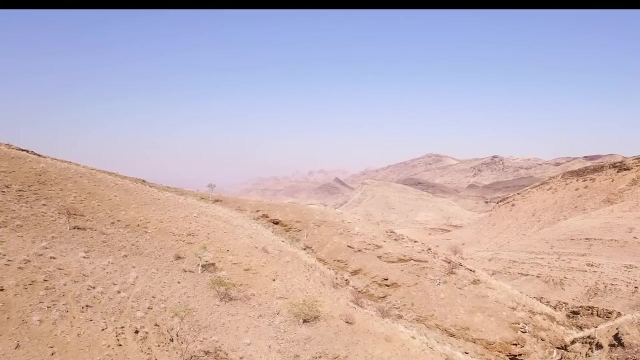 between Uma and Lagash, but that may just be due to a lack of records, more than based on reality. It is worth pointing out that Mayan-Edu is only known as ensi from the extant texts, which has led to some speculation that he ruled earlier. 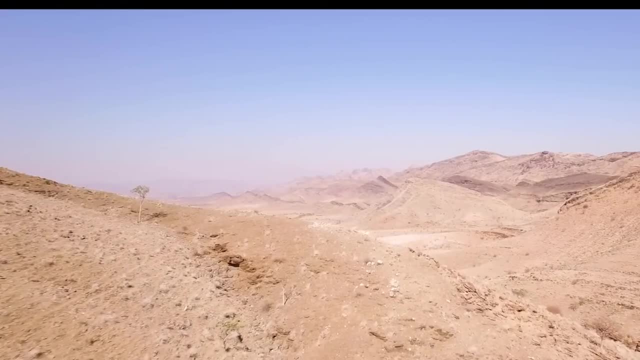 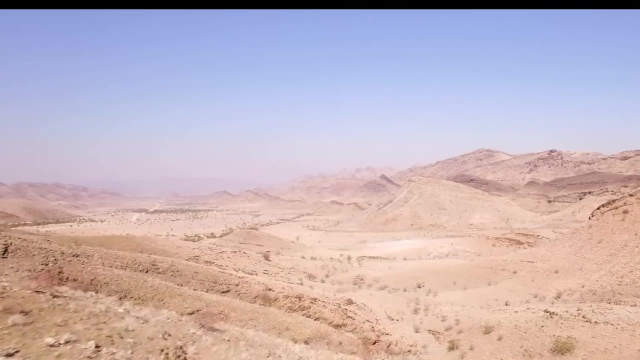 With that said, Mayan-Edu ruled for about 30 years, which, based on the evidence of the stele of the vultures and the cone of En-Natenah, means that he probably ruled after those events. The length of Mayan-Edu's rule indicates that Uma. 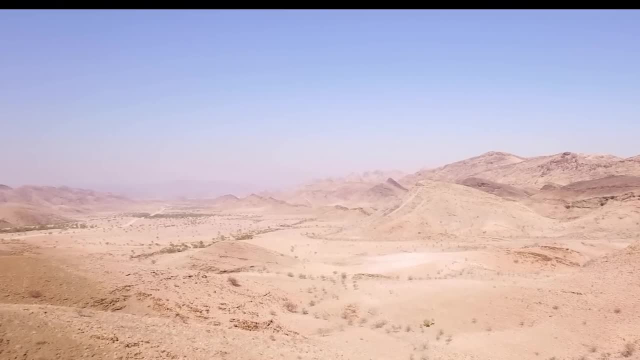 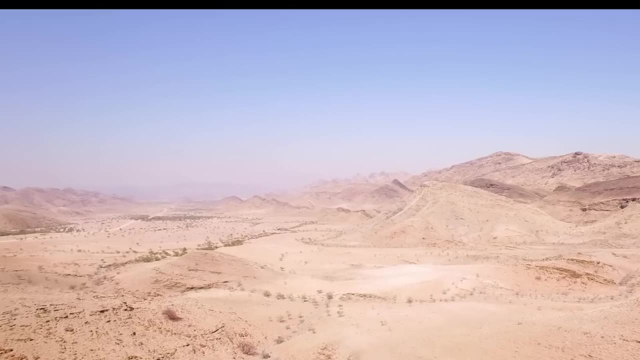 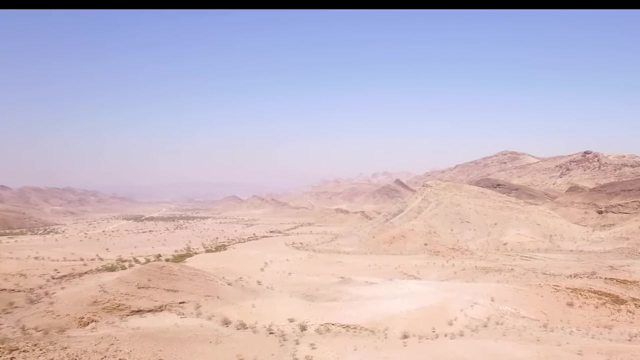 was experiencing a period of internal prosperity and peace. There is no evidence of war with Lagash or any other cities, and agricultural production which drove the ancient Mesopotamian economy was apparently stable. Mayan-Edu may have been succeeded by Ushurdu. 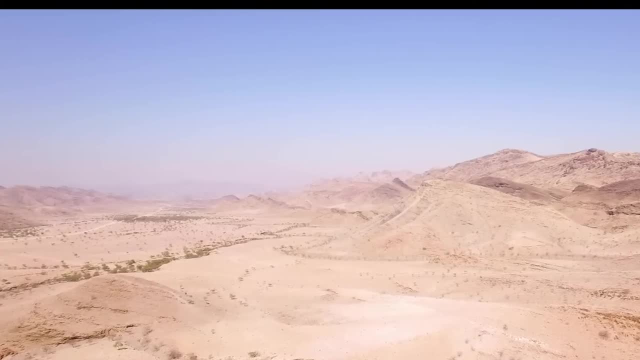 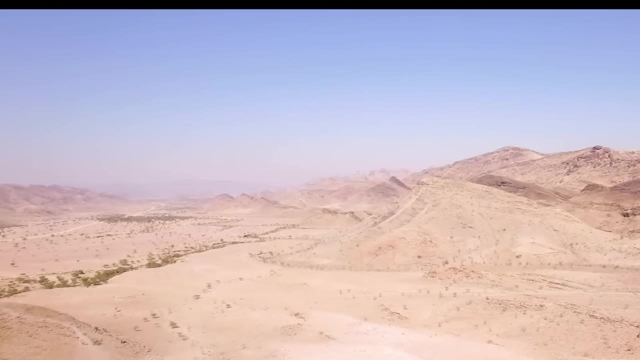 but, once again, due to a lack of royal inscriptions and genealogical information, it is difficult to say for sure. Ushurdu is known as an ensi of Uma, who ruled for at least nine years, but there is little additional information about his reign. 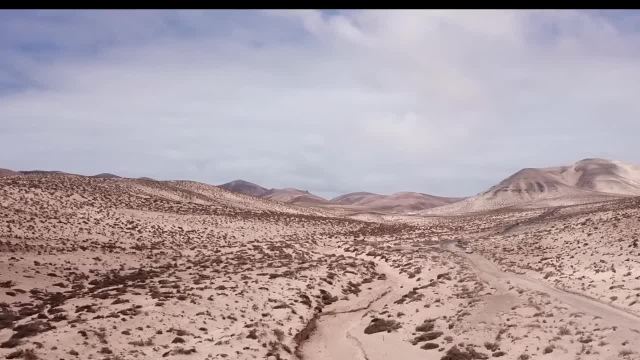 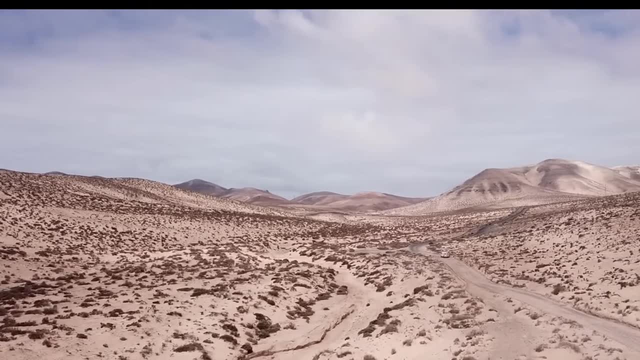 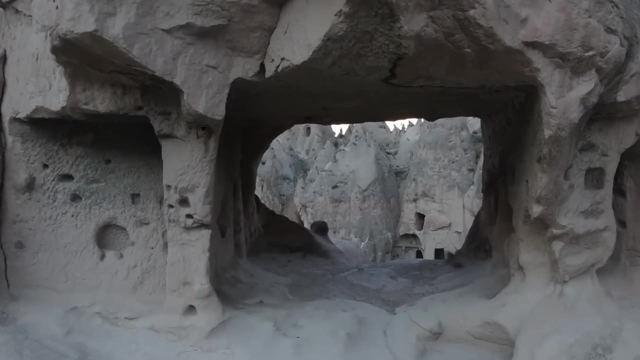 The final information, and perhaps most important: ensi was Ukush. Un-Kush was not important for winning any wars or carrying out significant building programs or reforms in Uma, but for being the father of Lugal-Zaghesi, who subsequently went on to rule all of Sumer. 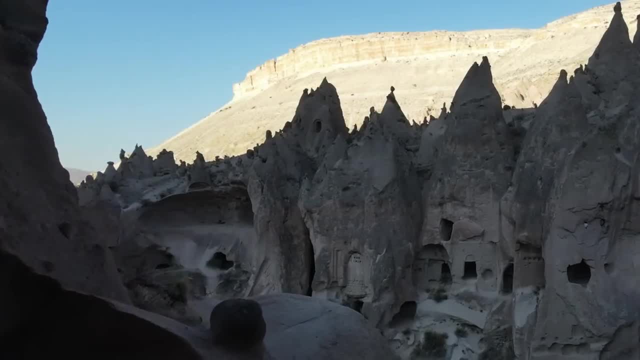 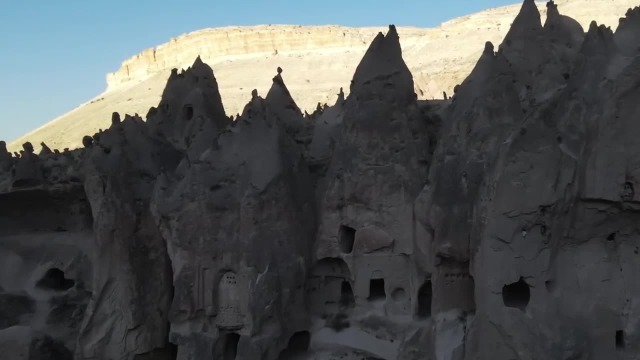 A vase inscription from the reign of Lugal-Zaghesi relates the genealogical information: Lugal-Zaghesi, king of Uruk, king of the land Isib, priest of An Uma, priest of Nisaba. 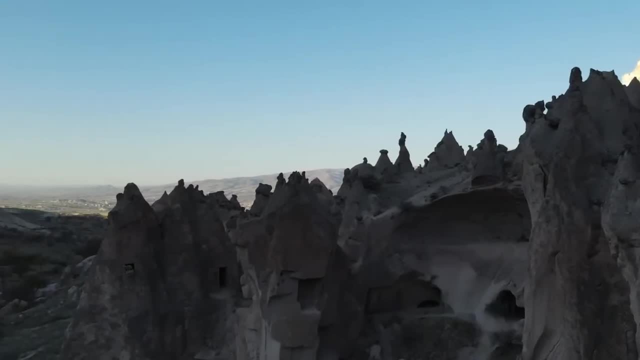 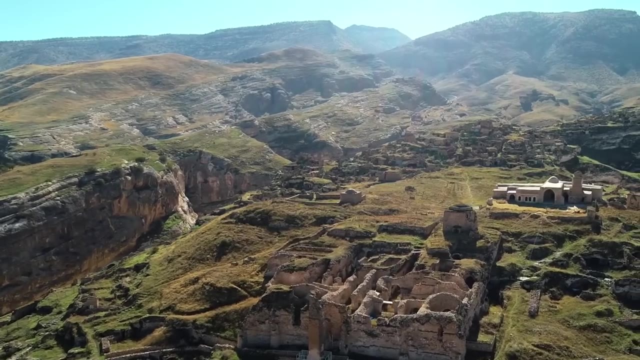 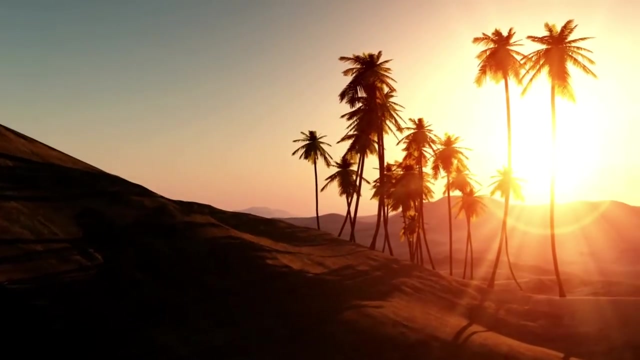 son of Ukush. governor of Uma, Uma, priest of Nisaba. Based on all of the known inscriptions, the above listed ensis ruled Uma for 140 to 160 years. Few details are known about their styles of rule, other than that Shara was their primary god. and that they hated the rival Lagash. The conflict between early dynastic Uma and Lagash is fairly well documented for the period, albeit not when compared to later periods in ancient Mesopotamia. It is important to consider, though, that in the mid-third millennium BCE literacy was not yet widespread and the genres of writing were somewhat limited. Royal inscriptions and administrative documents written on clay tablets and the cuneiform script were the primary literary genres from this period, But Mesopotamian historiography also began at this time. 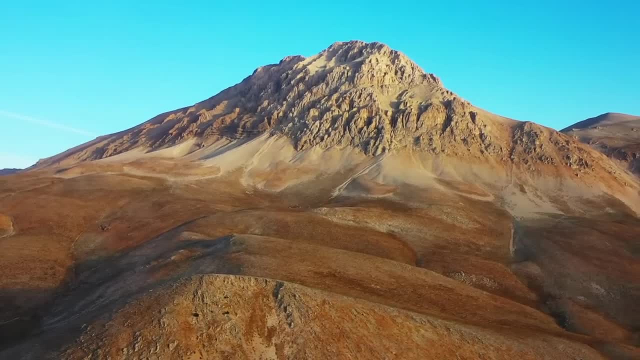 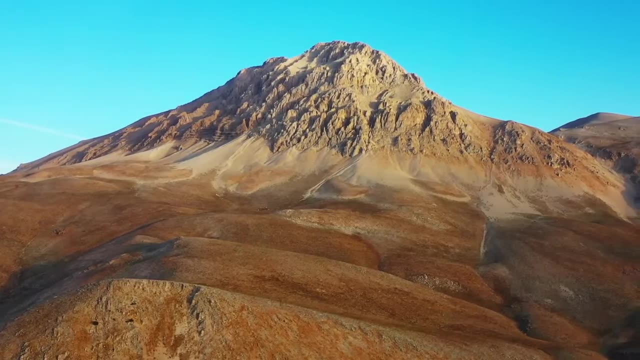 The term historiography can refer to a couple of different concepts, either the study of historical studies or the writing of historical texts, But in this case it is related to the Sumerian view of history and how they recorded it In this early period. 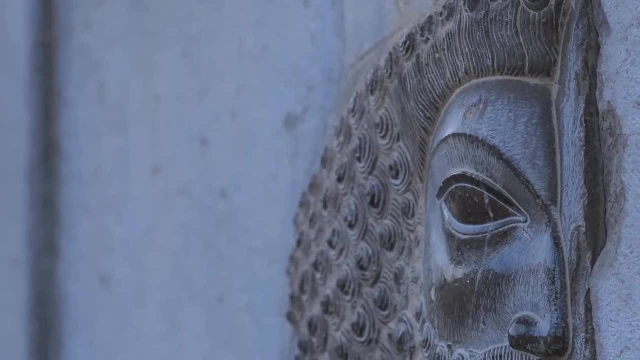 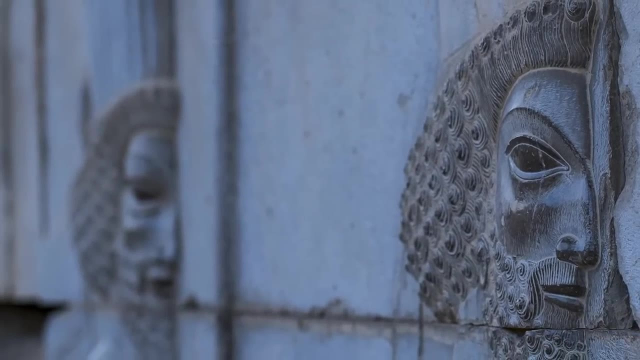 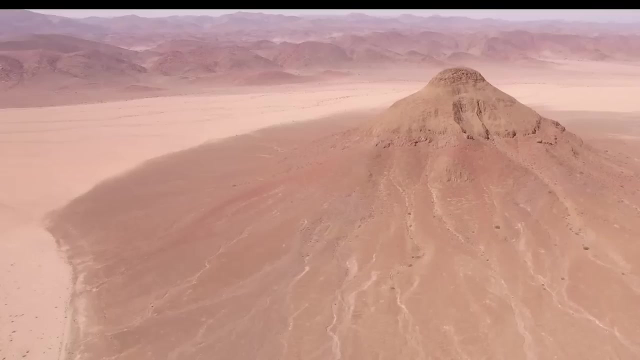 with historiographical writing in its infancy, the line between religion and historical fact was often blurred. The gods were depicted as playing central roles in historical events, and human agents could be granted mystical abilities such as foresight by the gods. Still, these texts are a good starting point. 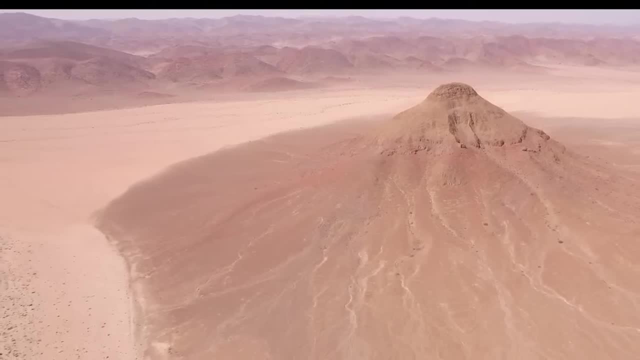 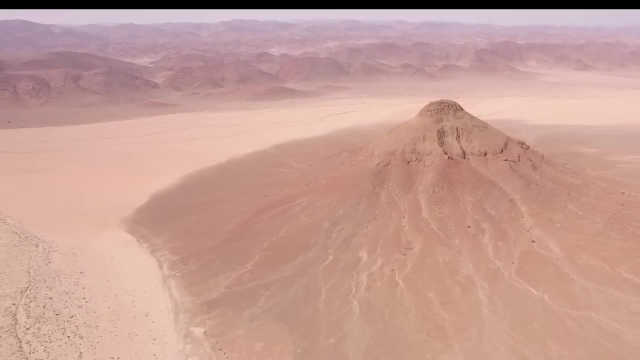 to unravel the details of the Ummah-Lagash rivalry. The ruined Sumerian city of Lagash is located 15 miles east of present-day Shattra in the province of Nasariya in southern Iraq, also known as Tell al-Ahiba. 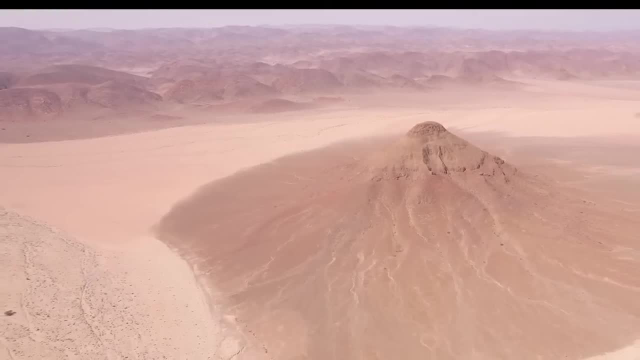 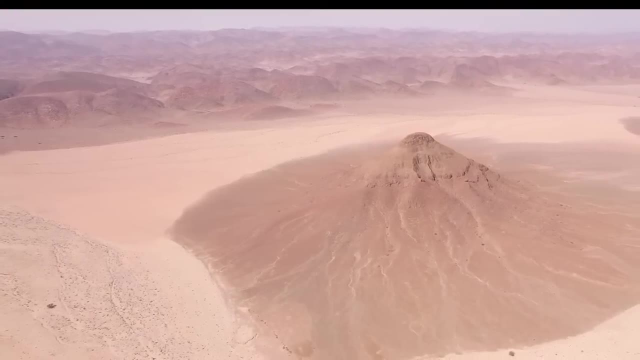 This was one of the largest urban sites in the ancient lands of southern Mesopotamia, At its height in the early dynastic period. the city is believed to have occupied a total area of approximately 600 hectares, Based on the presence of so many temples. 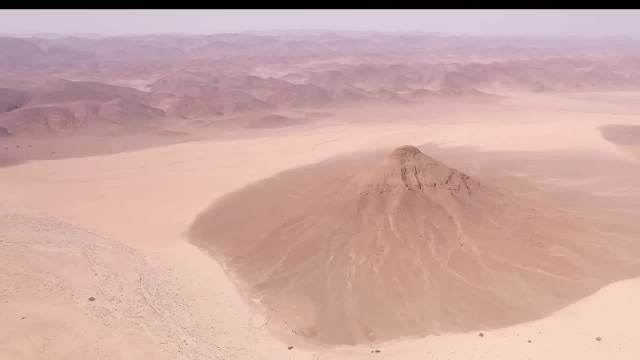 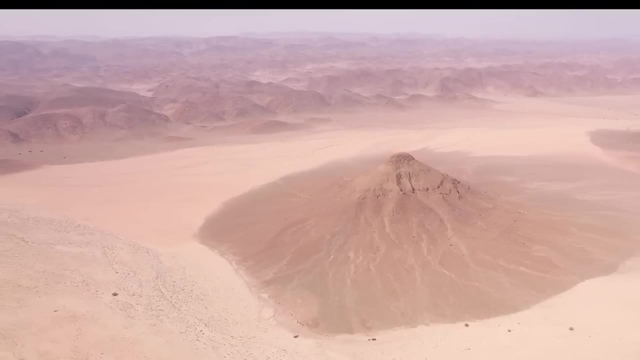 Lagash clearly served as the religious capital of the state. It is from the huge corpus of documents that have been recovered from the city ruins that historians learned so much about the ancient gods and goddesses that were worshipped by the ancient Sumerians. The temple architecture in the city is amongst the finest found in any of the ancient settlements in Mesopotamia. Lagash experienced a golden age of prosperity and growth in the early 21st century BCE during the reign of Gudea, a contemporary of Ur-Nammu. the founder of the third dynasty of Ur. It is no wonder that Gudea was worshipped as a god, Although Gudea was a fine ruler. after his reign ended, the city quickly succumbed to invasion and, over time, faded out of popular knowledge. 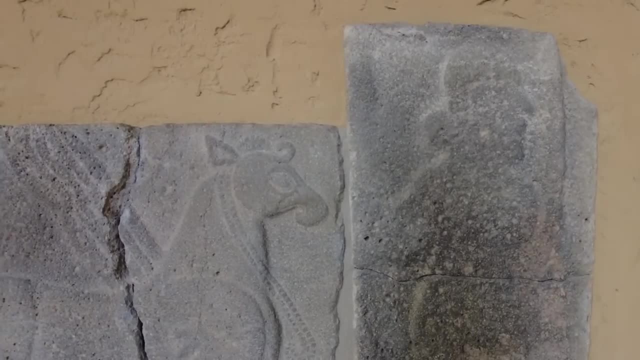 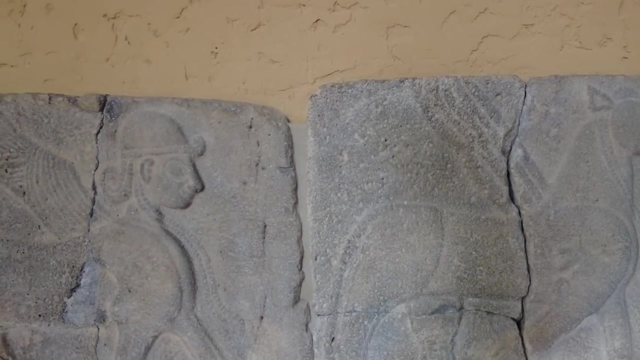 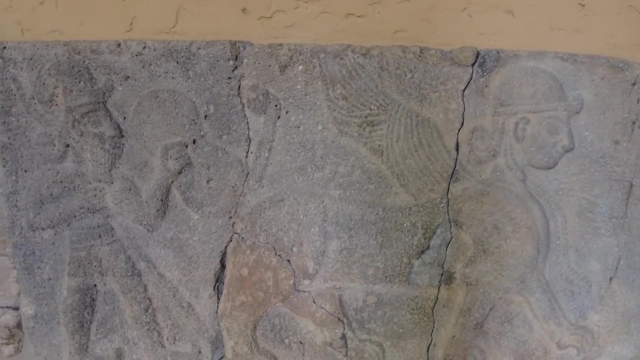 It is only because of excavations carried out there from the 1950s onward that the questions regarding this site's identity have been answered. Lagash can refer to the city itself or the state over which it dominated. Archaeologists have identified 17 distinct urban centers. 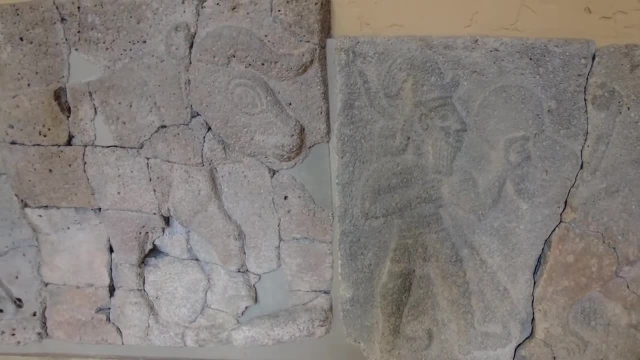 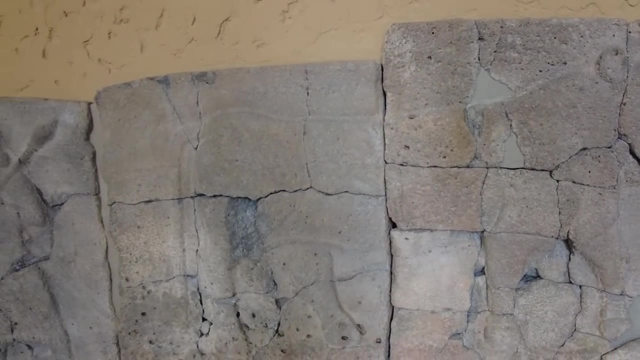 which were part of the state of Lagash, and epigraphic evidence has provided the names of approximately 40 smaller villages. Some of the other main cities in the state of Lagash were Girsu, approximately 15 miles northwest of Lagash. 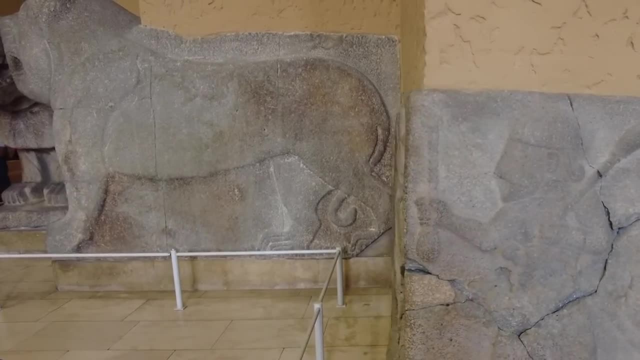 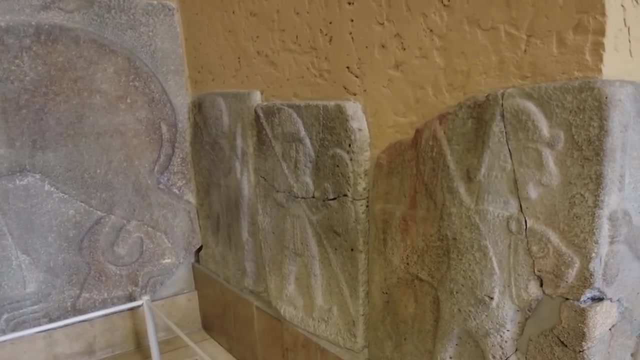 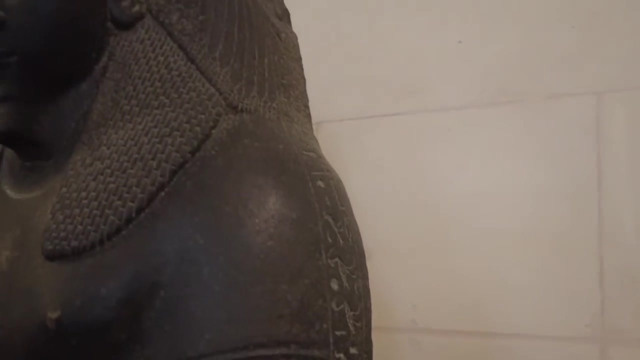 and Nina, approximately 6.5 miles away. Girsu periodically served as the political capital of the state of Lagash, for example during the reign of Gudea. Indeed, it was from the palace at Girsu that so many recent findings have been made. 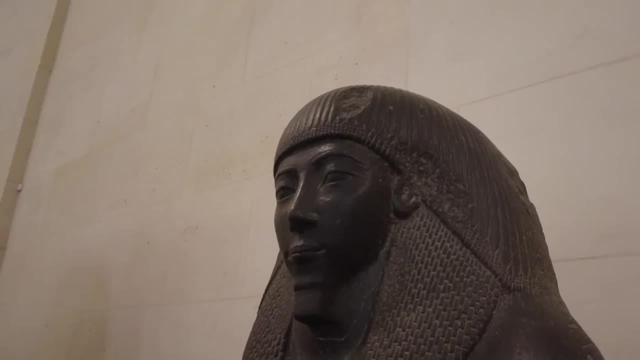 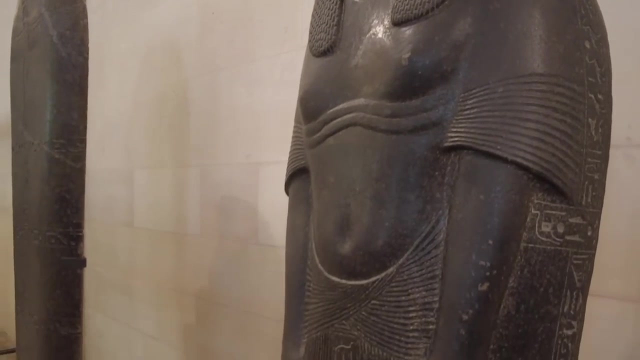 relating to the life of Gudea, including many of the famous statues depicting him. The city of Lagash was founded between the Euphrates and the Tigris, a short distance northwest from where the two rivers merged to form the Shat al-Arab waterway. 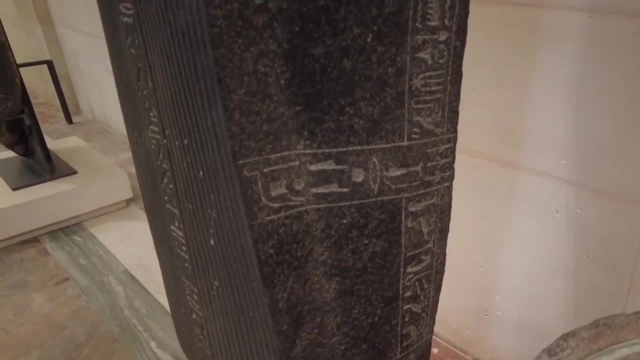 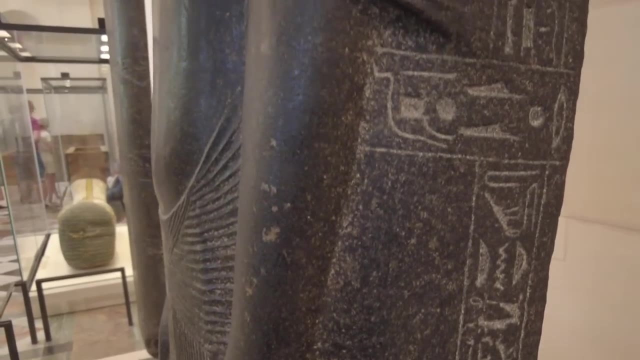 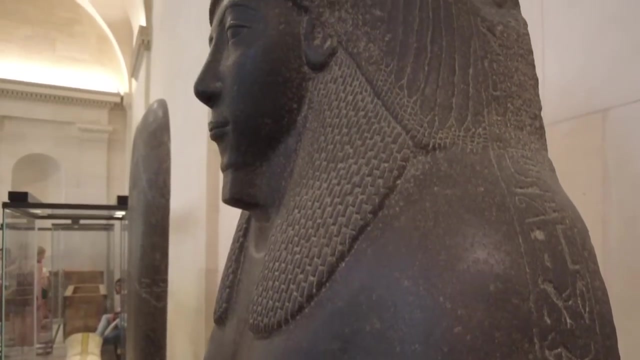 Two distinct mounds can be seen at the location today. One of them is known as Tell al-Hiba, the other goes by Zirgul or Shirpula. Lagash was significantly larger than other contemporary sites in Sumer, Like modern large cities such as London or New York. 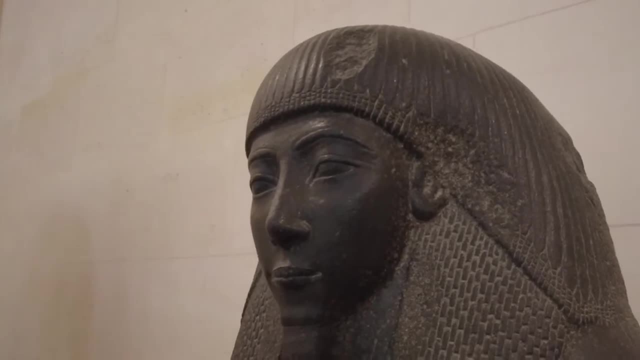 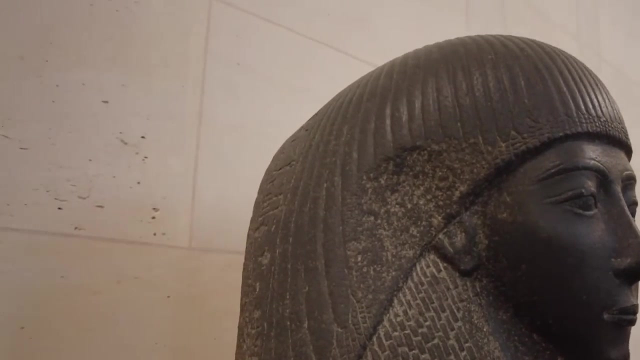 Lagash consisted of several distinct urban areas. Based on inscriptions found in the area, the names of these districts were Uruazaga, Ninaka and Dishkalati. Uruazaga was the religious quarter in the western area of the city. 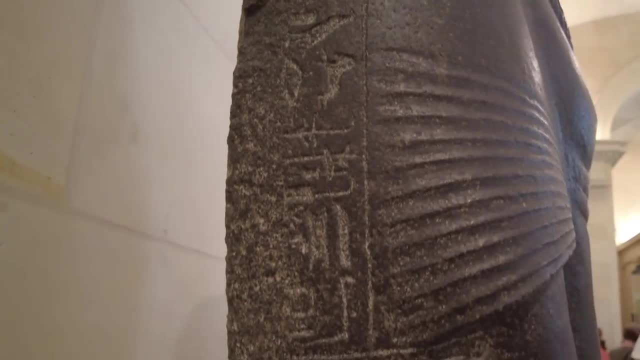 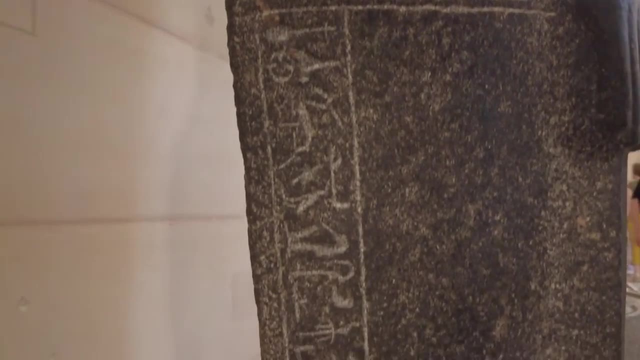 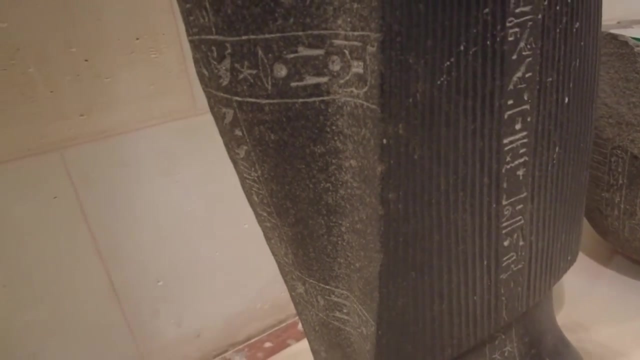 The temple precinct identified by archaeologists as Area A. Ancient sources also referred to this area as Uruku, the Holy City. It contained most of the major temples of Lagash. The location of Ninaki may have been somewhere around the four small mounds. 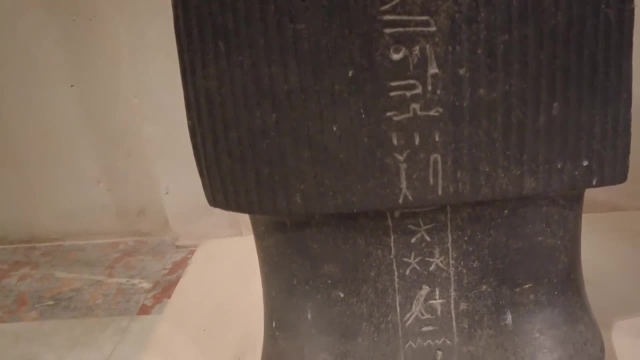 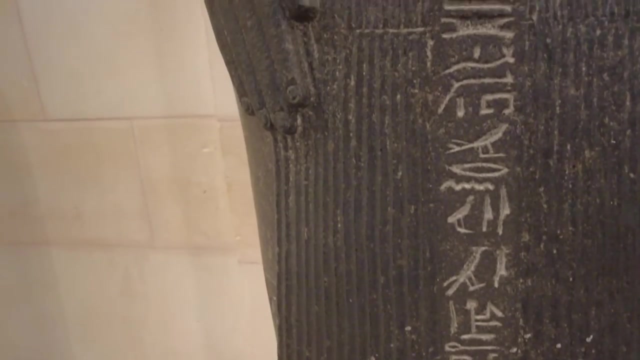 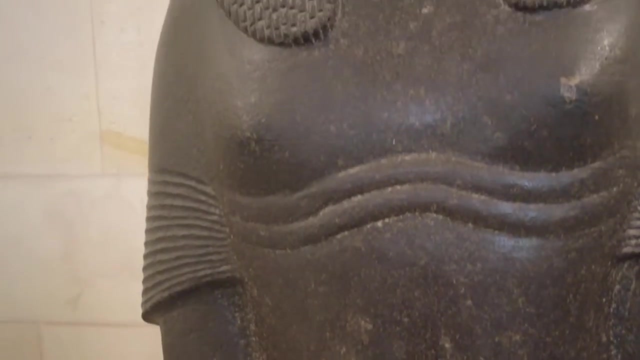 found roughly 1,500 feet to the west of Tell al-Hiba. An immense canal was dug through this area, running from the northwest to the southeast of the city. It was known as the Ninakituma Canal, the favorite river of the goddess Nina. 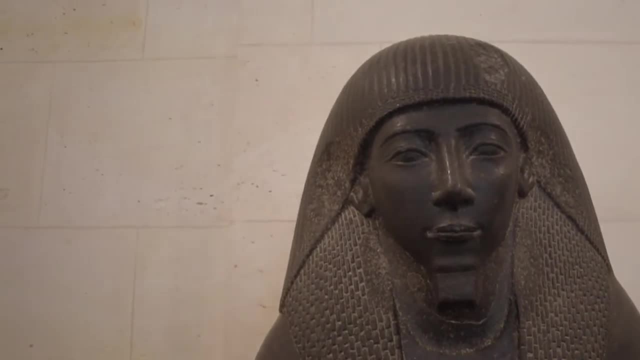 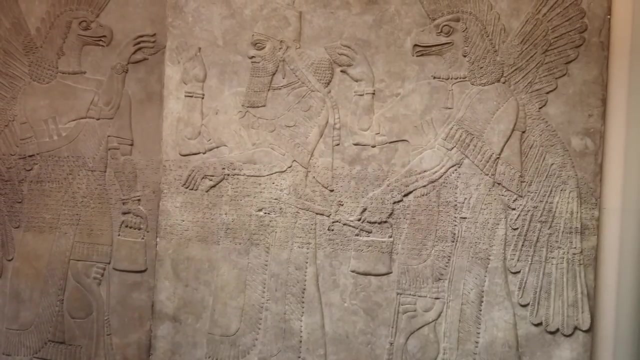 This provided fresh water from the tigress to the city's population. The other named district of the city was Dishkalaki, the dwelling place, and though its precise location is unknown, this may have been around the eastern side of the city. 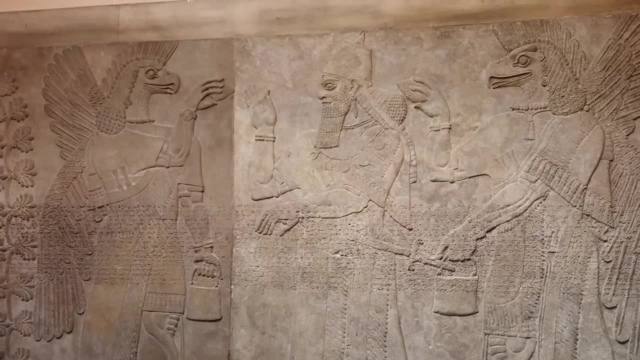 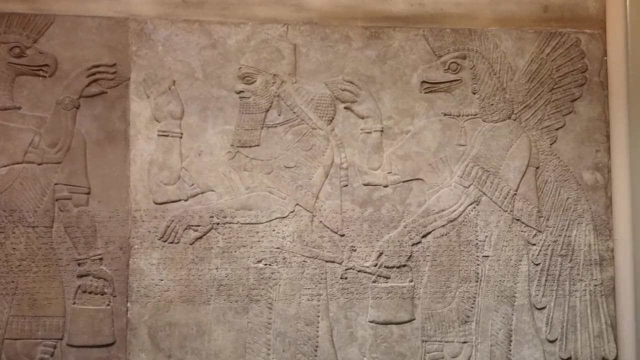 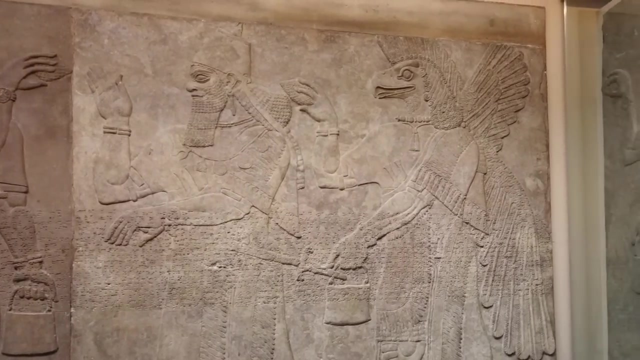 where archaeologists believe most of the city's population resided, separated from the temple buildings of the western side by the wide Ninakituma Canal. Much of what is known about Uma comes from Lagash, because inscriptions have been found there on a remarkable variety of objects. 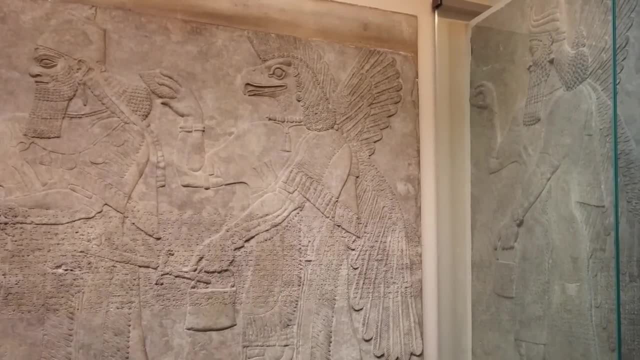 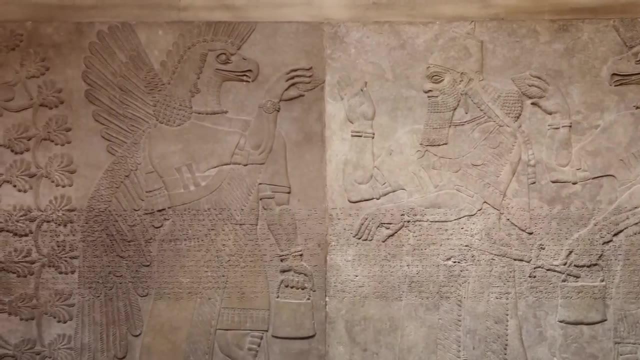 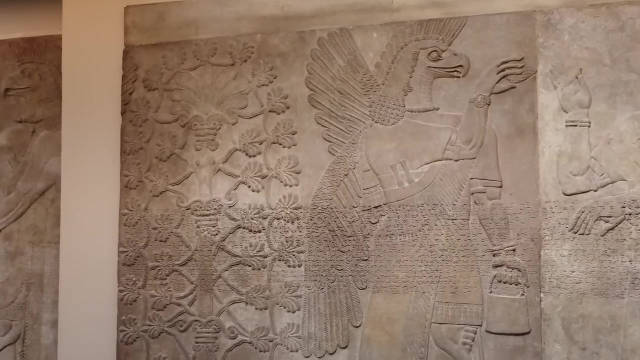 such as mud bricks, statues, vases, ceramic nails, foundation stones, carved door elements, lion heads and mace heads. A collection of inscribed cylinders found in Lagash has provided more than 200 texts relating to the reigns of eight different rulers. 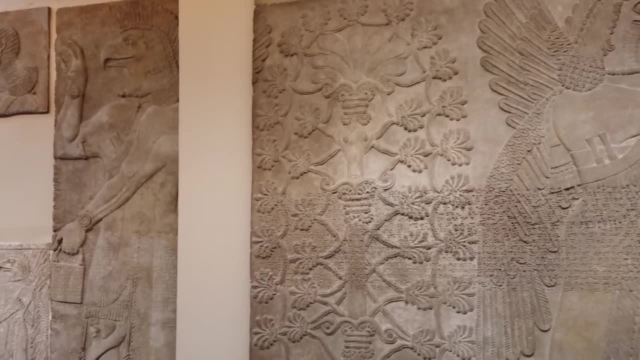 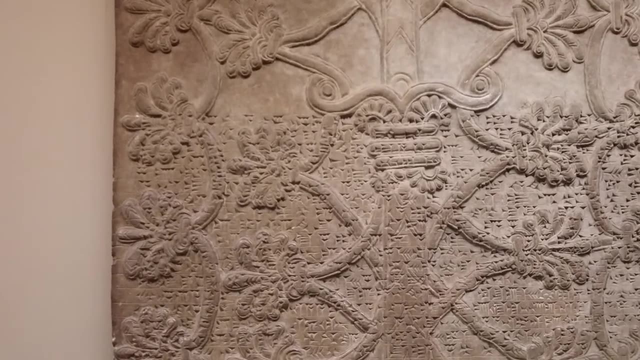 but mainly to the time of Budea, whose inscriptions are also considerably longer than the others. These inscriptions have served as significant sources of hitherto unknown details of life in ancient Mesopotamia. Many of the cuneiform texts were ration lists. 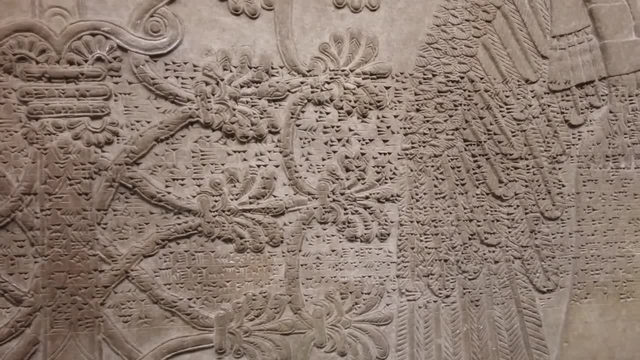 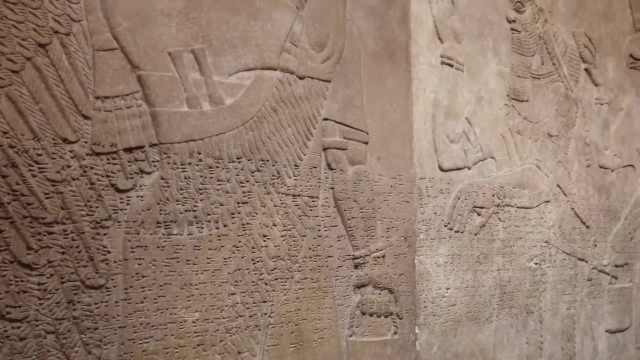 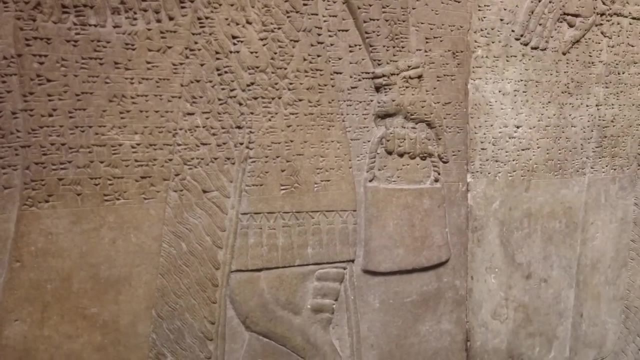 which recorded the distribution of different foodstuffs and other commodities as payment for work. Two texts of particular interest are the stele of the vultures and the cone of Enmetene Around the year 2430 BCE. Lagash ruler Einatum received the assistance. 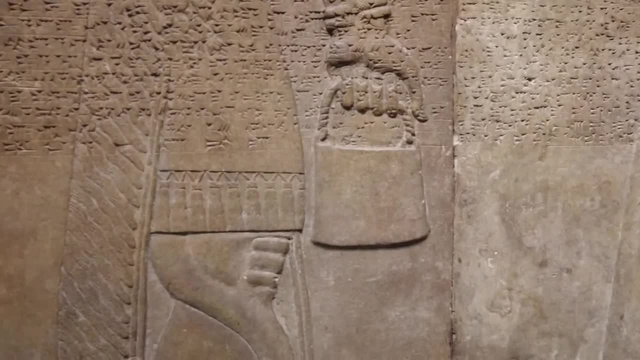 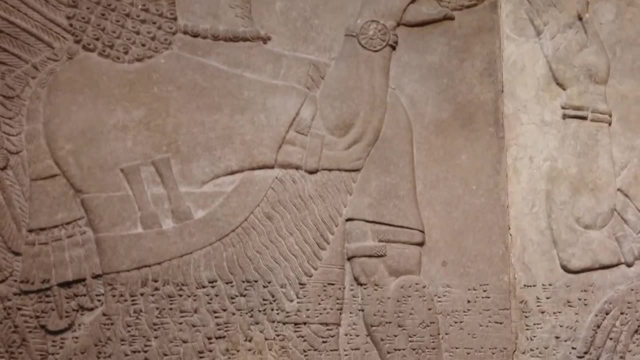 of Rugalura, king of Uruk, and once more went to battle against Uma, this time at a place near Disu known as Udige. Uluma was defeated and later slain in Uma, and it was in celebration of this victory against Uma. 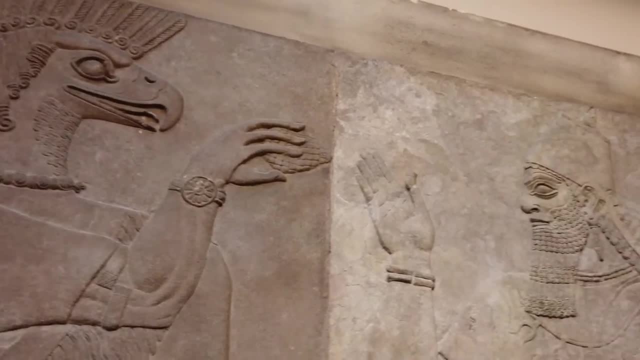 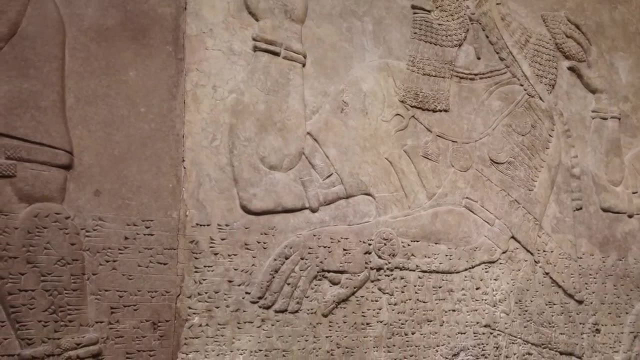 that the stele of the vultures was erected. This is a limestone stele discovered by archaeologists at Girsu in a fragmentary condition and given its name by the representation of vultures in one of the fragments. The largest fragment shows on its front side. 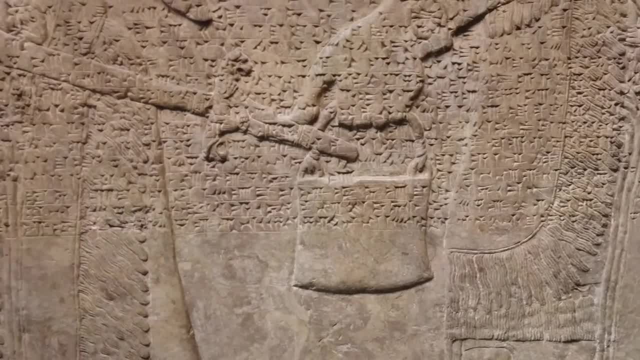 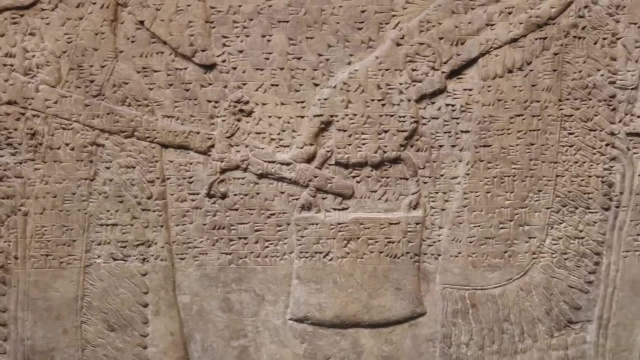 the god Ningirsu striking naked enemies that he has caught in a net. It also features the lion-headed Anzu. On the back of the largest fragment, Einatum is depicted leading his phalanx advancing in battle. Underneath this is an image. 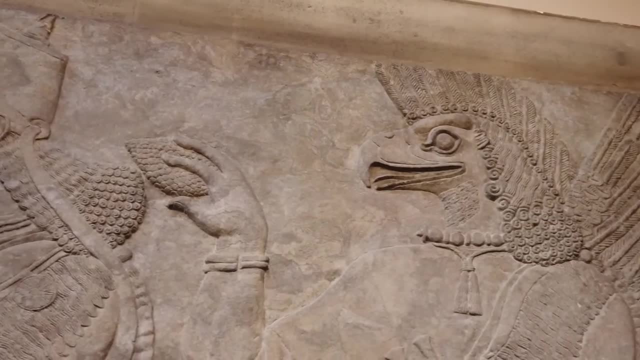 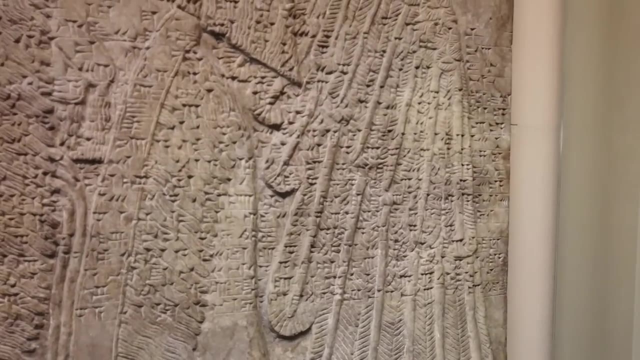 that shows the king on a chariot holding a spear in one hand. Another fragment of this face of the stele shows the enemies killed in battle. The stele of the vultures is one of the best preserved examples of a stela from the early dynastic period. 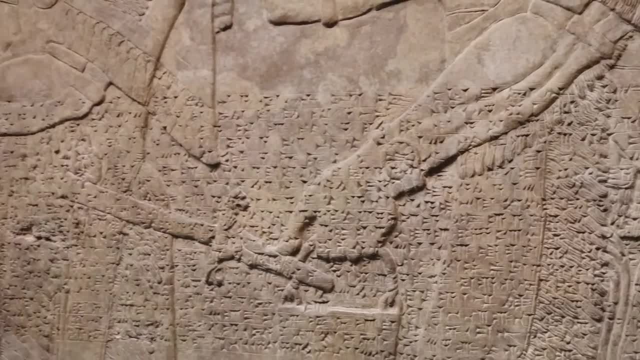 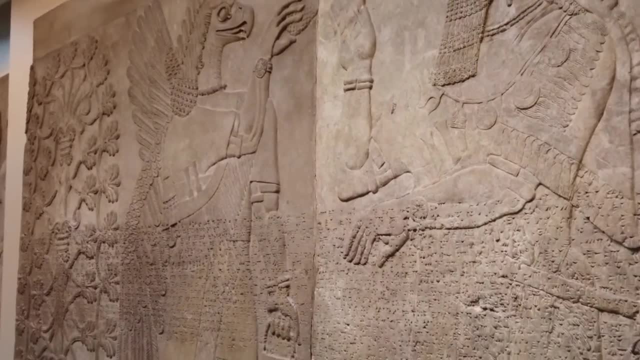 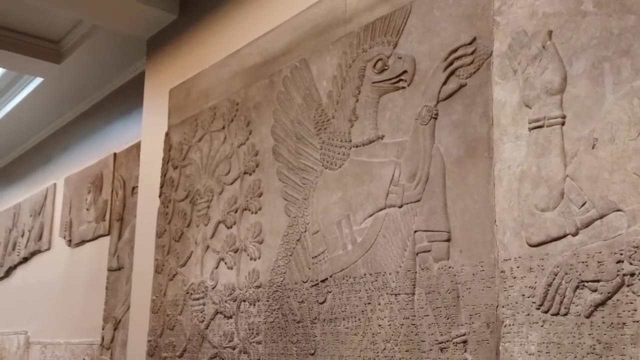 and also among the earliest historiographical texts known in ancient Mesopotamia. Indeed, since most who would have viewed the stele would not have been able to read the inscription, it is truly more of a visual than a written text. The few preserved lines of the text: 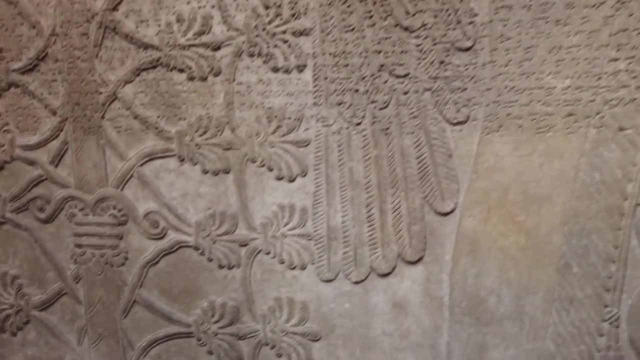 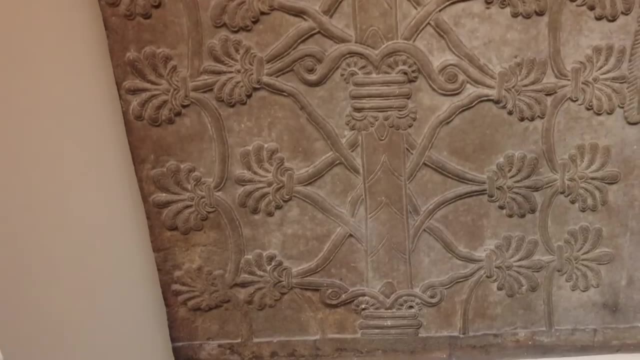 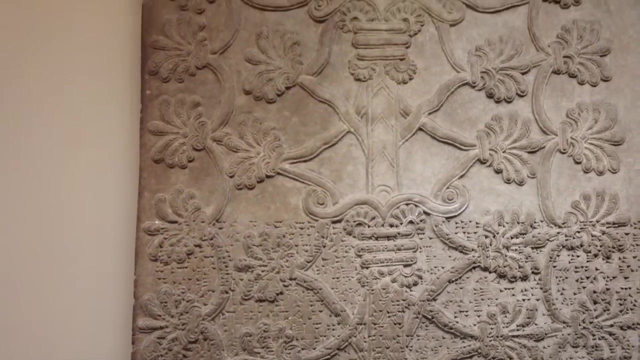 along with the images on the reversed side, tell of a war fought between Uma and Lagash over a no-man's land between the two city-states. It was a fertile, irrigated land that was apparently quite valuable to both cities, which coveted the land to feed their growing populations. 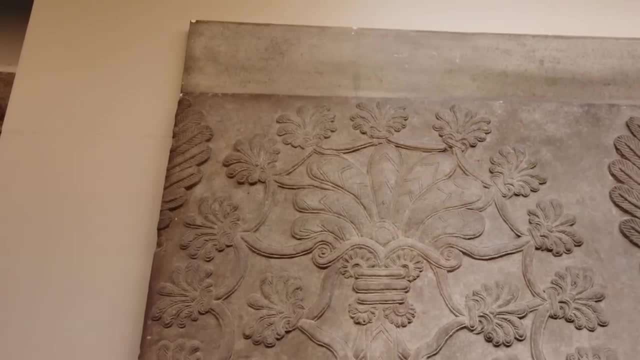 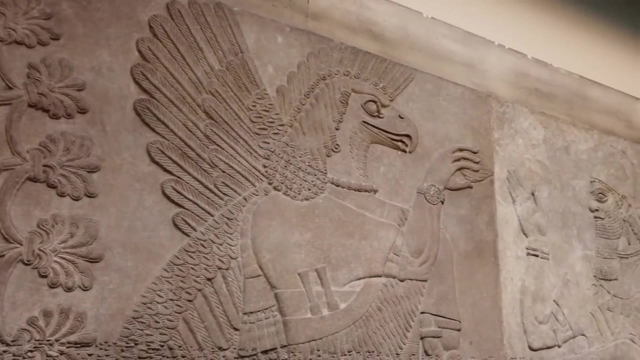 According to the text, Nintat in-see of Uma made the first move by moving into the neutral zone. Nintat, the governor of Uma, turned the matter into something that exceeds any word. He smashed that stele. 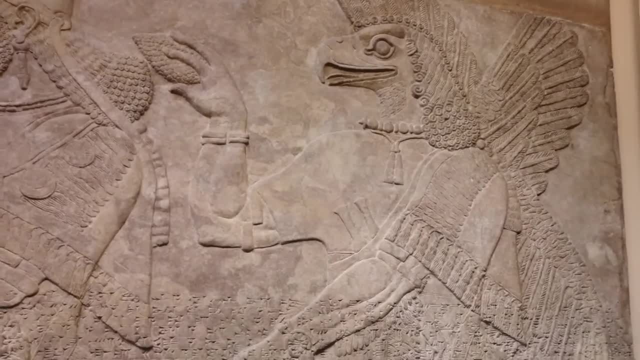 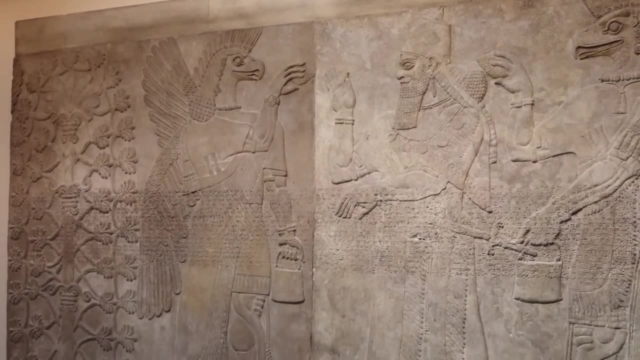 and marched on the plain of Lagash Nindirsu. the warrior of Enlil, at his just command, did battle with Uma. At Enlil's command, he spread the great throwing net over it and set up burial mounds for it on the plains. 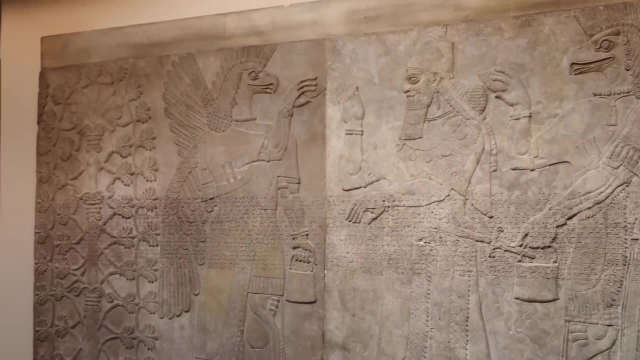 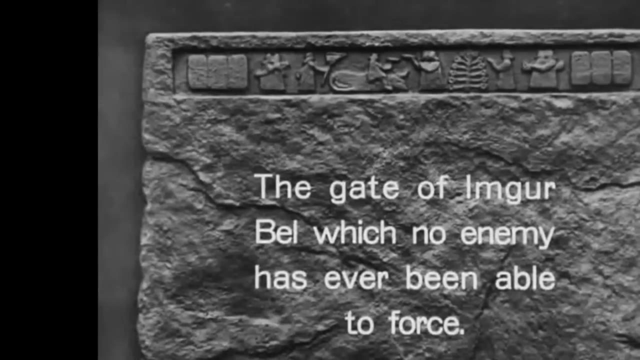 Since so little of the text on the stele of the vultures is intact and what remains is fragmentary, scholars are left to interpret the events based on the extant visual images. but due to the condition of the piece, that is also difficult. 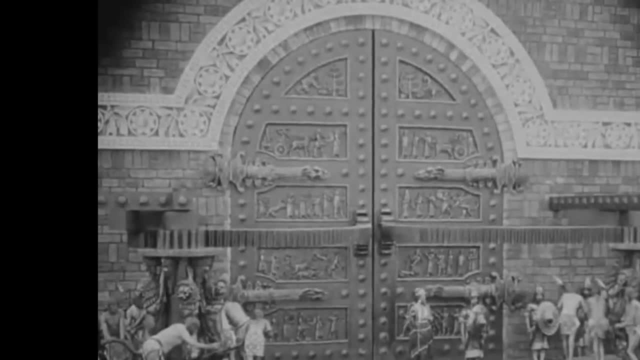 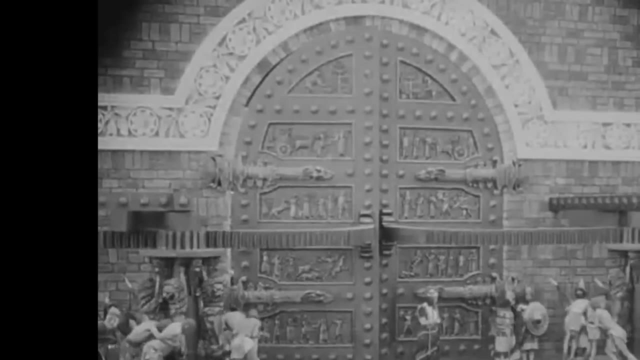 The obverse side contains two registers and the reverse side has four. The two sides can be read separately, but which direction one reads a particular side- from right to left or bottom to top- is extremely important and can determine the meaning of the narrative. 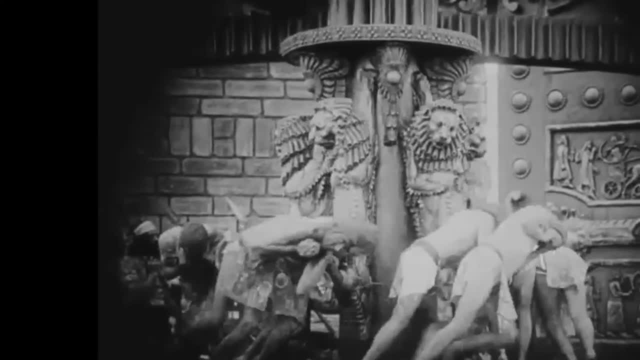 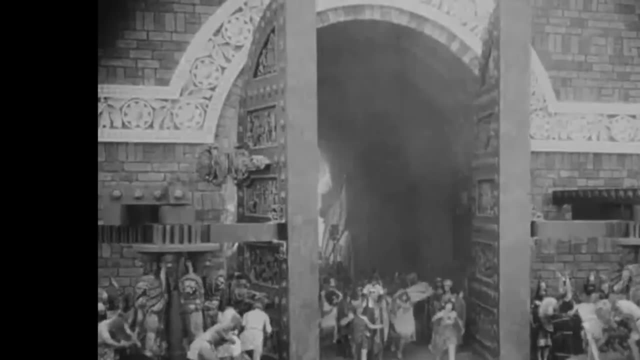 The obverse side tells the story from a spiritual or mythological perspective. The top register features a male figure, presumably Nindirsu, the patron god of Lagash, wielding a mythical zoo bird and holding Numenobuma in a net. 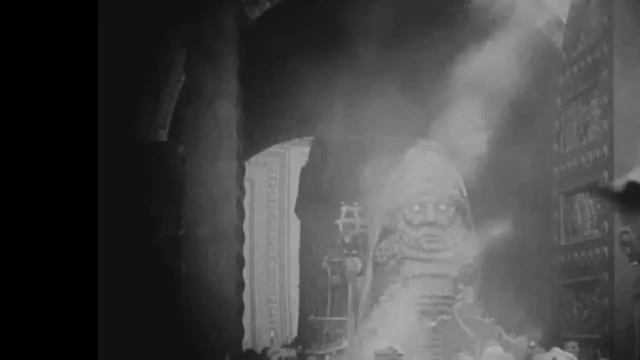 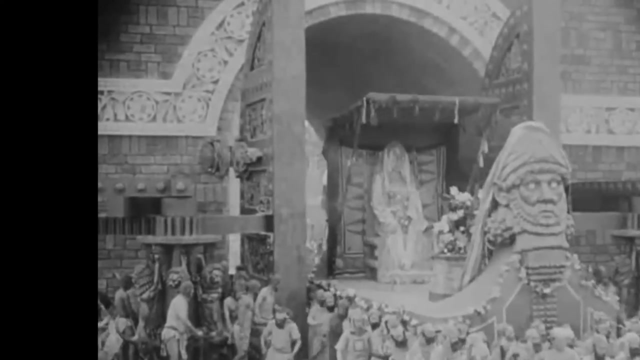 It should be pointed out that the zoo bird also had negative connotations in Mesopotamian mythology. It may be important for the purposes of the stele's narrative that in some myths it was Shara, the god of Uma, who vanquished the zoo bird. 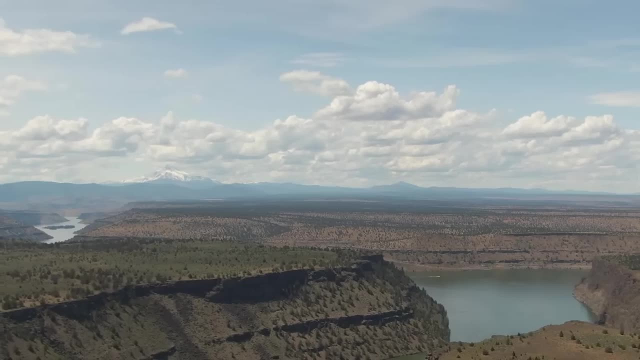 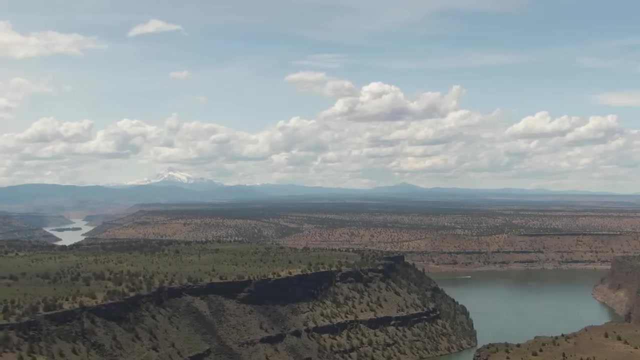 Nindirsu is accompanied by a female figure who is believed to be his mother, Nindirsag, The obverse side tells the idealized story of the war between Uma and Lagash. Nindirsu gives victory to his loyal followers. 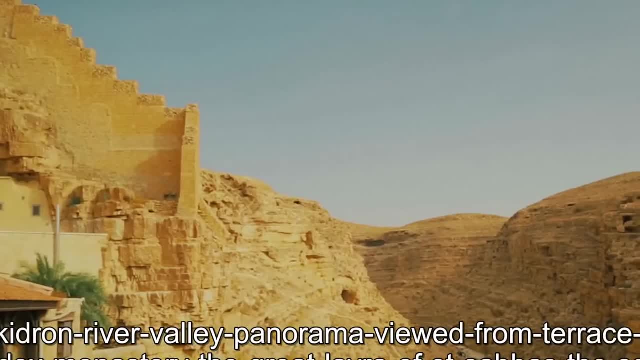 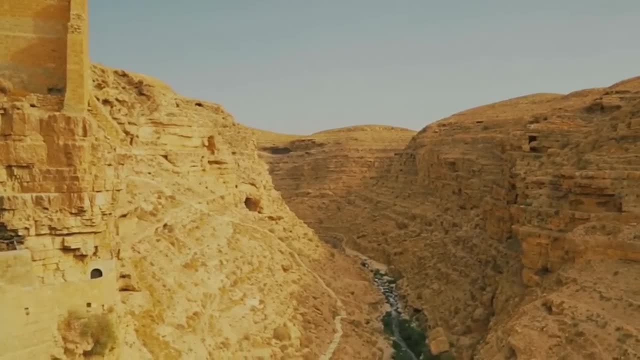 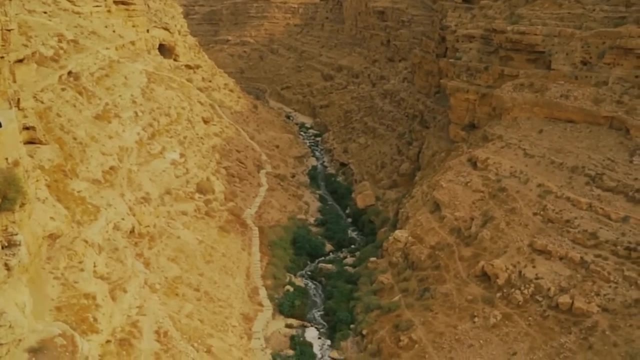 and vanquishes Uma himself. while the reverse side is much closer to a true historiographical text, The obverse side features a flock of vultures carrying the heads of the men of Lagash, and while this is clearly symbolic, it may also somewhat be truthful. 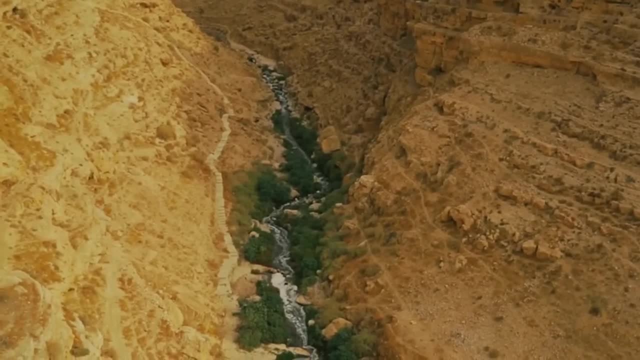 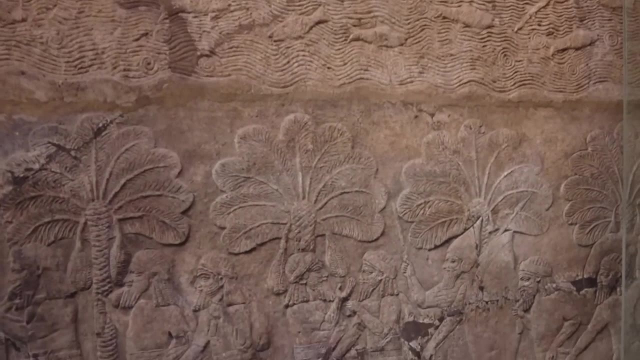 in the sense that vultures probably did pick at the remains of the dead after the battle. The top registers of the obverse side feature a military encounter with thirteen dead men of Uma gathered in a pile. The second register shows a group of soldiers. 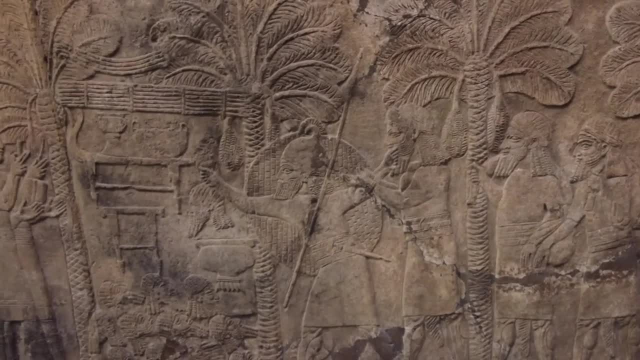 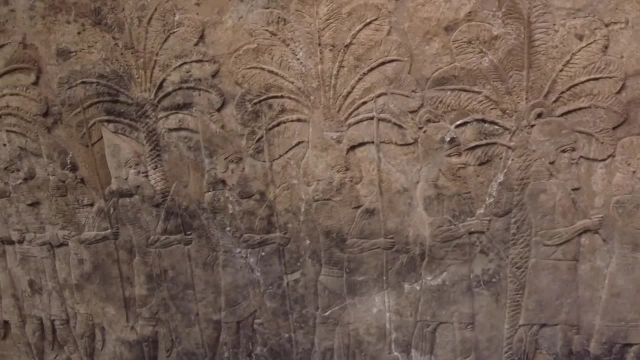 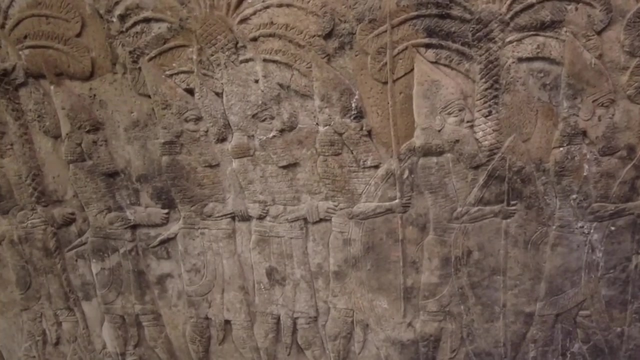 with spears and shields, following what is most likely the king or ensi of Lagash, who is in a war chariot. The third register depicts a figure seated in front of a bull that appears to be ready for sacrifice. To the bull's left is a pile of bodies. 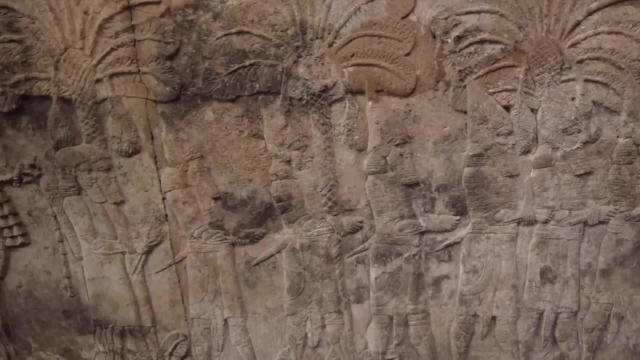 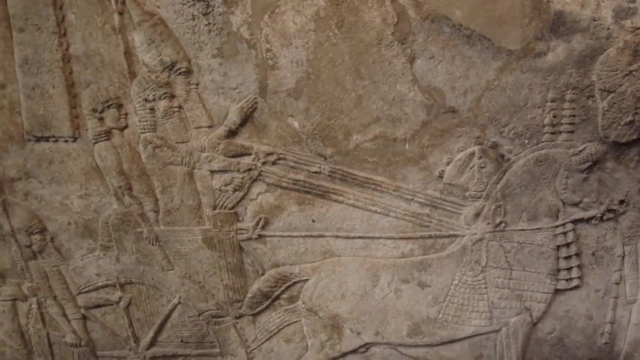 which are apparently the fallen warriors of Lagash. The fourth register appears to be another battle scene, with one man spearing another man. Obviously, the registers visually chronicle the war between Uma and Lagash, with the vultures in the upper right corner. 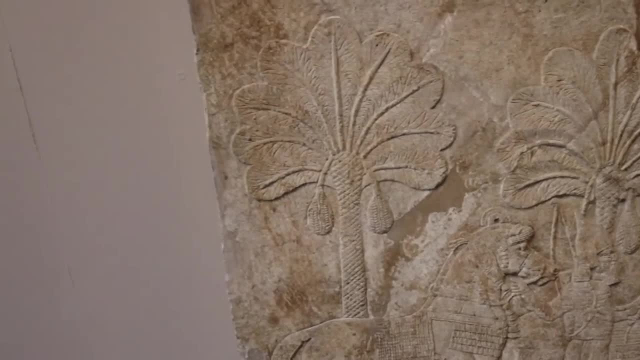 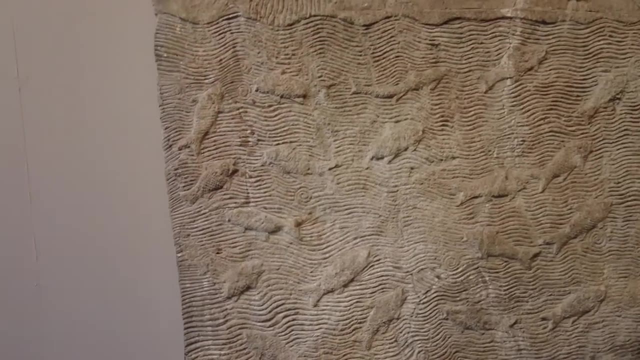 signifying Lagash's ultimate victory. Most scholars have assumed that the registers should be read from top to bottom, but Irene Winter suggested that they should instead be read bottom to top. Winter based her conclusion on similar early dynastic Mesopotamian texts. 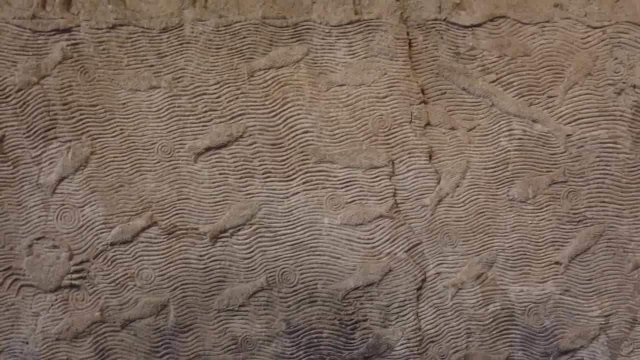 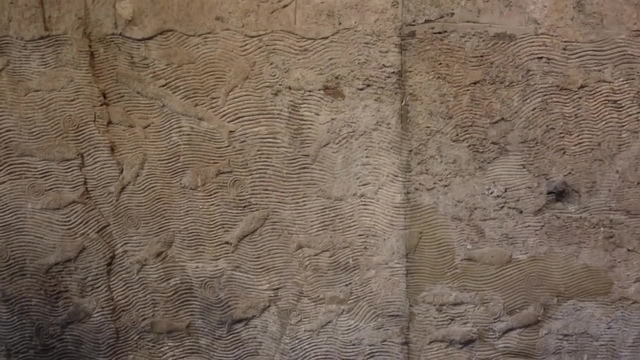 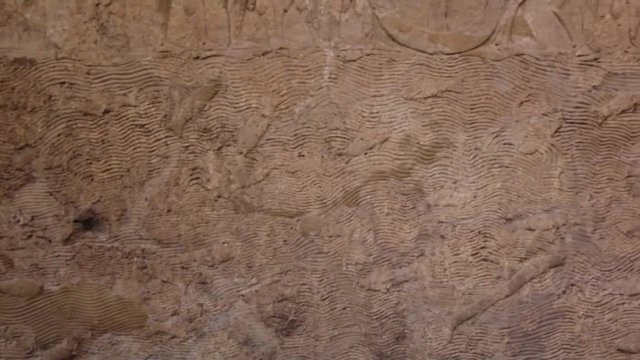 such as the Standard of Ur, which are usually read from bottom to top. The Standard of Ur is fully a pictorial scene without any text, depicting warfare on one side of Bastila and victory feast scenes on the opposite side. The connection between the military encounter. 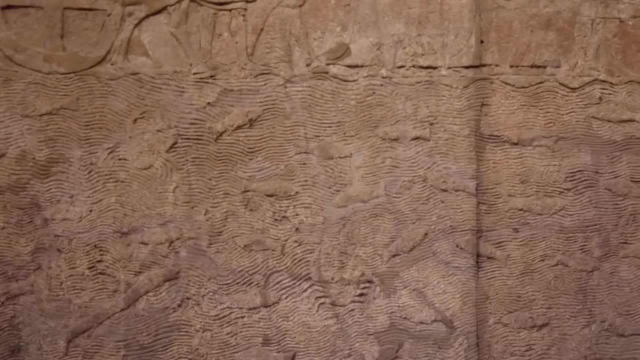 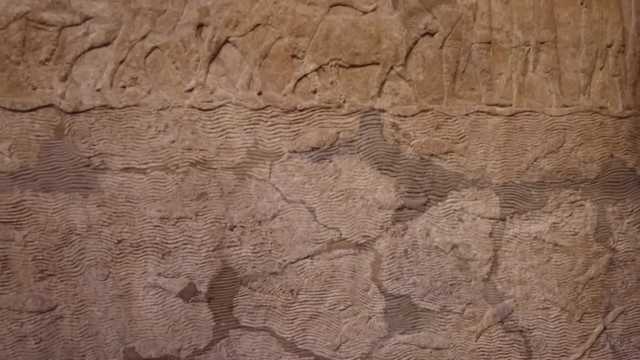 on the one side and the victory feast on the other are clear and not in need of accompanying text and, unlike the stele of the vultures, the Standard of Ur is completely intact. If the registers are read as Winter suggested, then the bottom register tells of the initial conflict. 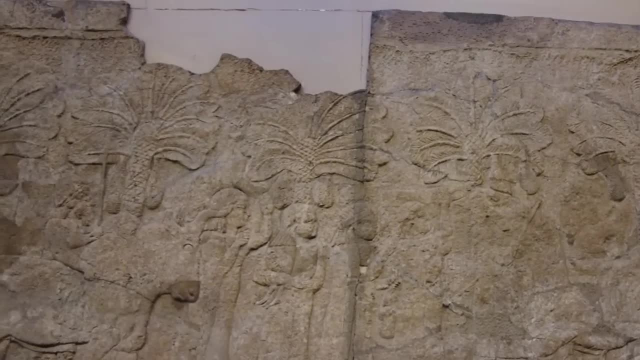 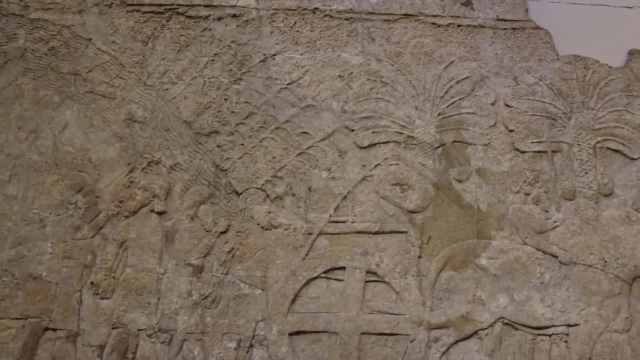 between Uma and Lagash, with the third register relating to a dream or vision Iannatum had before the conflict resumed. The dream is important in a theological sense because it justified Magash's war against Uma and assured them that they were on the right side. 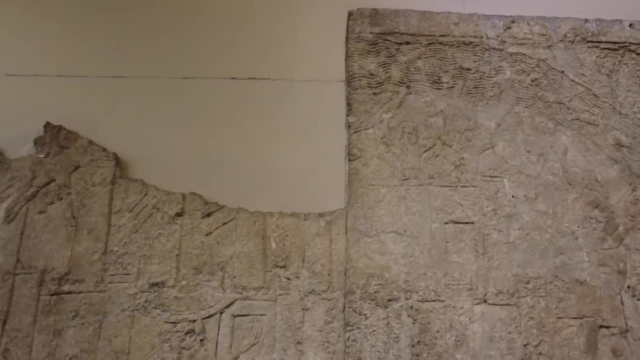 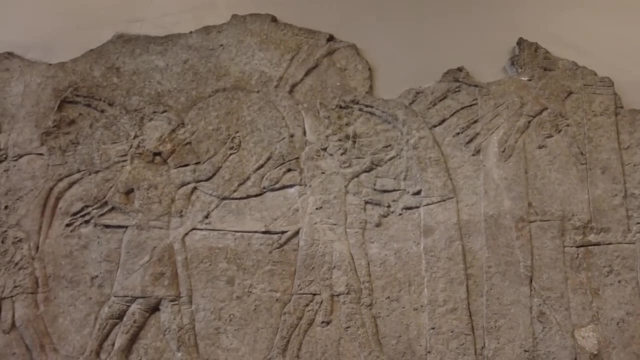 because if a god sent a king an omen of victory, then that king could be assured that he would in fact win. The second register then shows the king leading the troops to battle, and the top register shows the results: the utter defeat of Uma. 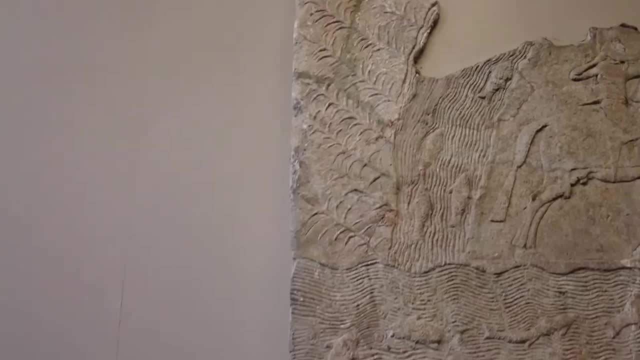 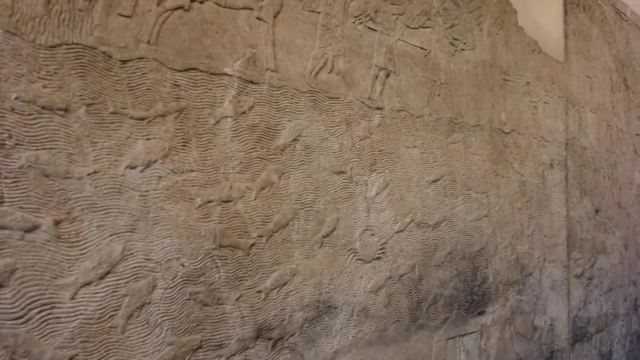 When read in the order and manner as Winter argued, the stele of the vultures does in fact read like the Standard of Ur and is somewhat straightforward. The second to the bottom register is perhaps the most confusing part, but if it represents a dream, as Winter believes, 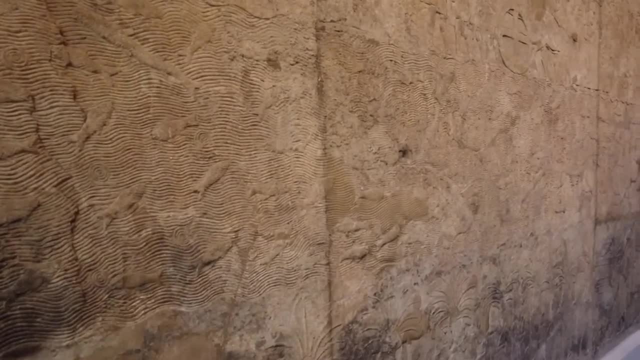 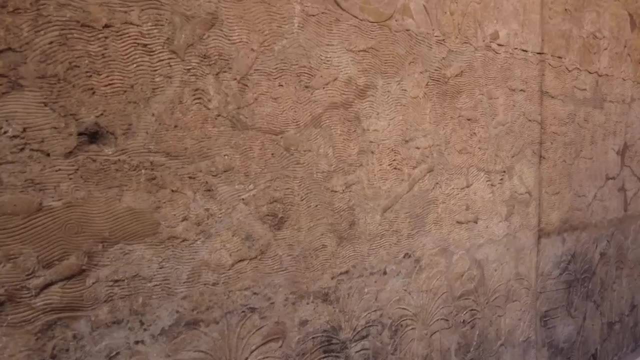 then it makes sense. The stele of the vultures is important for some of the details it relates of this conflict between Uma and Lagash, but it also relates some other important aspects of Sumerian culture in general. The second register from the top. 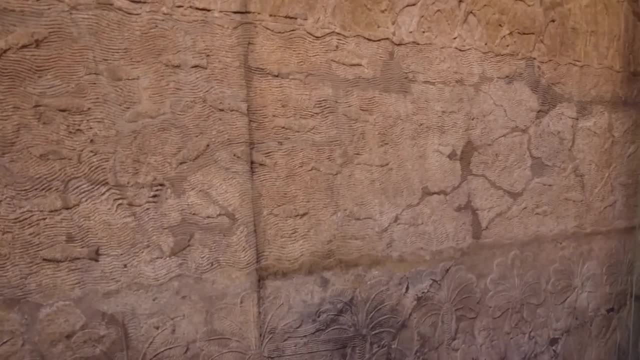 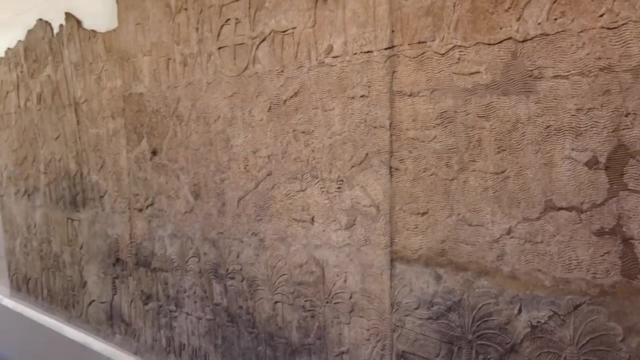 on the reverse side of the stele depicts how battles were fought in early dynastic Mesopotamia. Armies were well armed and fought in a shield wall, but, most significantly, they were led into war by their king or ensi. This became a tradition that was carried out. 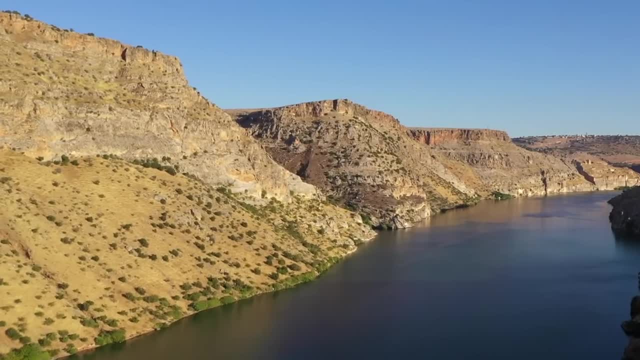 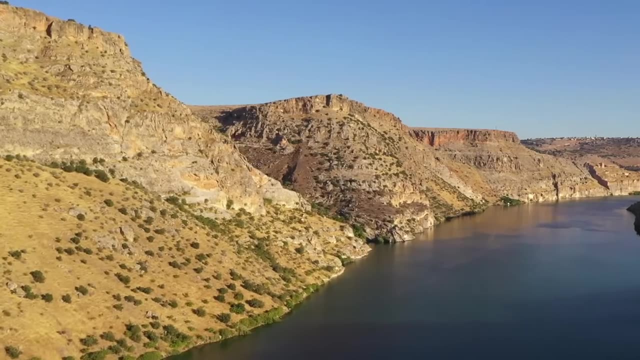 by Mesopotamian kings and governors throughout Mesopotamia in the early dynastic period, most notably by Sargon of Akkad. The fact that the ensi led his troops into war means that there is a good chance that Ninta of Uma was captured. 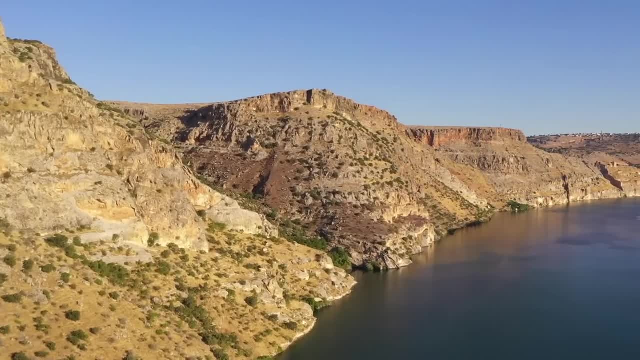 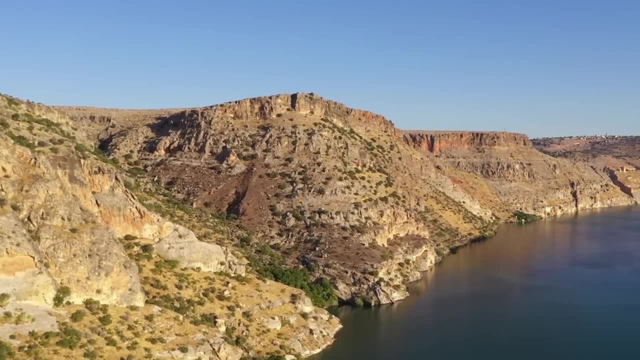 During or just after the battle. The text relates that the ensi of Uma was obliged to swear a fealty oath, although that does not necessarily indicate that he was present when his army was defeated. The stele of the vultures is also culturally important. 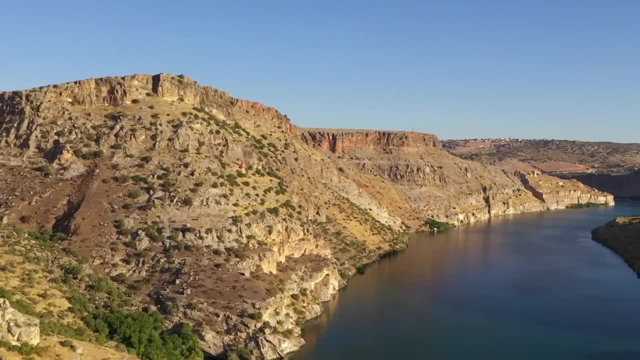 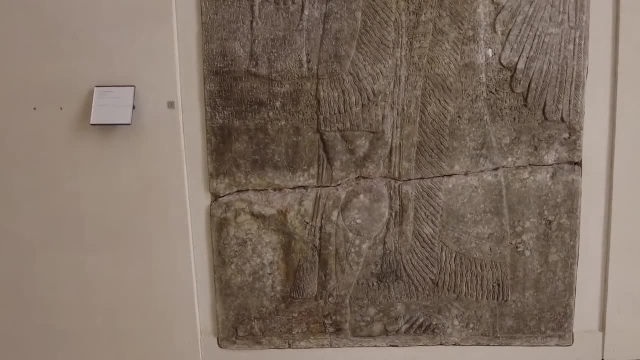 in other aspects, As were the earliest examples of Sumerian historiography and the oldest known example of a Mesopotamian battle relief, the stele of the vultures, likely served as a template for later Mesopotamian historiographical texts. 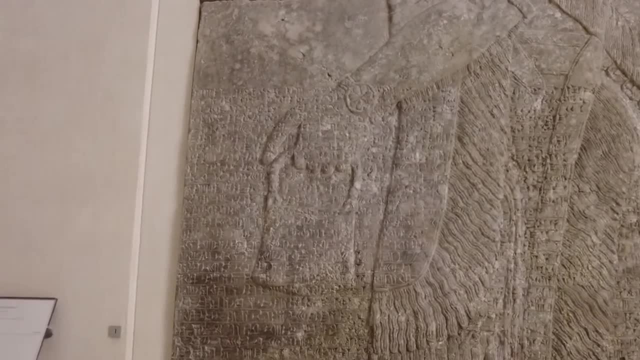 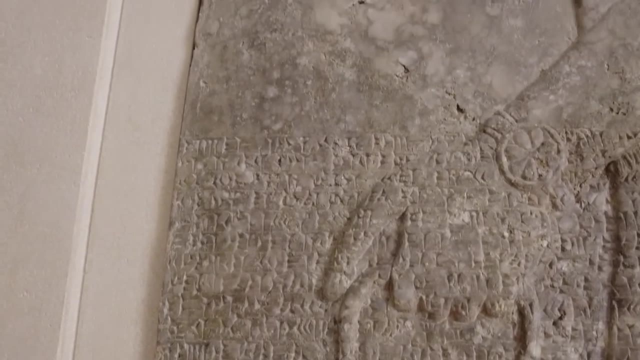 in the early dynastic period and beyond. After the early dynastic period, Mesopotamian historiography became much more developed and included more detailed battle accounts. The genre continued to evolve, culminating with the graphic Neo-Assyrian annals. 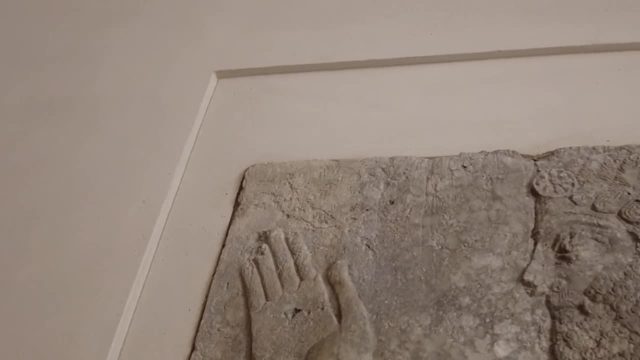 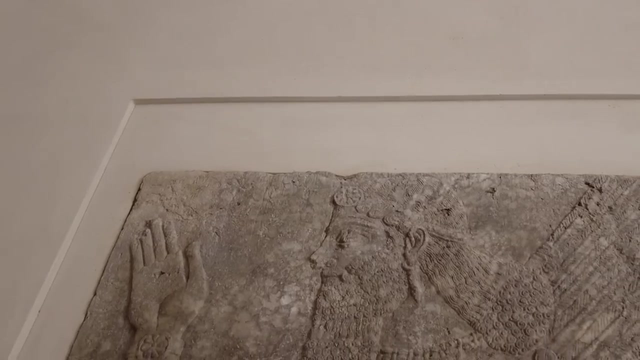 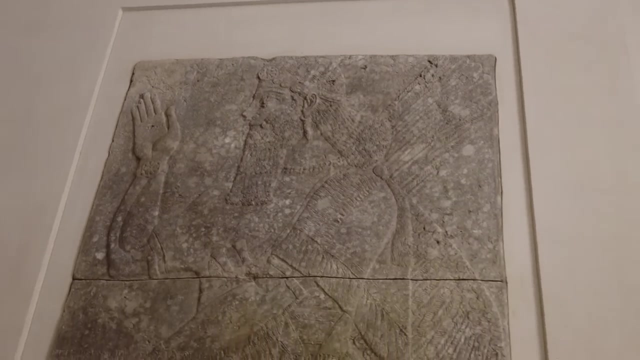 from the early 1st millennium BCE and the Neo-Assyrians certainly repeated the style of the stele of the vultures in terms of imagery and subject manner, Although the Neo-Assyrian texts were much more detailed. the visual representations that often accompanied the texts 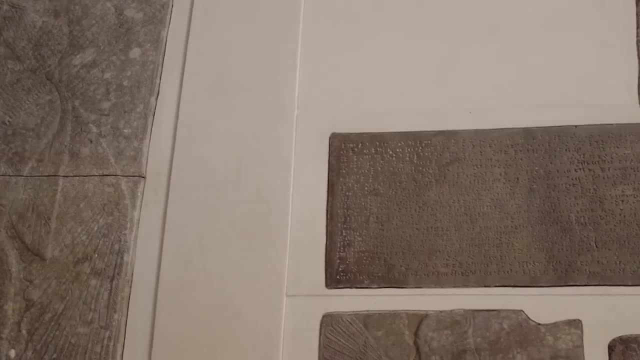 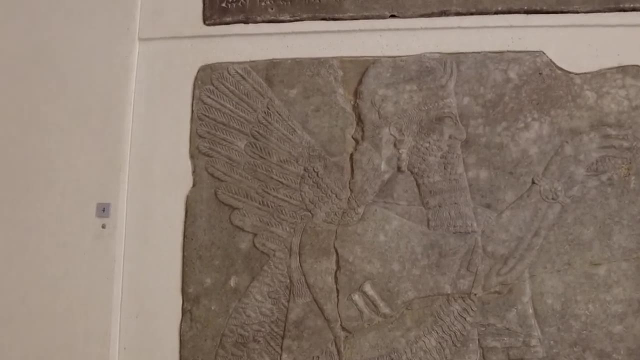 were rendered in the same multi-register format as the stele of the vultures. Not long after the stele of the vultures was created, another monumental text was created that further documented the Uma-Lagash conflict: a small clay, conical-shaped object. 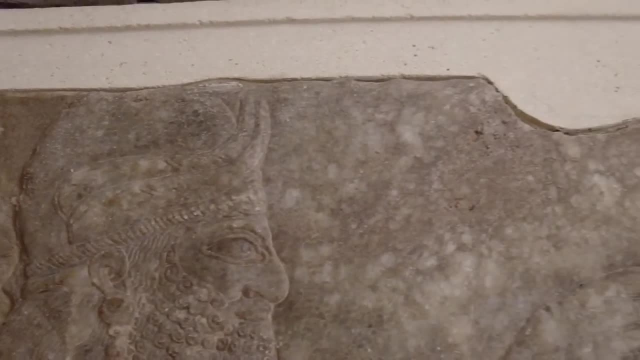 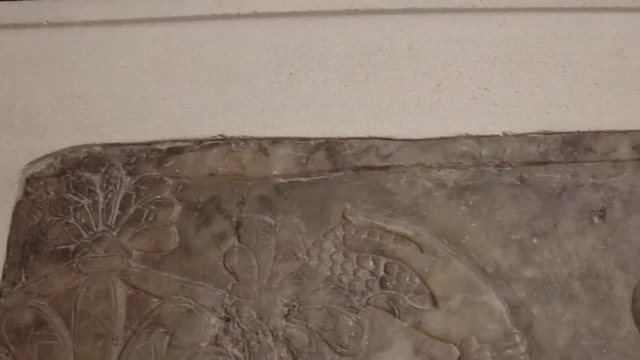 that became known as the cone of Entamena essentially picks up after the events of the stele of the vultures. The cone, which is inscribed in Sumerian genea form, is told from the perspective of Iannatum's successor in Lagash. 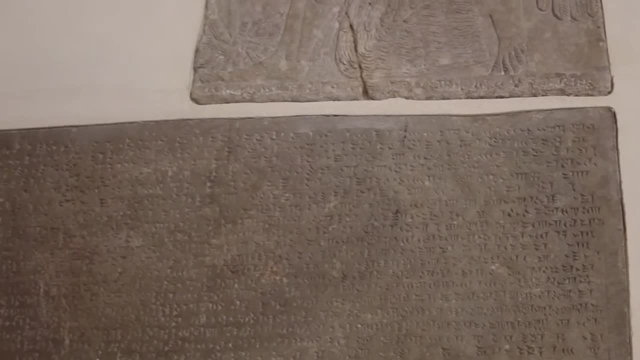 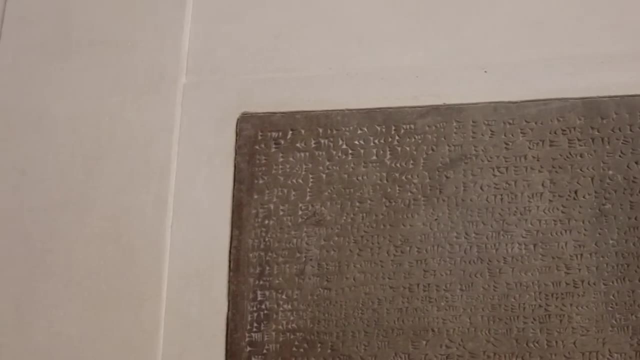 Entamena. According to the text, Enakale, the NC of Uma, after Ninta, infringed once more on the neutral zone between the two cities, incurring the wrath of Lagash. Part of the text reads: Enlil, king of the lands, father of the gods. 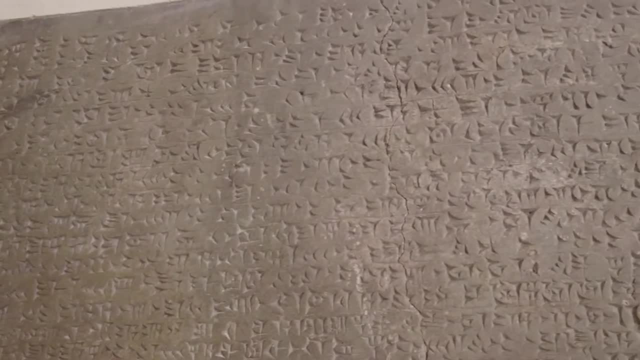 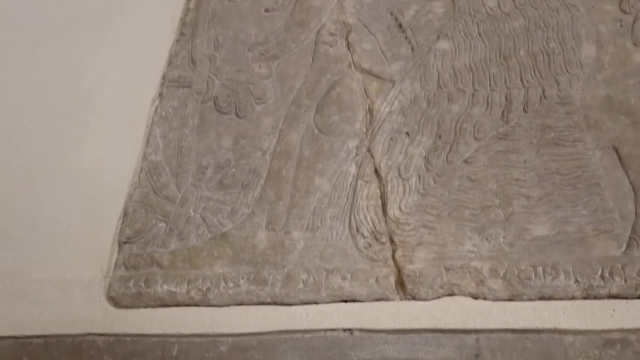 upon his firm command, drew the border between Nindirsu and Shara. Mesalim, king of Kish, at the command of the god Ishtaraan, measured the field and placed a stele. Ush ruler of Uma acted arrogantly. 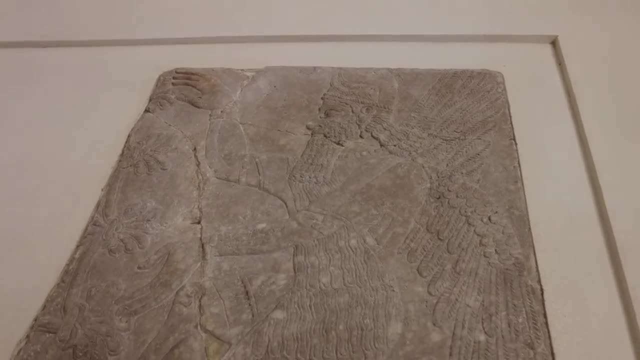 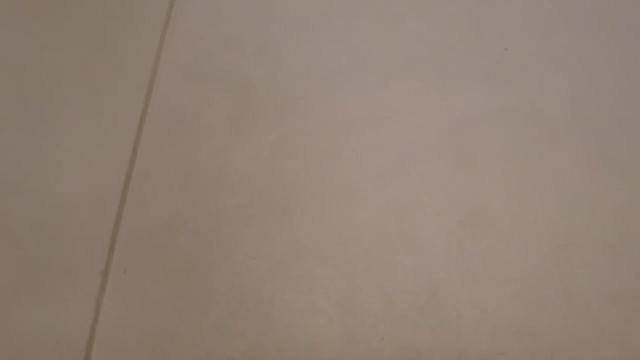 He ripped out the stele and marched onto the plain of Lagash. Nindirsu, the hero of Enlil, at the latter's command, did battle with Uma. Upon Enlil's command, he cast the great battle net upon it. 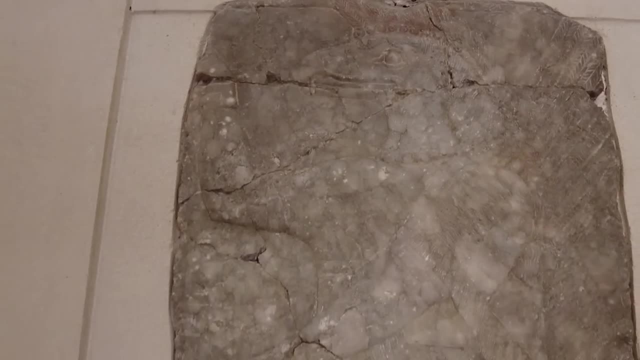 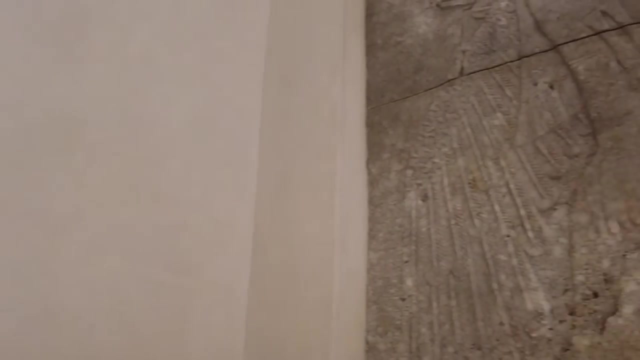 Its great burial mound was set up for him in the plain Iannatum. ruler of Lagash, the uncle of Venatena ruler of Lagash with Enakale ruler of Uma, drew the border At that time Il. 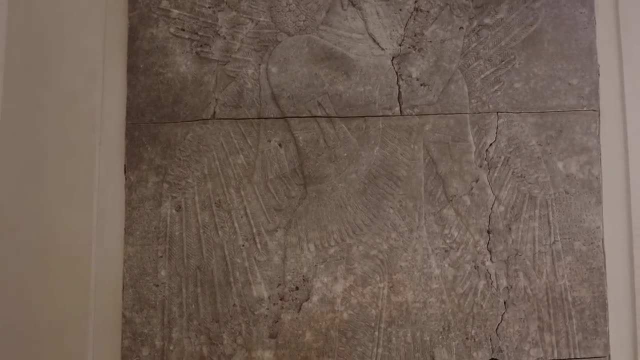 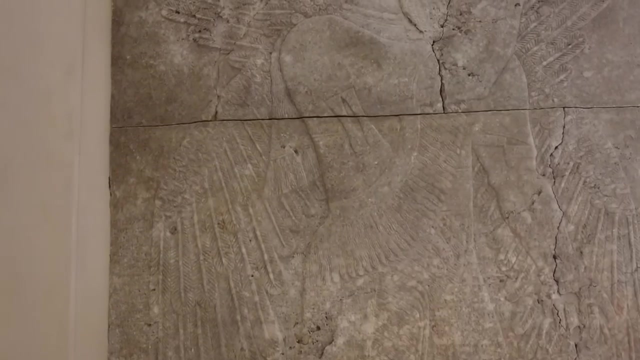 who was the head of the temple of Zabalan, made a retreat from Girsu to Uma. Il received the rulership of Uma there Into the boundary channel of Nindirsu and the boundary channel of Nanshe, the levee of Nindirsu. 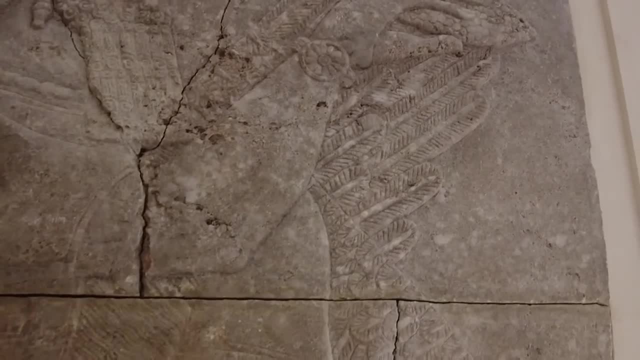 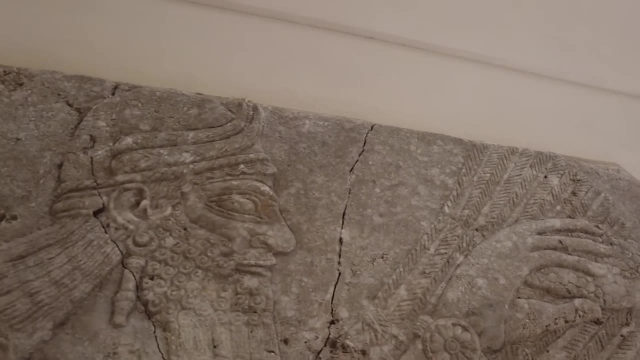 being at the edge of the Tigris and on the boundary of Girsu, the Nannun-dakikara of Enlil Enki and Ninhursag. its water was diverted If the man of Uma in order to carry off the fields. 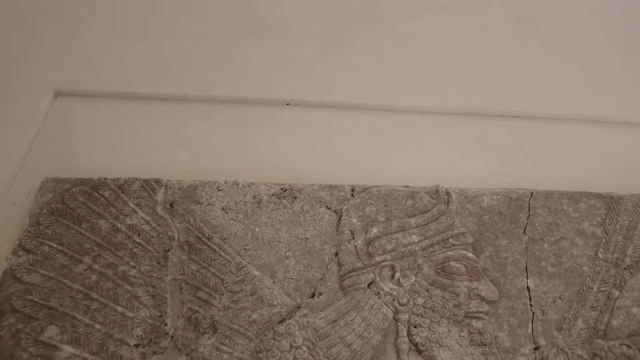 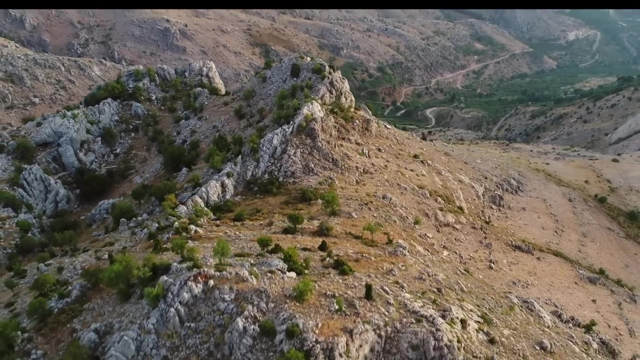 crosses the boundary channel of Nindirsu and the boundary channel of Nanshe, be he a man from Uma or a foreigner. may Enlil destroy him. may Nindirsu, after casting his great battle net, place his hands and feet upon him. 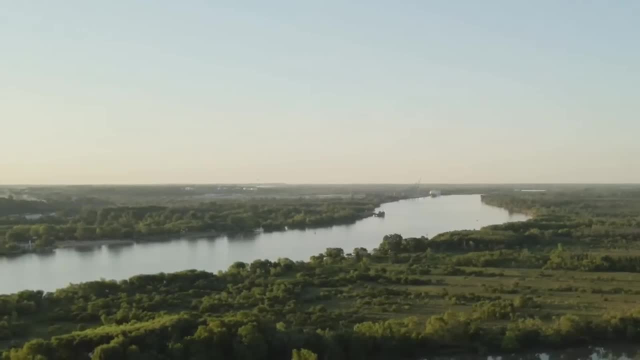 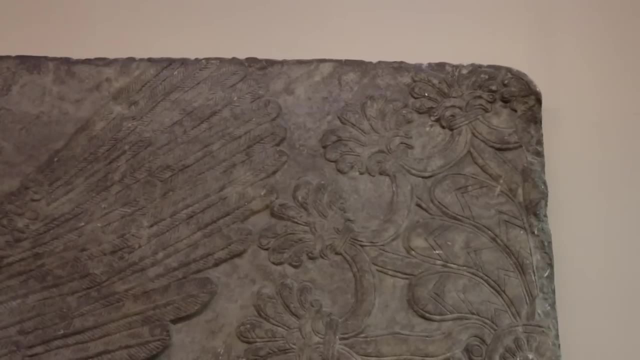 May the people of his own land, his own city, after rising up against him, kill him in the midst of his city. The text further chronicles how Inakale's successor, Uluma, also encroached on the neutral zone. 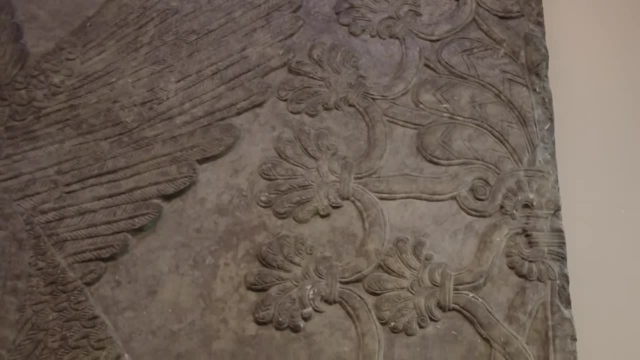 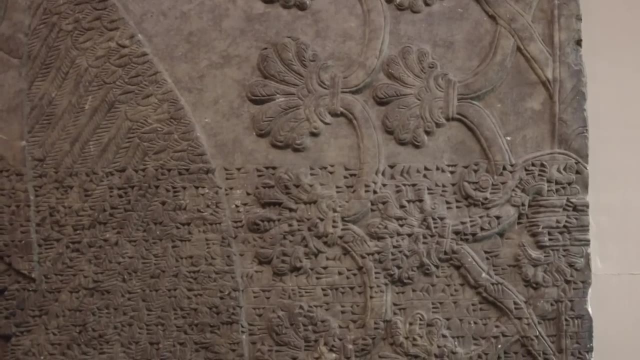 which led to more conflict. but when Il became the Ensi of Uma, he apparently came to an agreement with Lagash to once more respect the boundary conflict Based on the stele of the vultures and the cone of Entimena. 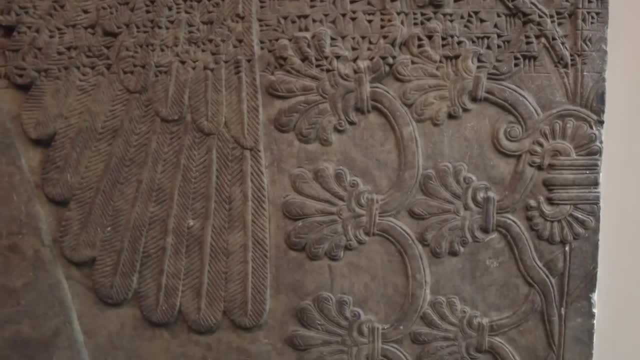 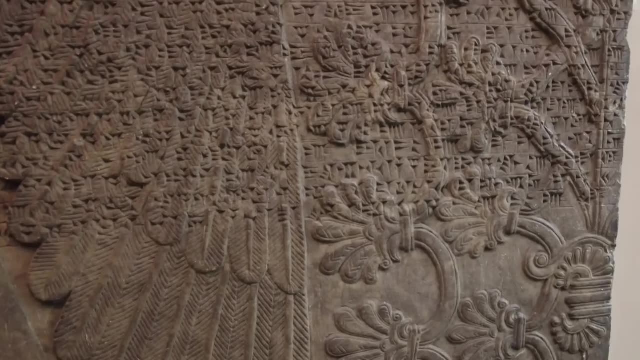 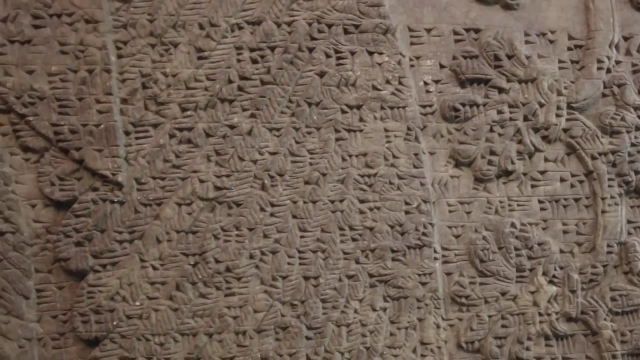 it appears that Lagash was clearly the superior city in the conflict, at least militarily. Archaeological and textual evidence shows that Lagash had a larger population and physical area, which would have given it a definite advantage in a protracted conflict over Uma. 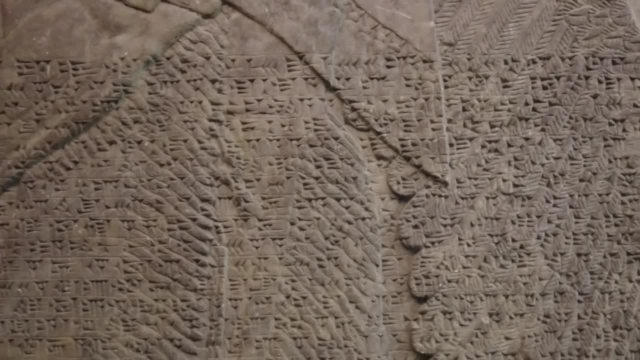 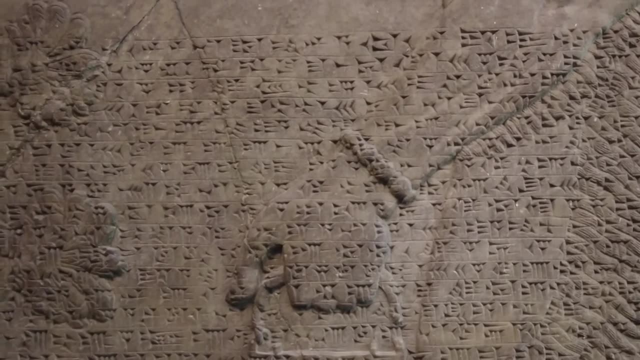 so it is likely that the texts are, for the most part, accurate. With that said, it must be pointed out that the texts were written from Lagash's ruler's point of view. In fact, while the historical and archaeological evidence suggests Lagash won most of its battles with Uma. 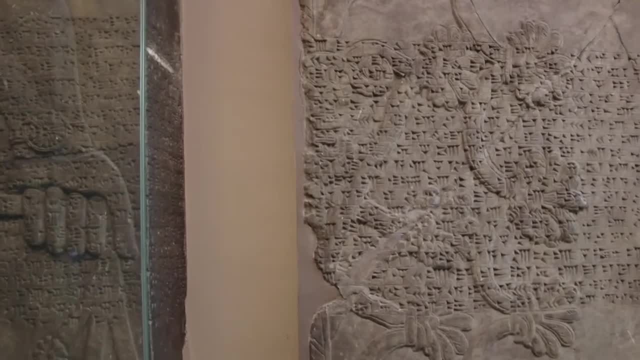 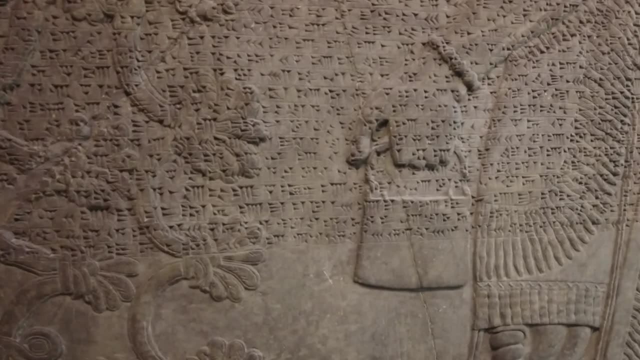 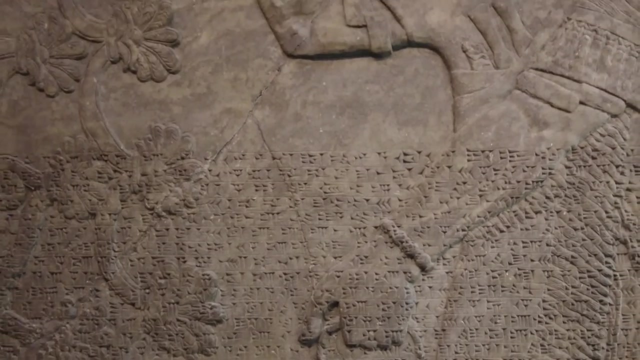 in the mid-third millennium. it eventually lost the war by the end of the third millennium, By the late third millennium BCE, the geopolitical situation began to change quite a bit in Mesopotamia, Although Uma and Lagash still occasionally battled for control of the lands near them. 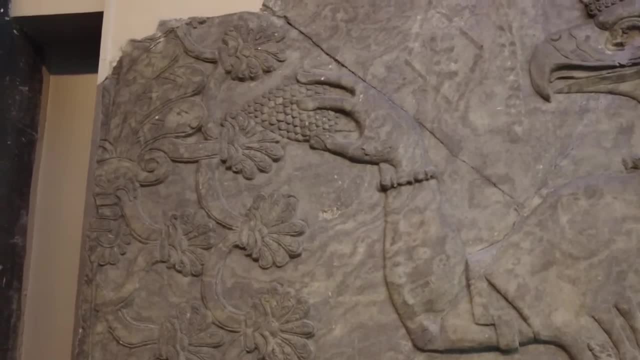 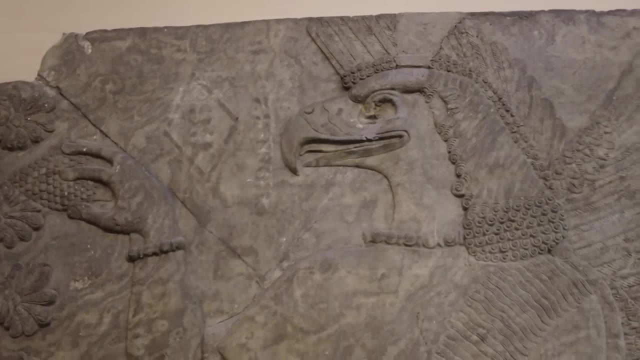 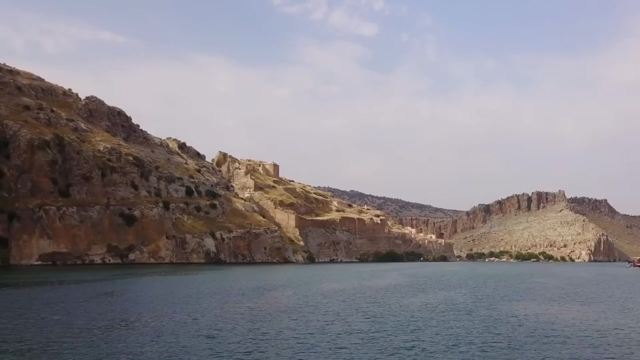 similar situations were being played out throughout Mesopotamia, and the Sumerians were no longer the most powerful ethnic group in the region. Semitic-speaking peoples north of Sumer began building their own powerful city-states that rivaled those of Uruk Ur, Uma and Lagash. 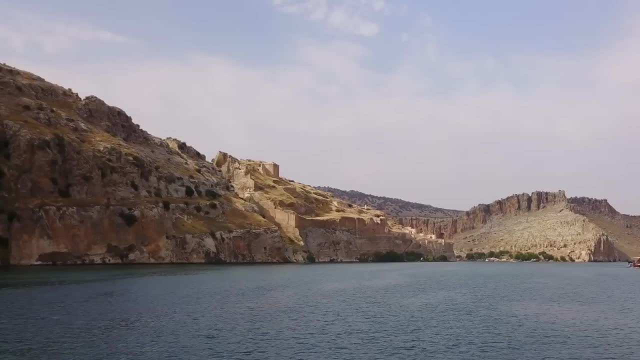 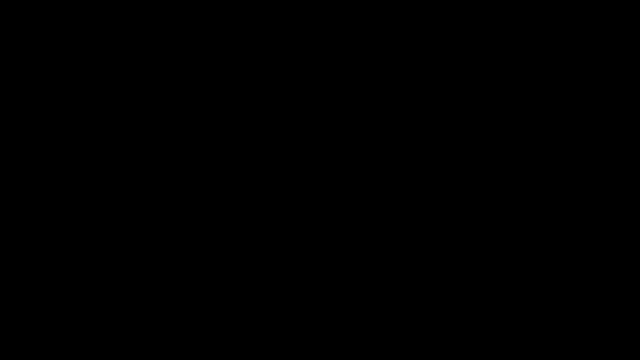 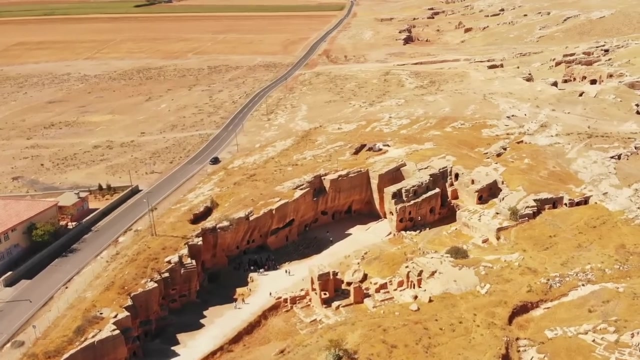 Wars began to involve more cities, much larger armies and took place over longer periods of time. Even if city-states wanted to stay independent and small, the emerging political situation would not allow them to do so, leaving them to make alliances and consolidate their forces. 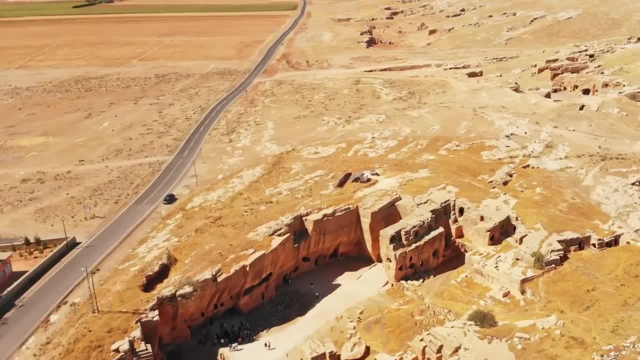 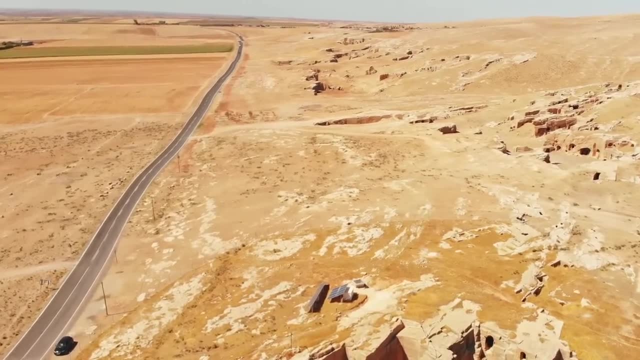 with other city-states to survive. Due to this new political dynamic, Uma and the other city-states of Sumer modified their relationships accordingly. Around the time that the events of the Khan of Antenna took place, the city-states of Mesopotamia- 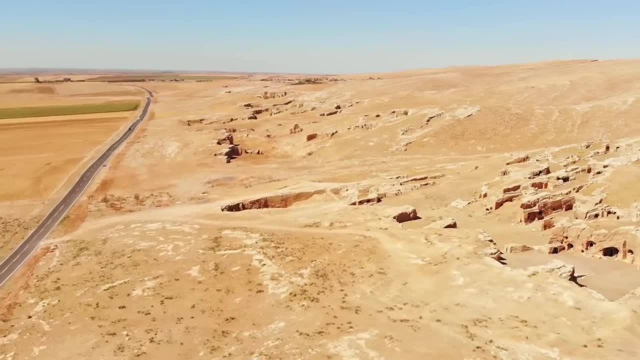 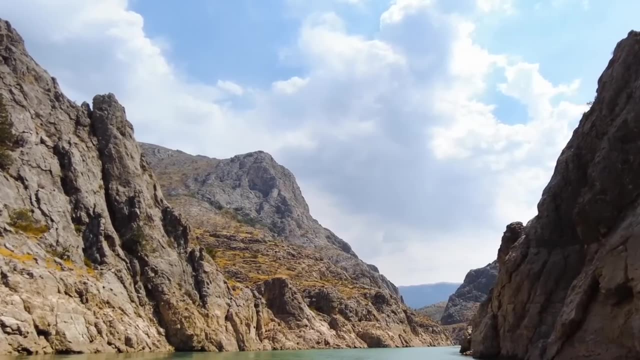 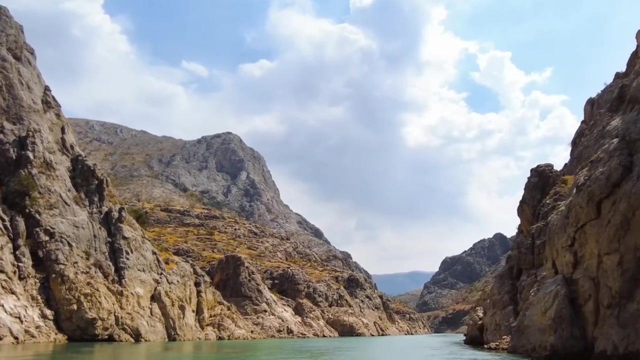 began reaching out to each other to form alliances, which eventually led to the formation of larger regional states. The formation of alliances that were taking place was a fluid process, though, And they sometimes involved strange bedfellows. For instance, Uma and Lagash were briefly allies. 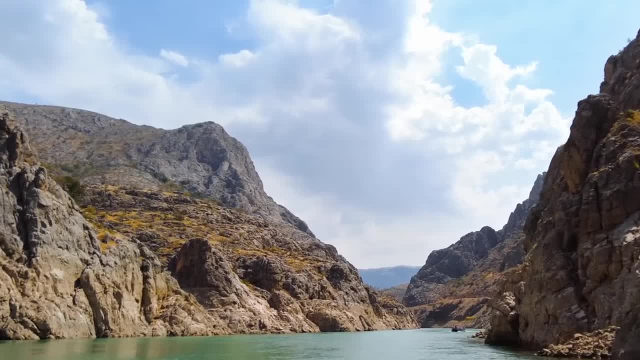 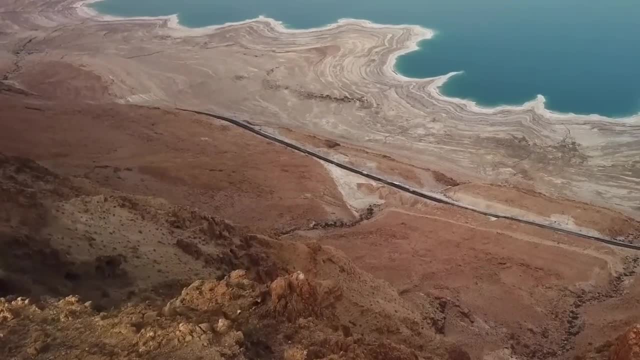 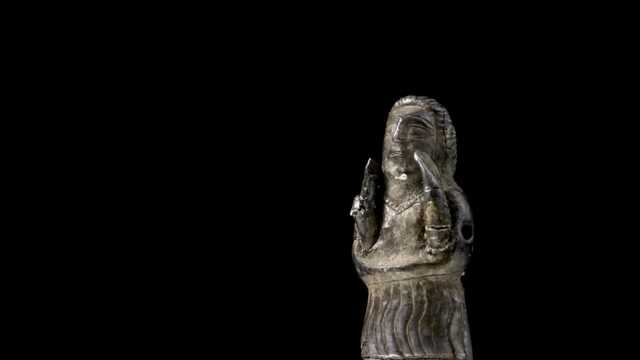 around 2500 BCE, before the events discussed by the Khan of Antenna fractured the alliance. The long history of antagonism between Uma and Lagash was not enough to override an alliance of convenience. But at the same time, the alliance was short-lived. 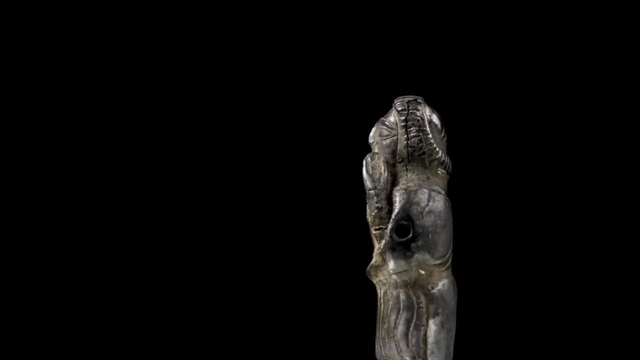 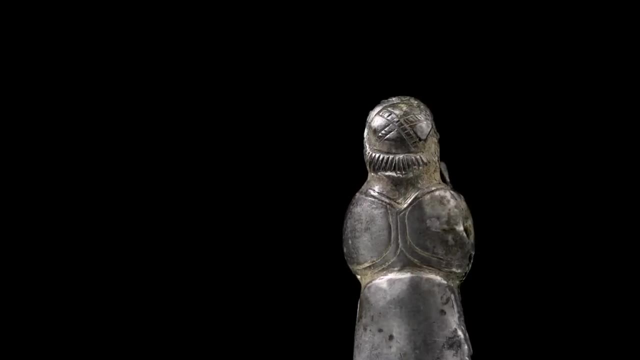 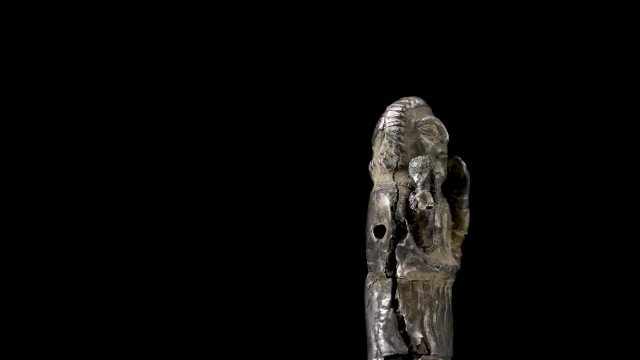 indicating that the border conflicts still festered. Eventually, stronger forces in Sumer and to the north would forcefully put an end to the Uma-Lagash conflict once and for all. The process of unification was facilitated by strong leaders who were willing to use military force. 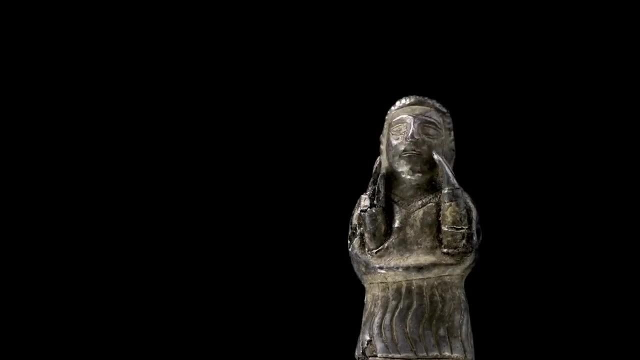 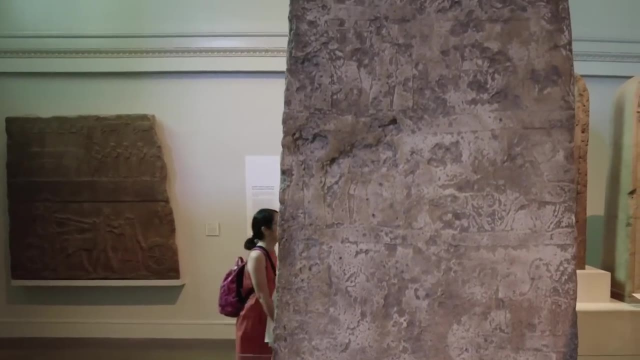 on recalcitrant cities. Lugal-Kidini-Dudu was the first of these notable Sumerian strongmen. He was the king of Uruk and later became king of the Lagash-Uruk-Ur confederacy, just before 2400 BCE. 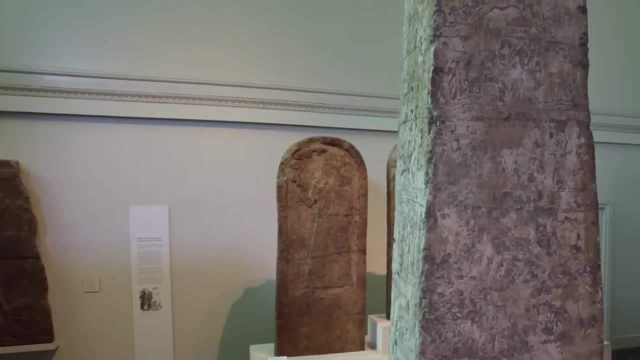 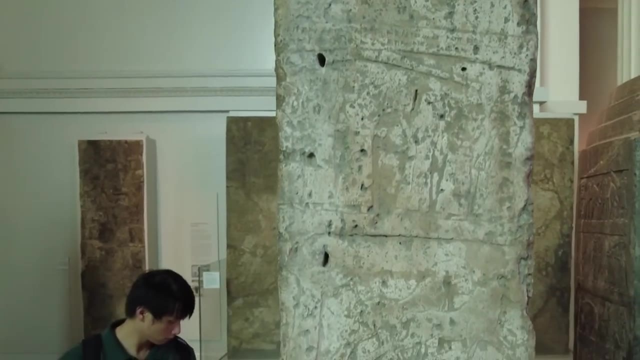 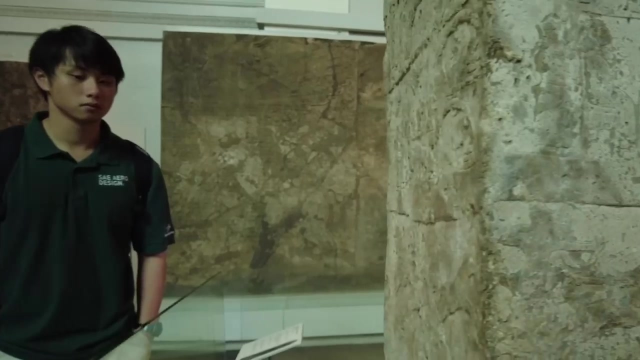 Uma was later absorbed into the confederacy, which quickly evolved into a unified Sumerian kingdom. Unfortunately for Uma, though, other than Lugal-Zaghesi having come from Uma, the city would fail to rise to the top of the Mesopotamian hierarchy of cities. 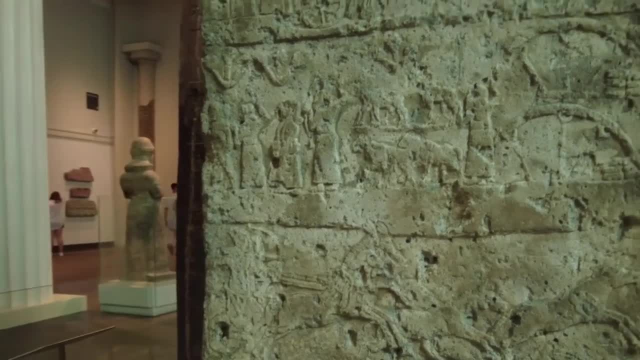 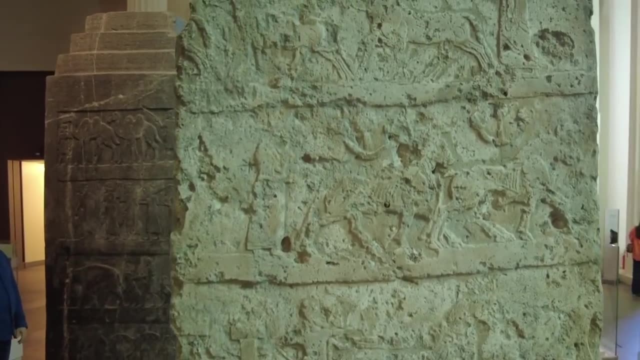 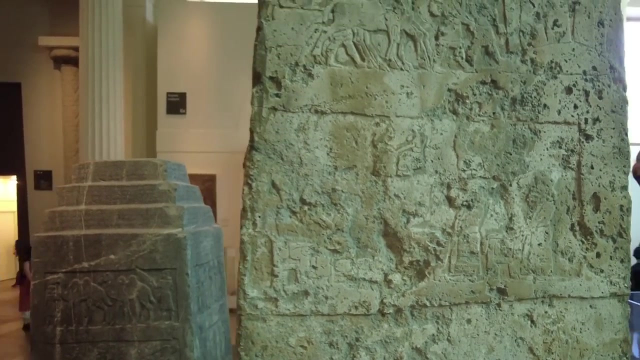 Uruk and Ur continued to be the most important Sumerian cities in the late Panastic period due to their size and prestige. All the other Sumerian cities, such as Uma and Lagash, looked to Uruk and Ur as examples of high Sumerian culture and civilization. 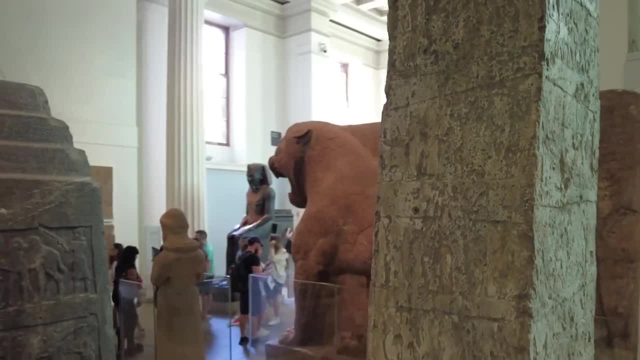 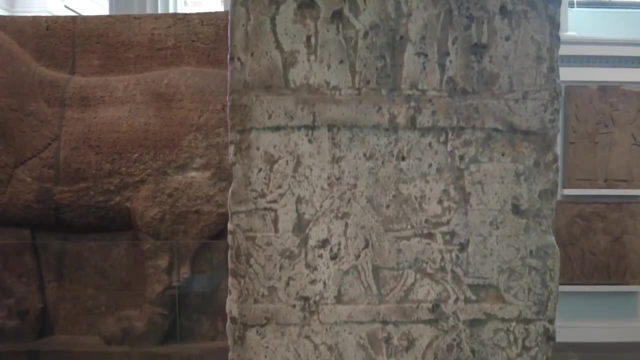 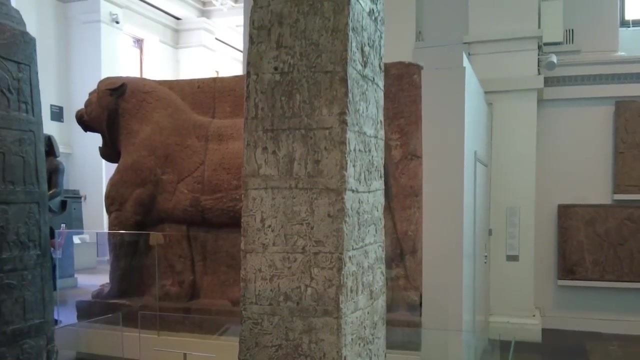 So they served as the inspiration for the period of regionalization and unification in the mid-third millennium. With that said, the force that made unification possible came directly from Uma, because Bukush, the final listed Ensi of Uma, was the father of Lugal-Zaghesi. 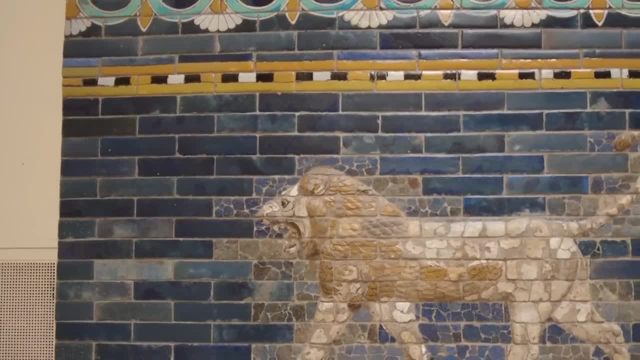 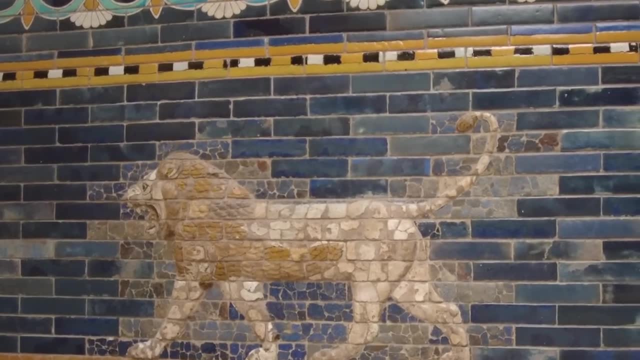 It was Lugal-Zaghesi who ultimately won the war of unification of Sumer, even as the details concerning how he did it are scant. Apparently, Lugal-Zaghesi was a new type of ruler unseen in earlier periods of Mesopotamian history. 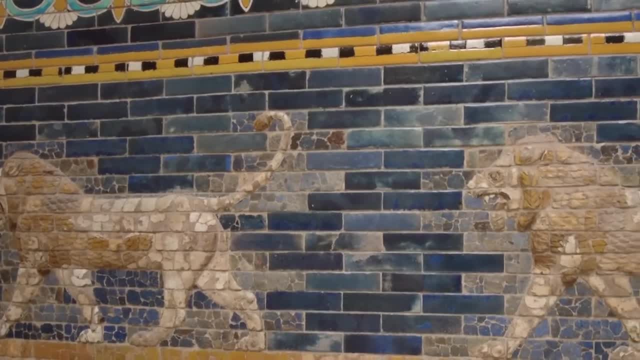 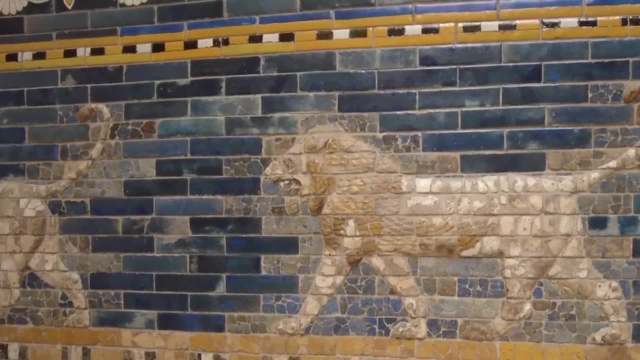 He used brute force when necessary, but he was also diplomatic, effectively using the carrot-and-stick approach to forge a new empire. Uma's old army, Lagash, was the final holdout and, according to one text from the period, Lugal-Zaghesi. 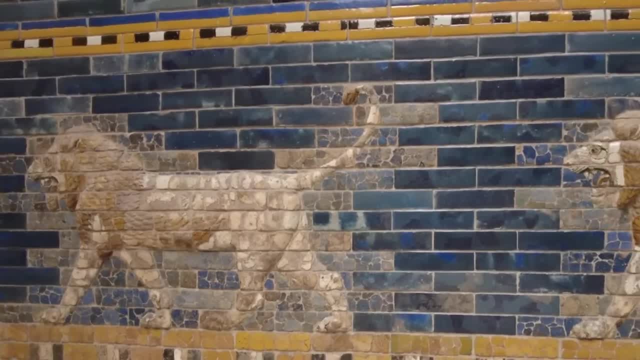 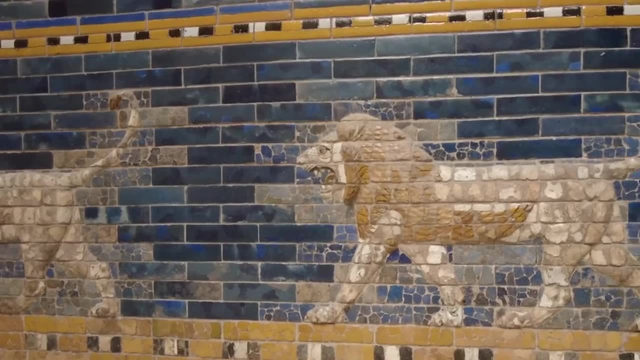 Lugal-Zaghesi did not spare the city any indignities. The man of Uma Lugal-Zaghesi, because he has destroyed Lagash, has sinned against Ngirsu. May the hand he has used against him. 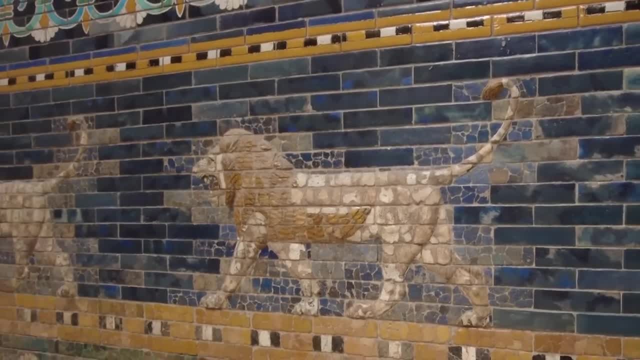 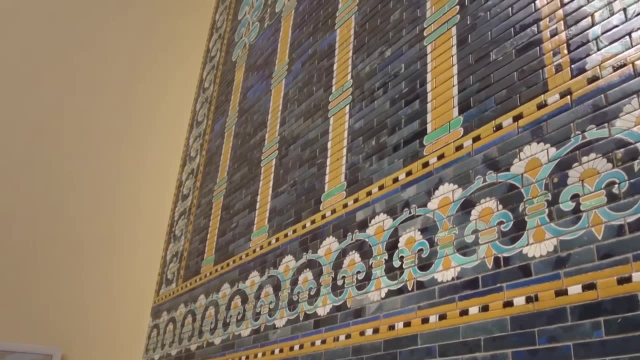 that is, the god be cut off. Uru-Mgina, king of Ngirsu, had committed no sin. May Nibdana, the goddess of Lugal-Zaghesi, ruler of Uma, carry this sin on her neck. 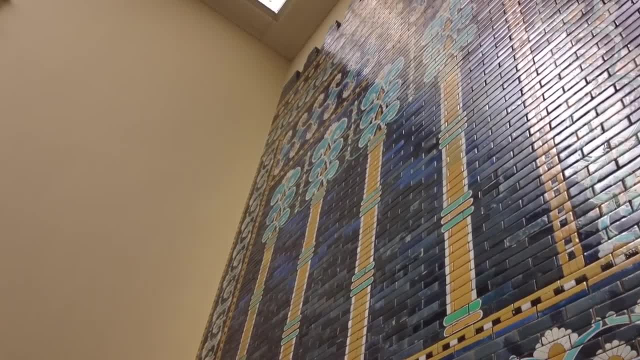 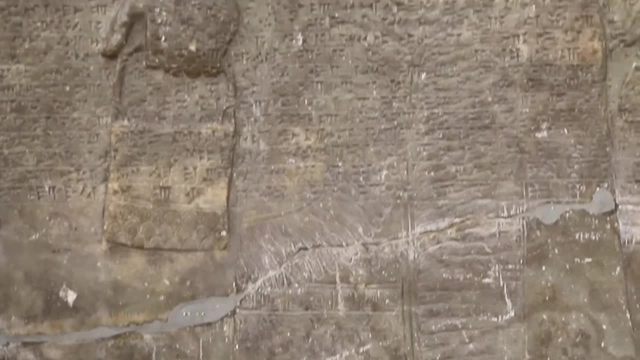 As it turned out, Lugal-Zaghesi and Uma would not have long to enjoy their time at the head of the new Sumer, because a new foe would come from the north and once again rearrange the geopolitical situation: The period of Sumerian dominance in Mesopotamia. 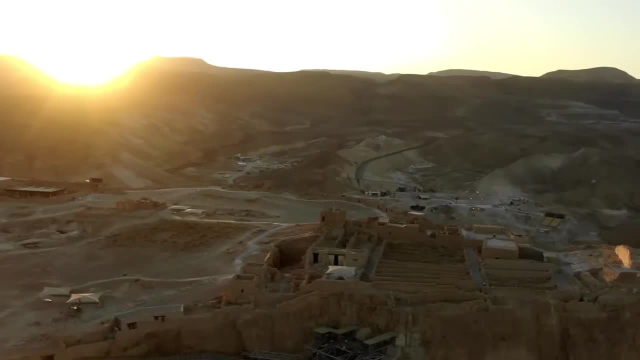 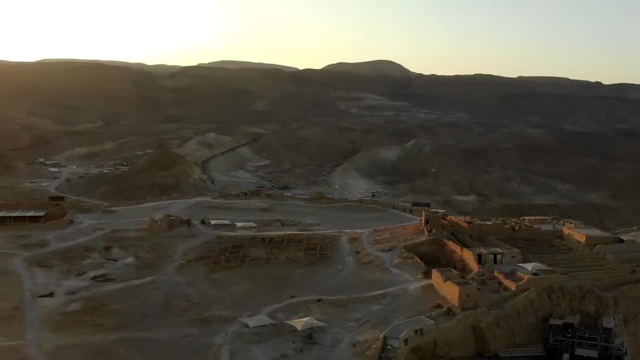 came to an end when Sargon of Akkad came to power. Akkad was a Semitic-speaking city and region to the north of Sumer that grew in influence as the Sumerian cities were battling for hegemony of their own areas and Sargon established a powerful dynasty. 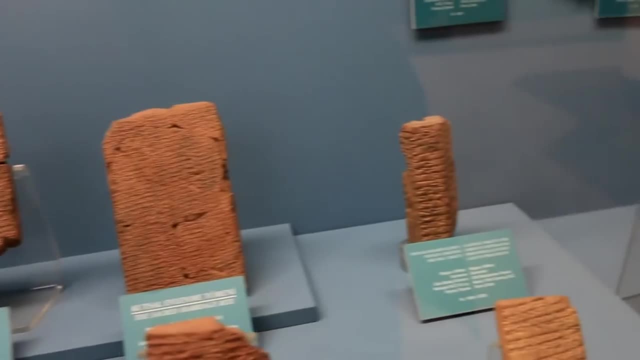 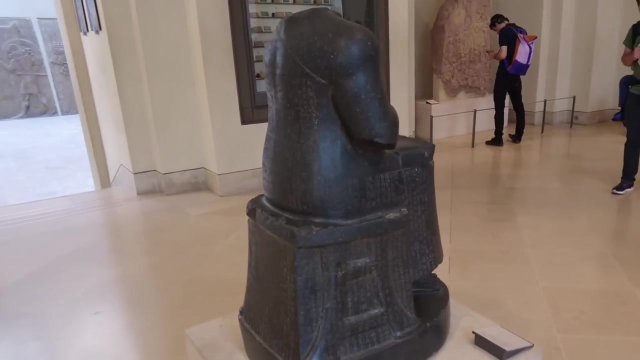 in Akkad, but he was still unable to crack the Sumerian resistance until fissures developed among the Sumerians. Apparently, Irikagina, the Ensi of Uruk, was envious of Lugal-Zaghesi's power. 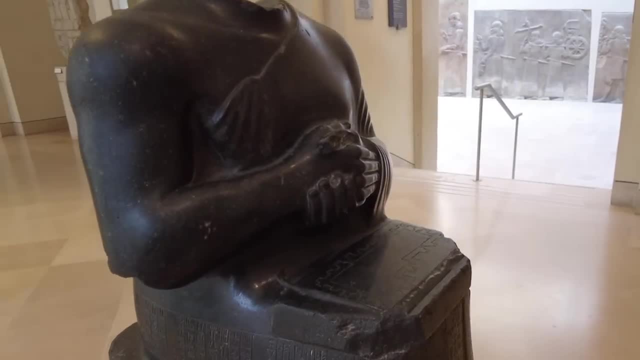 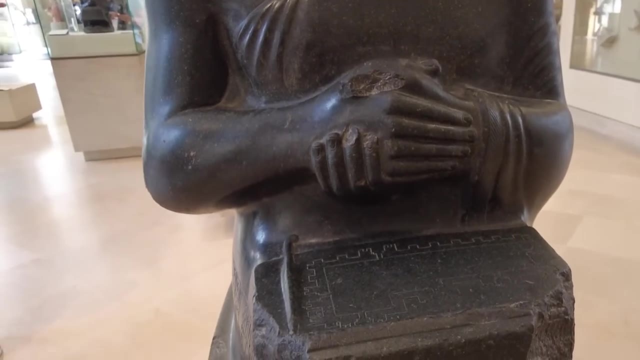 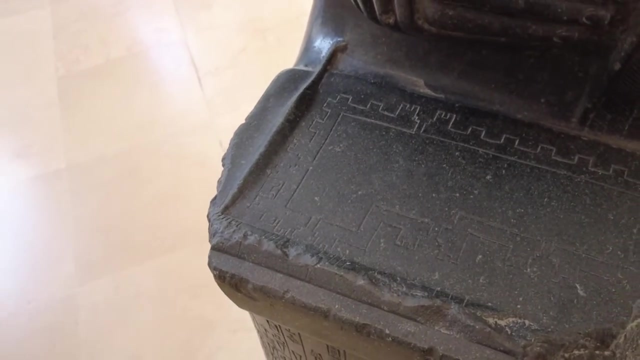 and his city's reduction in status. Either because he hoped to make Uruk and himself dominant once more, or perhaps just for pure revenge, Irikagina invited Sargon to Sumer to take care of Lugal-Zaghesi. The actions were documented in a text. 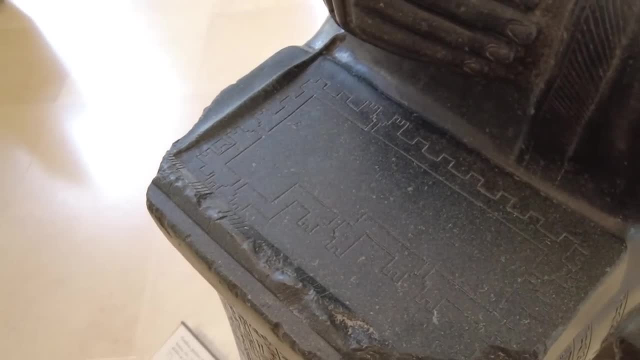 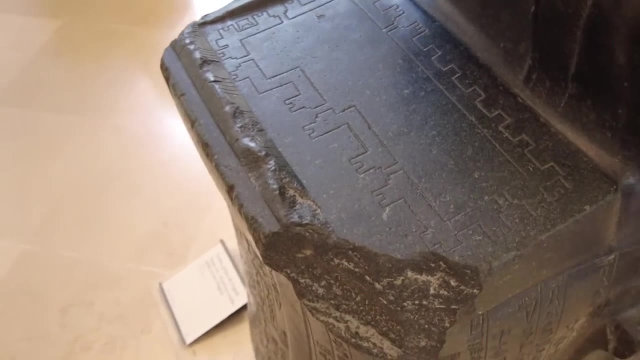 known as the Lagash Lament, part of which was cited in the previous paragraph. After describing how Lugal-Zaghesi was victorious over Lagash, the text relates that he was then defeated by Sargon. Sargon, king of Agane, overseer of Ishtar. 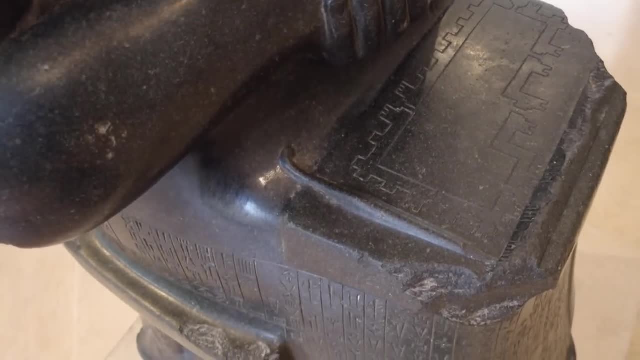 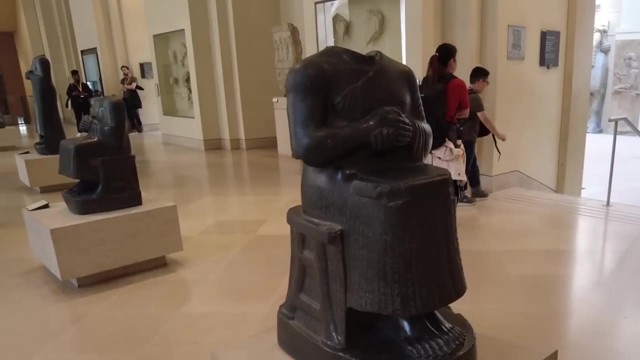 king of Kish, anointed priest of Anu, king of the country, great Ensi of Enlil. he defeated Uruk and tore down its wall In the battle with the inhabitants, in the battle with the inhabitants of Uruk. 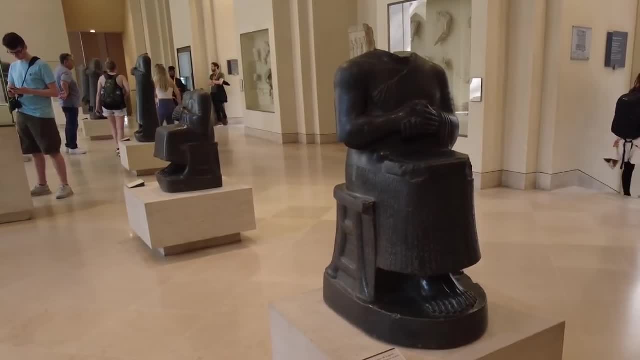 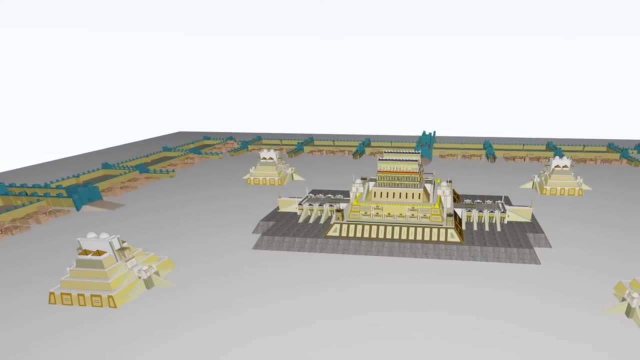 he was victorious. Lugal-Zaghesi, king of Uruk, he captured in this battle. He brought him in a dog collar to the gate of Enlil Sargon, king of Agane, was victorious in the battle with the inhabitants of Ur. 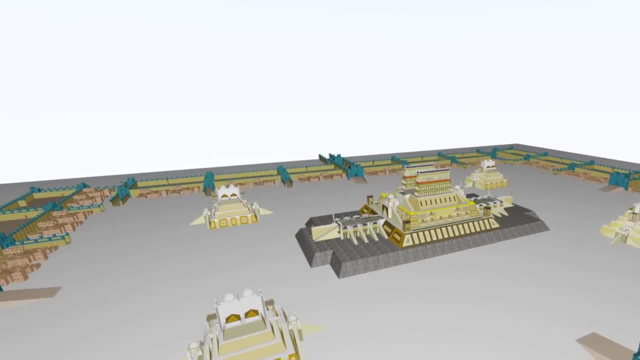 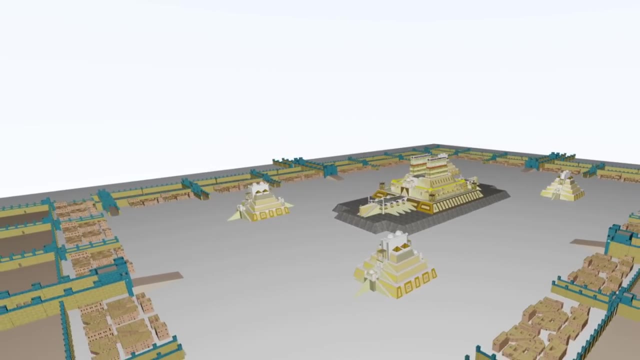 their town, he defeated and tore down its wall. He defeated the town Eninmar and tore down its wall and defeated also its entire territory. from Lagash as far as the sea, His weapon. then he washed in the sea In the battle with the inhabitants of Umma. 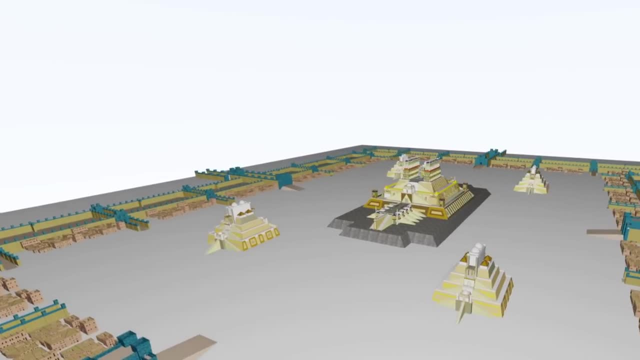 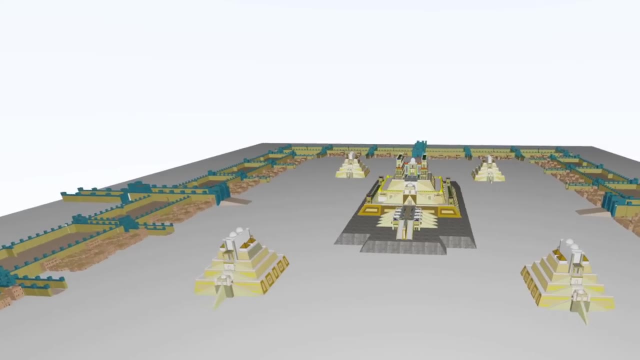 he was victorious. their town he defeated and tore down its wall. Although Sargon is the king mentioned who defeated Lugal-Zaghesi, the war probably took place late in his reign, so it may have been his son and successor, Rimush. 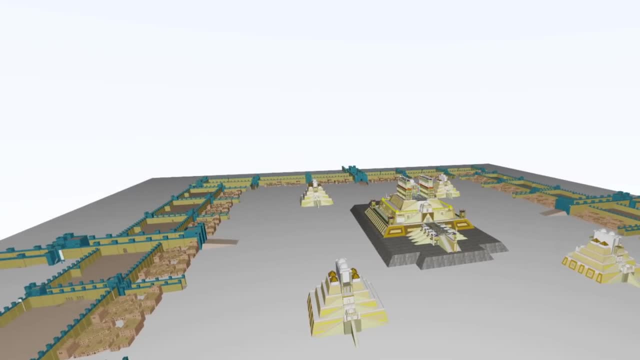 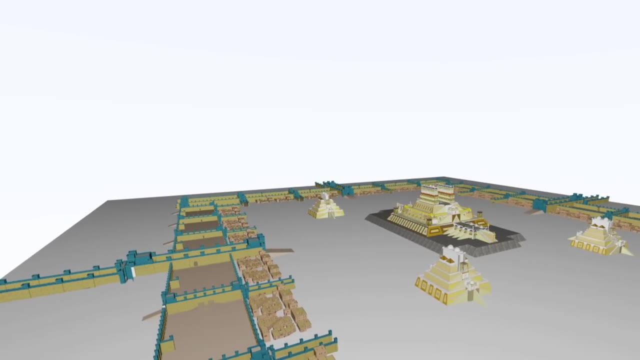 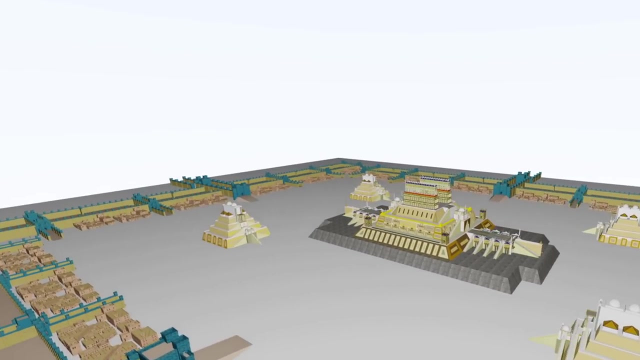 who actually tore down Umma's walls. Umma certainly did suffer devastation and it appears that its development was set back, But, as discussed further below, Umma once again became influential during the third dynasty of Ur. Most of what modern scholars know. 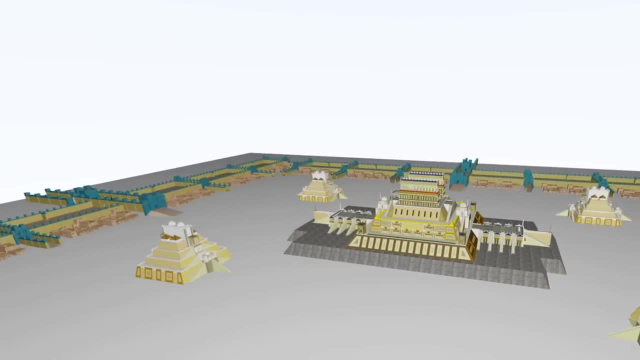 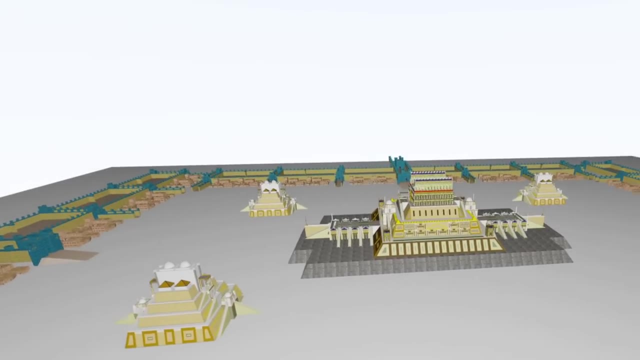 about any ancient culture, at least in terms of primary sources, tends to come from official texts. An official text can be characterized as historiographical in nature, such as the stele of the vultures or the cone of Entenmena. 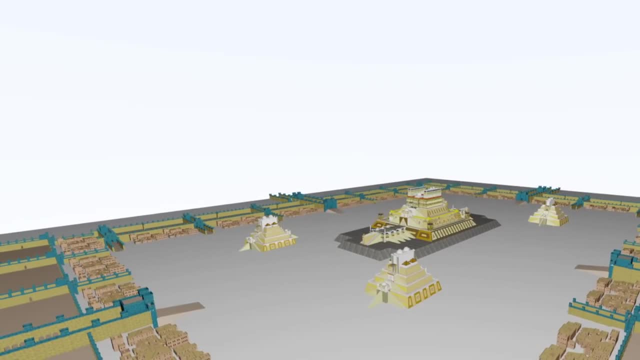 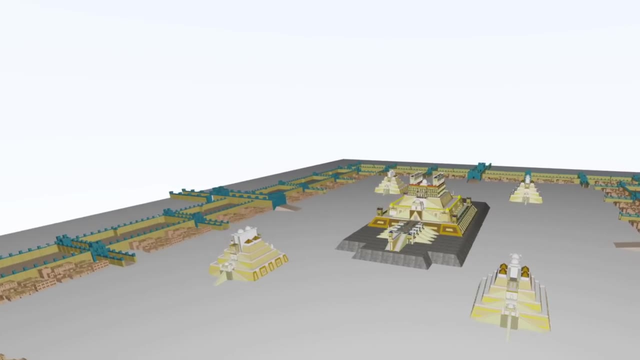 or other inscriptions that relate to it. It can also relate to a ruler's reign, such as an edict, a diplomatic agreement or a royal religious inscription. Of course, some of those examples are religious or mythological in nature, But no matter how they are categorized. 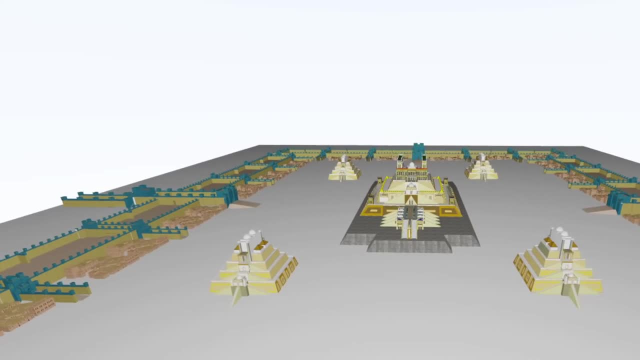 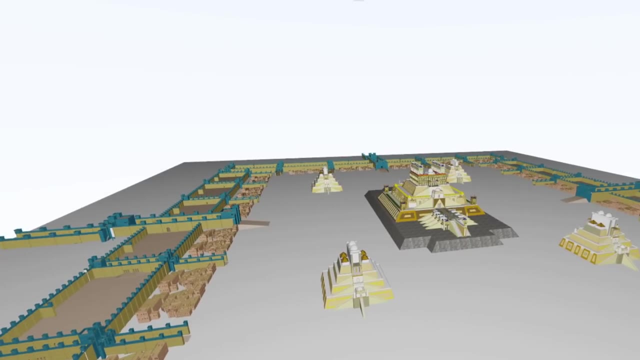 they offer information about ancient culture's political history. It is due to these texts that historians know Umma was a major player in Mesopotamia during the early dynastic period and that its major rival was Lugash, who was the leader of Umma. 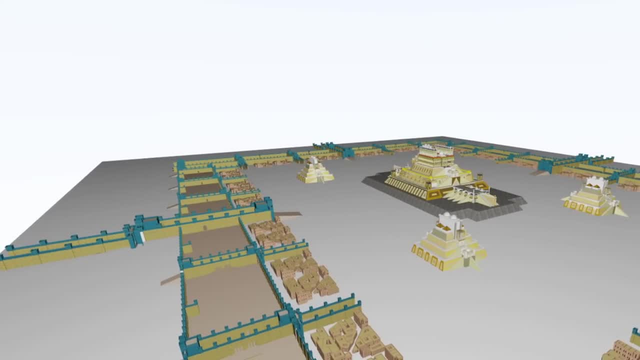 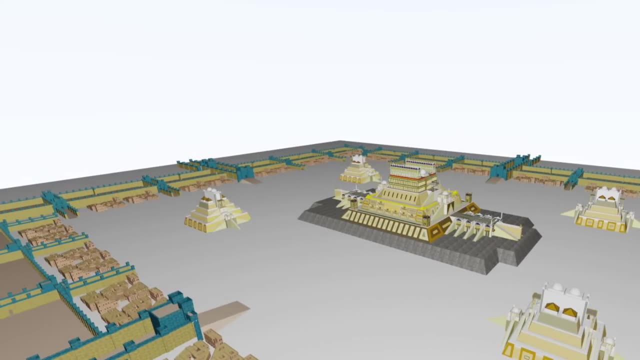 This knowledge helps develop an outline of Umma's history in the early dynastic period, but it only tells part of the story. Most of the people were not directly involved with the geopolitics of the early dynastic period and, although some of the men may have been drafted, 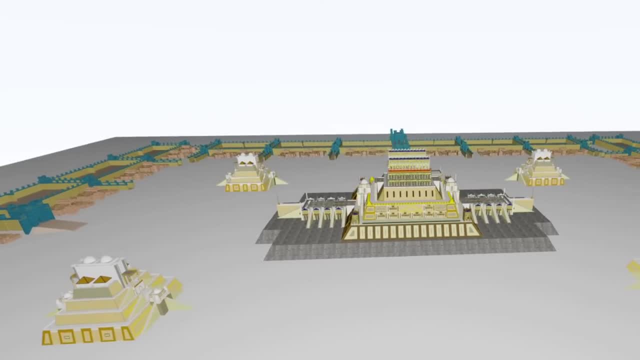 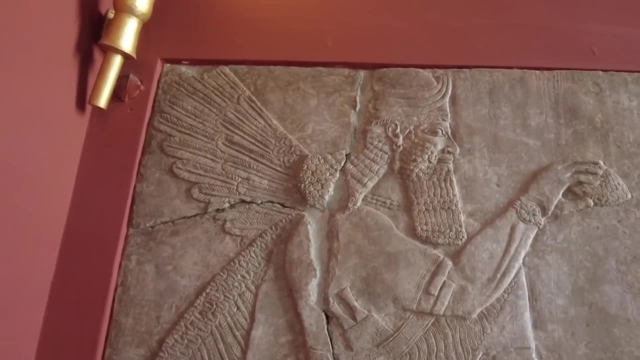 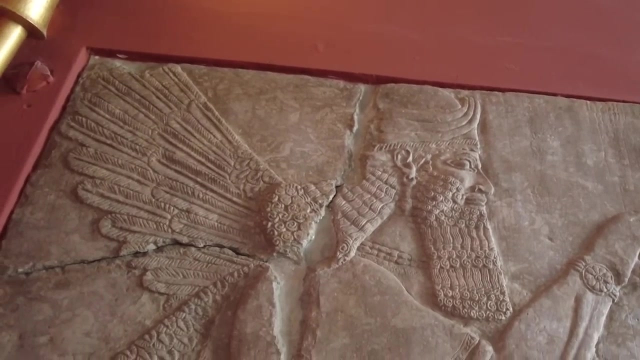 to fight in the wars. the decision was never theirs to make. Fortunately, there were enough literate people in early dynastic Umma that a vague image of life in the city can be painted. Writing began to be used more to record non-official business transactions. 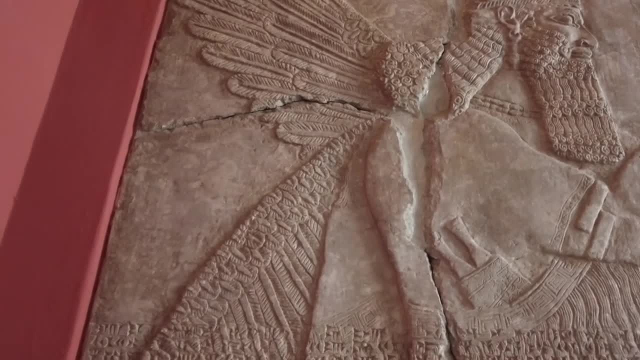 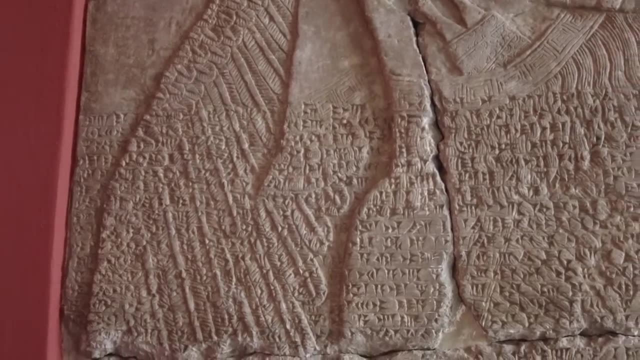 in the early third millennium BCE, And though, in theory, the temples owned all the land in Umma, and in all Mesopotamian cities for that matter, a limited form of ownership was permitted, which allowed a free market to flourish Many of the non-royal inscriptions 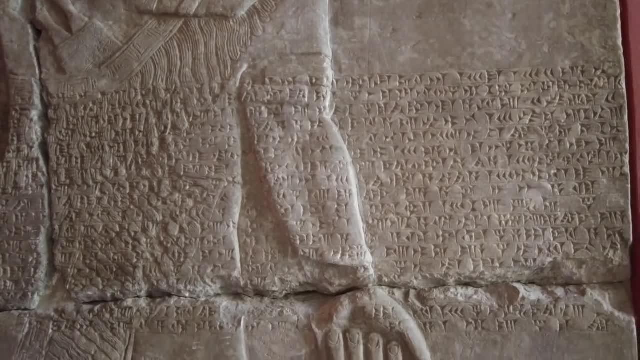 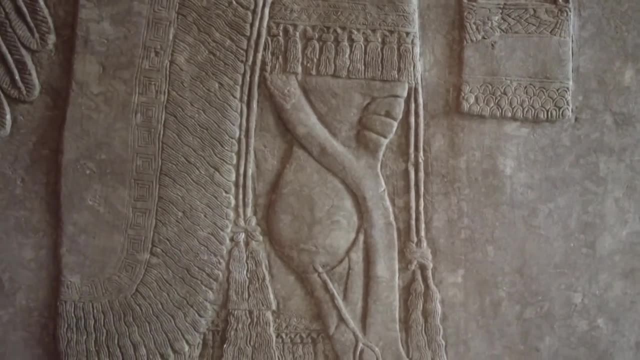 from the early dynastic period record these transactions between private individuals such as the stele of Ushumgal, who was a priest of Shara. The stele of Ushumgal is a gypsum alabaster piece that is over eight inches high. 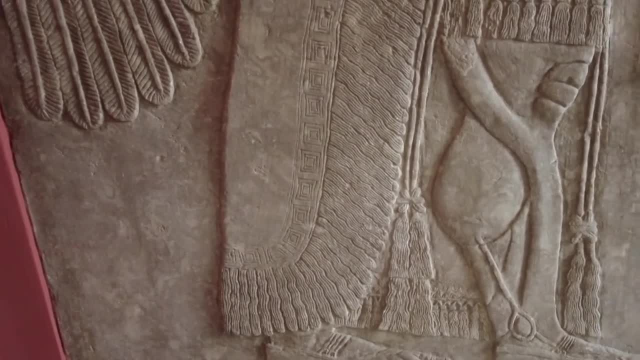 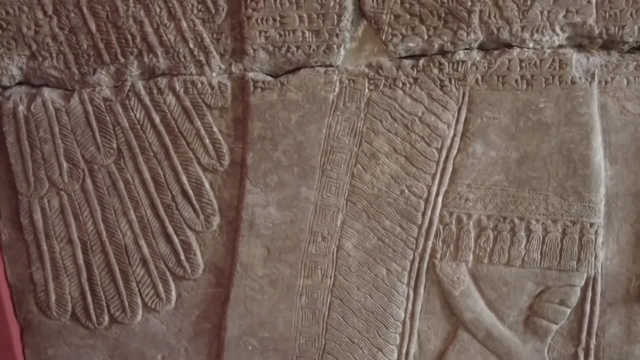 five inches wide and almost four inches deep. The inscription details the sale of three houses, three fields and some livestock, although it does not say who is selling or buying the properties. The accompanying images show Ushumgal and his daughter conducting the sale. 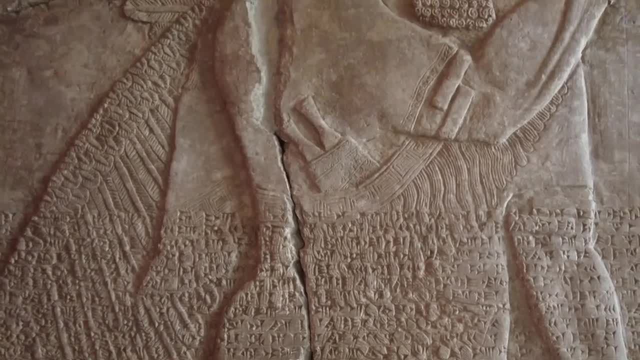 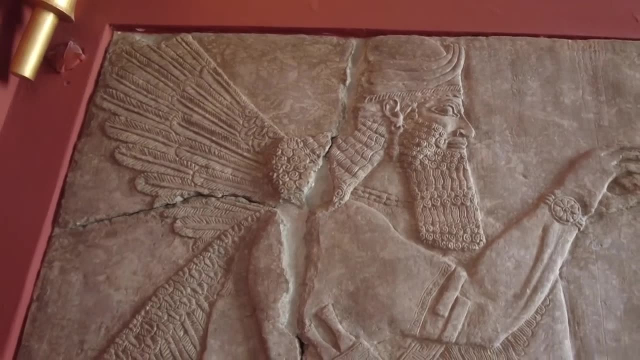 and the fact that Ushumgal's daughter is depicted instead of a son is certainly a point of interest. It could be that he simply did not have a son, but it is notable that he would include his daughter in an important business transaction. 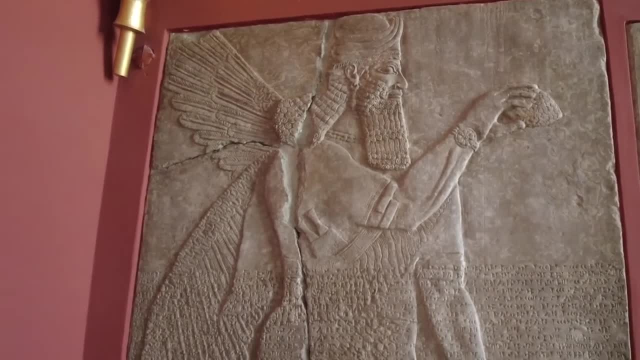 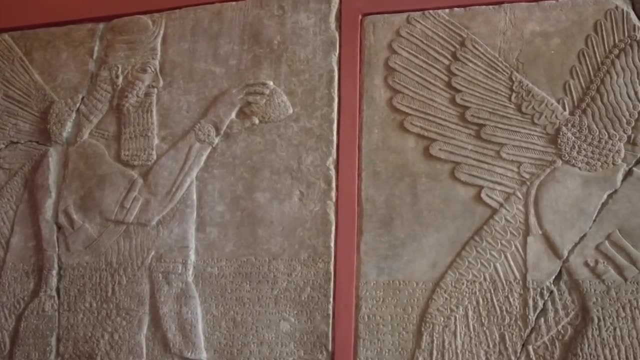 and this may be utilized for further studies on the role of women in the ancient Mesopotamian economy. Since many of the details of the sale are not related and Ushumgal was a priest of Shara, it may be that he was conducting business. 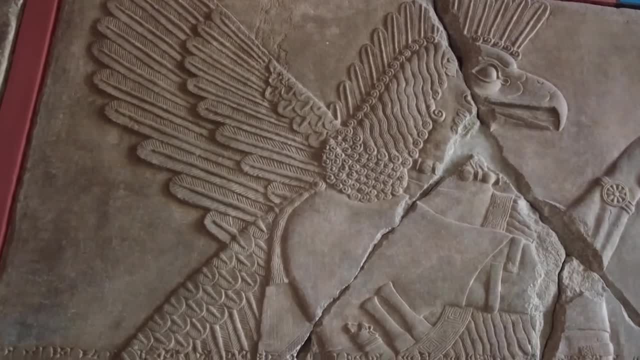 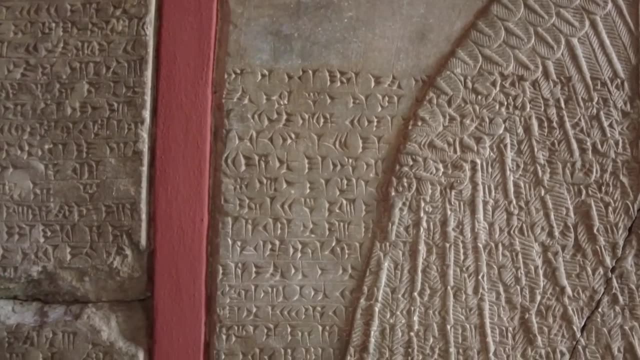 for Umma's Shara temple. Shara was a temple that was not only the patron god of Umma, but also important in the general Sumerian pantheon. Shara was the son of Inanna, the goddess of love and war. 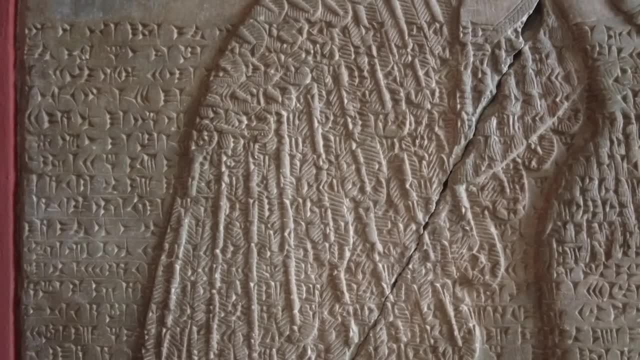 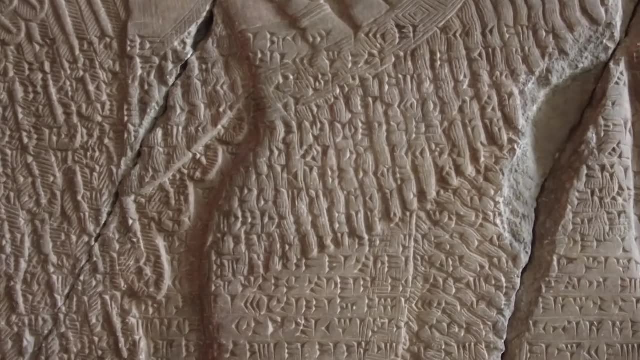 and was often called the firstborn of Ishtar, with Ishtar being the Semitic name of Inanna. Although worship of Shara does not appear to have been widespread outside of Umma, he did play a role in some Sumerian myths. 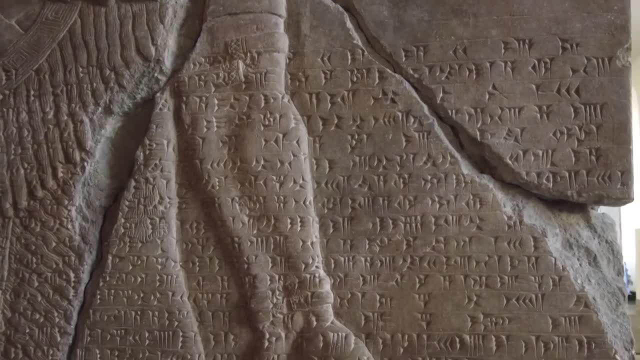 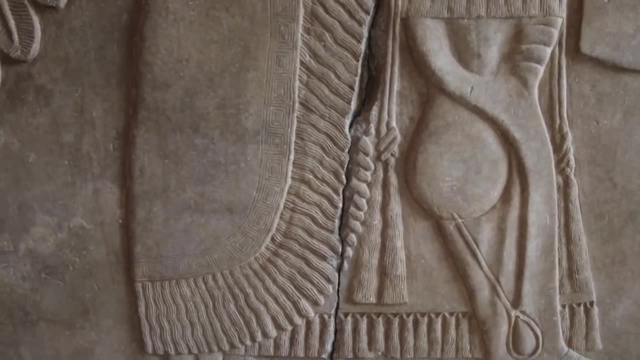 In one particularly interesting myth, Shara of Umma plays a role in the vanquishing of the mythical zoo bird. A later Akkadian version of the myth reads: They called Shara the firstborn of Ishtar. He, who give the orders, addressed him. 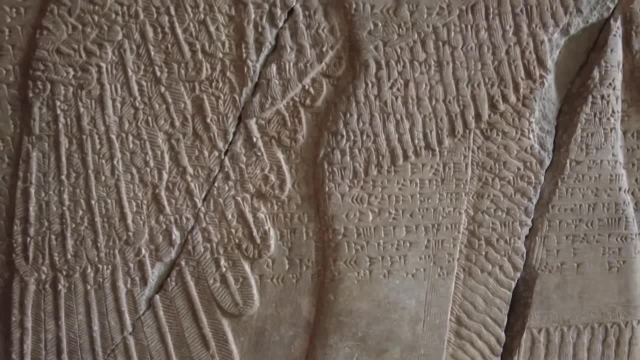 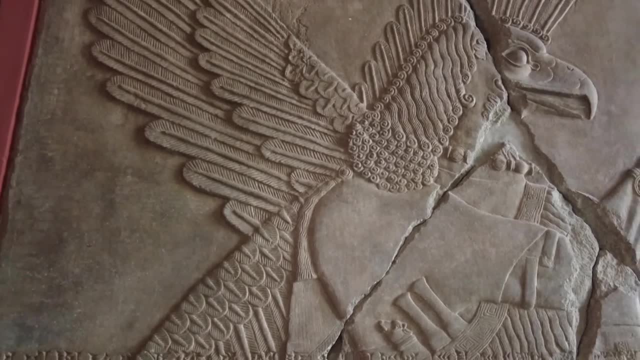 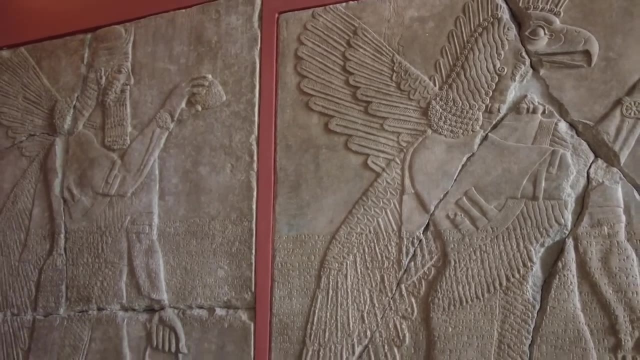 Thou potent one, all conquering Shara, immovable thy onslaught, bring lightning upon zoo with thy weapons. Thy name shall be greatest in the assembly of the great gods. Among the gods, thy brothers, thou shalt have no equal. The zoo bird was depicted in numerous instances of Sumerian art. 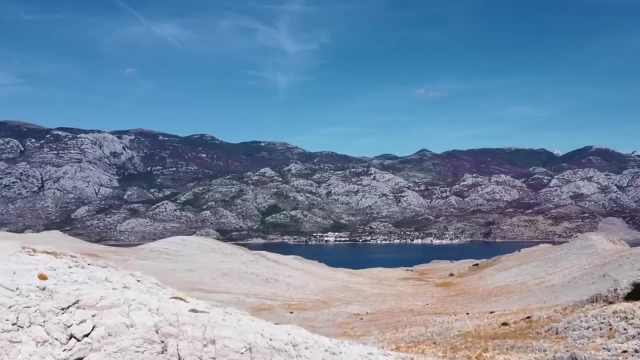 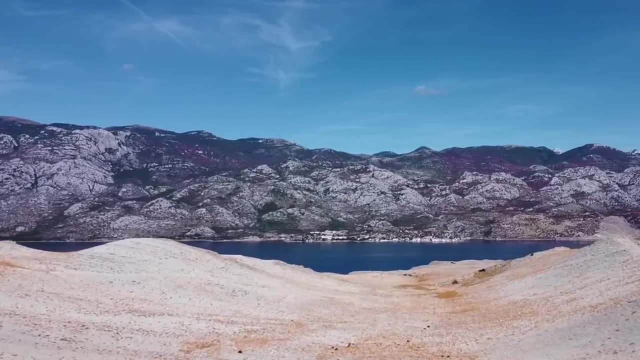 such as the Steed of the Vultures, always as an embodiment of sheer power. In this case, the gods called upon Shara of Umma, with his martial abilities, which were no doubt inherited from his mother, to repel the zoo from the realm of the gods. 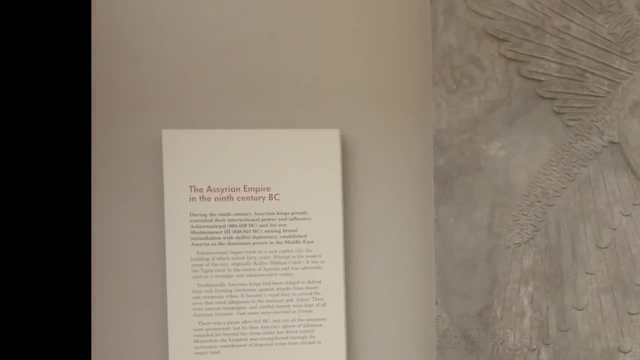 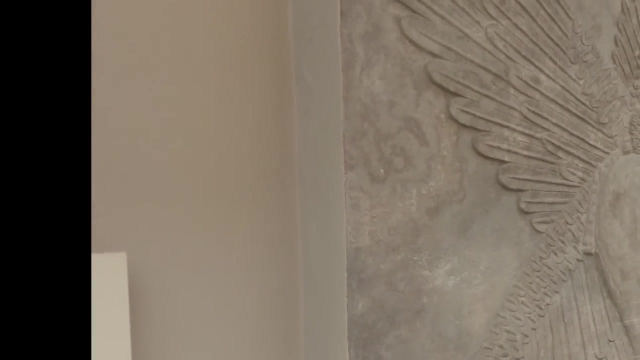 Both Shara and Umma also play a crucial role in another Sumerian myth. The myth often called Inanna's descent to the underworld is a dark tale where, as the title indicates, Inanna visits the land of the dead. 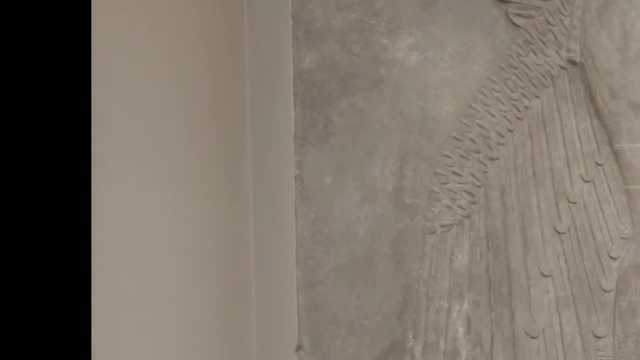 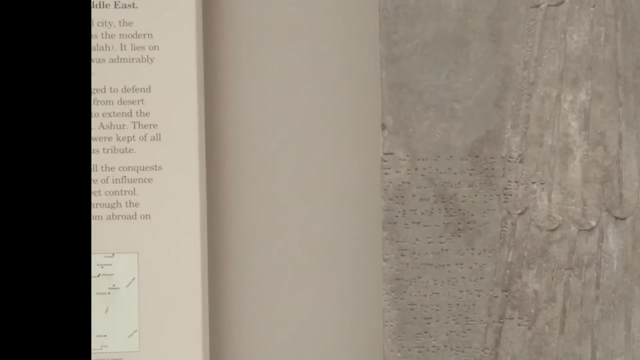 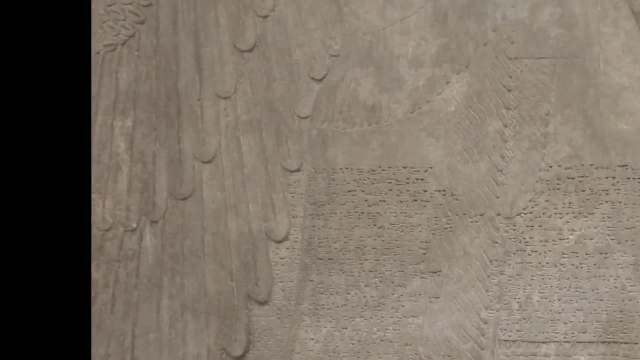 which is the domain of her rival and sister Ereshkigal. The already dark myth takes a macabre turn when Ereshkigal impales Inanna, but she is later revived by the magic of the god Enki. Inanna then returns to Mesopotamia. 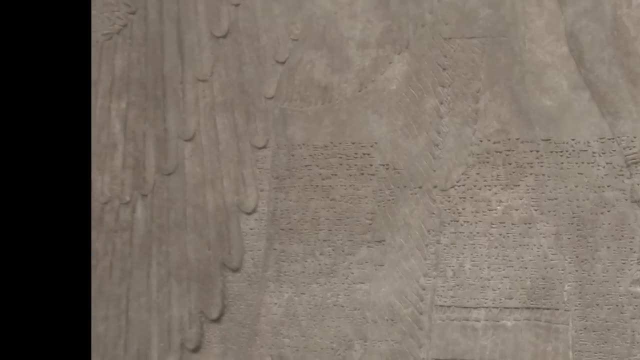 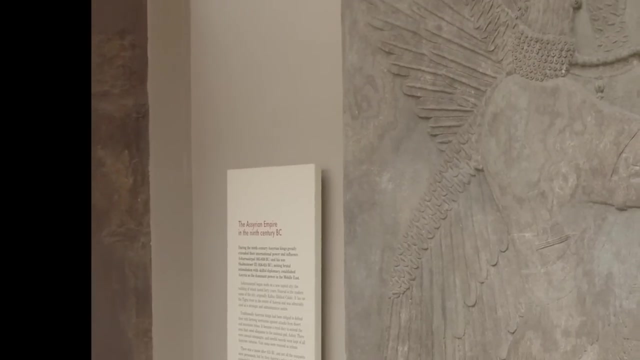 but she is clearly a different goddess because she is now accompanied by demons and other dark spirits as she visits each city and their gods. When Inanna came to Umma, she went straight to Shara's temple, Sigkur Shaga. 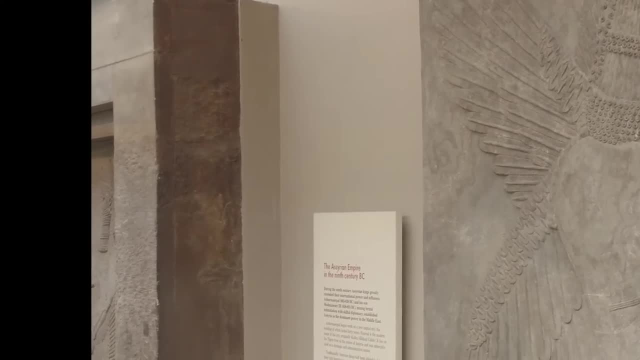 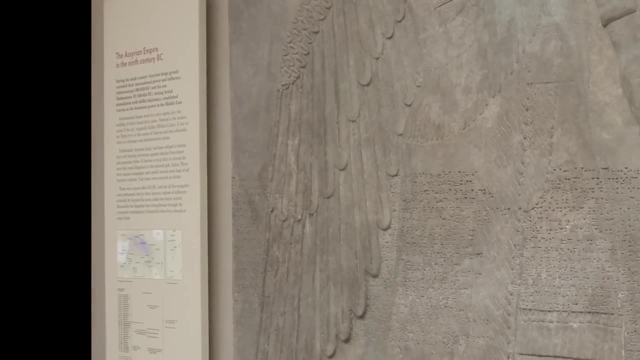 According to the story, Let us accompany her in Umma to the Sigkur Shaga. Let us accompany her In Umma from the Sigkur Shaga. Shara threw himself at her feet, sat in the dust, dressed in sackcloth. 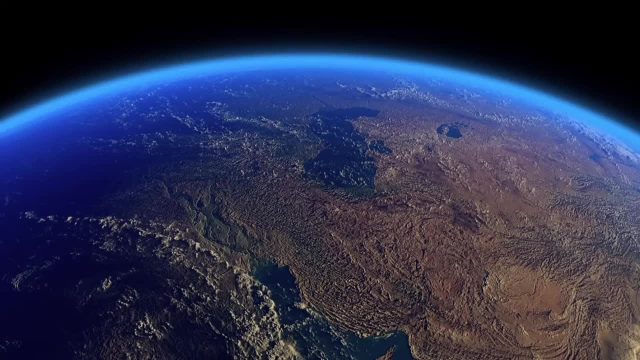 The demons say to the pure Inanna: O Inanna, wait before thy city, Let us carry him, Let us carry him off. It should be pointed out that Umma was not the only city that Inanna and the demons visited, but Umma and its god Shara. 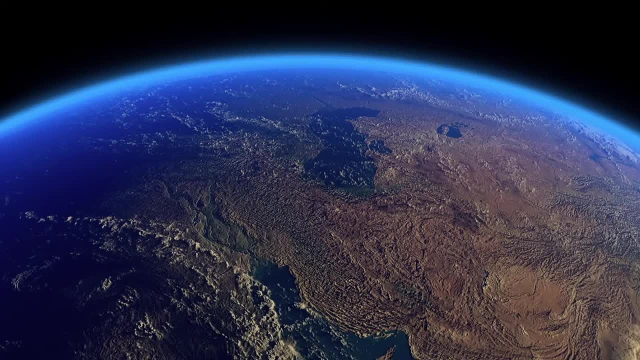 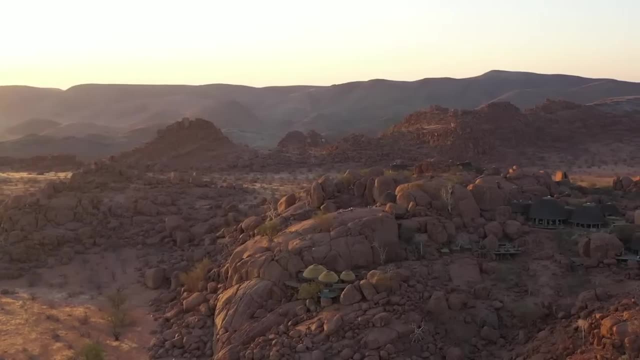 did not help Inanna when she was killed in the underworld, nor did any of the gods of the other cities she visited, so it was clearly meant as a punishment and a warning to people not to turn their backs on Inanna. Other ritual and mythological texts. 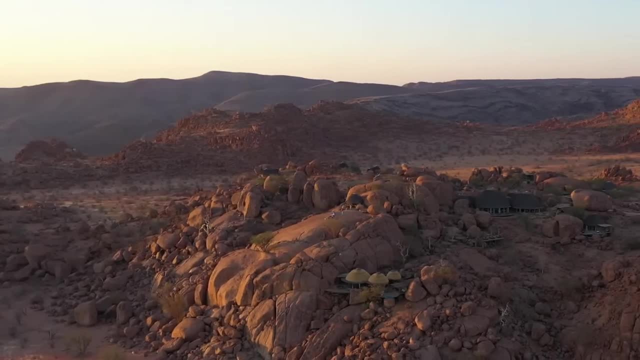 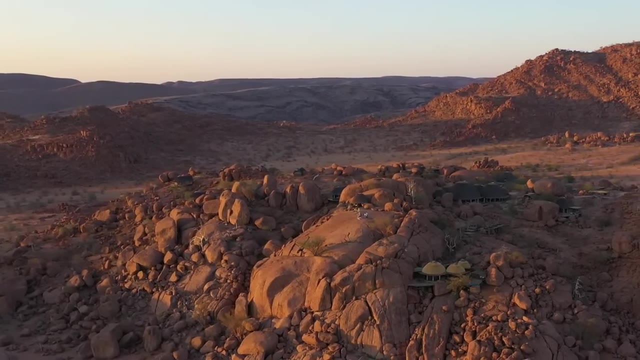 discovered in Umma and other places that relate to Umma indicate that a number of other gods were also worshipped in the city. The people of Umma worshipped Enlil and other gods and goddesses, with Nidabba, the goddess of scribes and grain. 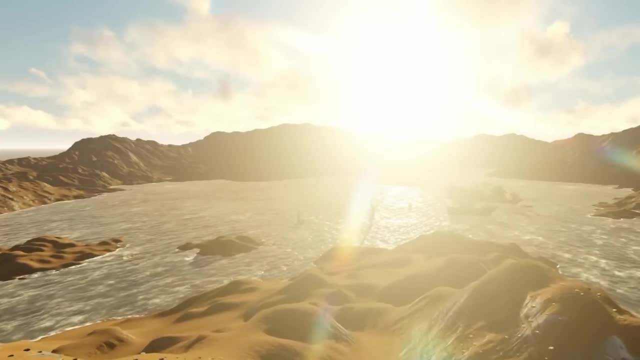 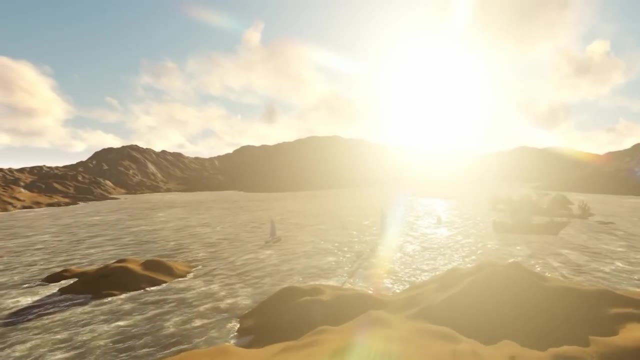 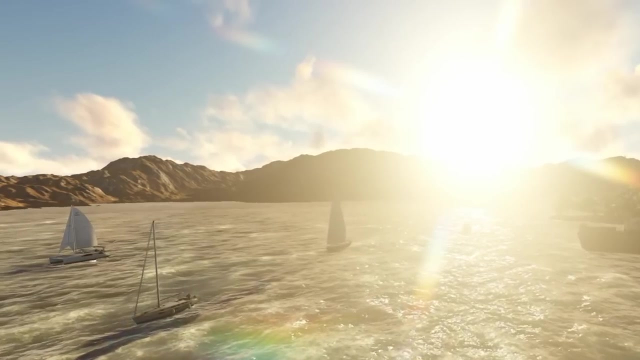 being very popular. It is no surprise that Nidabba was popular in Umma, since agriculture and literature played an important part in early dynastic Umma culture. Clearly, early dynastic Umma had a well-developed literary collection that included royal historiographical 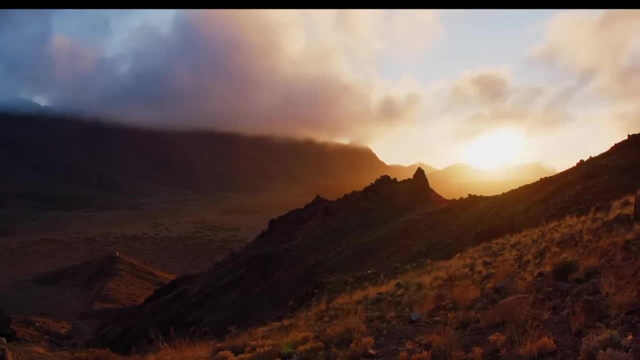 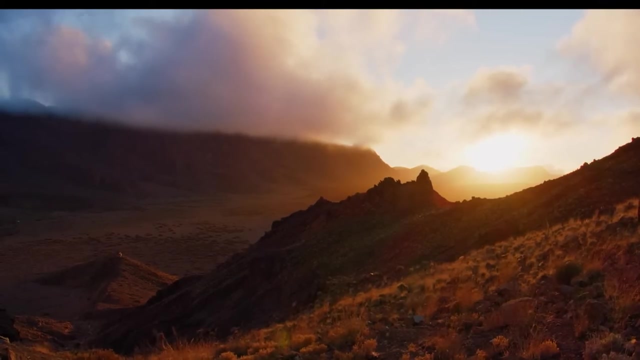 business and mythological texts, But some early examples of fine Sumerian art were also created in Umma during this period. The definition of what constituted art in the ancient world is a bit ambiguous, especially when considered by modern definitions. The people of ancient Mesopotamia. 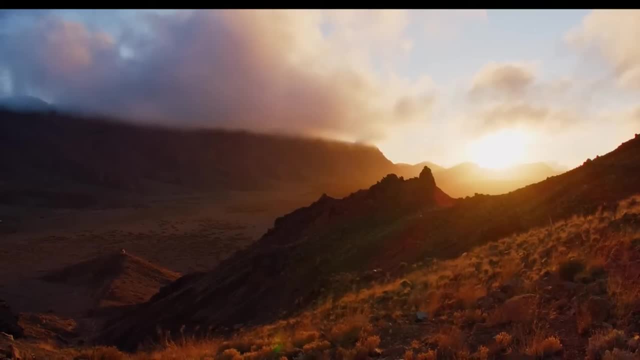 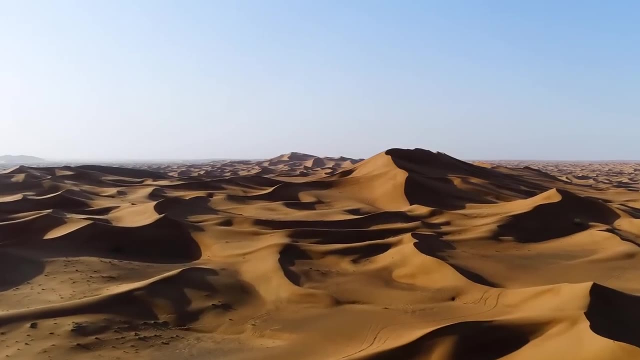 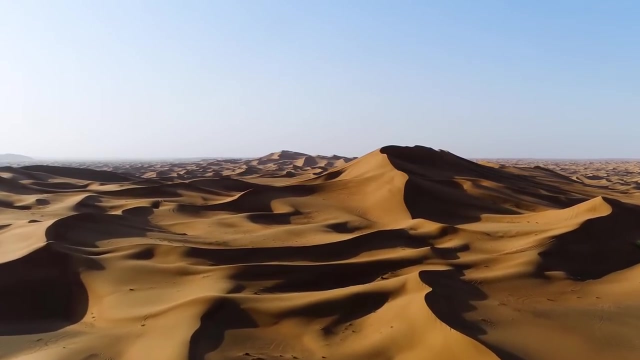 did not create art for the sake of art, as modern people do, and everything they created had a specific function. For example, the stele discussed above were created and offered in a religious or political context. Stele were usually installed in temples and inscriptions. 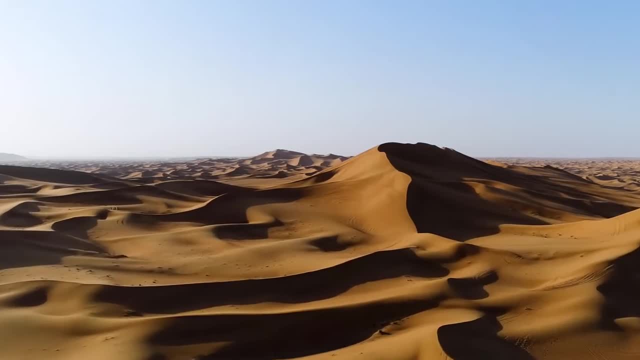 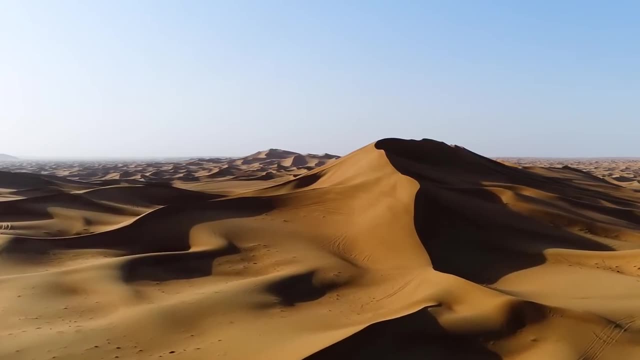 maybe in palaces, but Mesopotamian art was never in the homes of the elites simply for them to enjoy. The art of Umma was either created in a political or religious context, and the two were often intertwined, Of course. modern people, 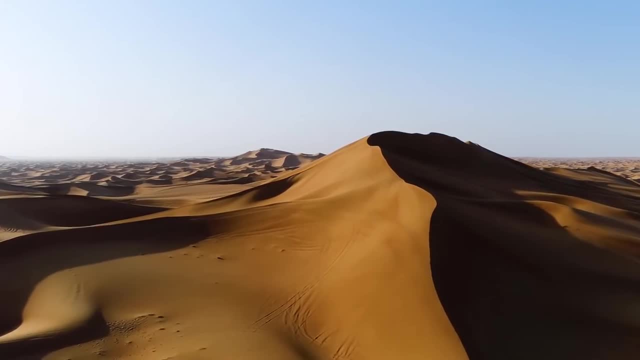 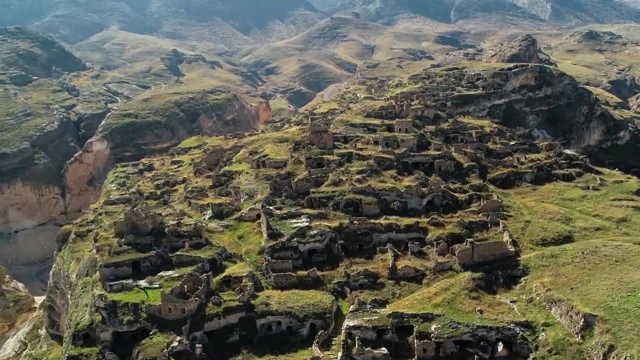 can still consider the stele and other similar objects to be works of art, and many of them are housed in art museums today. For the most part, the art of Umma follows the general Sumerian style found throughout Mesopotamia. 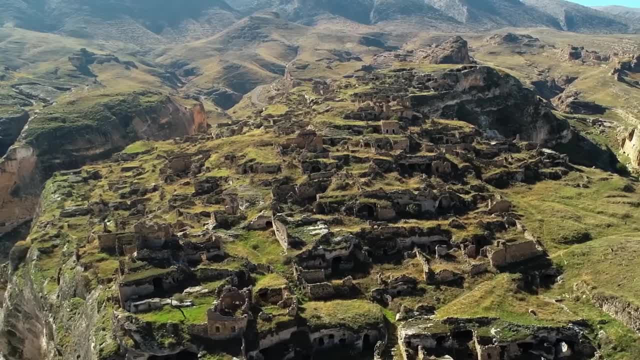 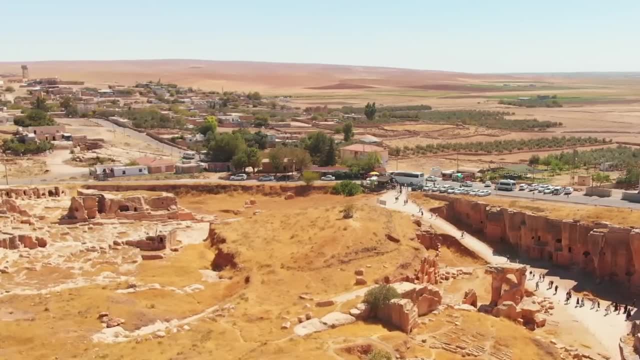 A number of different Sumerian notifs have been identified on figurines and seals excavated at Umma, namely the bull-man figure. The bull-man figure, which was common on royal seals in the early dynastic period, was usually rendered as having the head of a bull. 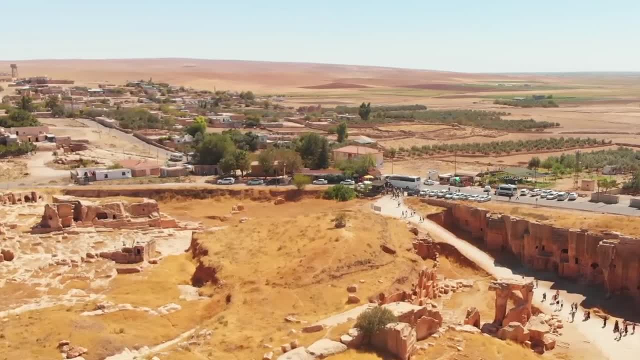 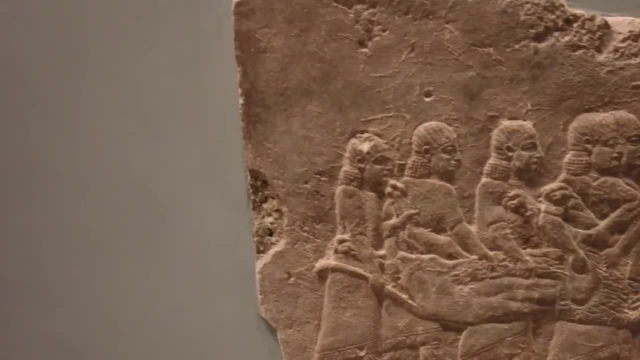 the torso of a man and the legs and tail of a bull. Often, the bull-man was depicted in a semi-heraldic pose, holding off a lion on either side with his arms. A rare sculptural example of the bull-man was discovered in Umma. 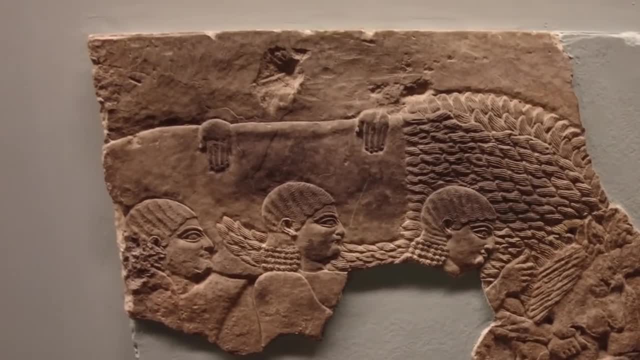 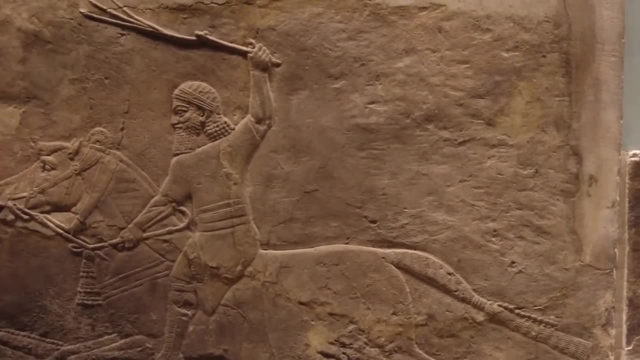 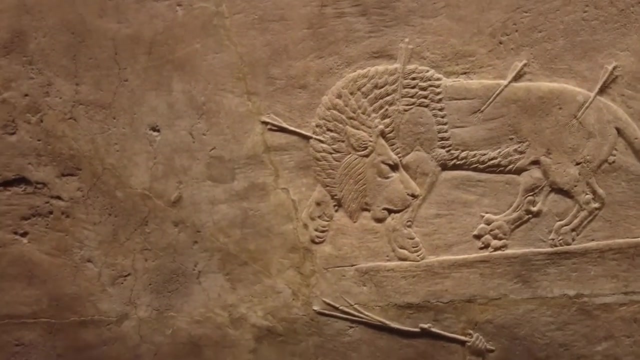 The tall, slender bull-man sculpture was made of green serpentine and is believed to represent a demon, although the precise iconography remains a mystery. It could be that the bull-man represents one of the demons who accompanied Inanna when she returned from the underworld and visited Umma. 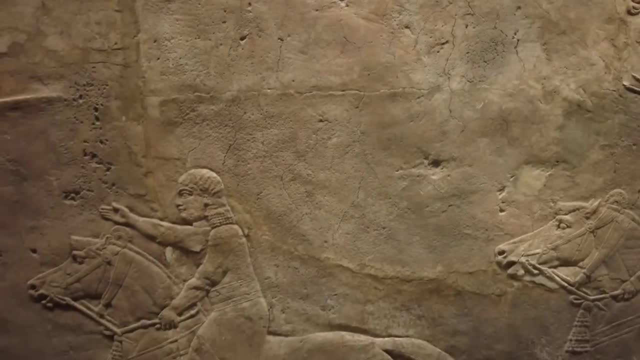 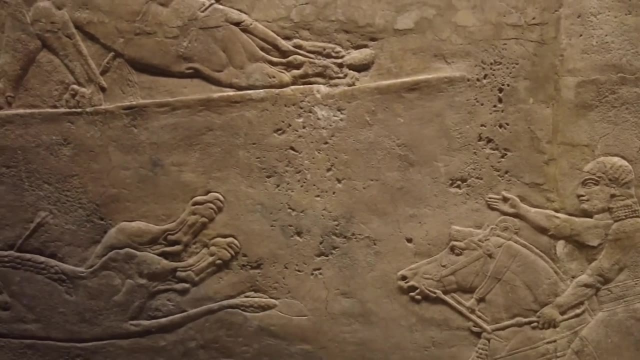 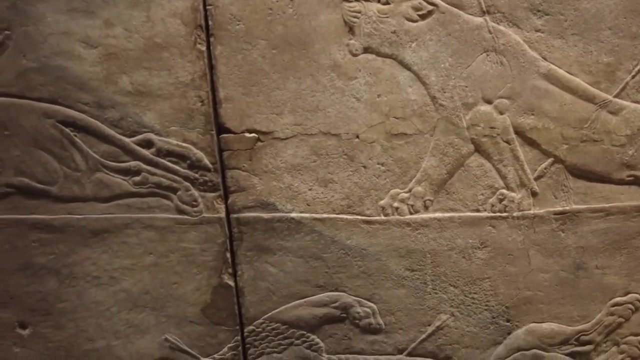 and some of the other Sumerian cities, but this remains unclear. The general lack of texts from Umma in the early dynastic period creates a certain degree of mystery and endless questions Once the third dynasty of Ur, or the Ur III dynasty, came to power. 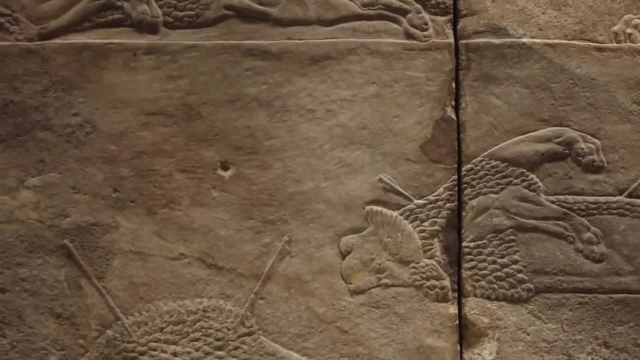 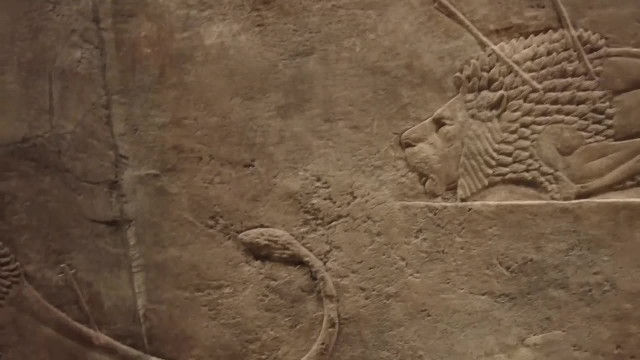 more written records were created, leading to a clearer image of life in Umma. The Akkadian dynasty ruled most of Mesopotamia firmly until a period of confusion took place after the rule of Sharkalishari, 2217-2193 BCE. 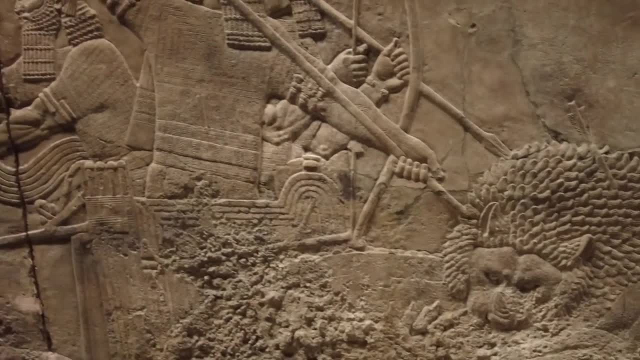 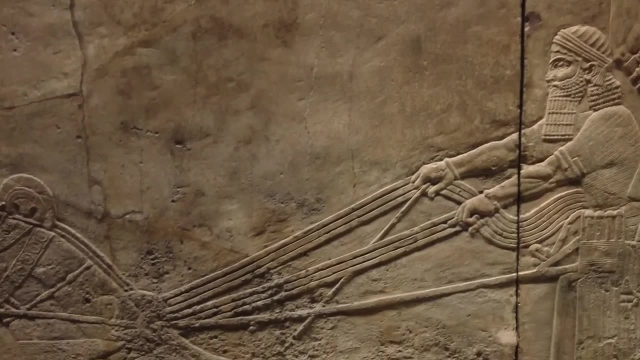 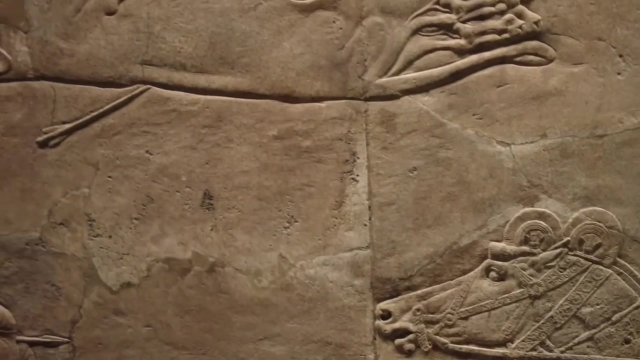 The Akkadian dynasty limped forward through the reign of Shuturu, 2168-2154 BCE, until it totally collapsed. Mesopotamia then entered into a brief political interregnum, but it did not last very long, since the idea of regional states 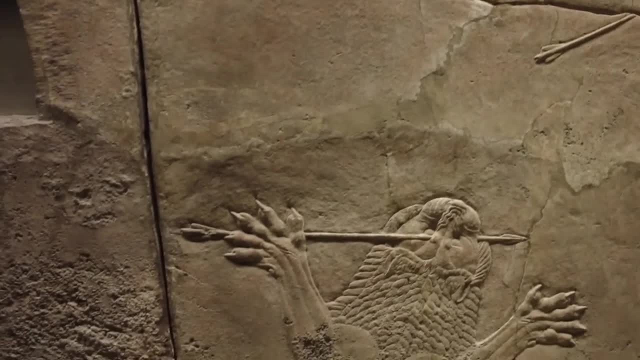 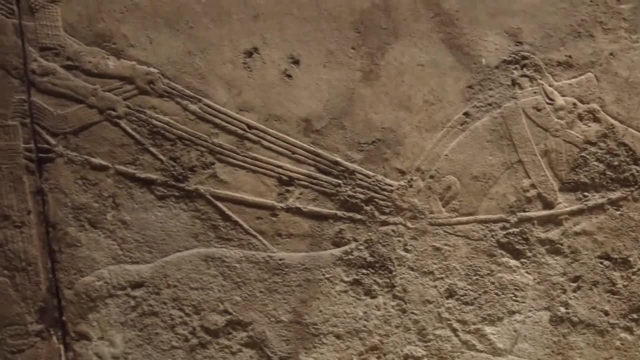 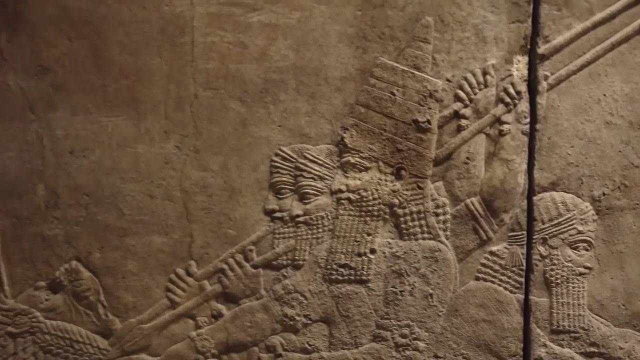 had already been established in the late, early dynastic period. Once Akkadian rule was over the Akkadian dynasty, the early old city-states of Sumer realigned and Sumerian cultural dominance was quickly reestablished around the city of Ur, which became the capital. 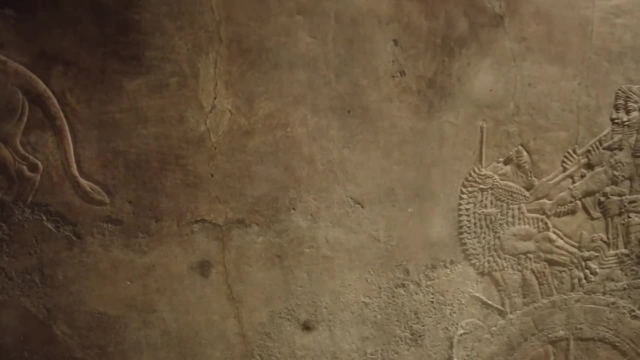 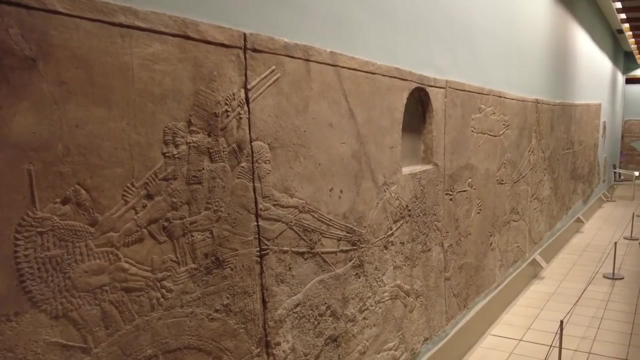 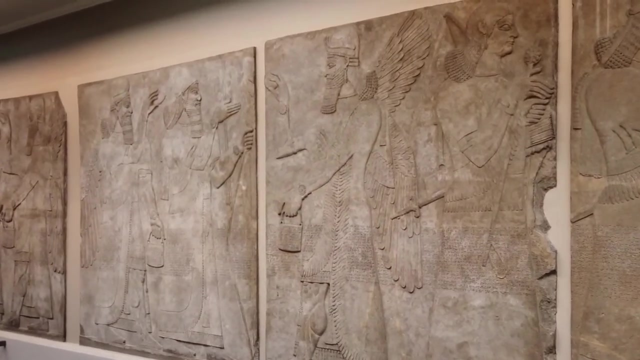 of the Ur III dynasty. After the Semitic language of Akkadian briefly enjoyed primacy in written materials under the Akkadian, Sumerian made a comeback during the Ur III dynasty. The first king of the dynasty was Umar. Once again Umar. 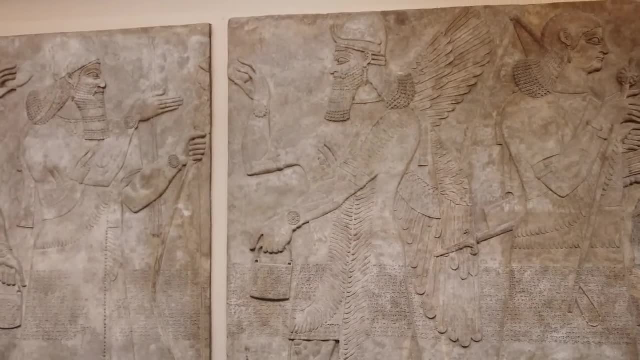 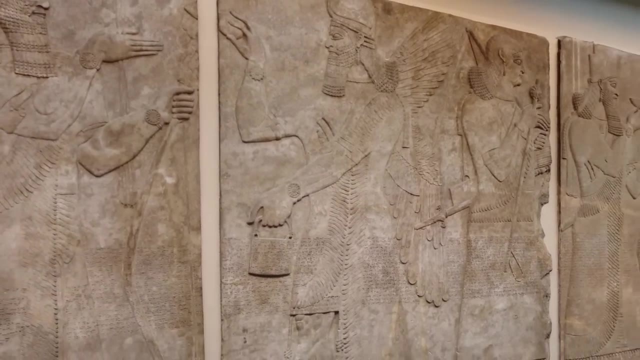 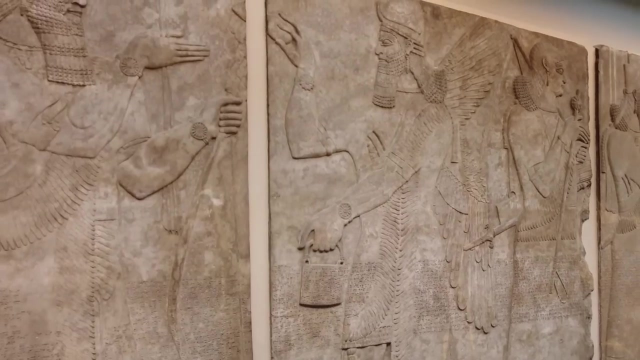 and the other cities of Sumer played a vital role in the cultural development of the region. Although the number of written texts greatly increased during the Ur III dynasty, of which many concerned Umar, very few of the documents relating to Umar were political in nature. The Ur III dynasty empire was fairly centralized in the period between 2094 to 2047 BCE, when the Ur III state began integrating other Mesopotamian cities into its empire through conquest. Chulgi and his successors then immediately went to work to ensure that they could. 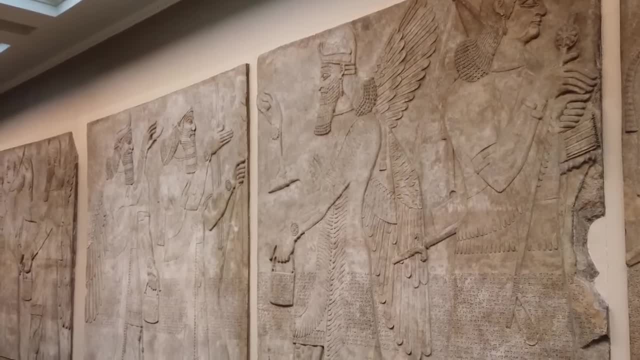 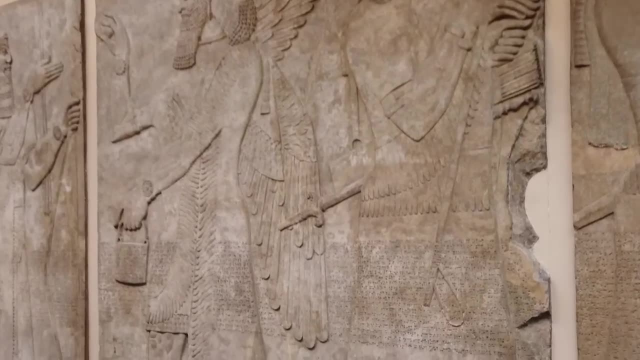 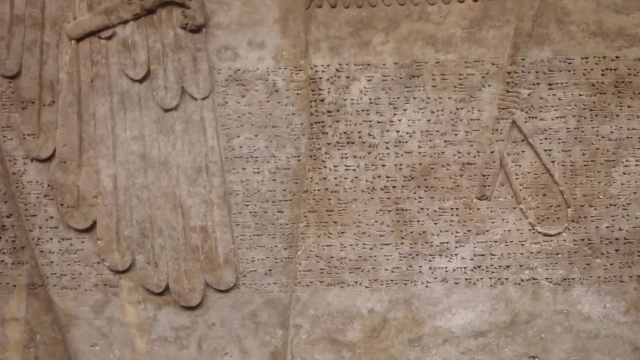 control their vast new empire by installing their own encis in each major city, which included even larger rural areas than in the Ur III dynasty. Each city-state also had at least one general, although some had multiple. Buma maintained its status as a first-rate city. 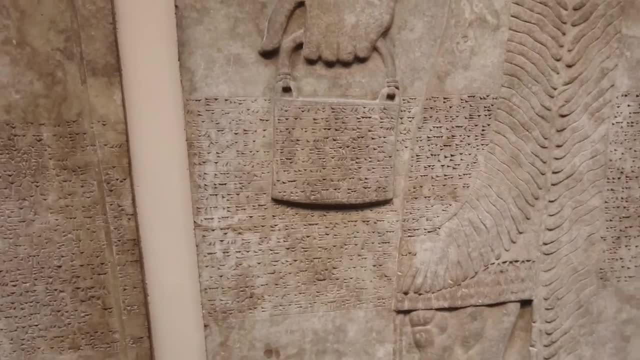 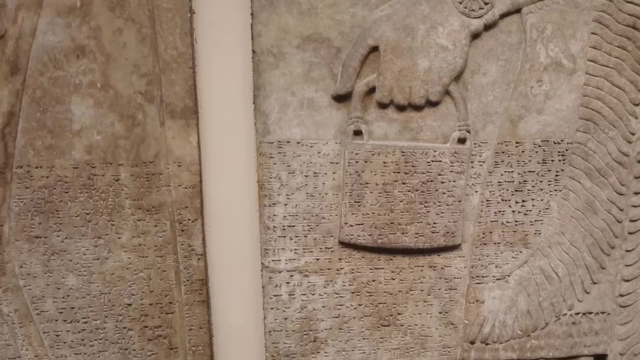 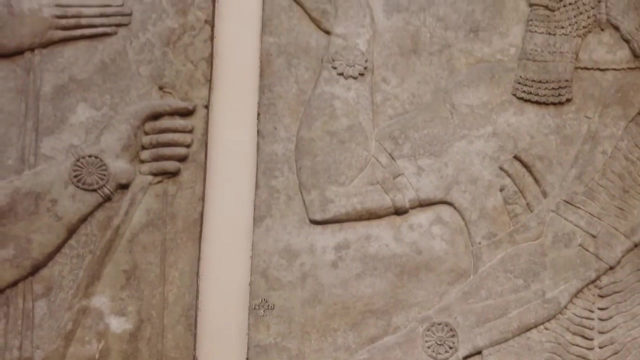 under the Ur III dynasty. so it was given a governor, slash ensi, but several generals also patrolled and were garrisoned in the district slash province. The extra generals may indicate that the old wars between the city-states would not be renewed under their watch. 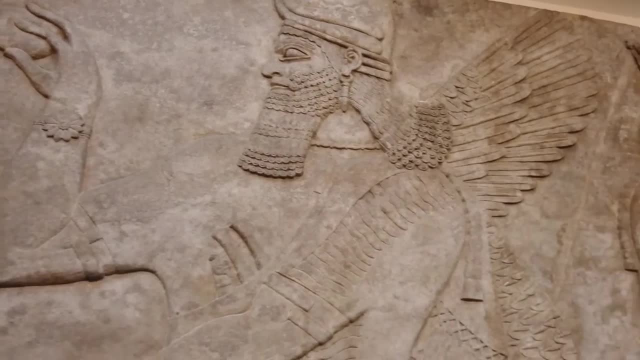 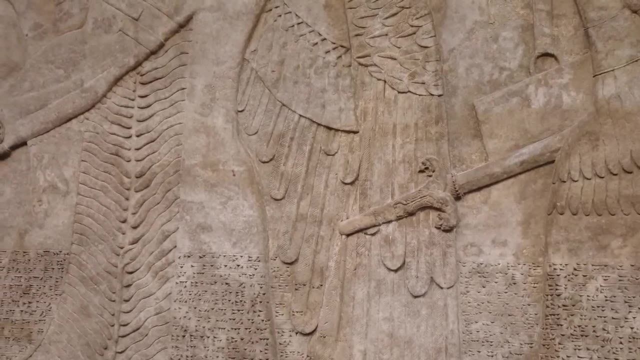 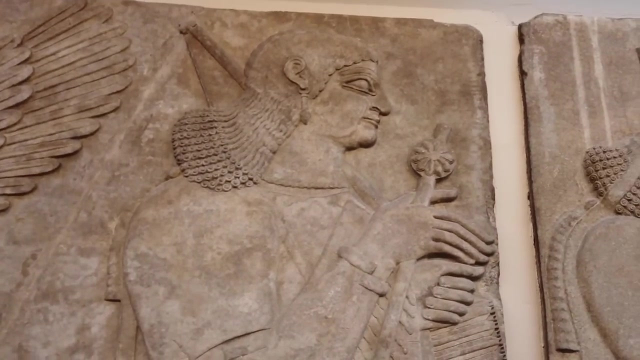 Based on the available primary source evidence, though, it appears that Uma's true importance during the Ur III dynasty was economic, not political. Thousands of Sumerian cuneiform tablets discovered by archaeologists at Uma have revealed that there are more than 19,000 tablets believed. 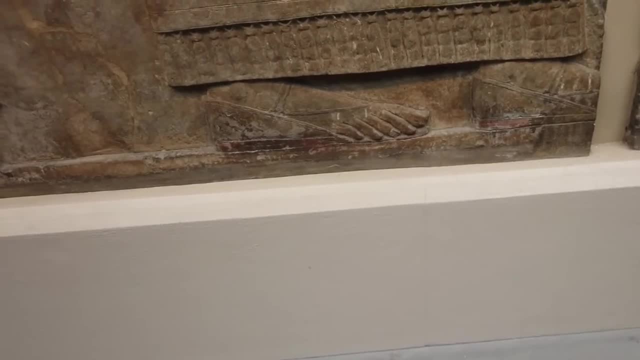 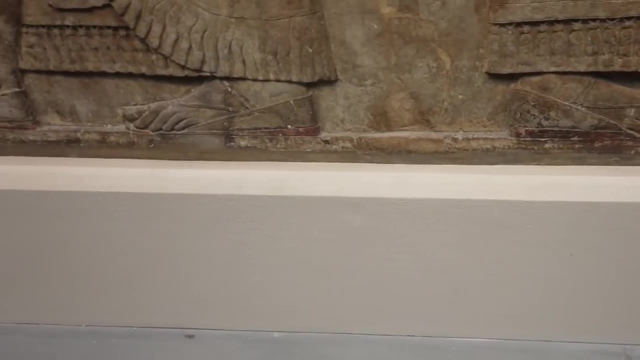 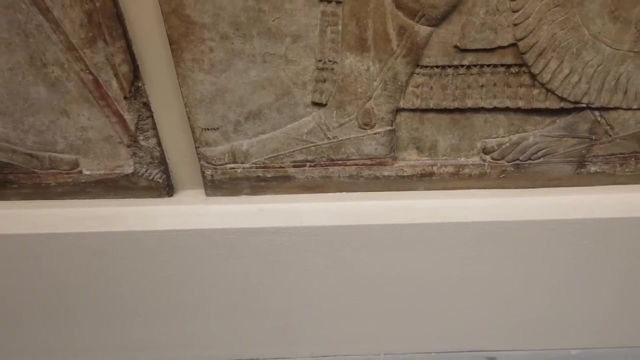 to have originated in Uma, which help modern scholars determine much about the manner of trade, what was traded and who was allowed to trade. The documents show that, although trade was highly centralized and overseen by the rulers in Ur, it was carried out by independent contractors. 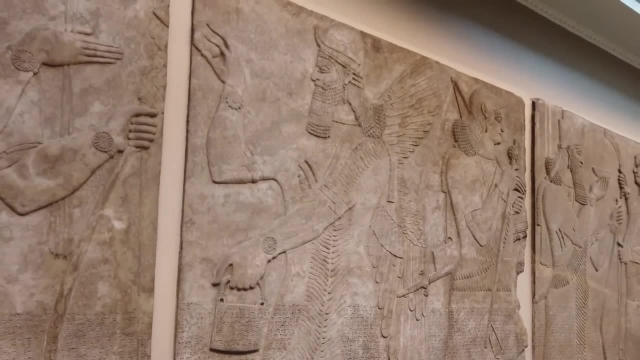 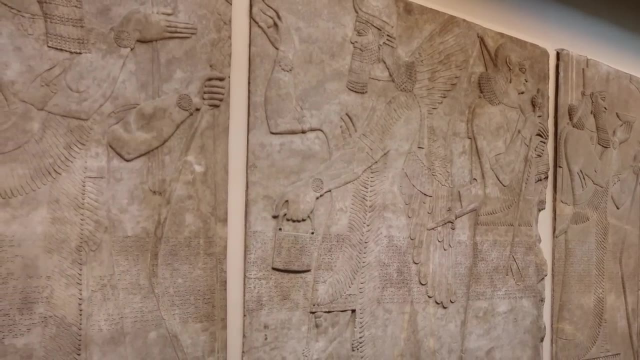 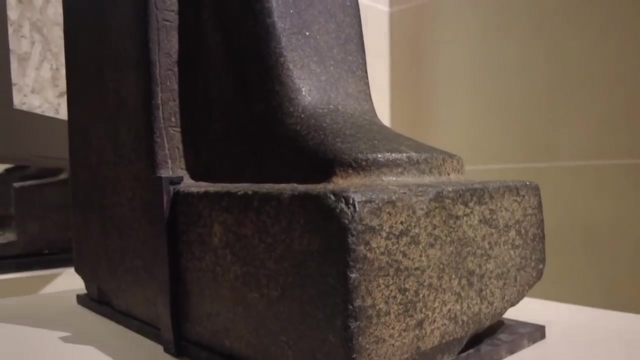 which, in the case of the documents in question, were the Ur of Islam. with goods coming in directly over trade routes to the Zagros mountains, to the east, Arabia in the west and the Levant in the northwest, Secondary trade routes brought other goods into Mesopotamia. 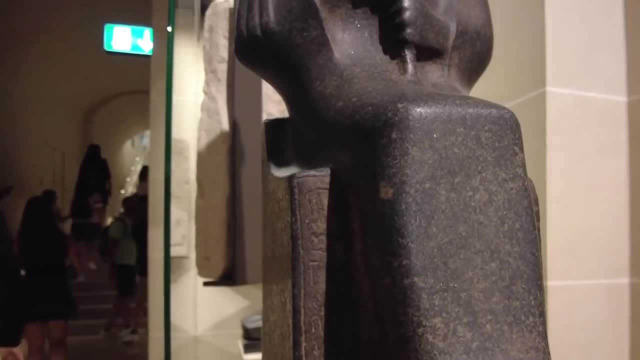 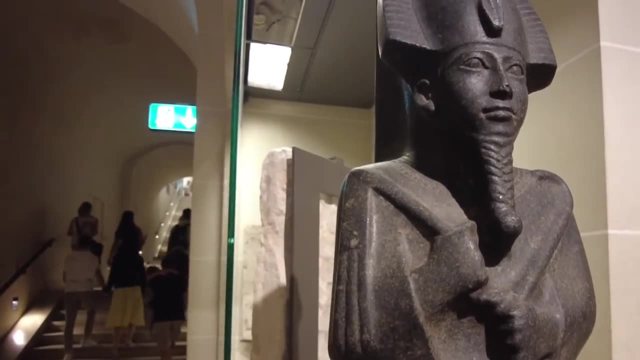 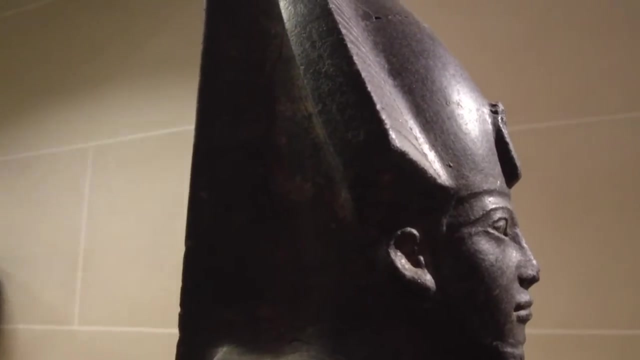 from as far as Egypt and Afghanistan. The documents also show that, although the Uma merchants were, for the most part, free of Ur's control and not micromanaged, they were connected to the Ensi, or the temples in Sonwe. These merchants were required to give part of 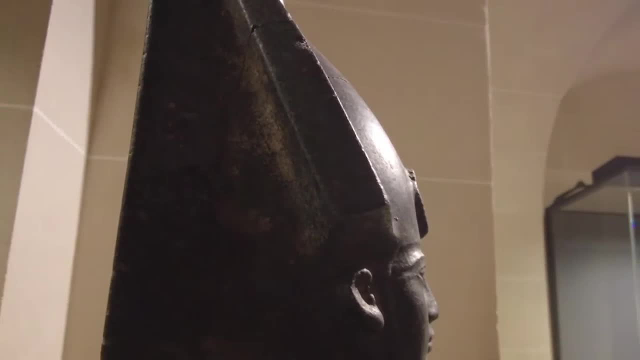 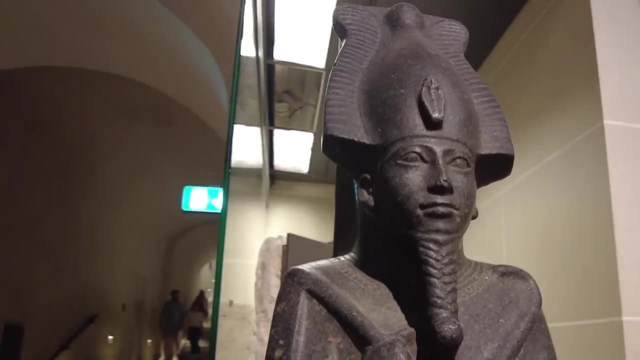 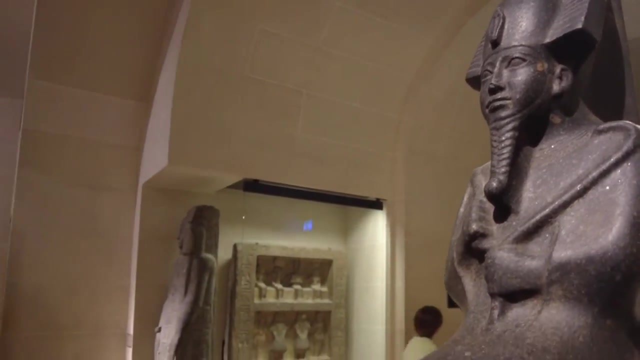 their profits to them and would also receive capital from them. A percentage of the materials acquired would be used for the upkeep of temples. Food, bitumen, gypsum and other materials used in rituals, for instance, would be earmarked for particular temples. The tablets show that the amounts 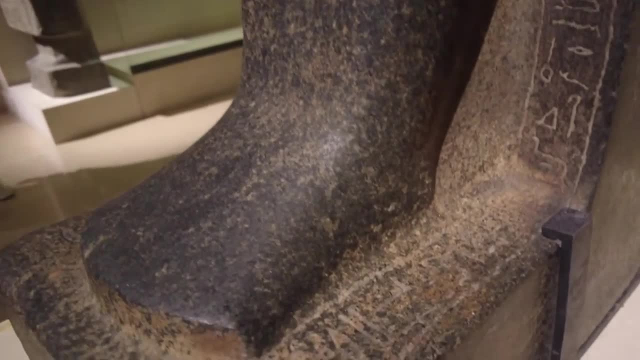 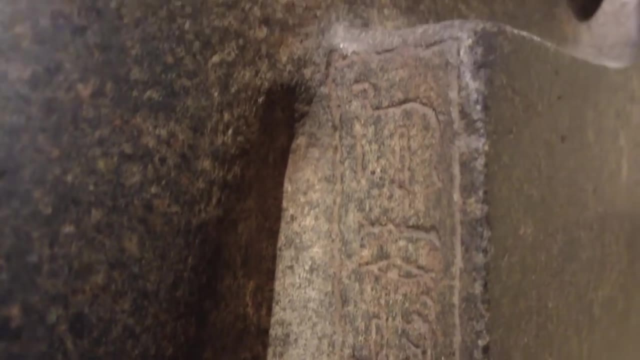 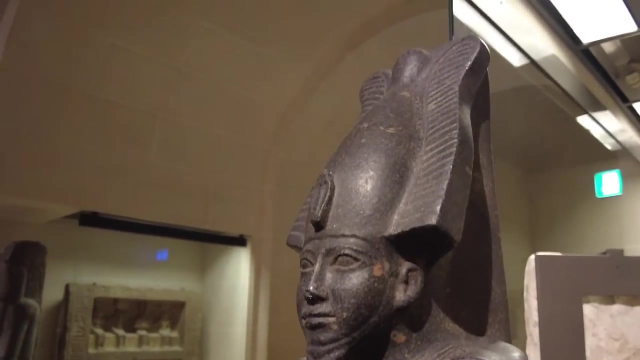 were well documented, as well as the method used as a standard of value. Perhaps the most fascinating aspect is that silver was used as a trading standard. The Uma merchants did not use silver as cash in coins the way the Lydians would much later, or the way coins are used today. 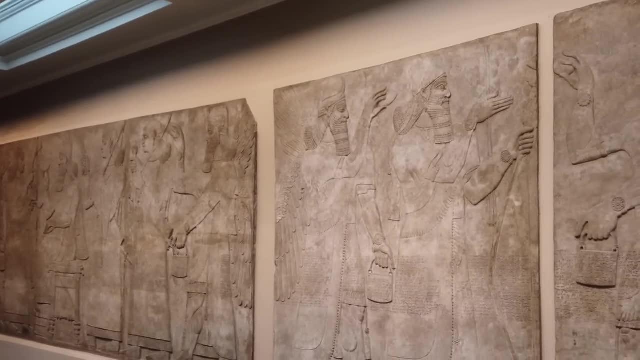 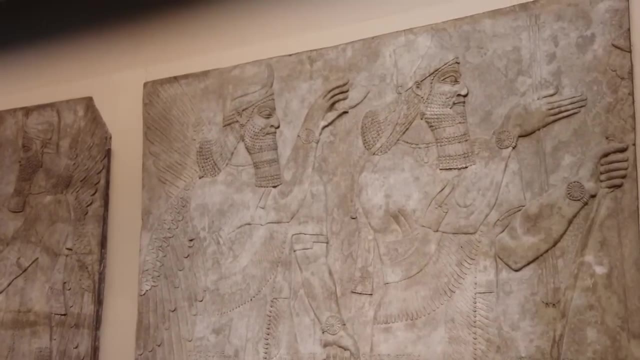 but they did use it as a store of value and the money of account, In other words, everything the Uma merchants traded had a value and the value was based on the weight of silver. Most of the empire's silver stores were held in Ur, but merchants 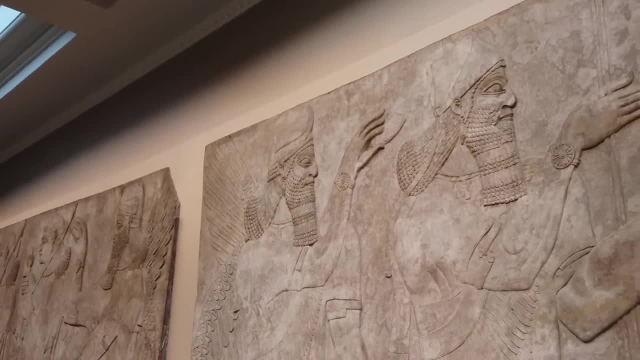 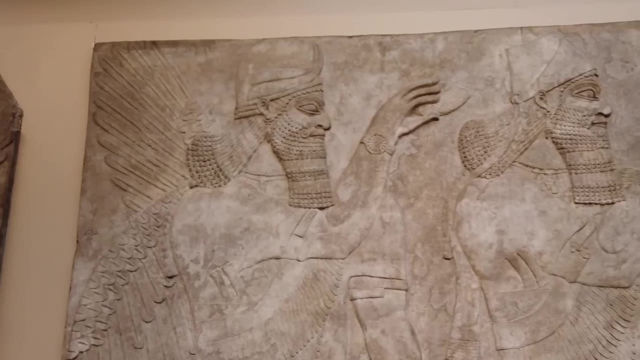 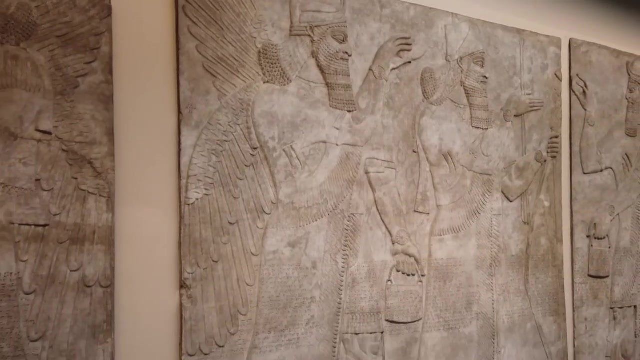 could buy supplies from the government and use this capital to fund their operations. The silver could then be used to trade with other merchants, especially foreign ones. The value of silver would fluctuate, the same as it does today, depending on demand, with scarcities leading to greater demand. 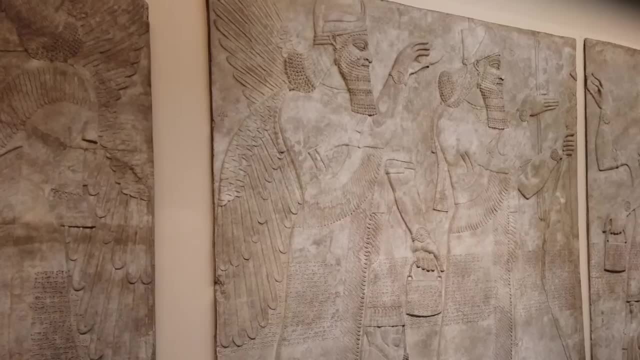 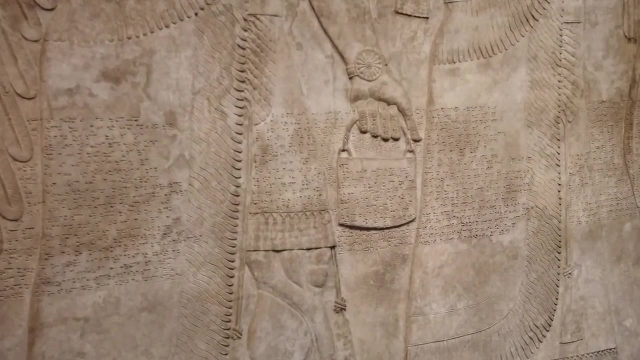 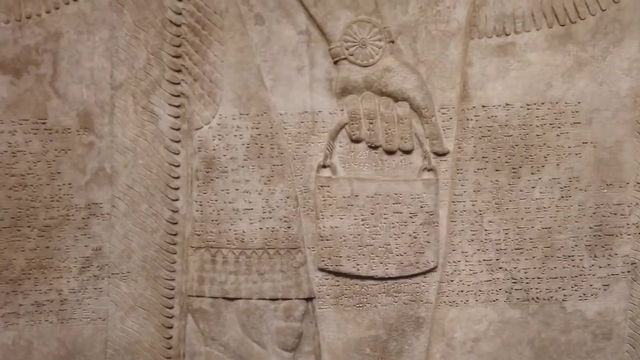 which in turn would lower the price of commodities. Conversely, just as with today's economy, a surplus of silver could lead to inflation and higher prices. Trading in the local market of Uma was usually silver free. It was a commodity for commodity, with the trade prices based on. 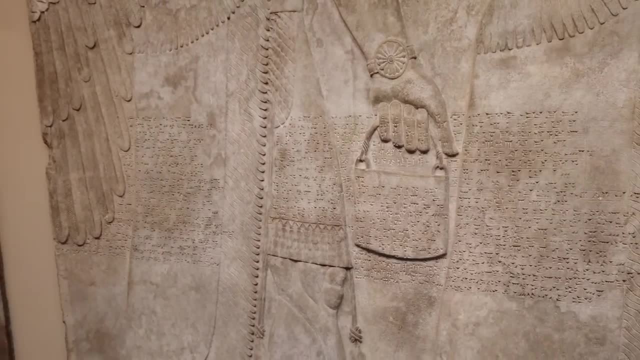 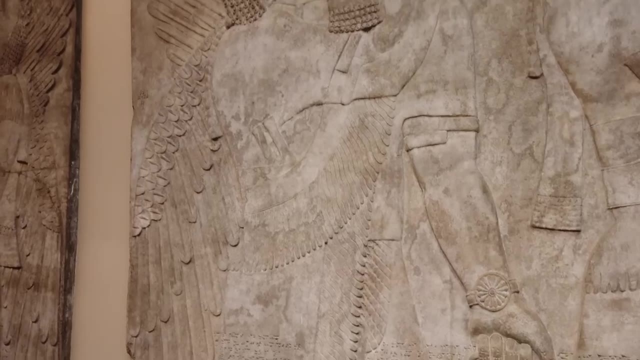 the current value of silver. This was actually quite an incredible step forward in terms of macroeconomics Before this period. barter was usually fairly simple and for the most part, involved haggling on each transaction, but the use of silver as a standard. 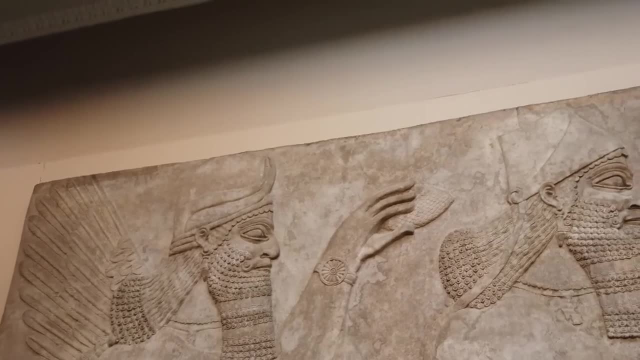 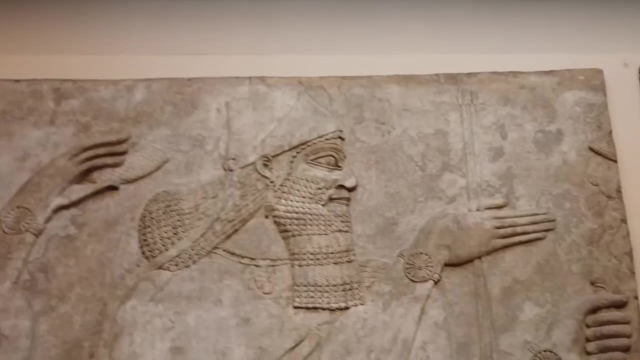 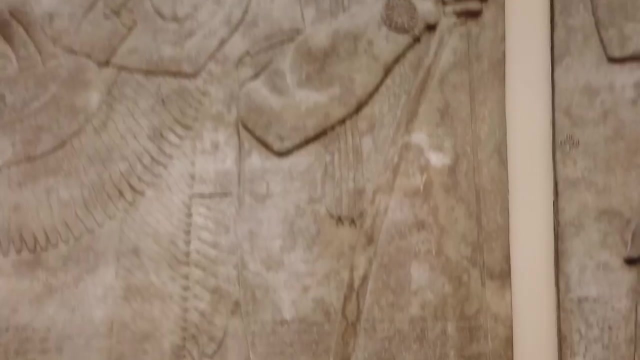 allowed larger and foreign transactions to take place. This type of trading was only possible with a well regulated system. The system that the Uma merchants took part in was overseen by the Comptroller who was assigned by the Ur3 Royal House. The Comptroller basically functioned. 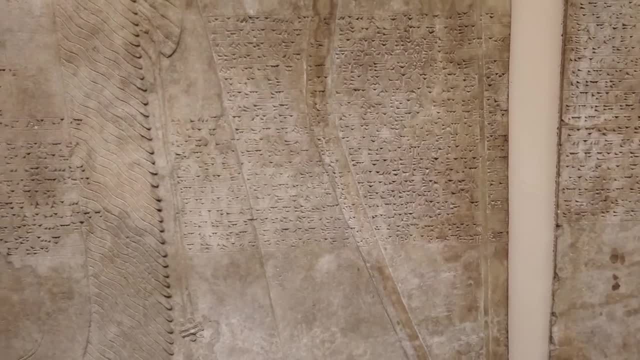 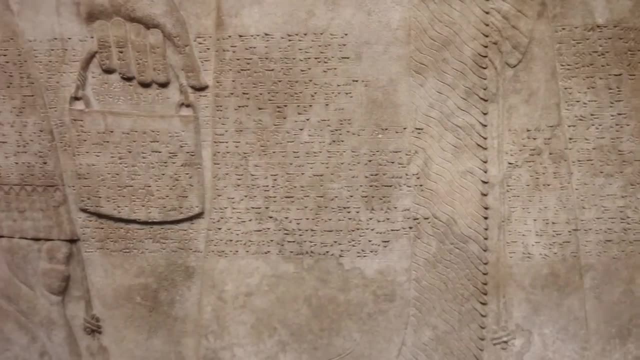 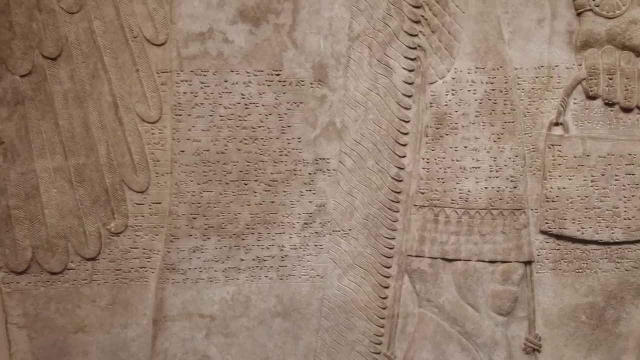 as a middleman, receiving capital goods from the NC and then releasing the goods to the merchants. Generally speaking, payments could either be made directly to the Comptroller or, more often, they were acquired via loans. The documentary evidence shows that loans played a role in the Ur3. 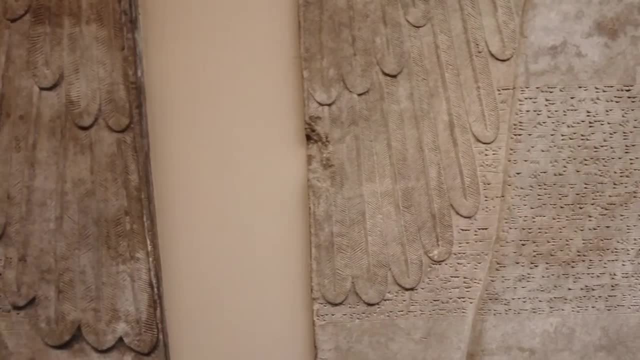 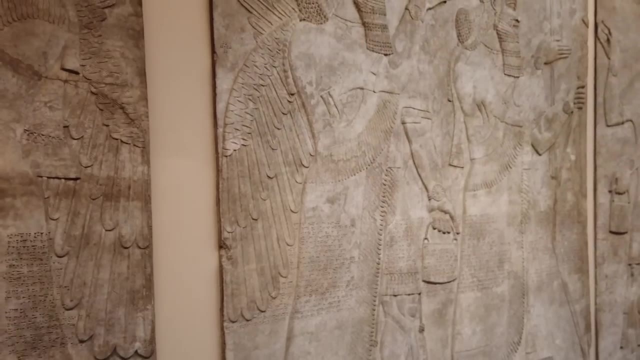 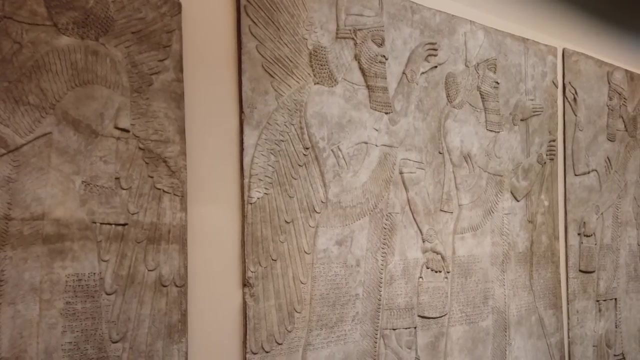 economic system in general and more specifically, with the merchants. Interest free loans were usually issued for a short term duration, often a month, and were usually person to person. Interest free loans were relatively small and often related to the acquisition of domestic goods and tools needed. 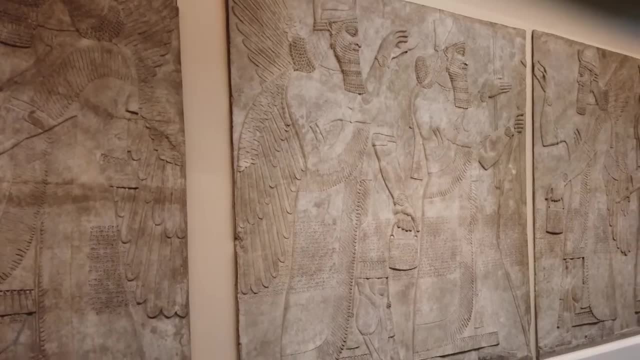 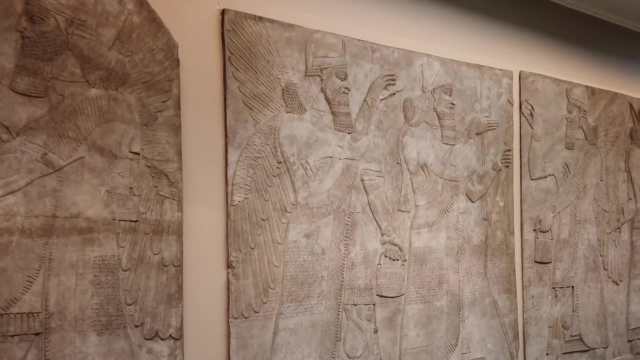 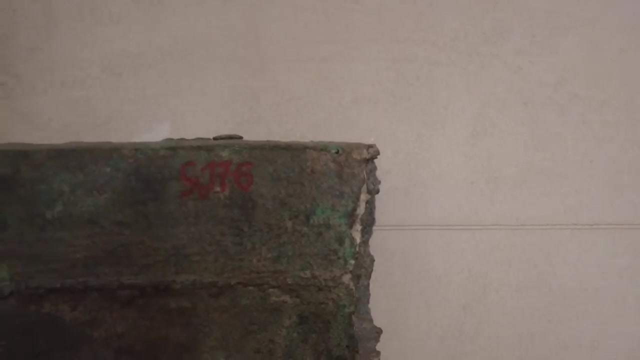 for improvements. Larger loans were granted by merchants to other merchants and were accompanied by interest rates that would make modern credit card companies blush. Silver was loaned at 20% and barley at 33%, with the latter being more expensive because it was in high demand. 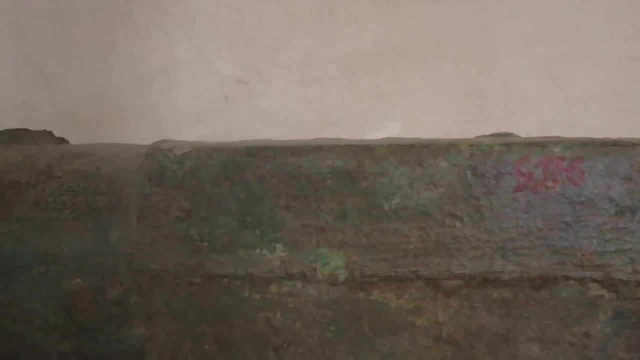 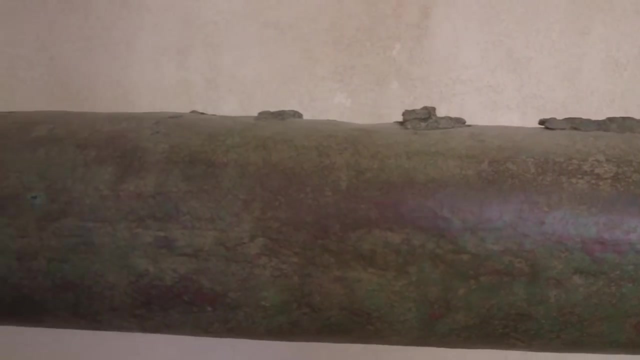 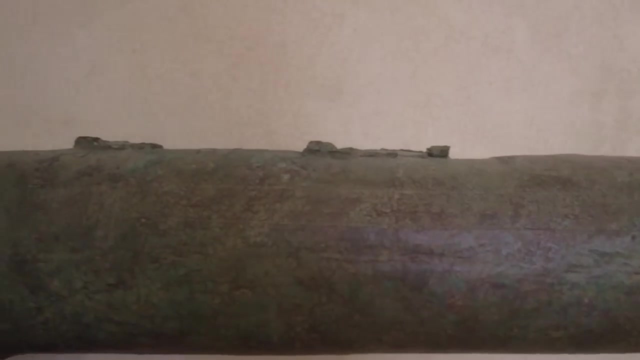 in the same seasons with a larger segment of the population. Merchants may have used silver for their accounts, but the vast majority of the population of Uma have no use for the precious metal. The thousands of silver account documents from Uma reveal that the merchants of the city led active. 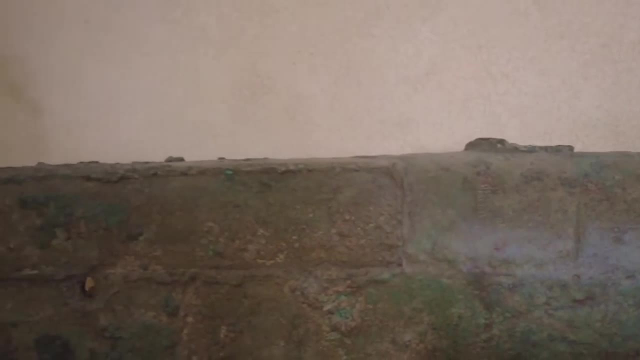 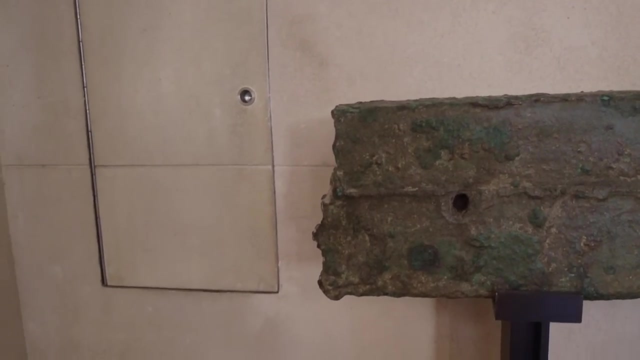 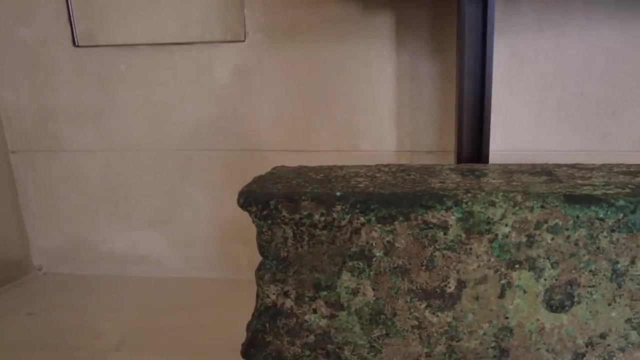 lives that took them great distances away from their city. The Uma silver account documents, as well as documents from other Ur3 cities, reveal that Uma merchants were allowed to travel hundreds of miles in the city to acquire exotic goods. More often, though, the Uma merchants 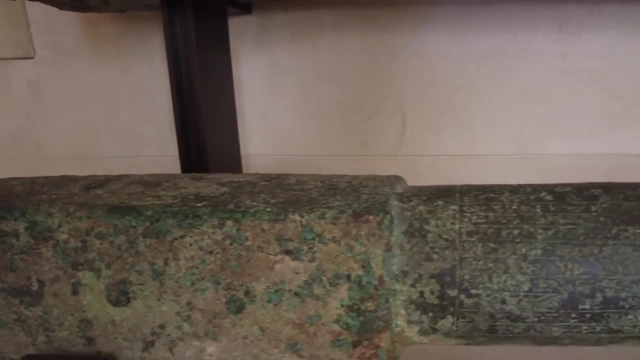 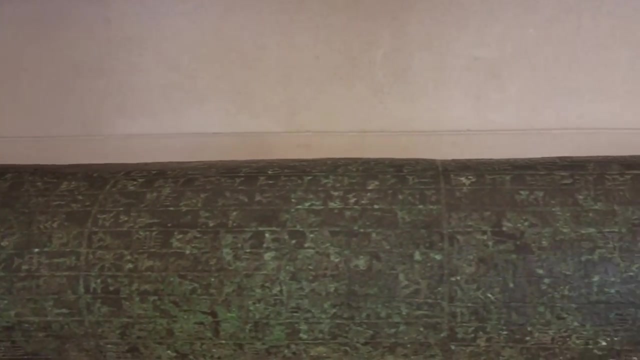 would trade their goods more locally to the villages and towns within the Uma district. The merchants would use donkey caravans to bring some of their goods to market, but because Uma was located in the middle of Mesopotamia, it had access. 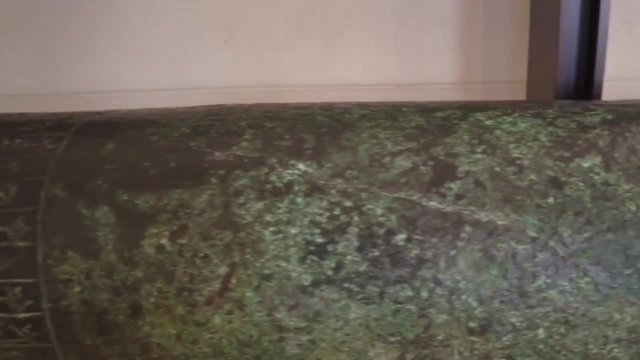 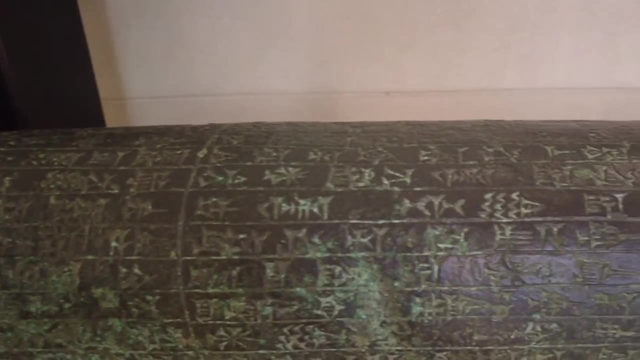 to plenty of canals. Merchants would fill reed boats with domestic goods and travel through the canal system for several hours for a trip that may only be longer trips on the Tigris or Euphrates rivers, bigger and sturdier log. 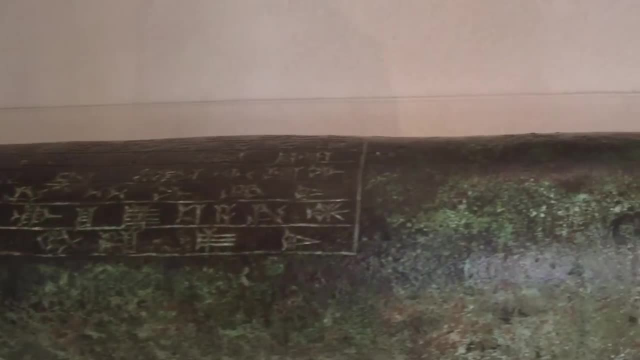 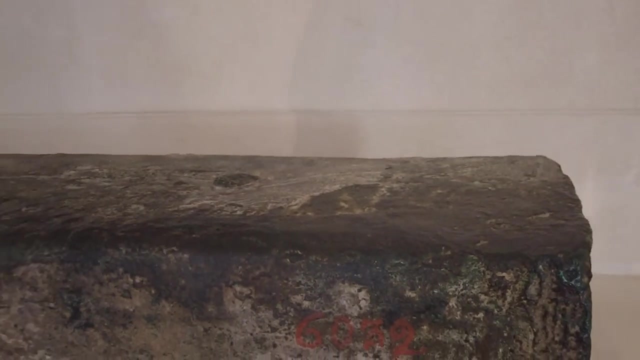 rafts were needed. Once the merchants arrived at their destination, they would unload and meet with their merchant contacts and begin the process of barter. As stated above, silver generally determined the prices of goods, but scarcity and demand also played a role. 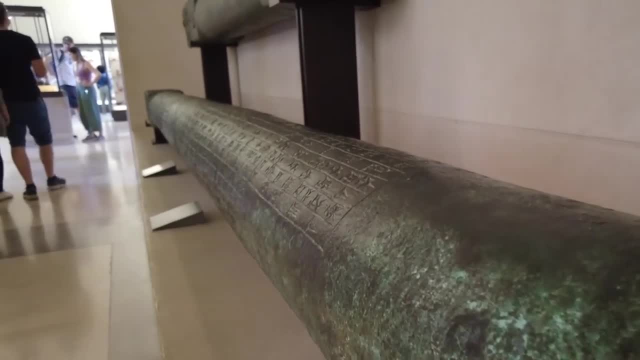 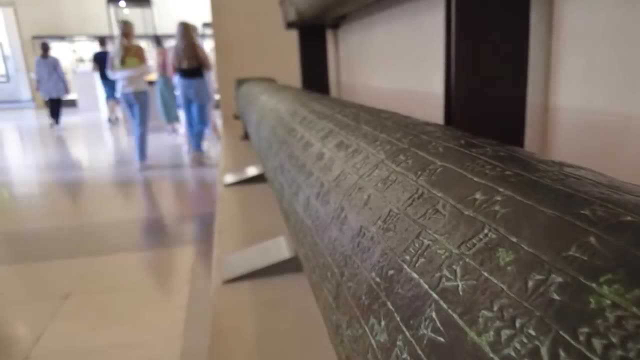 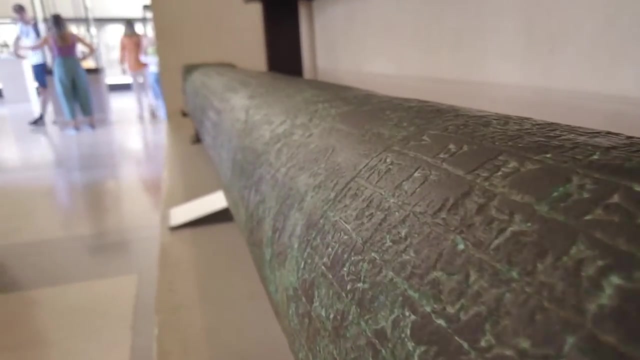 Uma merchants traded several domestic products, including some of the following: Alkalis animal products, honey, bitumen, balsam, fish grail oils and vegetables. The merchants would then bring some of the following exotic goods back to: 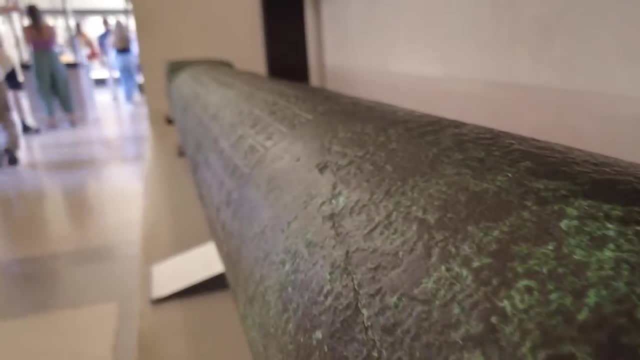 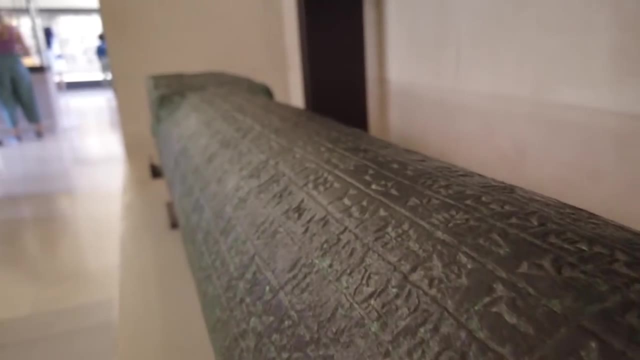 Uma fruits, metals, resins, spices and lumber. The merchants of Uma certainly played an important role in the city's economy, but they were just one class in a somewhat privileged class. The vast majority were peasants who worked the fields that were owned. 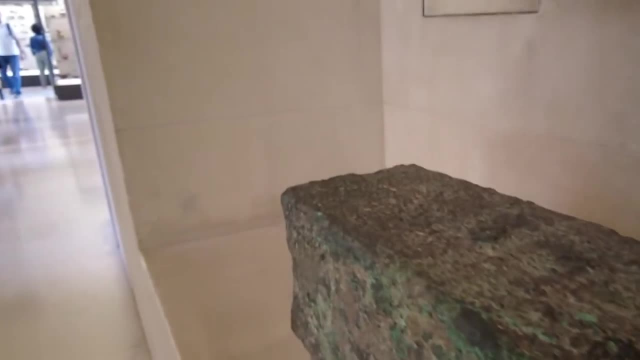 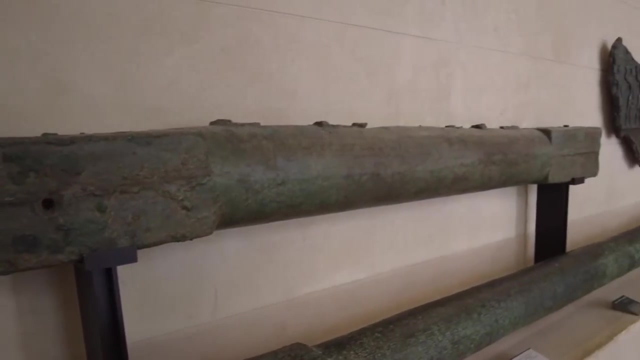 by the royal dynasty or one of the temples. Within the peasantry there were free men and slaves. although the free men had few rights at a modern sense, Free men were protected from assault, theft and other misdeeds. at least they would be theoretically. 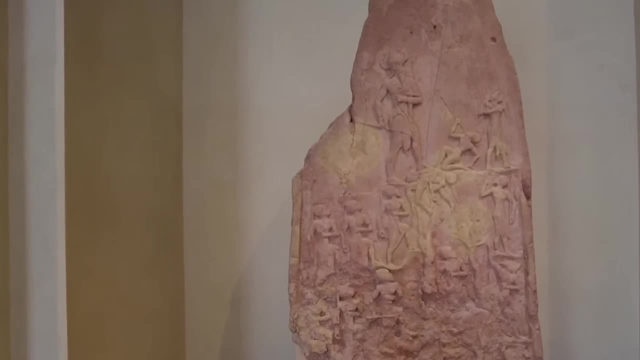 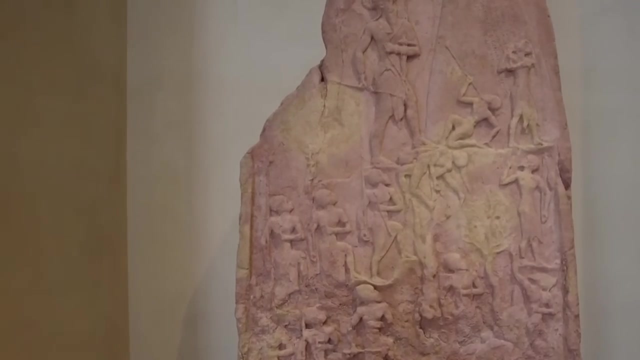 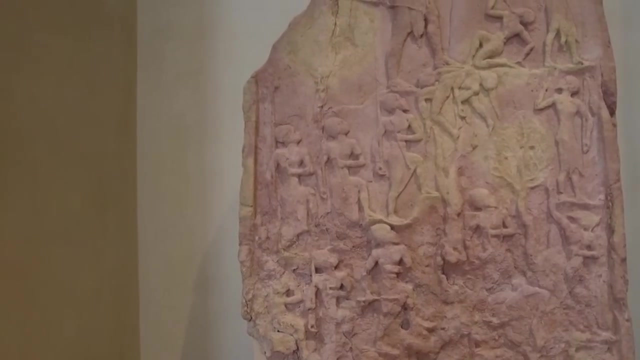 remunerated if wronged, but they were still compelled to work on public works projects along with slaves and conscripted work gangs. Just above the peasants on Uma's social ladder were numerous artisans and skilled and semi-skilled workers, which included shepherds, Thousands. 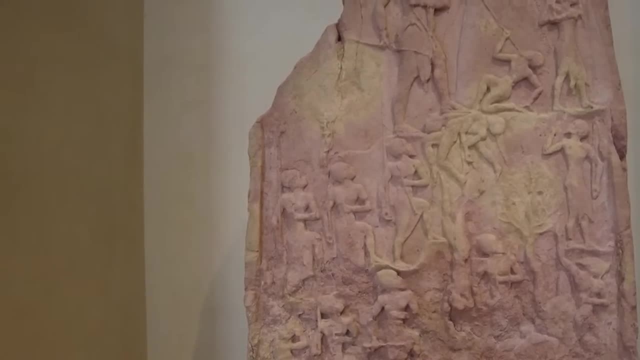 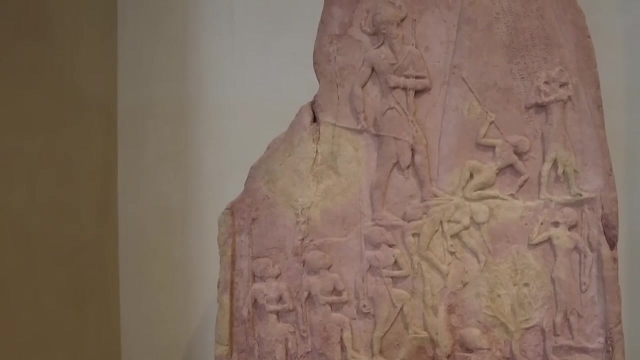 of extant cuneiform tablets relate to the activities of the Uma shepherds. Although the shepherds worked in the agricultural industry, they were a much more privileged class than the peasant farmers. Instead of having to spend their days toiling in the fields to harvest barley. 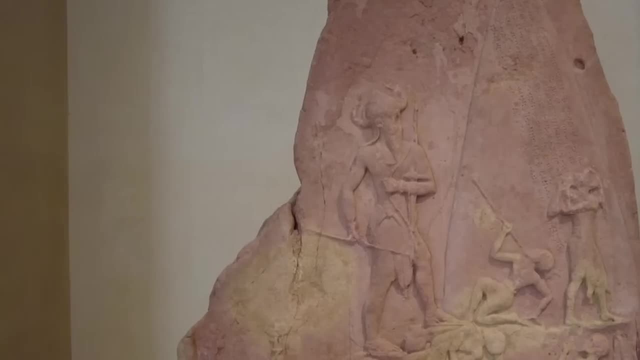 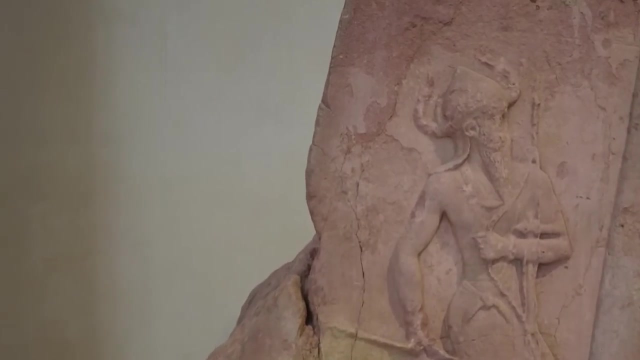 most of which went to the ensi and or the temples. the shepherds enjoyed more freedom and a higher standard of living, mainly because the herds they tended either belonged directly to the state or to one of the many local temples. The records show that 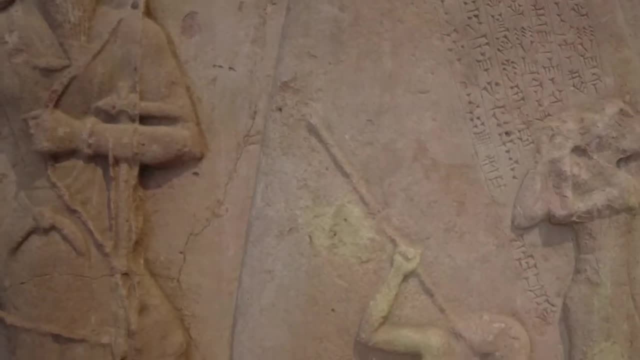 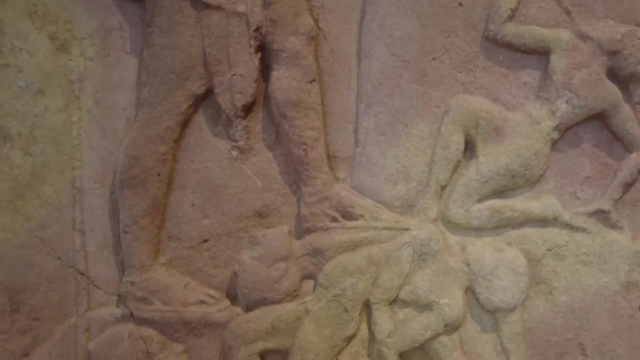 herding was an important and massive operation which involved a certain amount of skill and expertise by the shepherds. Not just any peasant could be a shepherd, as the position was usually hereditary. The shepherds were also literate or semi-literate, as they needed to. 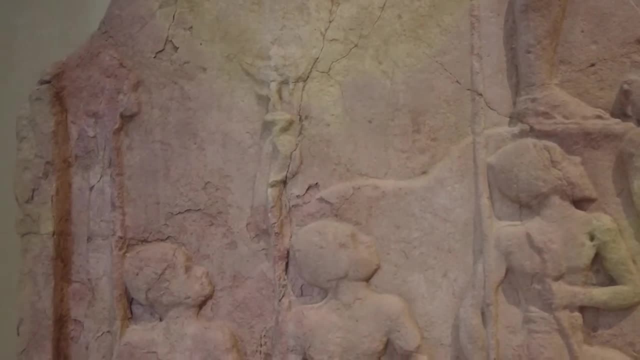 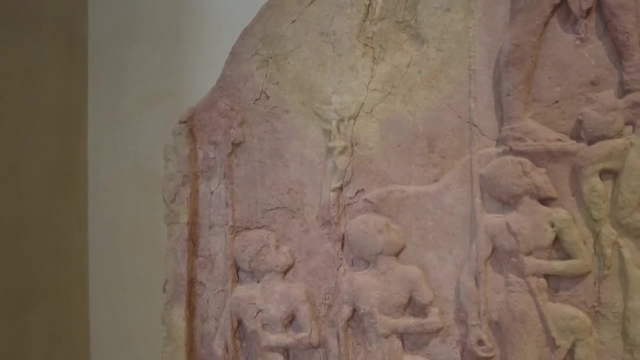 read and write basic business documents. There were as many as 50 shepherds herding up to 10,000 sheep and goats at any one time in Uma. The herd were fed on fields farmed by the peasants with any animal that died. 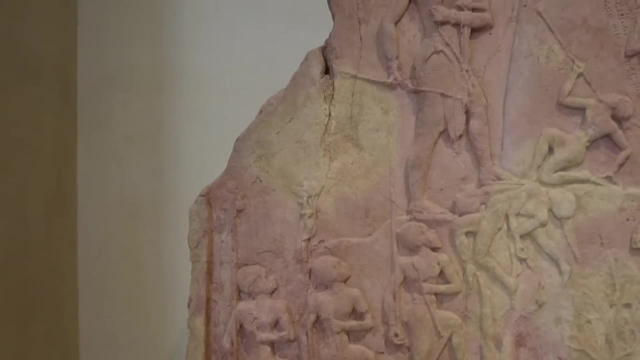 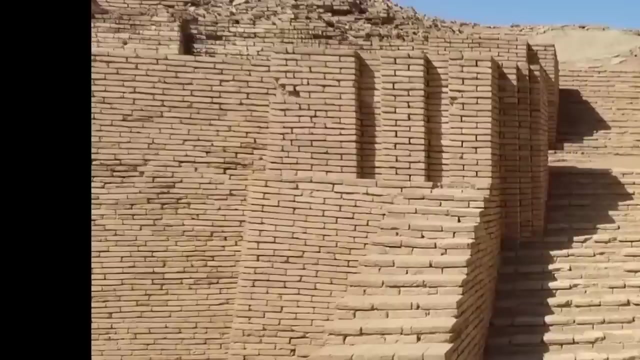 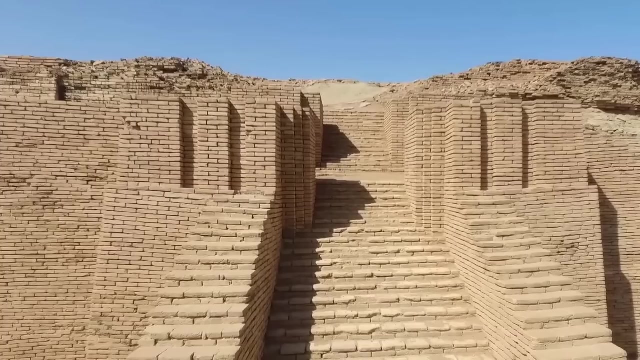 maturingly, being given to the temples for offerings or sold to the peasants. The animals were sheared twice a year for their wool or hair, which was then sent to the markets to drive the Ur III economy. Despite Uma not being properly excavated as of yet, the combination 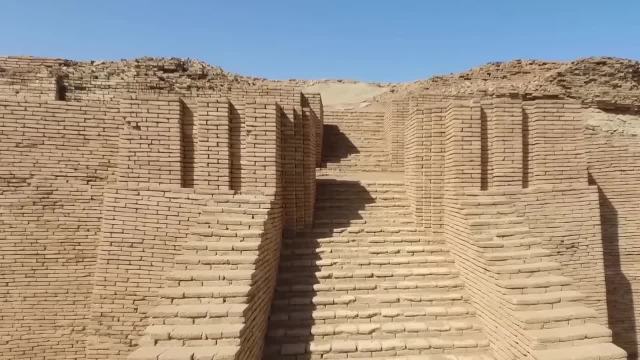 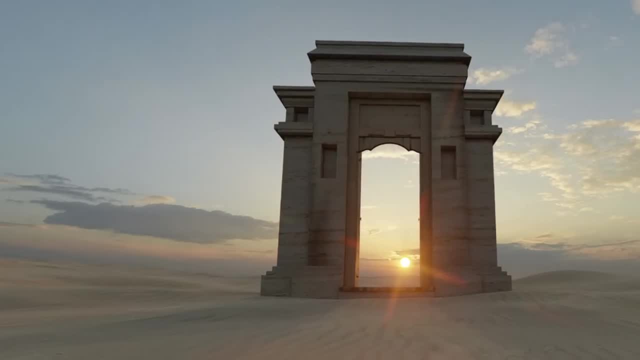 of texts so far examined paints a picture of quite a lively town. in the Ur III period, Canals would have connected the edges of the town with the inner city, bringing water to the peasant farmers and merchants from other points within Mesopotamia, Although it is 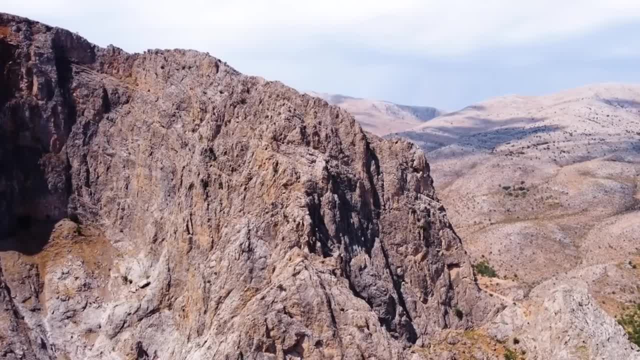 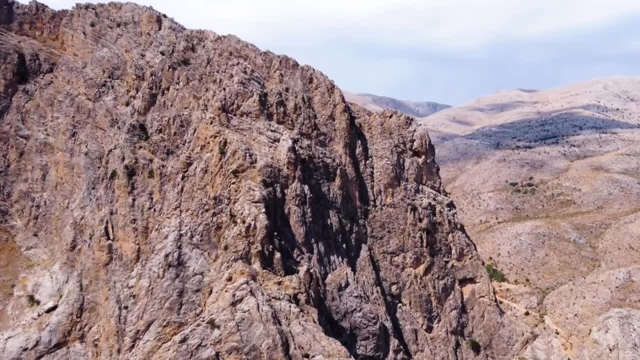 yet to be unearthed. the Shara temple would have been the centerpiece. It may have been a ziggurat structure. as in Ur and other major cities, Priests and scribes could have been seen kneeling around the Shara temple throughout the day. 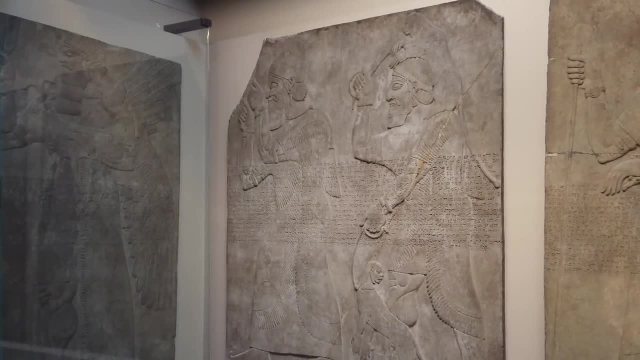 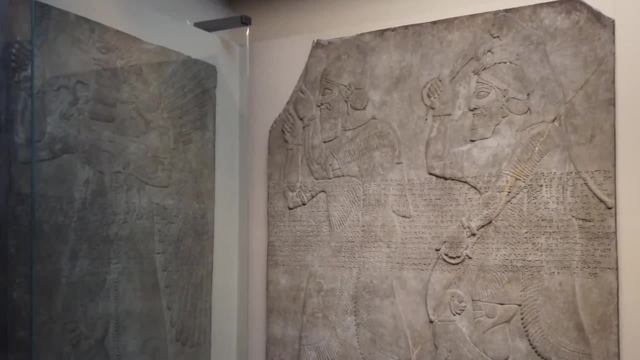 creating important documents and taking them back and forth to the Ensi Bustling with. the most activity would have been Uma's market. After receiving their loans from the comptroller, the merchants would have made their deals in the market for local goods that they could then. 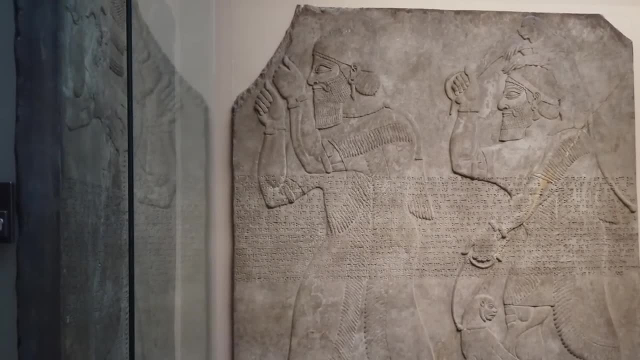 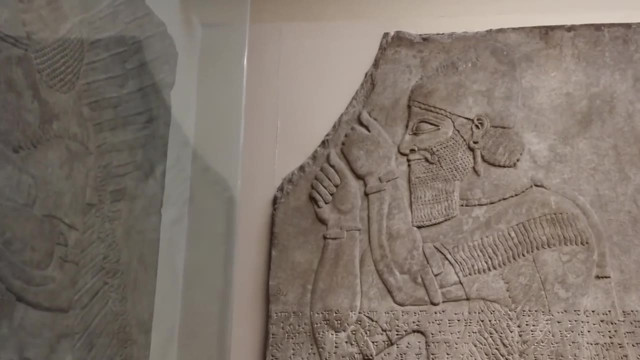 take with them abroad. As some merchants were preparing to leave Uma, others would have arrived with timber, lapis, lazuli and stone for additions to the temple complex. Because Uma has not been properly excavated, it is not known for sure exactly how much. 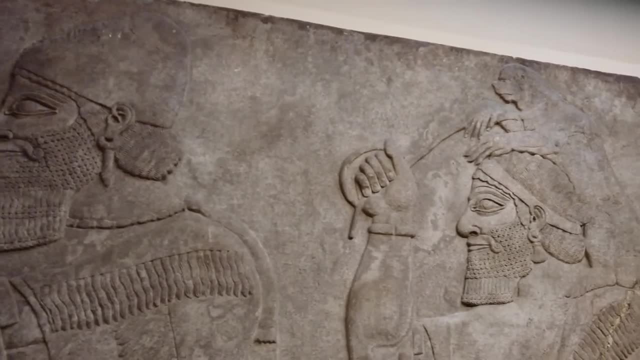 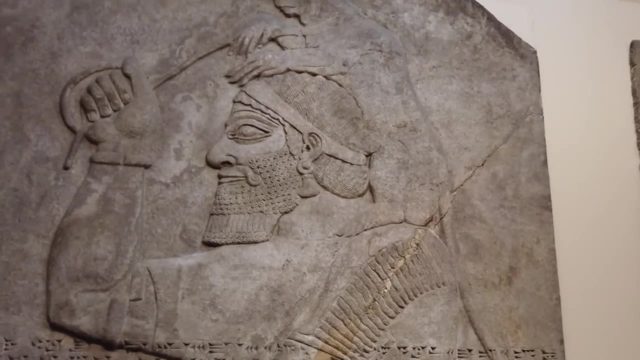 area, Uma, encompassed By the Ur III dynasty. though the district province of Uma, which would have included several smaller towns, villages and rural areas, was quite large, The area to Uma's east and south was much more densely populated. 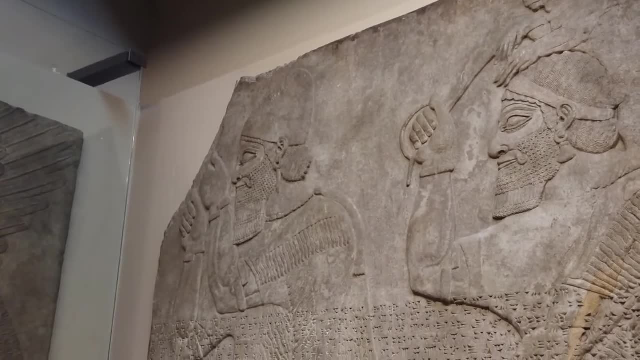 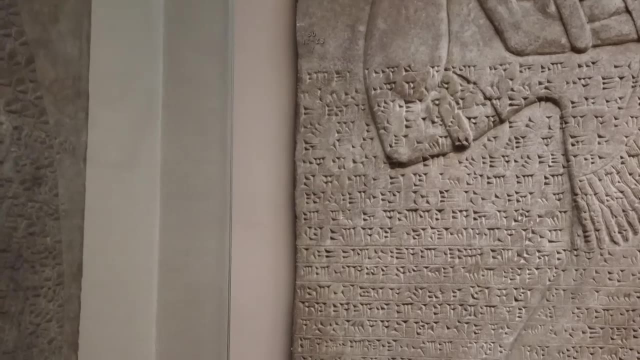 so the city's border probably did not extend far in those directions. The ancient boundary with Lagash was probably intact, although Girsu eclipsed Lagash in importance by the Ur III dynasty. Uruk was about seventy miles to Uma's direct south, and 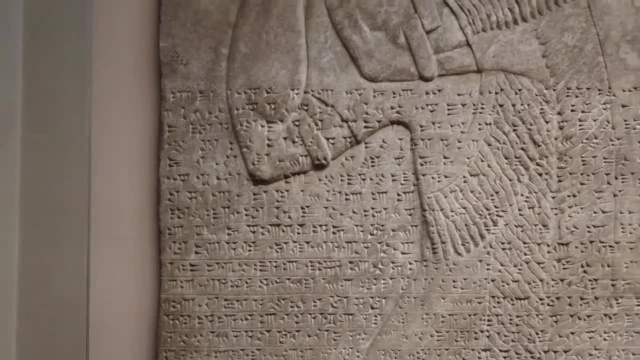 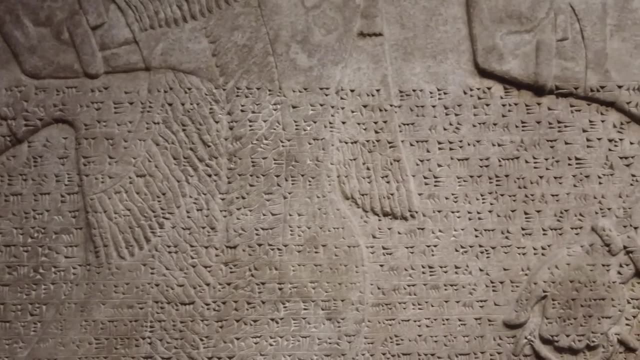 to the southeast were Larsa and other important cities. Since Mesopotamia was less densely populated, the area was more concentrated to Uma's south. Its boundary may have extended all the way to the Tigris River. Based on the limited archaeological 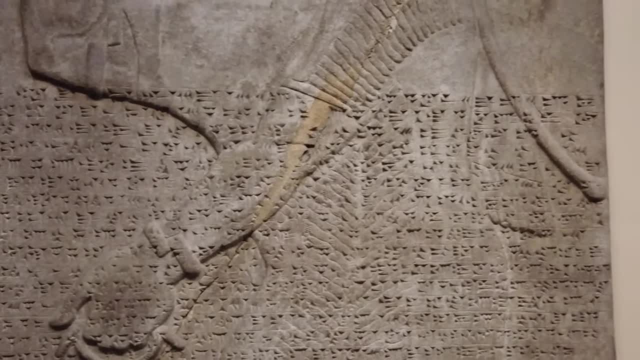 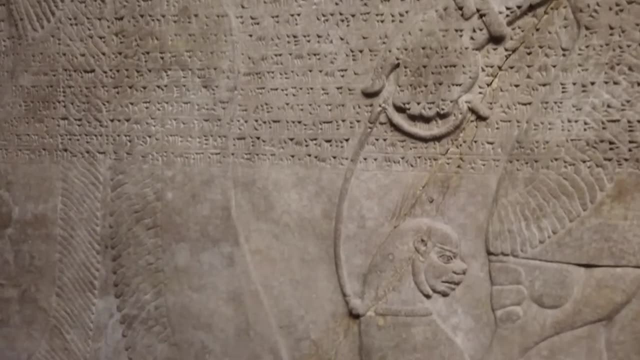 and textual data available, combined with evidence from other Sumerian cities in the Ur III dynasty. some scholars have conducted studies that estimate Uma's size and population. Driel included in his study of Uma's size the town of Apisal and the non-urban. 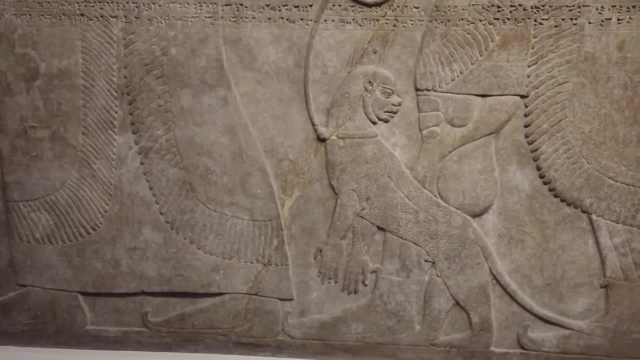 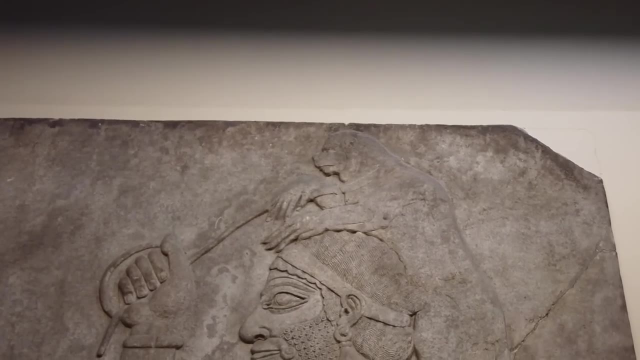 district of Gudina-Mushbiana, among other localities. Since Uma's population in all of the localities that were included in Uma district are unknown, the area included in the study could have been larger or smaller and, as Diel noted previous studies. 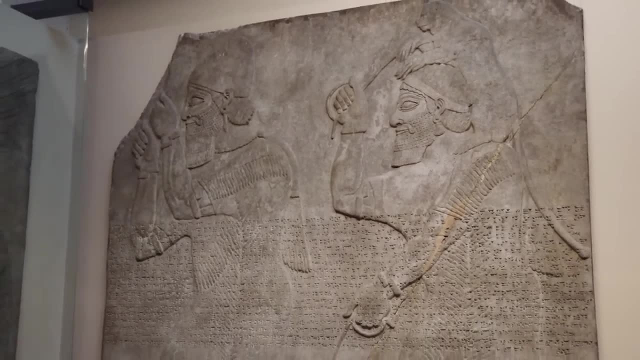 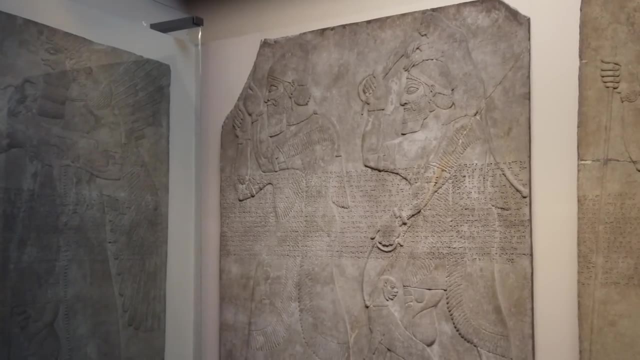 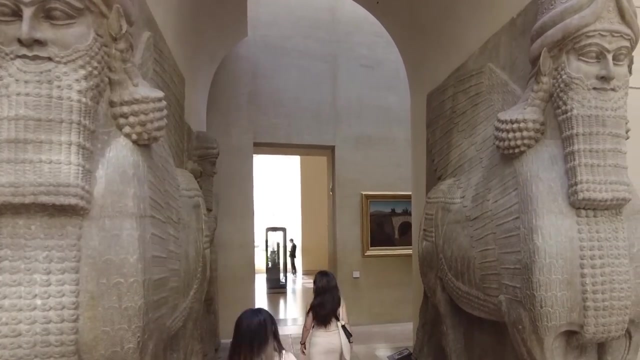 have in fact included varying numbers of localities. It is believed that Uma's sphere of economic influence included more than 700 square miles and 300,000 acres, which, although large, is smaller than Ur and even Lagash. Modern scholars have faced some 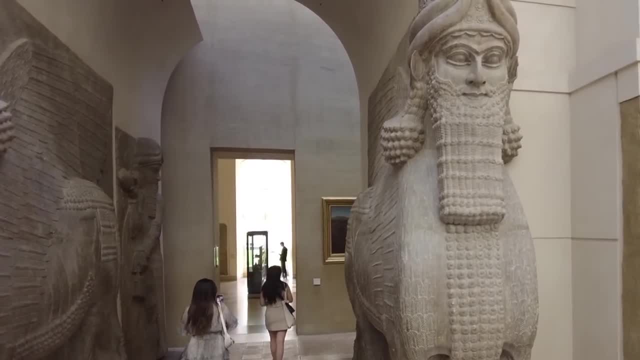 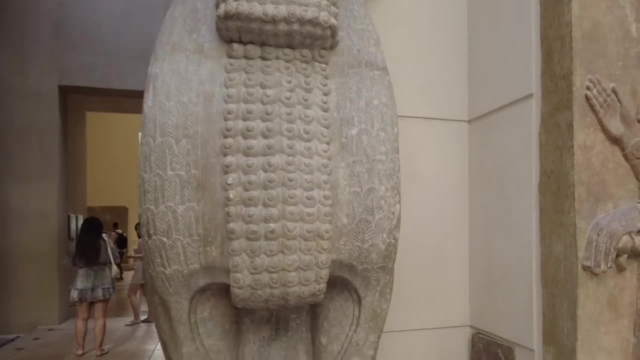 of the same barriers when attempting to estimate the population of Ur III Uma. Again, estimates are based on a combination of texts and guesses about the physical size of the city and the region, But because it is not known for sure, this can result in a wide range. 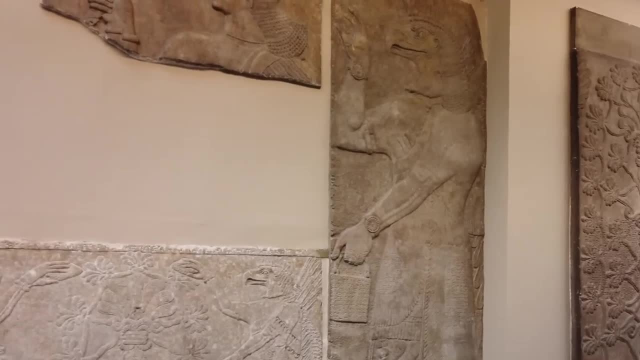 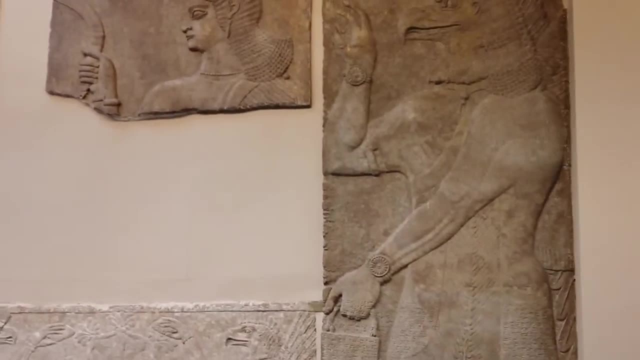 of approximations, Adams believes that Uma's population was at least 20,000 people, although his study was not directly concerned with Uma's size. Driel considered a number of previous studies, but based his conclusions on the number of plow teams associated. 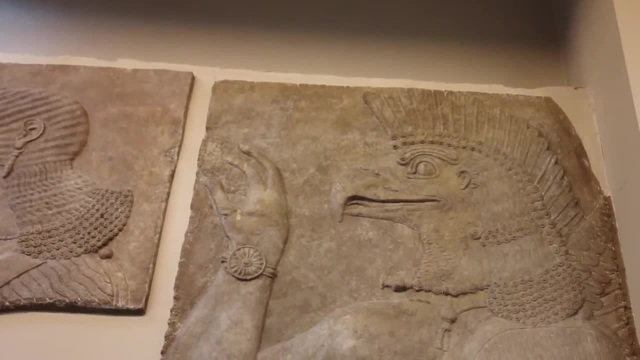 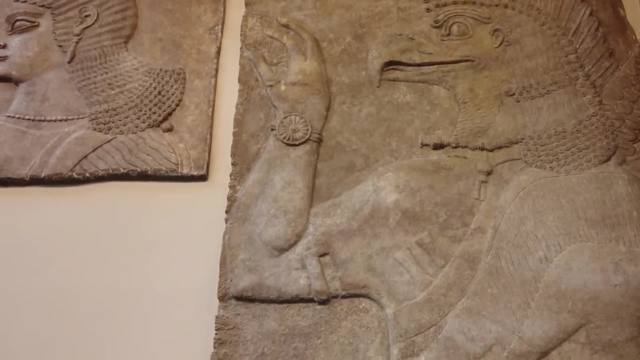 with the city and number of people they could feed. he concluded that there were about 200 plow teams in Ur III Uma and that yield rate at the time was 1 to 10, which would indicate that the population was near Adams' estimate. 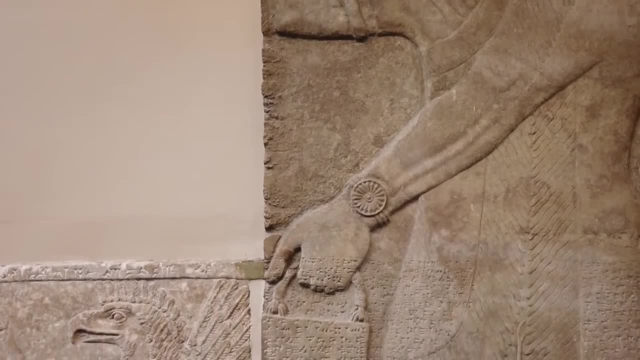 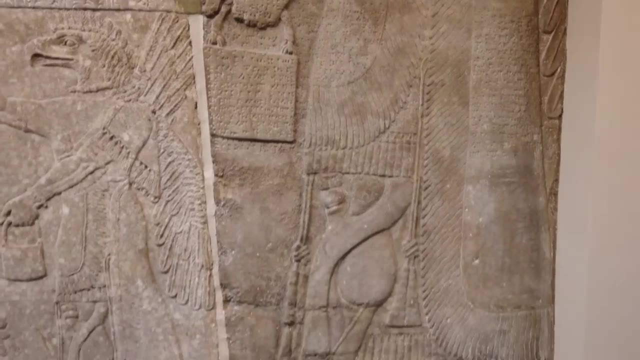 although the size of the province remains even more questionable. Regardless of the exact numbers, there is little doubt that Uma was one of the most important Ur III cities. It may not have been as large as Ur, Larsa, Girsu and Lagash, but there is no doubt. 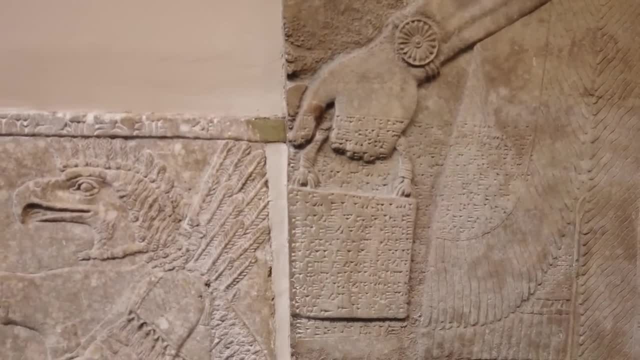 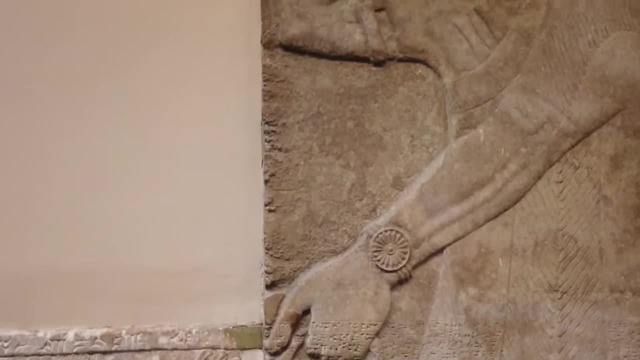 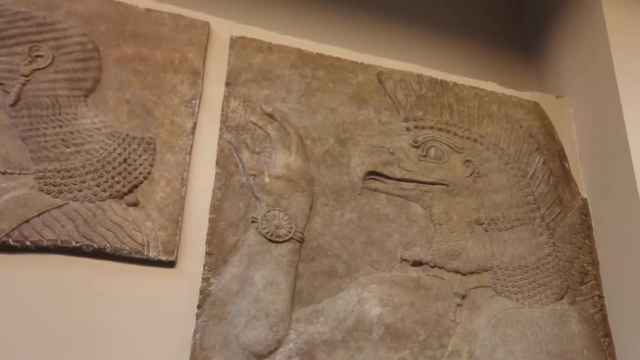 that it was an important economic and religious regional hub. Ultimately, Uma's prospects were intertwined with the success of the Ur III dynasty. When the Ur kings were powerful, Uma prospered, But when tragedy struck Ur, it also directly affected Uma, As the merchants of Uma reaped the 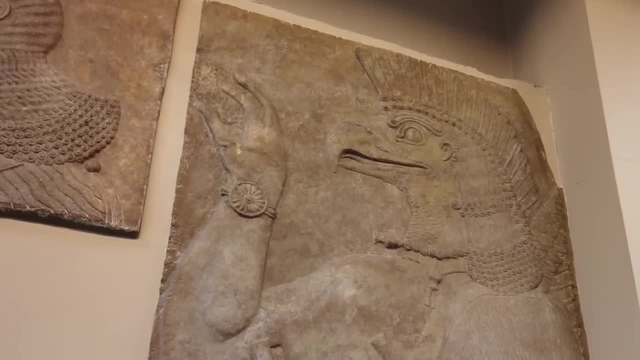 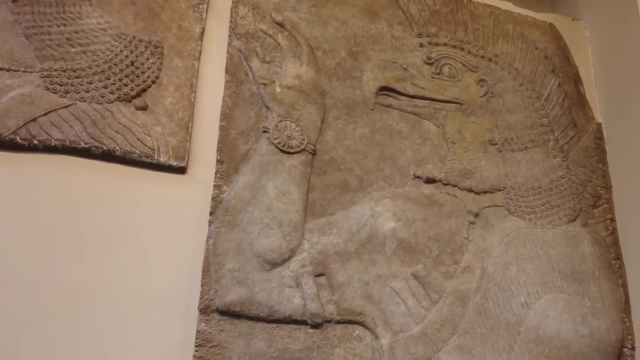 benefits of their far-flung trade and brought products to the city's markets and temples. it probably seemed as if the Golden Age would never end, But within the span of a few hundred years, everything quickly collapsed and Uma was reduced to ruins. 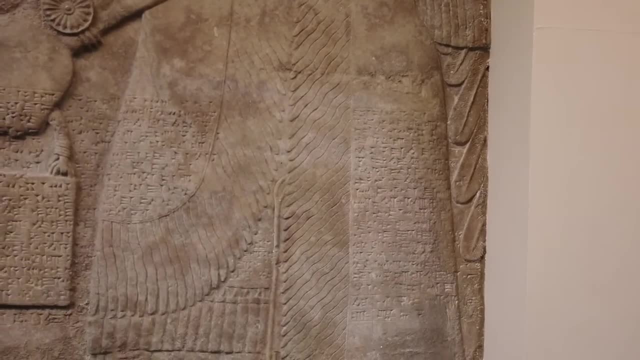 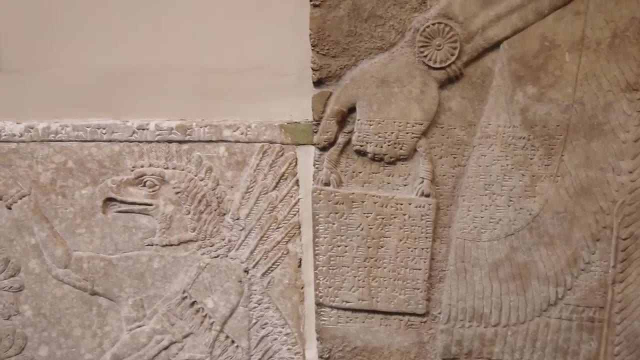 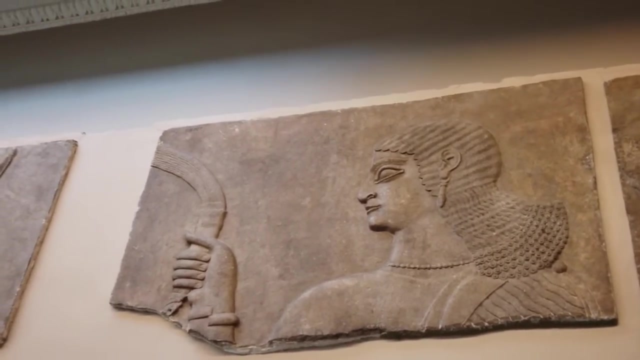 The Ur III dynasty was the largest and most successful Mesopotamian dynasty up to this point in time. Its kings were able to wrangle the disparate groups of Mesopotamia under one dynasty for a period of just over 100 years, and they were able. 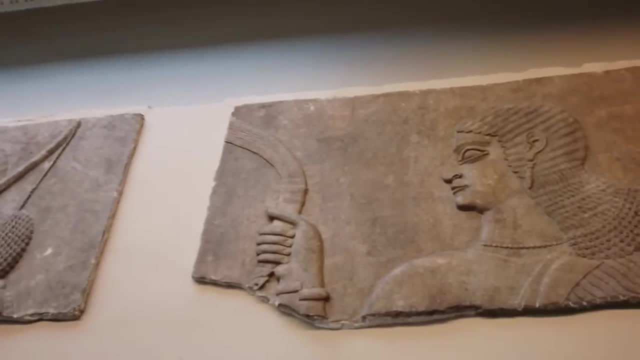 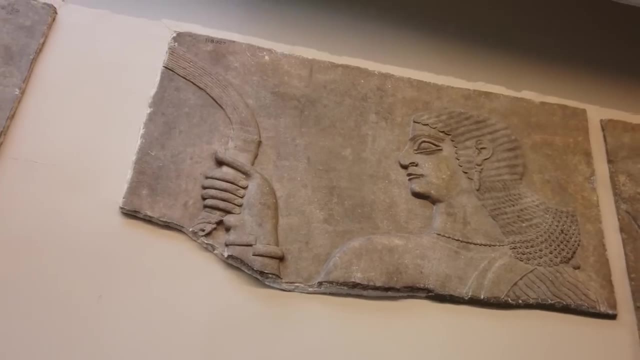 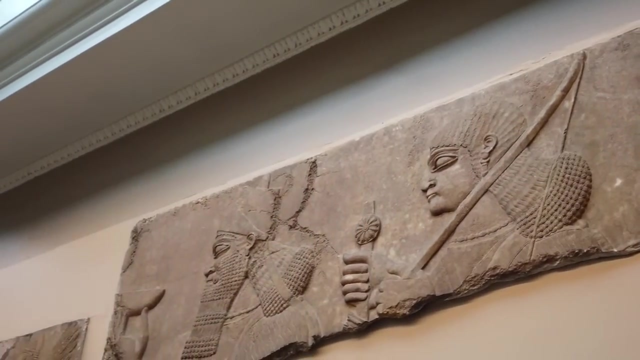 to do so primarily through diplomatic rather than military means. The Ur III dynasty was a confederation of city-states and provinces that were tied together through a combination of cultural affinity and economic progress. But when those bonds began to fray, especially the economic ties, then the empire quickly unraveled By the reign of the last Ur III. king Ibisen reigned 2028 to 2004 BCE. regional provinces such as Uma began to assert their independence through their merchant activities. The merchants of Uma and other Sumerian cities began operating. 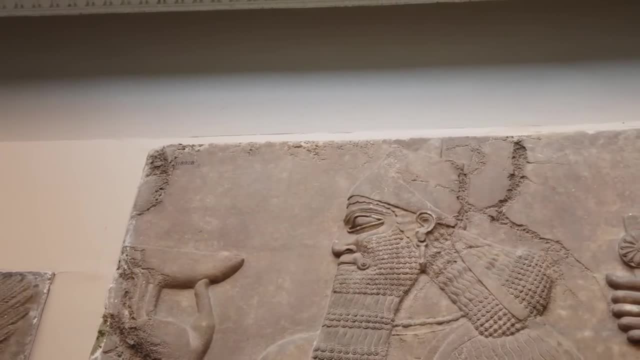 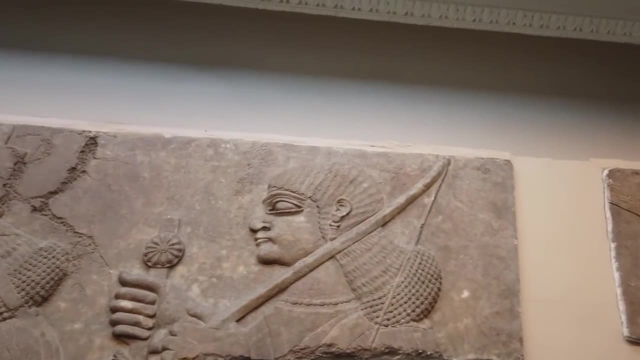 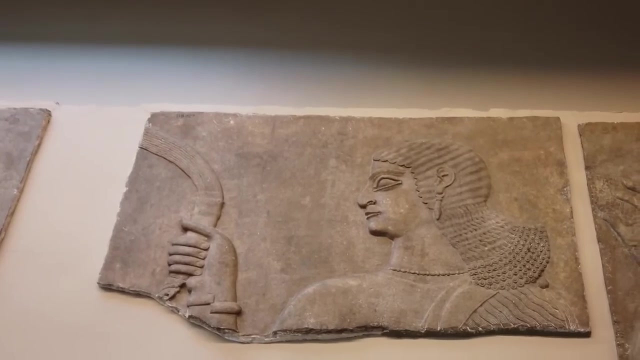 independently of Ur, sometimes even trading with Ur's enemies. Perhaps somewhat surprising is the fact that the decline of Ur and Uma is fairly well documented. Things got so bad late in Ibisen's rule that many of the more important provinces, such as Uma, quit paying their taxes. 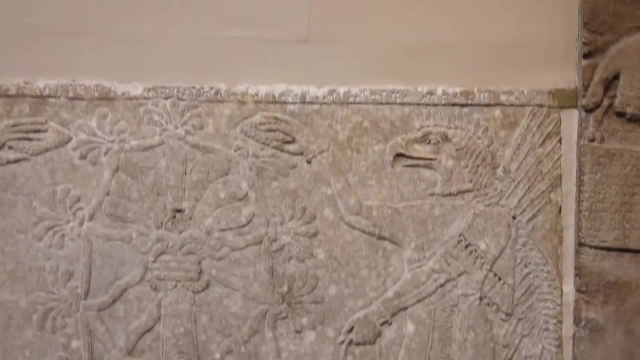 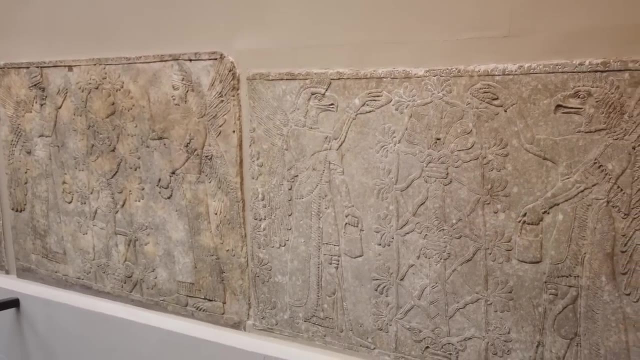 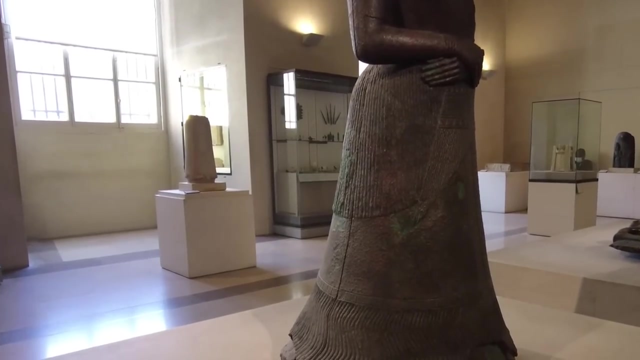 to Ur and their scribes quit dating documents, which was effectively a proclamation of their independence. The final coup de grace came when the Elamites invaded and plundered Ur around the year 2000 BCE. But if the Ensi and merchants thought they would be, 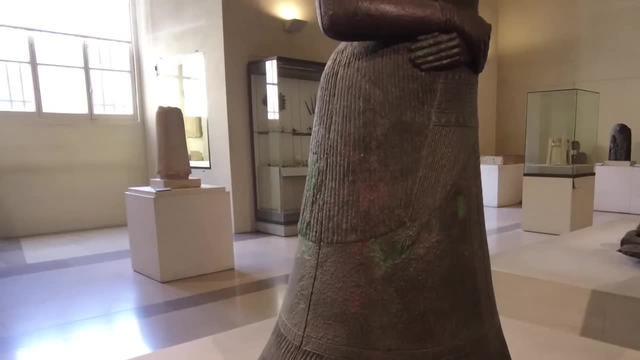 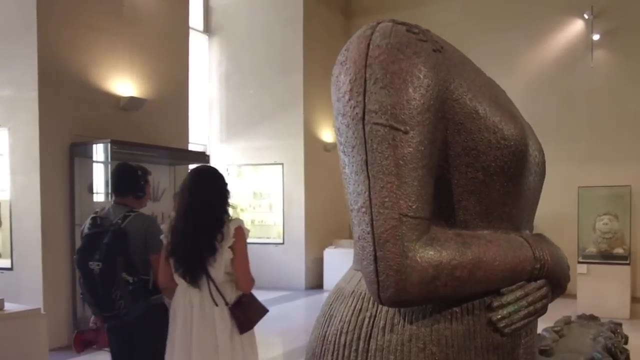 spared because they were involved in business with the Elamites. they were sorely mistaken. All of Sumer was sacked and looted by the Elamites, which was documented in the pseudo-historical Sumerian text known as the Lamentation of Ur. 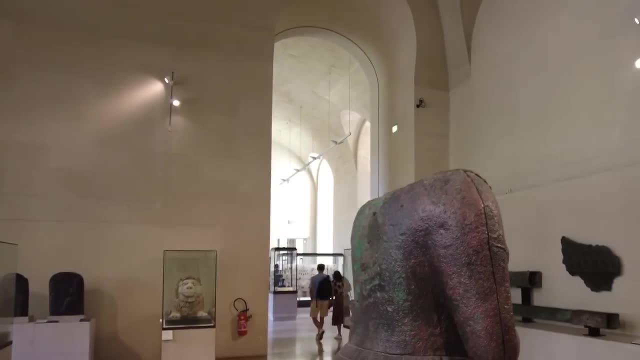 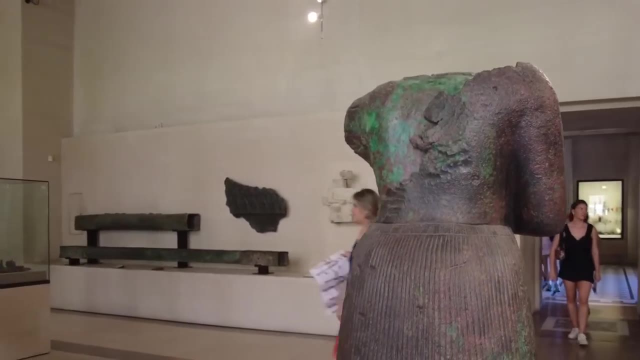 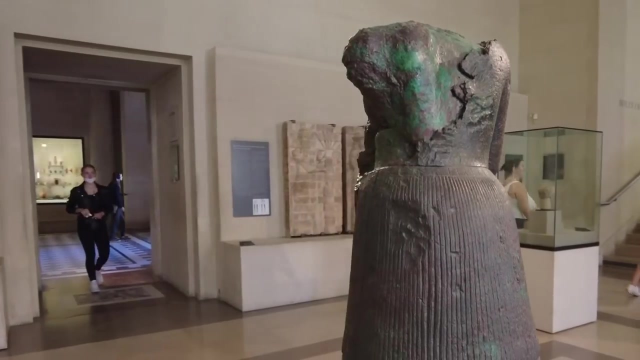 The text notes that Uma and Girsu, once rivals, were equally devastated. In Uma, a bitter storm blew over Sigursag. Shara forsook Ima his lofty dwelling place. Ninguln wept bitter tears in her destroyed city. 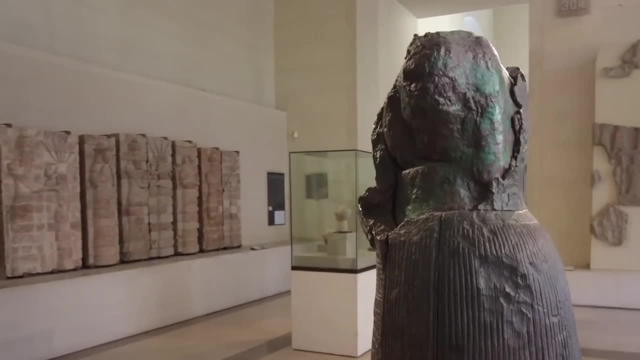 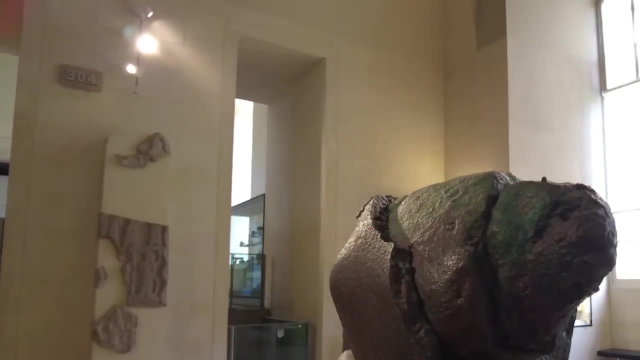 On my house, whose riches have not been returned. bitterly she cried. Girsu, the city of heroes, was turned into a cowardly place. Ningirsu forsook the Enninu. Mother Bao wept bitter tears in her house, Urukug. 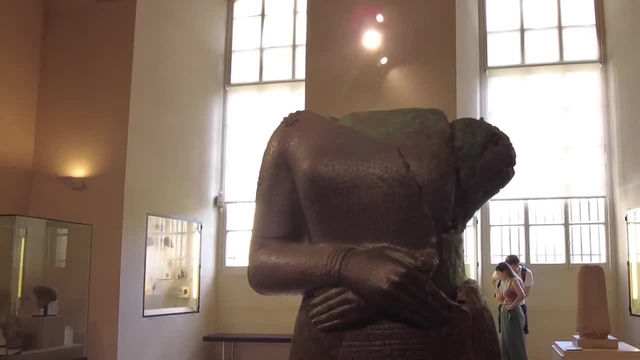 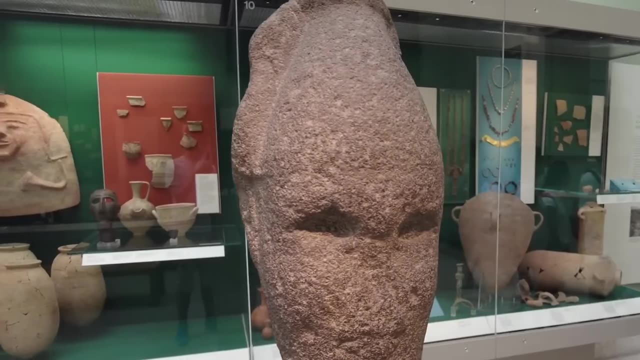 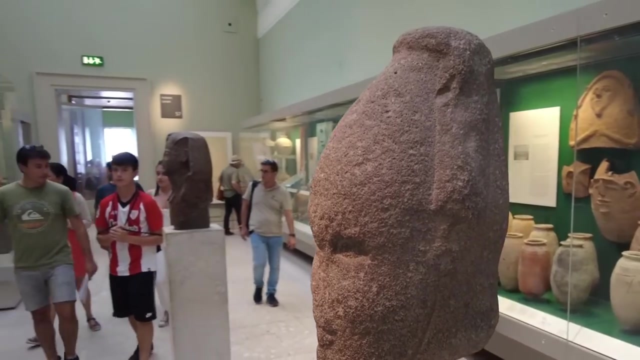 Oh, my destroyed city, Destroyed house. Bitterly she cried. Another version of the Lamentation tells a similar story. Shara has abandoned the Ima. His sheepfold has been delivered to the wind. Usahara has abandoned her house, Uma.